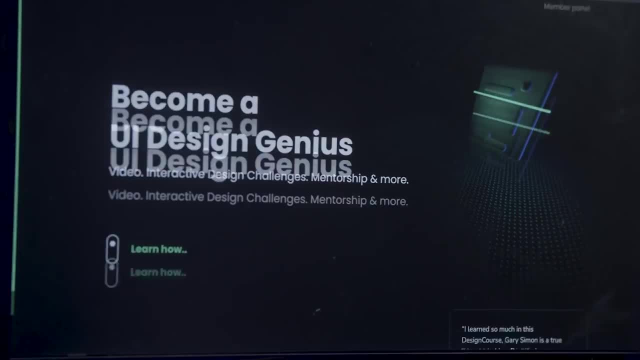 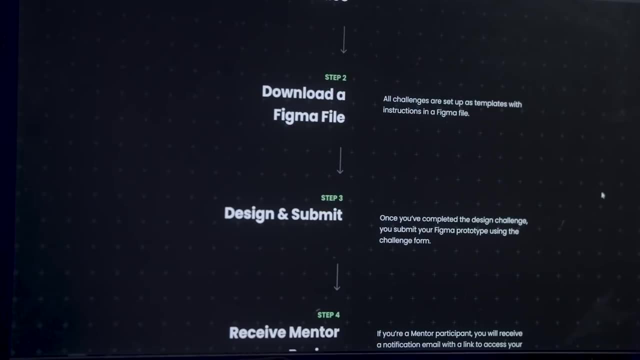 the description, and if you're interested in learning more about how to design great-looking websites, that's also currently available at designcoursecom. Again, look in the YouTube description for that, and I'll shut up now and let's get started. All right, so let's go ahead. 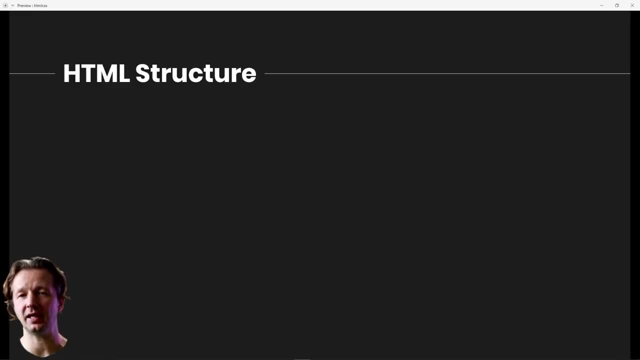 and get the obvious out of the way. I am a floating head today and that's because I just chose to wear a green shirt- a hit record- and here I am- a green- rather a lack of a green shirt- and a 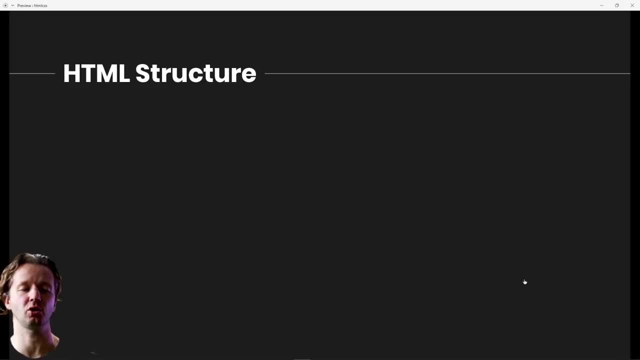 floating head. So, anyhow, I'm going to get started, So let's get started. So let's get started, So let's get started. here We're going to talk about our HTML structure. This is just a few slides to make this go real quick. This is just going to be real fast. I like to get our hands dirty. I don't. 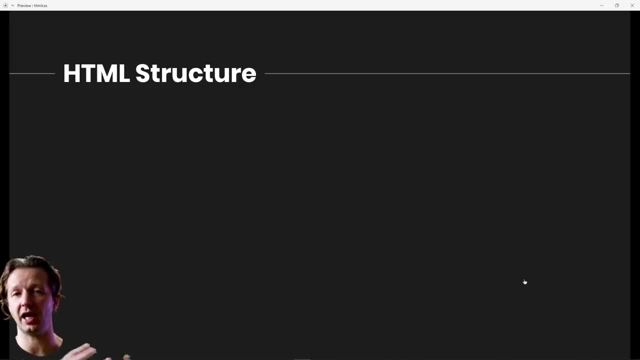 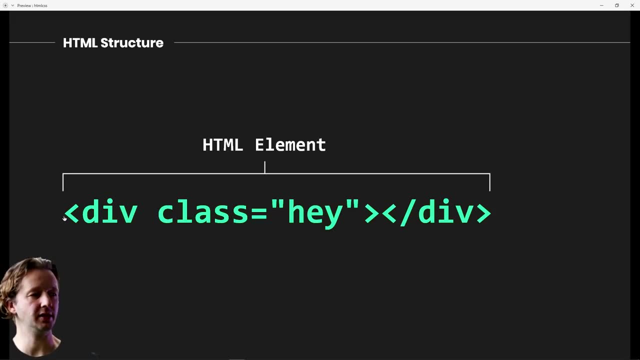 like to do this theory stuff, but it would make sense real quickly to talk about HTML and CSS structure and how, overall, it is structured. So first, this is an HTML element, basically, and this is how most of them look In the context of a full webpage. 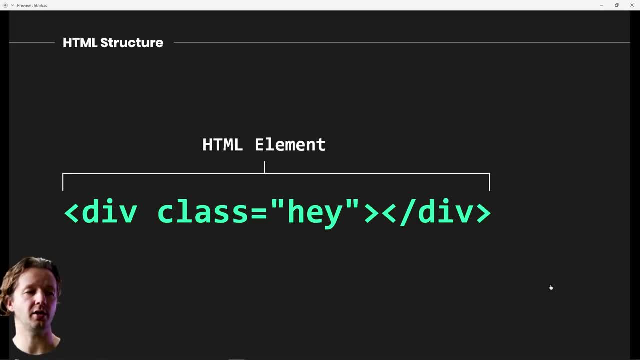 you're going to have a lot of HTML elements, and you're going to have a lot of HTML elements and you're going to have possibly hundreds of these and you can nest them inside of each other and do all this cool stuff. So let's break this down. So first we have what's called the opening. 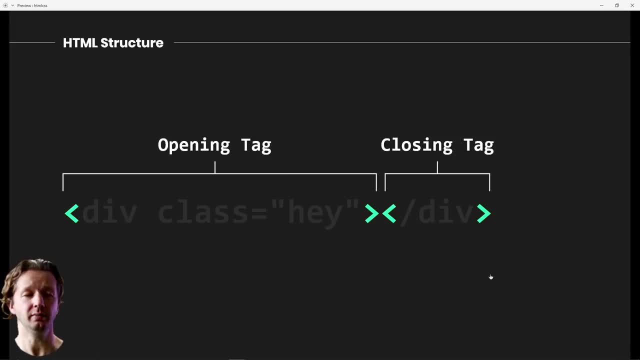 tag and the closing tag. Now, some HTML elements are self-closing, In other words, they don't have this little ending portion right here and it would essentially just be this opening portion. but most of them, most of the time you're writing HTML elements, they're going to have an opening. 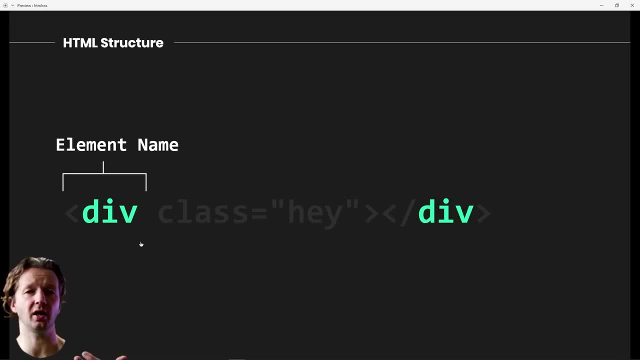 tag and a closing tag. Next up, the HTML elements are going to have a lot of HTML elements, and next up, the HTML element name is defined right after this less than sign, And so this one's called div. There are many, many, many others, dozens, if not over a hundred. After that we have 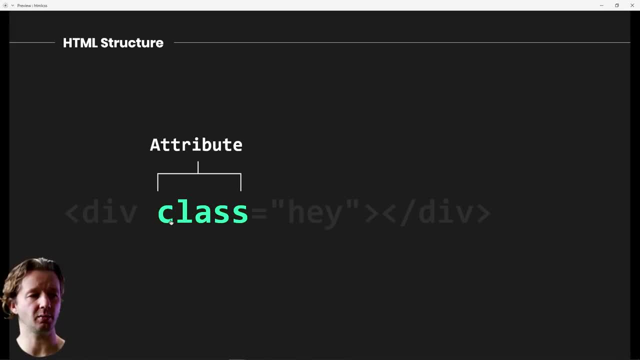 the attribute. So inside of an HTML element sometimes you can have attributes and sometimes you don't have to. Class is an example of one of the many attributes that you can use. Now, some attributes allow you to specify, or most rather a value of some sort. All right, So in this case it's hey, It's whatever you want. 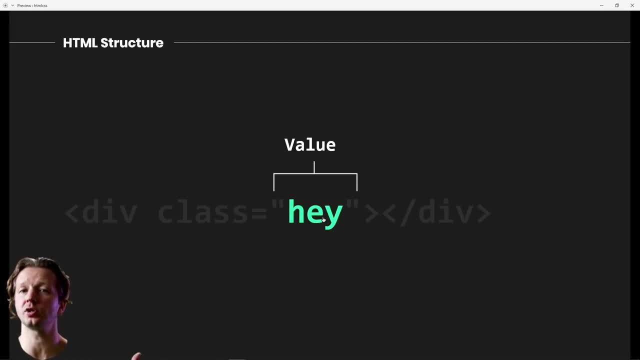 to make it and it's how you can reference it in both JavaScript and CSS in order to style it Now right here. sometimes, and I'd say most of the time, you have content between the opening and closing tag of your HTML document. All right, Now let's say, for instance, we're talking about 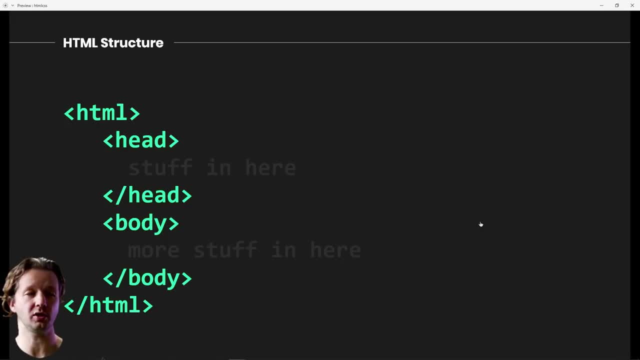 a whole HTML document itself, like indexhtml, which you may have seen Or may not have. This is the overall structure of an HTML document, So you have the opening HTML tag here and the closing. So that's always going to be your first line and then your very top line. 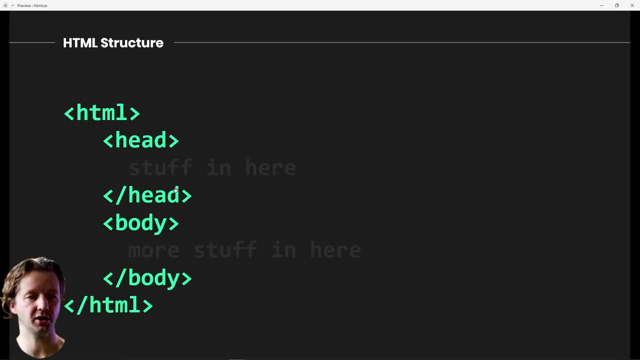 And then inside we have two major areas. You have the head section and you have stuff in here, And the stuff in here is really just configuration stuff. So, for instance, the top of the browser, there might be a little title there. You specify tags in there, the title tag. You also. 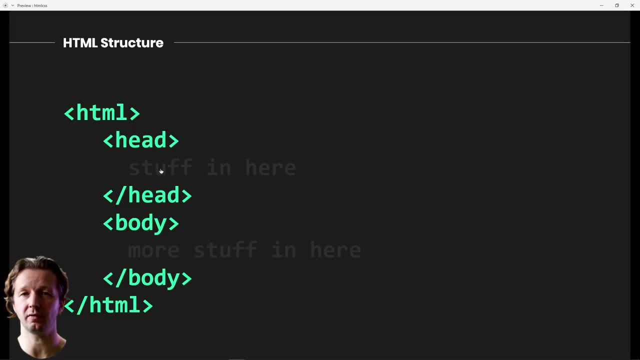 have meta tags for the search engine, stuff like keywords and the description that shows up in the Google search results. You also have an area where you can specify or link a CSS document that helps you style the stuff that's down here. So then you have the body element and inside of the body, 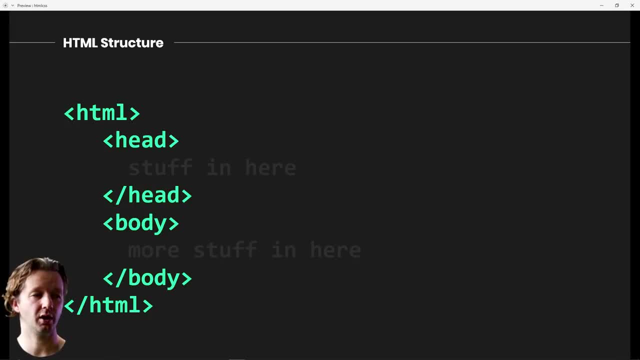 element. that's where you're going to be working most of the time. So this is where almost pretty much all of your HTML elements and those tags is going to be within the body tag. Whatever is within the body tag is what actually shows up in the browser on your desktop computers. 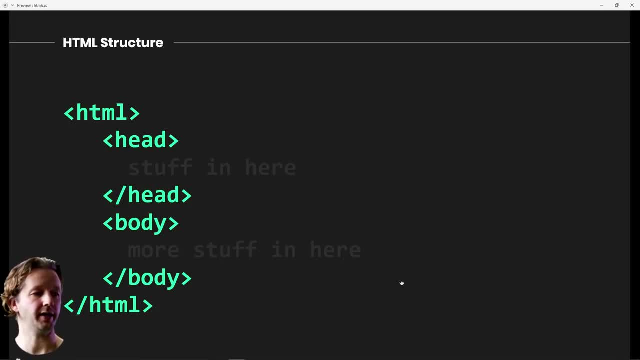 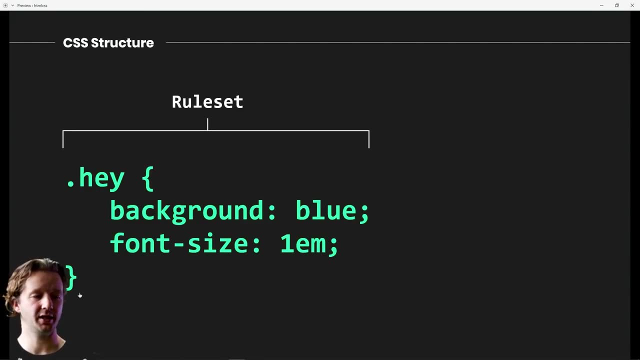 and also on your phones and stuff like this. All right, So let's talk about CSS structure now. So this here is what CSS essentially looks like, And this overall right here is a rule set. In a big example where you have a full website, you may have hundreds of these rule sets. 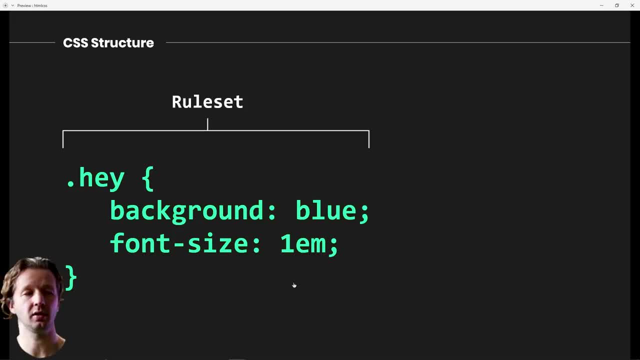 just different rule sets to style different parts of that website. So you may have hundreds of these rule sets to style different parts of that HTML document. All right, So CSS, by the way, is nothing without HTML If you don't have the body element or any of the stuff that's inside of the body. 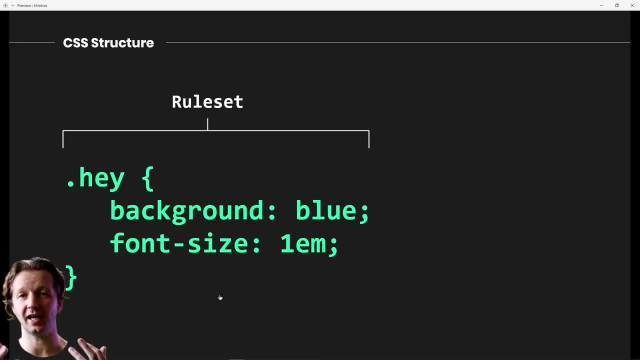 element, then CSS means nothing. HTML is the skeleton of your body and CSS is the flesh. All right, It's how you configure the appearance of HTML, And I'll show you what HTML looks like without CSS, and it just sucks, right. It would be really weird if we saw a bunch of humans walking. 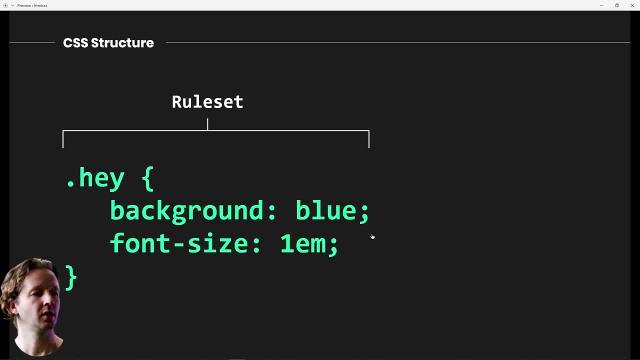 around with just skeletons, right? So think of it like that, All right. So this is a rule set, this whole thing, right here, this whole block. So let's break that down, All right. So the first part of this rule set: it's called the selector. There are several ways that you can create. 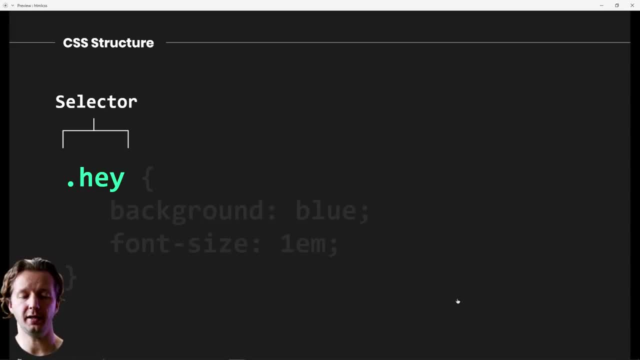 selectors, but basically what it's saying is all right in the HTML document and the HTML elements that we're looking at. which element are we trying to style? All right, It's that tag name. So in this case, notice how there's a. 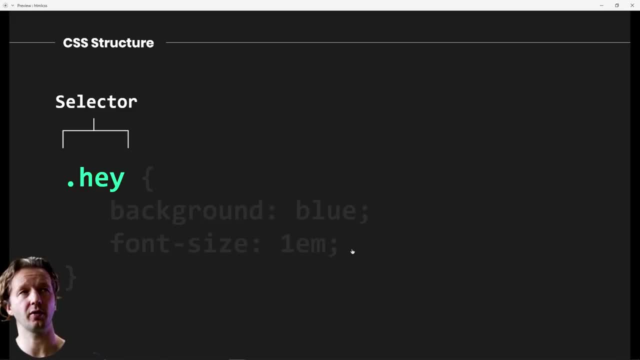 period. and then it says: hey Well, in our previous example, when we were going over HTML, we had this right here. Well, if you're trying to reference this element and you're trying to style it like, give it a background of blue and make it a font size of one M unit, well, 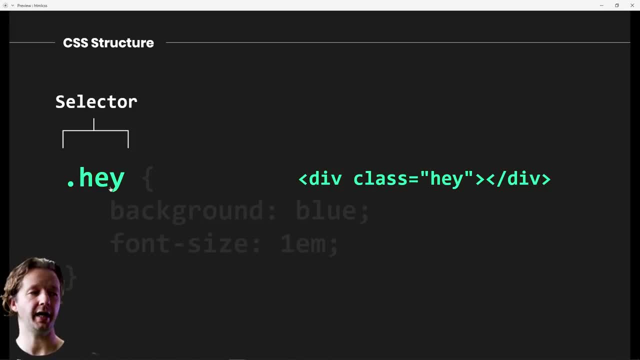 then you would say: if you're referencing a class period, hey, So the period means a class. So, by the way, if you're not sure what the class attribute means- a lot of this stuff I'm kind of glossing through pretty fast. but just to give this a definition, let's say you have multiple 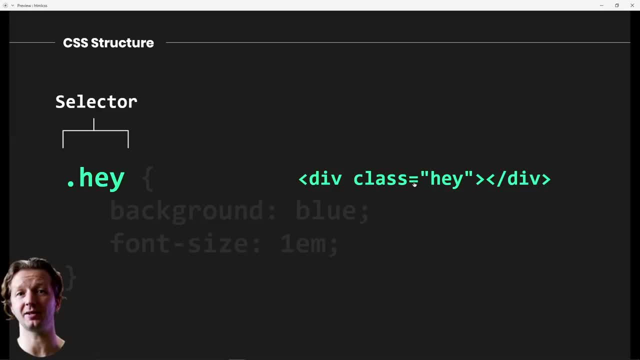 elements in your HTML document and then you're trying to style it. Well, if you're trying to style your HTML document, that you want to style something about them similarly, you give them a class, and this is one of the use cases. Now you could also, as a selector, just choose div. You. 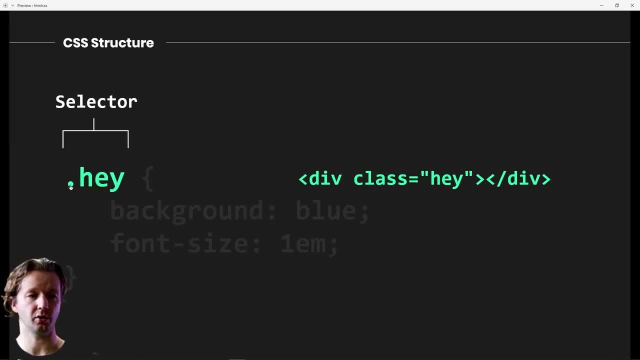 could put div right here without the period, And that means you're creating a selector that's based on an HTML element itself in the name of it, And that means anytime you have a div element in your HTML document, whatever is defined in here will be defined on all of them. Next up is what's called a 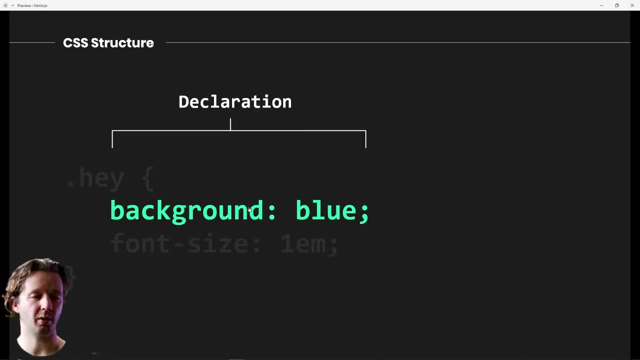 declaration. Next up is what's called a declaration. Next up is what's called a declaration All right. It's basically a property and value pair. You can have many declarations within a rule set, All right. So this one's going to make the background blue. This one's going to make the 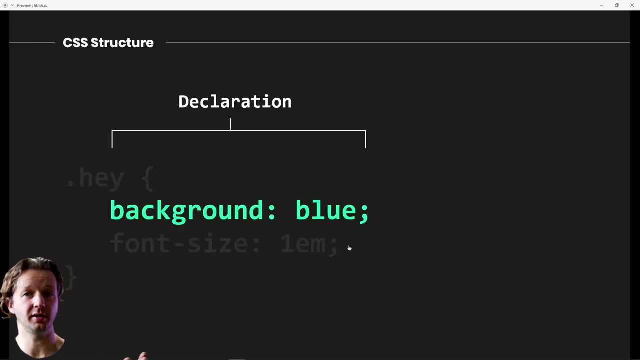 font size: 1M unit, And you can literally have dozens upon dozens of declarations inside of a single rule set. So, like I said before, now we have a property which is a part of that declaration And of course we have the value right here And that is essentially it. That's a very 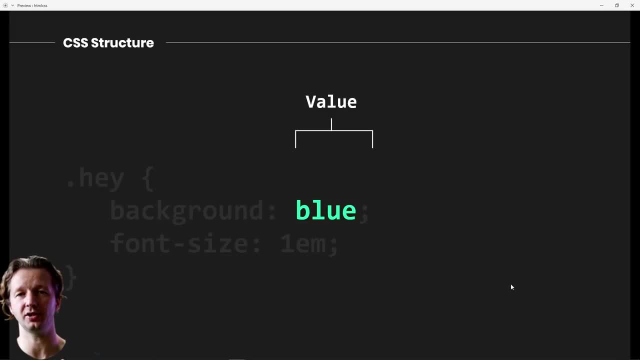 quick rundown of the structure of both HTML and CSS At this point. if you've never touched it before, I don't expect you to really understand it, because you don't have the context yet, You haven't actually written it and haven't been able to see what it does in the browser. So that's what. 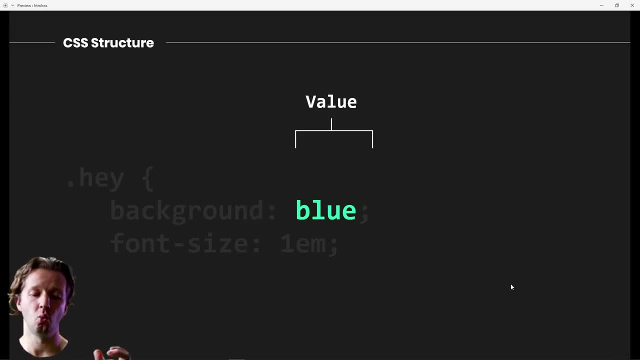 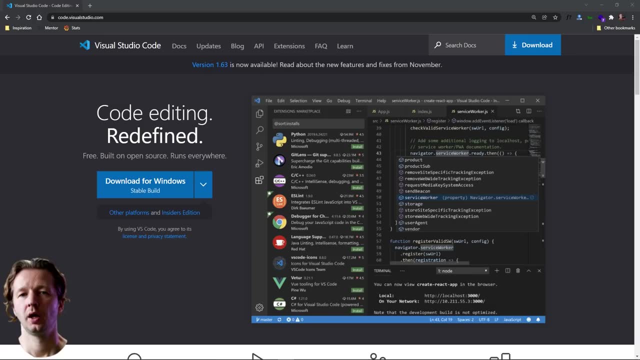 we're going to do now? We're going to get our hands dirty with actual HTML CSS and working to build a design that we saw at the very beginning of the video. Now, in order to rate HTML CSS and many other languages, you need what's called a code editor. Now, right now, at the time of 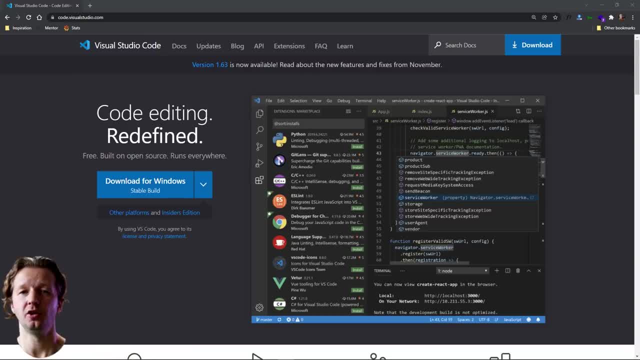 recording this video, and this has been the case for at least several years. the most popular code editor to use is from Microsoft. It's called Visual Studio Code right here, And the URL for that is codevisualstudiocom. rather, And this is the most popular, And guess what? It's free All. 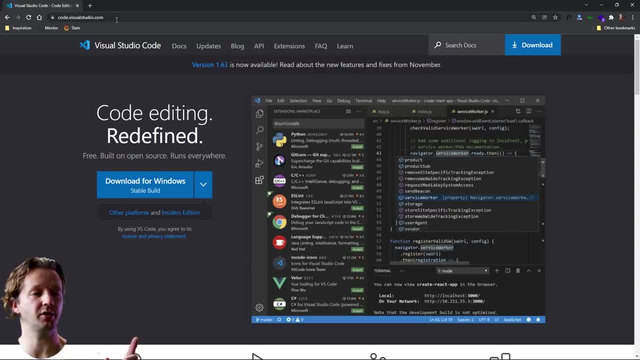 right. So I'm going to want you to go to that URL, codevisualstudiocom, and download it for your OS, For Mac OS, And there's also Linux available for you- hackers who use Linux- And then download it and get it installed. So pause this video, get it installed and then come back. So, in order to get, 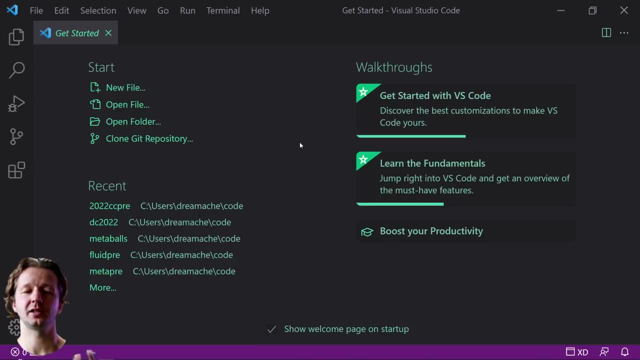 started, assuming you have Visual Studio Code up as well. And, by the way, just a quick thought here: If you're really interested in development, it's going to help you tremendously to get two monitors. All right, And for me, I hate working on a laptop. Many people do it. No, that's fine. 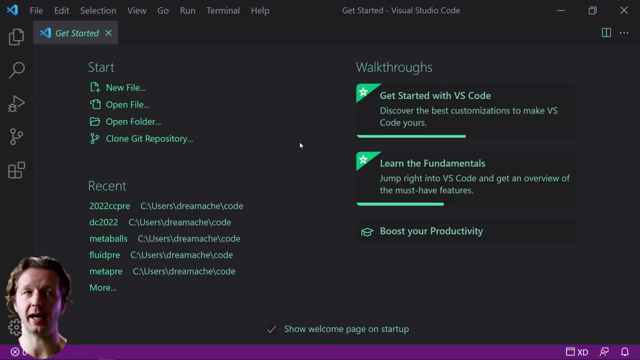 But if you really want to be as efficient as possible and you're at home or you're at an office or whatever, get a second monitor, because you can put your code editor on one monitor And then on the other monitor you can have your browser. 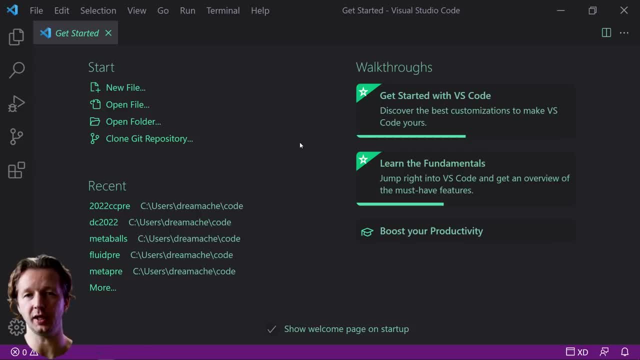 which is auto reloading every time you're making changes to it, And that way, when you're working on a website or a web app of some sort, you can just switch back and forth, Because otherwise, if you only have one monitor, then most of the time you're going to have to come down here and 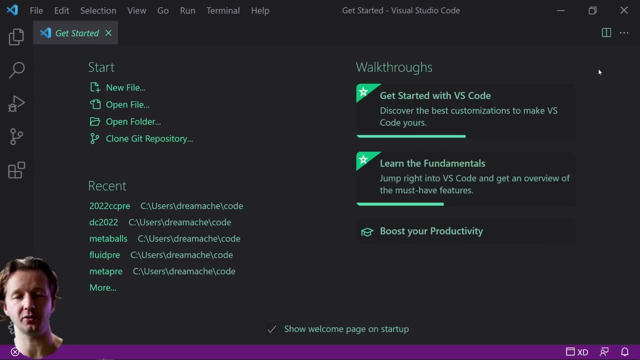 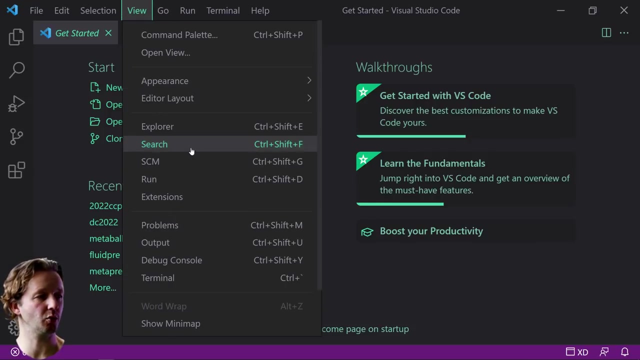 then click in order to show up your browser, And you have to switch between back and forth on them. So let's go ahead and get started here. What we want to do is we have to create a folder in order to store our new website, And so what we want to go to is view and then terminal. 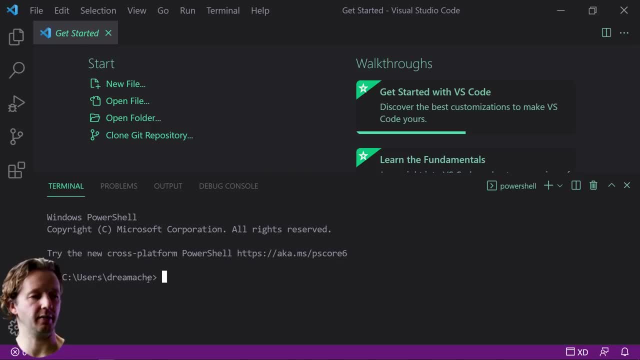 right down here, All right. So right here this: by default in Windows. it's going to put you in your users, your username folder. I have a folder in there called code, So if you don't have it you could type mkdir code. 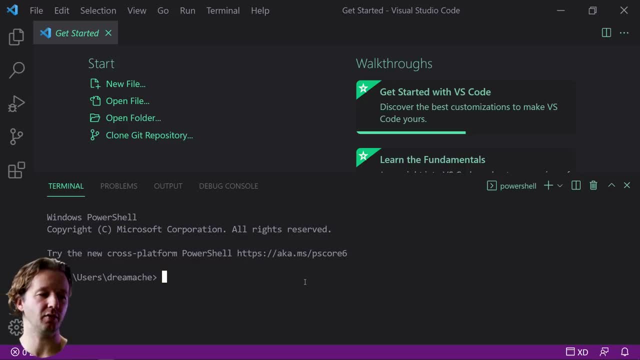 I'm not sure what that same process would be for Apple. I've never used Mac ever. So, yeah, just Google it if you don't know how. So we're going to go to cd code, because I already made that, And then we're going to make mkdir, a new folder, And in here we'll just call this: 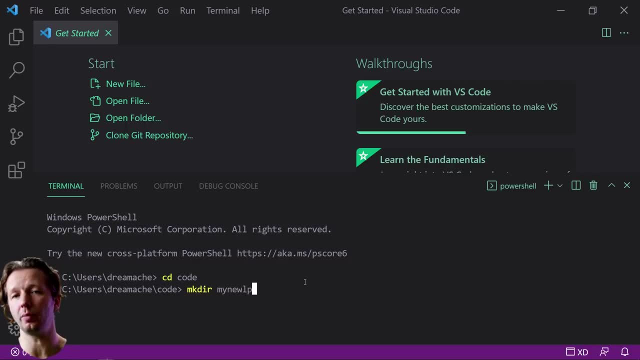 my new LP for landing page. A landing page is like the first page, like the home page, basically. So now we're in there, Now we can type cd lp to hop into there, And now we can just hit code period or we could just hit open folder. 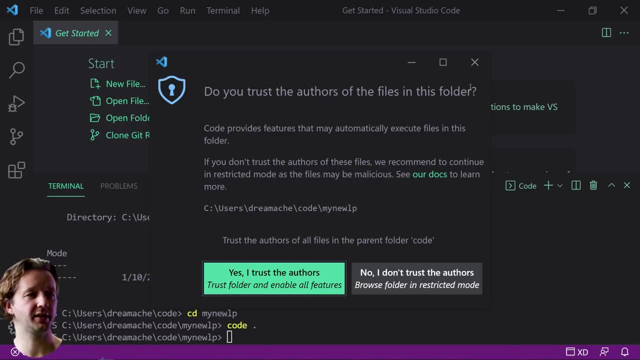 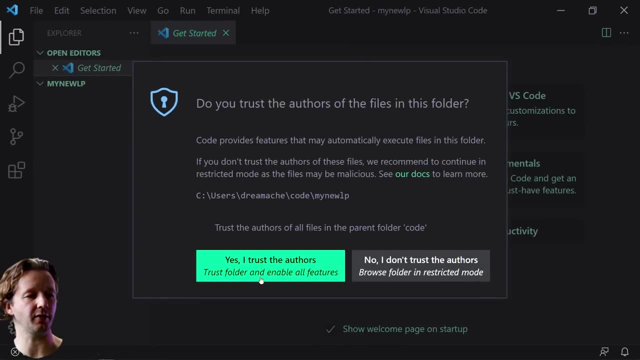 just to show you what code period does. When you type that, it just gets a Visual Studio Code instance, like another copy of it, out here in your browser or on your desktop. rather Yes, I trust authors, And there we go. Now we can see where it says: my new LP. This is the folder. 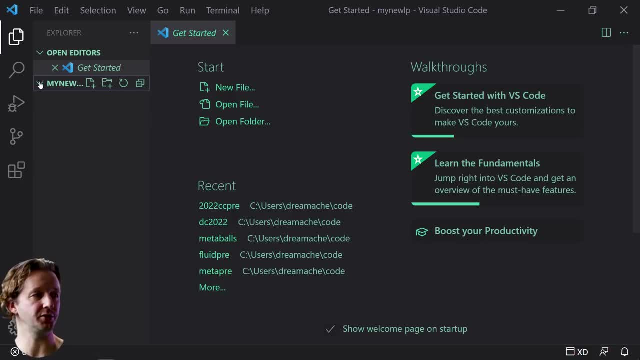 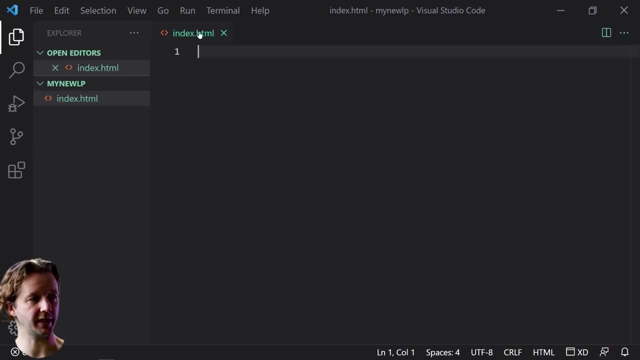 that we're currently working with within our instance of Visual Studio Code. So now we want to go back to the file, So indexhtml. let's close that little window right there, And this is where we write our code in the code editor. As you can see, this indexhtml is highlighted, It's. 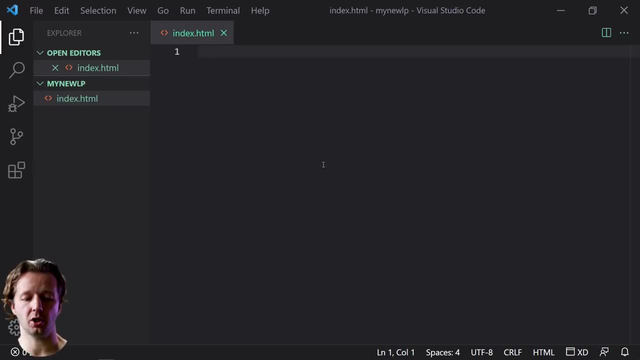 currently selected up here. So one of the great things about Visual Studio Code is what's called Emmet E-M-M-E-T. If you do a channel search on my channel here on YouTube, you type in Emmet, you'll see a crash course. I did on it, But basically it helps you write HTML faster. 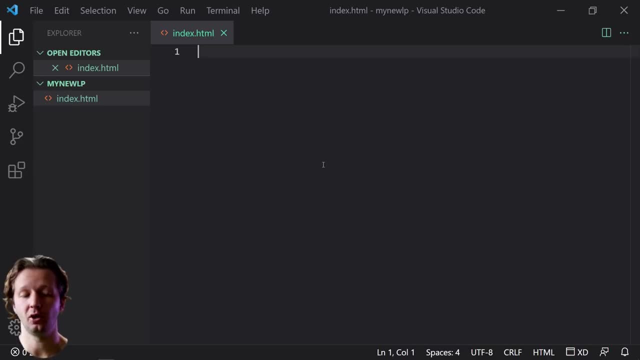 So one of the first things I do. it is the first thing I do Whenever I'm starting off a new HTML element or document. rather, I just put in a shift exclamation point, hit enter and there we go. It creates the quick. 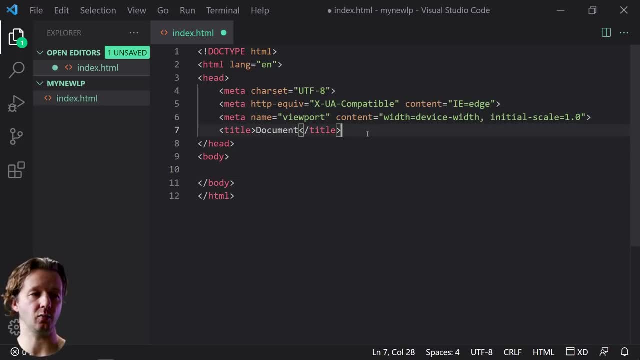 boilerplate code that you would otherwise have to write by scratch or by hand, essentially. So, as you could see, there are some things up here like the doc type HTML. You don't ever touch that, You just leave that there. Here's the HTML tag, right here. Here's the closing one. So 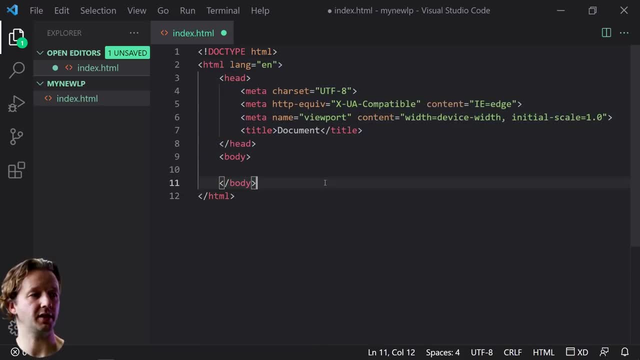 this is the opening and closing, And then inside of it we can see this stuff. Now we have, like I showed you before, the structure. We have the head with a bunch of stuff in it, like the meta tags, as I mentioned before, and also the title, And then we also have our body element And this is: 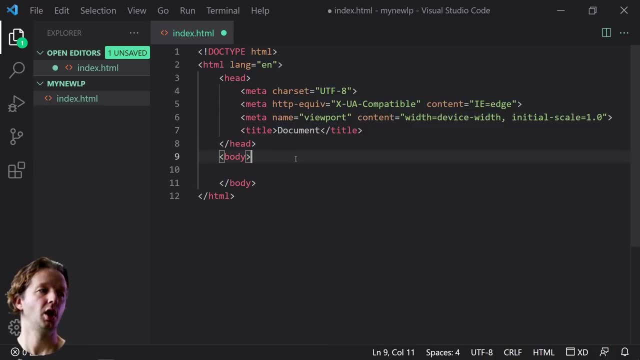 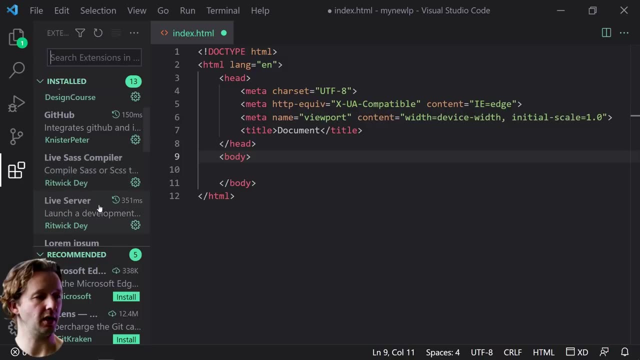 where we're going to be spending most of our time writing stuff. So there is an extension that I want you to use here for Visual Studio Code, and it is called Live Server. What's cool about Live Server is if we go back here after you install it and you reload your. 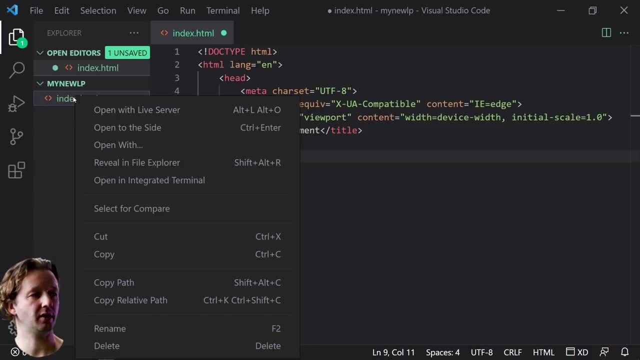 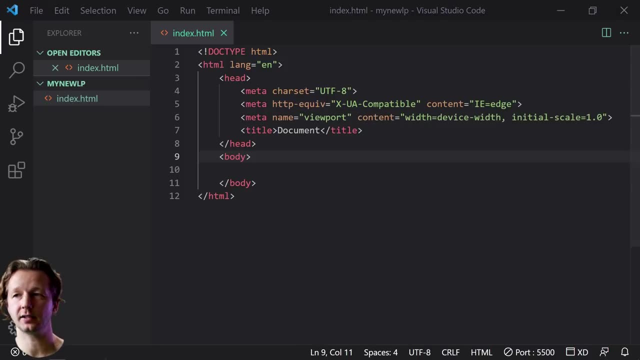 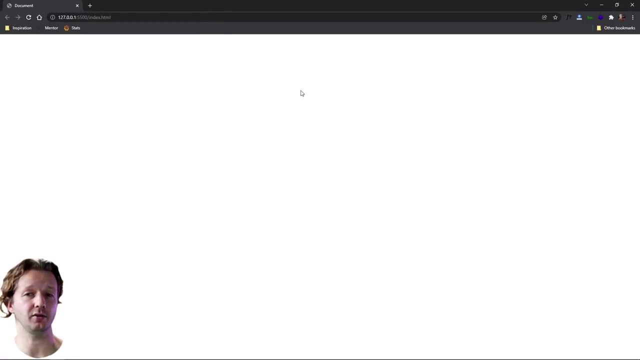 instance of this Visual Studio Code. you can right click our indexhtml and put in left click rather open with Live Server. When it does that, it's going to open up whatever your default browser is- mine's Chrome- and it's going to show you what your HTML element looks like, your document. 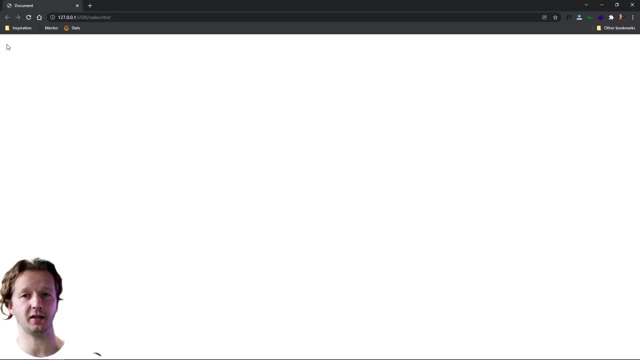 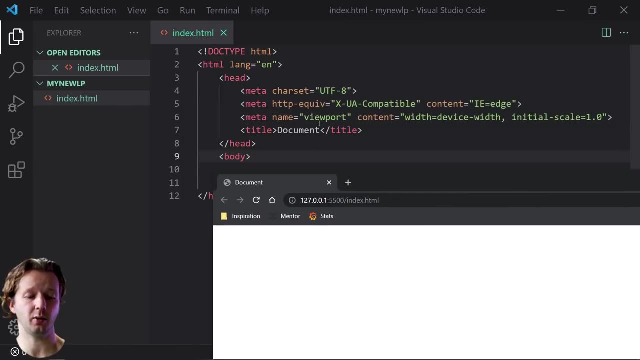 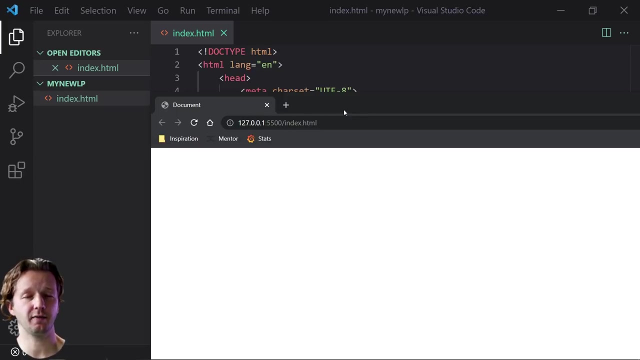 Right now it's just white and there's nothing in it, because we haven't specified anything within it. So what's also great about it is, whenever we make a change to this document and we save it with Control S, it'll automatically refresh this for us. That's why it's really handy for us when 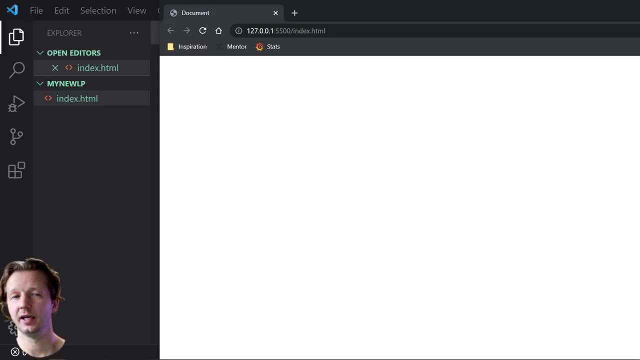 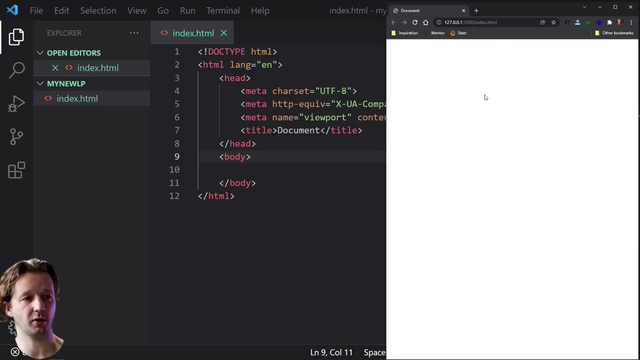 we're working with this to have two monitors, But of course I'm not recording on two monitors, so I am going to have to probably go back and forth In a little bit. I will probably show this right here and then the code editor over here. Okay, So what we want to do when we 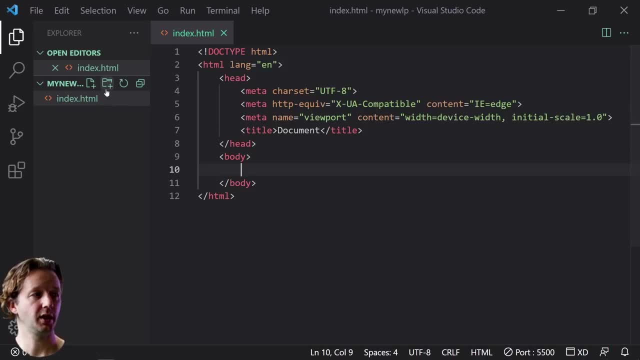 Actually is to get our CSS document ready as well, And typically when you're dealing with a structured project, you'll have a CSS folder, because you might have multiple CSS files to write your CSS in. So we're going to create a CSS folder called CSS, So you click this little plus. 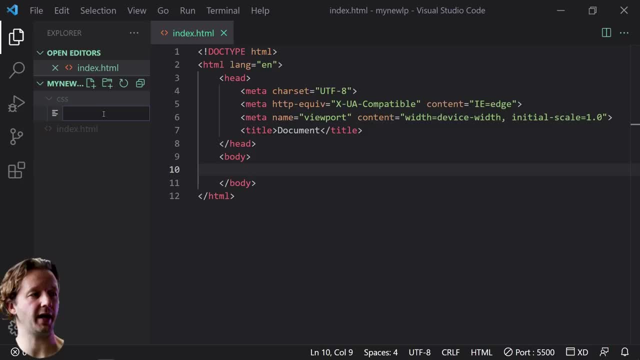 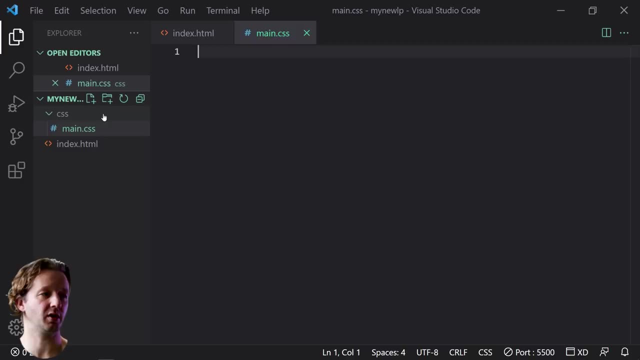 folder icon and then you click the new file icon and we're going to put in- We can name it- something like maincss, Some people name it indexcss, whatever you want, and that's good. Now for the purpose of this tutorial. I am kind of going a little bit ahead of what you probably 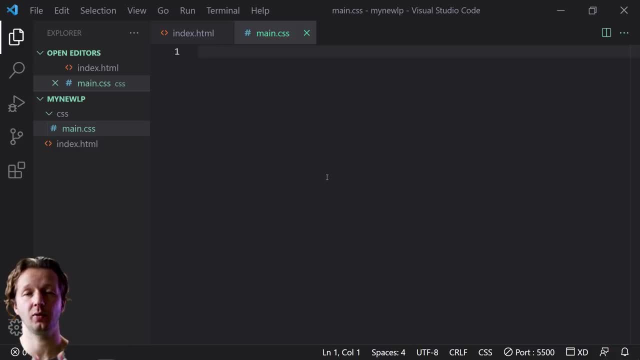 should be doing at this point And we're going to not write. We're going to write CSS, but we're going to write it in Sass. So I know this is confusing you. Sass is just a way to write CSS in a more efficient manner, But really I'm only going to use one feature of. 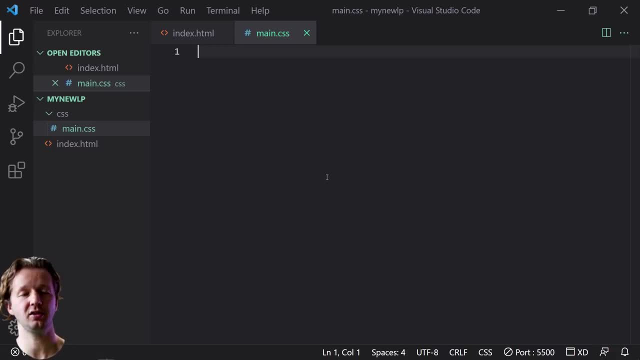 Sass, and that is nesting rule sets within each other. You can't do that with plain CSS as of yet, And so I'll show you what that is, But otherwise, everything I'm doing is just plain CSS, But in order to do this, we have to right click this. We're going to rename it. 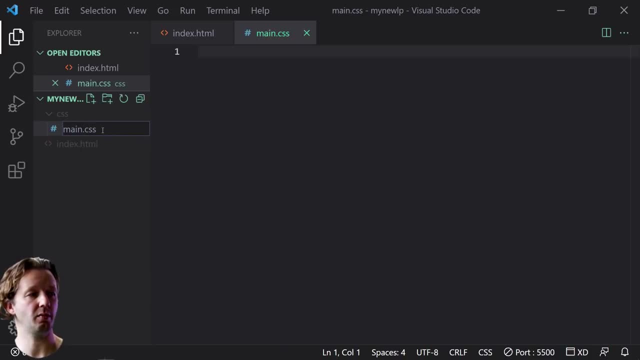 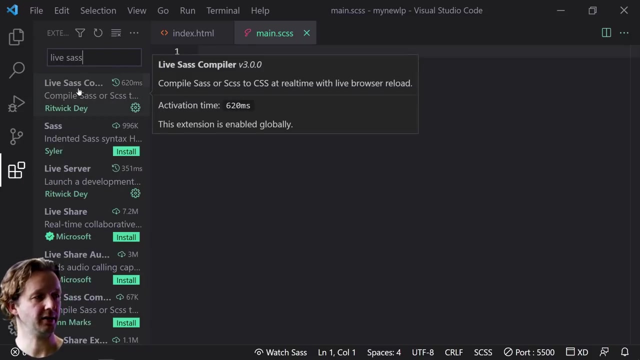 And so we're going to change it from maincss to mainscss. All right, Now I have this little Sass icon. that's the logo for Sass showing up, because I have an extension called the live Sass compiler. So if you type in live Sass compiler, right there you. 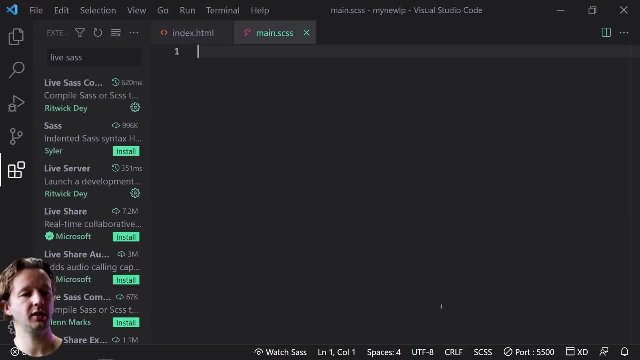 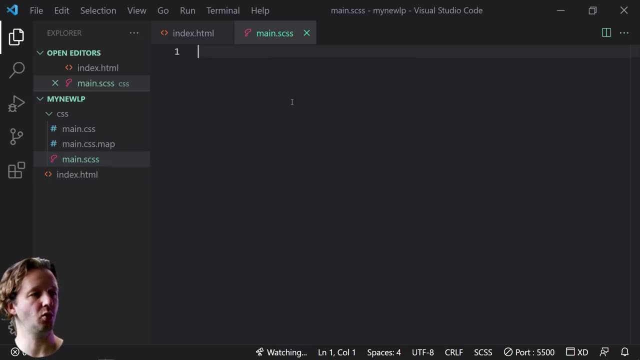 want to go ahead and install that. Once it's installed and you reloaded, you can click watch Sass. All right. So what this does essentially is when you write inside of your mainSA Three document, for instance, you don't have to do this If I type in body background blue and I hit save. 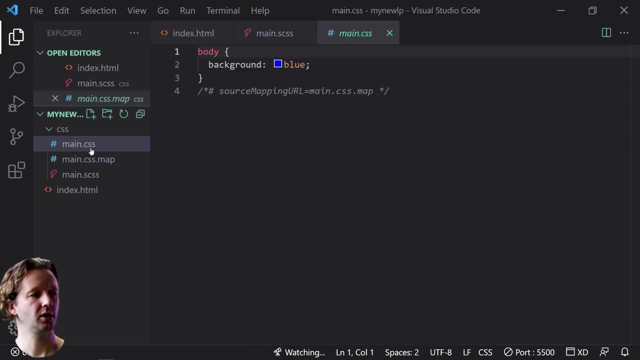 you'll see, it creates two other files. Ignore the map file, But the maincss file- that is what's going to be linked or referenced there- is probably going to be linked to the maincss, But then just do a little test here now Marat, Here's what it's going to look like And then this is what's going toеч. 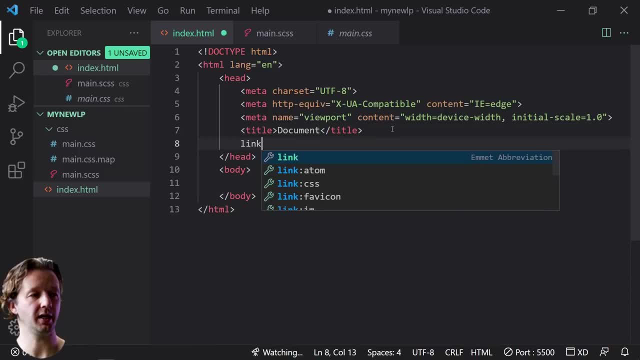 referenced here for this HTML document. So we're going to type link and then enter. That way we don't have to write all this other stuff that's necessary for this HTML element to work. So the href is the attribute. That's one of many attributes. You know, content is an attribute. 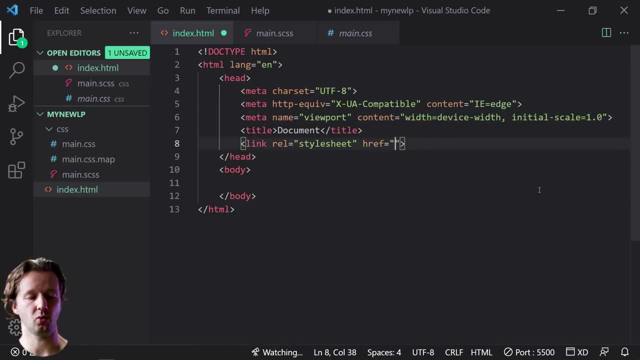 name many different attributes. like I mentioned, We're going to reference that file location. So it's in a CSS folder: forward slash, maincss. We can just click right here. So now, if I go back to the browser, it is blue, a very bright, horrible blue that might make you blind. 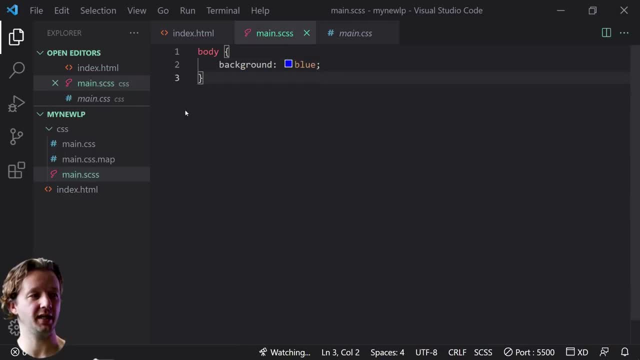 But that's how that essentially works. So we're writing our CSS in this sass file, but it's all getting compiled down into this other file called CSS. And so just to show you one of the benefits of being able to write in sass and one of the core features that 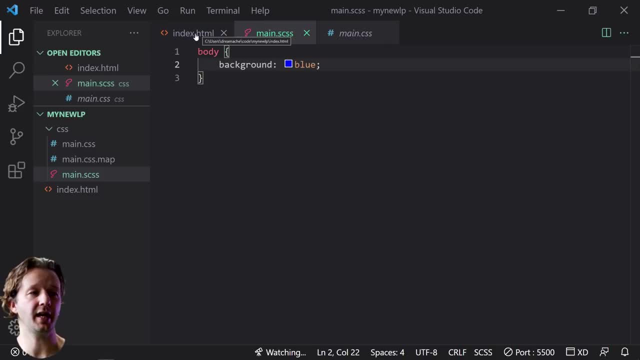 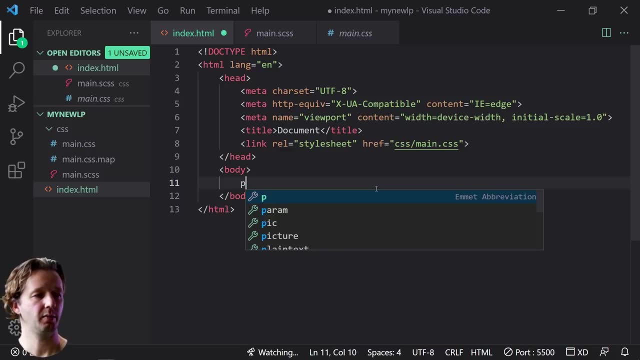 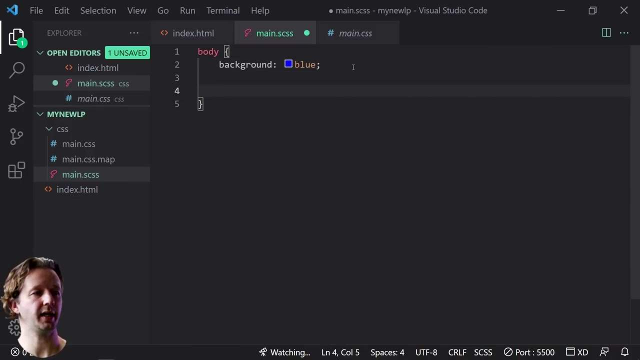 the primary features of sass I'm going to use is the nesting. I can show you an example real quickly, So you don't have to follow along. I'm just going to put in P like for a paragraph, Hello, I'm going to hit save. So what I can do now is I can say P. 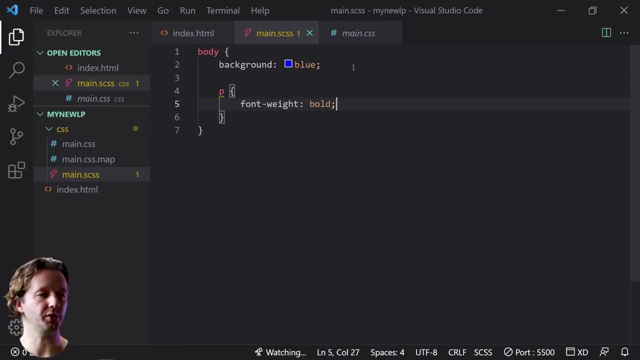 and I will say font weight: bold. All right. So if I go back here it is now bold. It's pretty small, probably hard for you to see. but this nesting you cannot do regular CSS. So for instance, if you look over here, 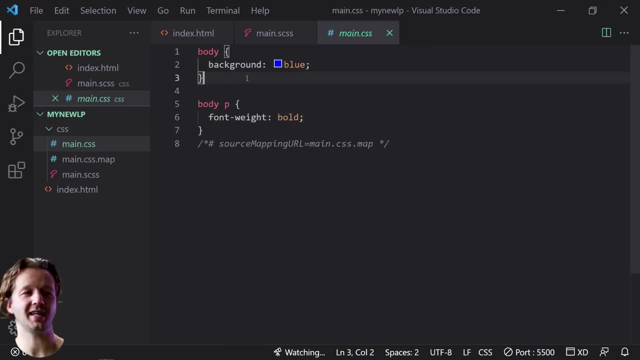 I'm going to say font weight bold. I'm going to say font weight bold. I'm going to say font weight bold. Notice how they're not nested All right. So that's just. it's for organizational purposes, essentially, for the most part. So that's why I'm doing that. I did want to explain that a little. 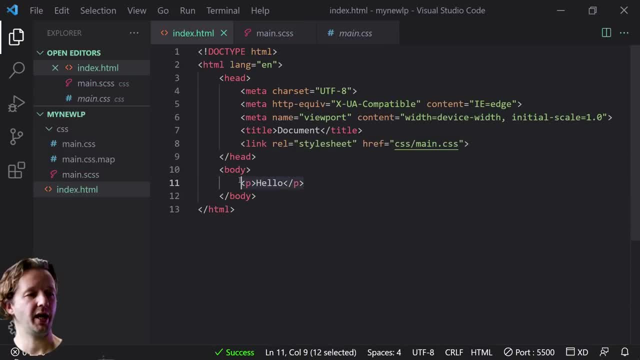 bit All right. So, going back here now, what we have to do is we need to, and also you can specify a nice title, like my new LP, whatever. That's what will show up on search engines and all that stuff, And also on the browser title or the browser, the bar that you actually click, and 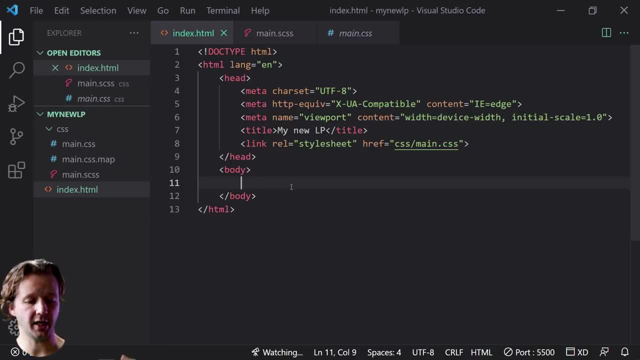 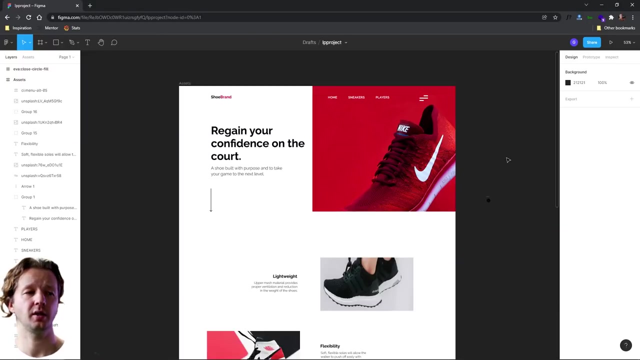 drag around. So now what we want to do is actually take a look at our design and then start writing our HTML. You got to have your HTML first before you start writing your CSS. All right, So here is the Figma document. I'm going to go ahead and actually link this into YouTube description so that you 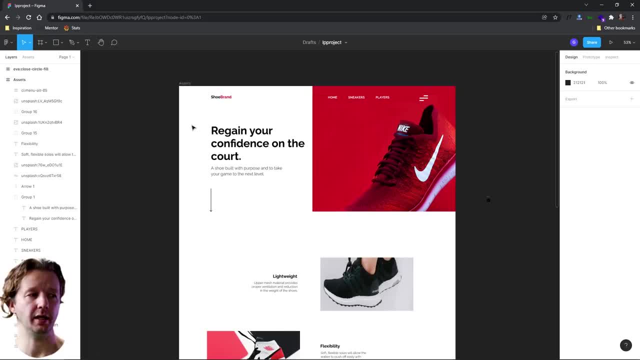 have access to this so that you can look at it as well, And this is typically how you would be doing in a professional setting. I very rarely do you just start off designing a website when you're working with your HTML. So I'm going to go ahead and do that. So I'm going to go ahead and do that. 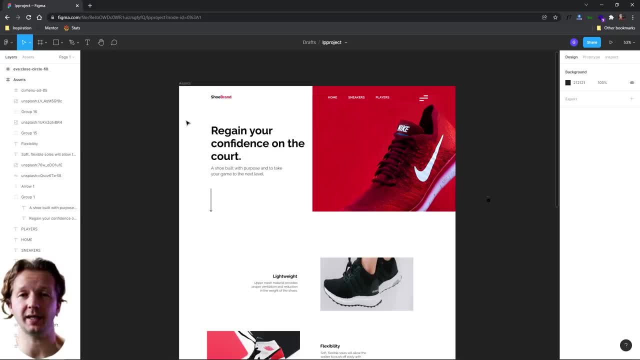 You want a mockup, preferably done by somebody who's a good designer. If you want to become a good designer, member, visit designcoursecom, because that's what I teach as well. But nonetheless, outside of the spam right there, you want to look at an actual, polished preferably. 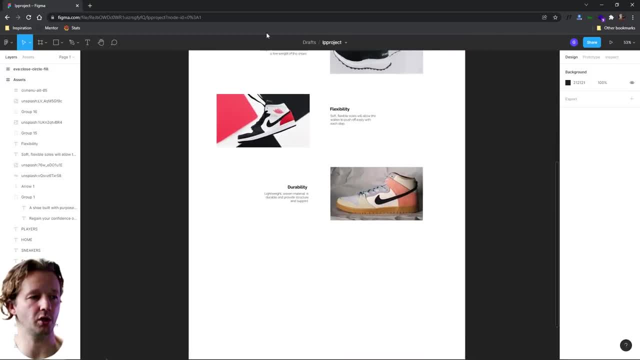 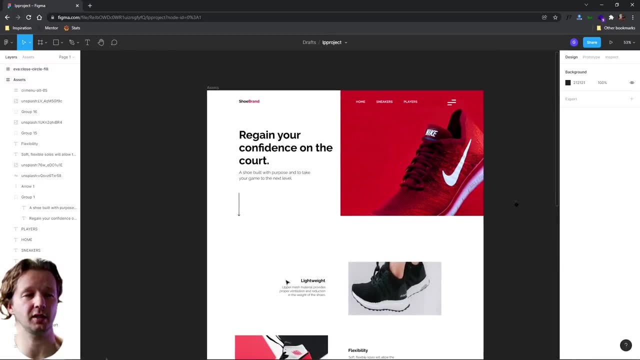 high fidelity document where it's going to show you what you want this to look like. This is all we're going to do All of this right here. it doesn't look like much, but for a crash course, this is a lot to take in, All right, So this? 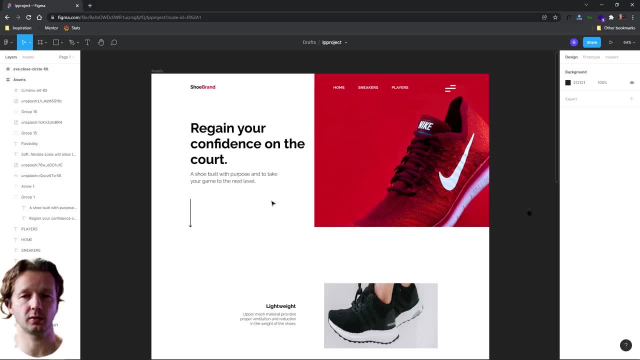 this is the desktop version. When I'm structuring and writing my HTML, I like to see the full experience, the full desktop experience. I don't want to look at the mobile version, because mobile versions can leave things out intentionally because you don't have as much space, So it 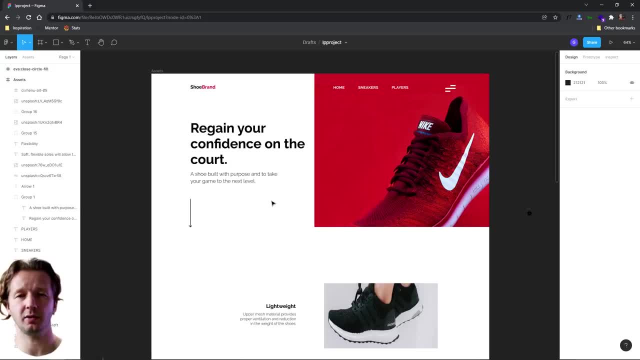 simplifies things. But for HTML or HTML is always going to be the same and we have to create all the HTML elements for the full experience. So I start from top down, All right, So when I'm thinking about what I'm having to do, I'm going to go ahead and do that. So I'm going to go ahead and do that. 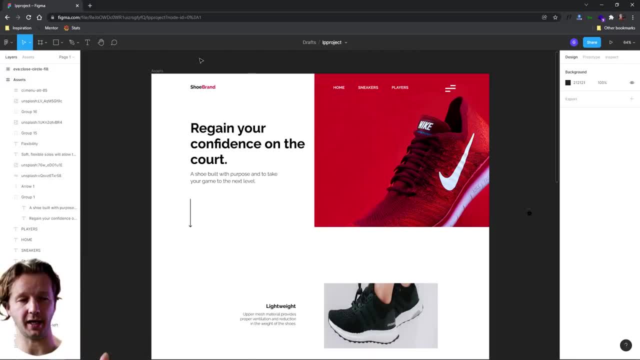 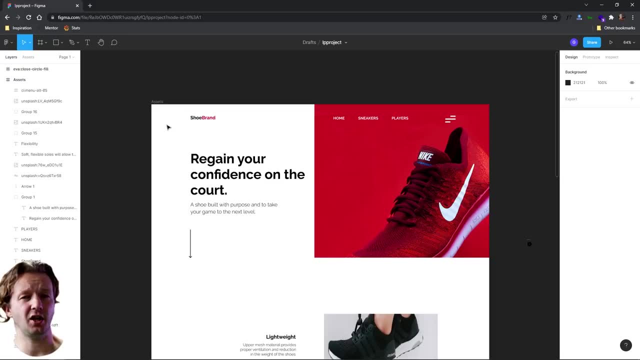 How I'm structuring things. I it's starting from the top down. We don't work from the bottom up, Okay, When I'm like looking at the structure of things. So the very first thing that I usually ask myself is: does this need any type of container? So by container, I mean: 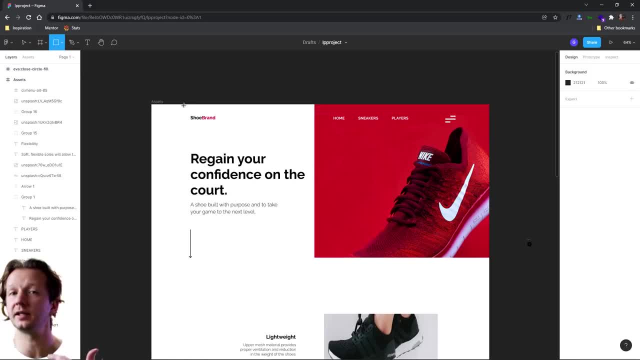 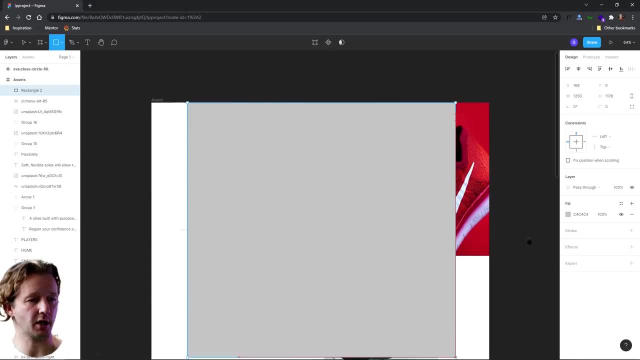 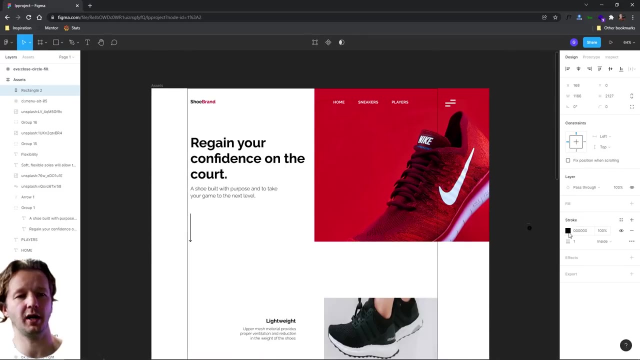 we can visualize this. This isn't going to be a part of the design, but if I take this rectangle tool, we can kind of draw a bound right here, bounding box around this whole thing. that kind of just contains everything Right here. So if I get rid of the fill and just give it a stroke, you don't have to follow along. 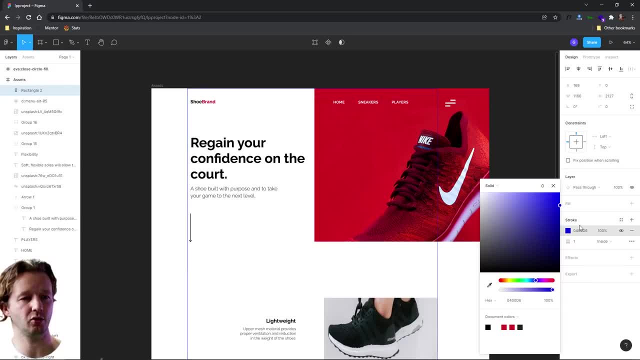 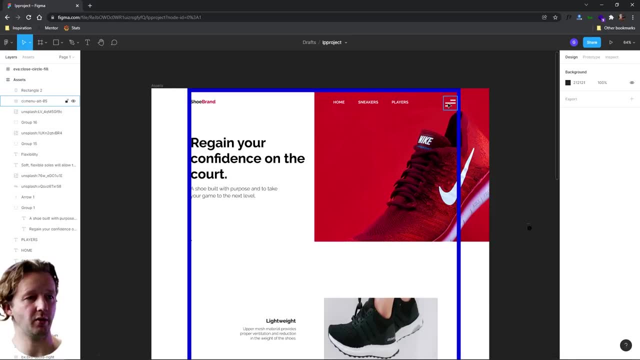 by the way, I can make this. maybe we'll make it blue and then we'll make it pretty thick. Let's drag this out to include that little hamburger menu icon, which actually this isn't going to be there during the desktop version, So let me remove that and we'll write a line, is there? 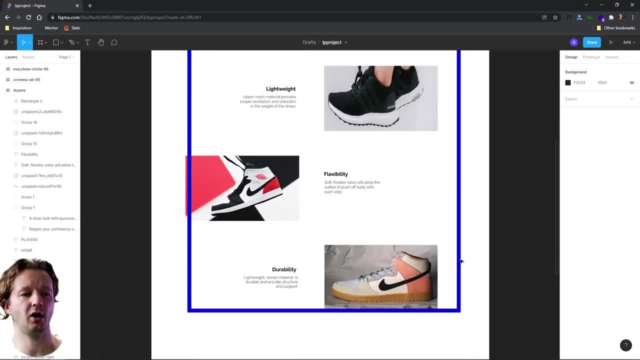 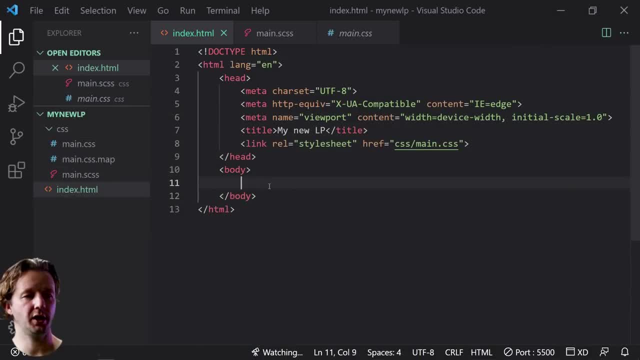 we go. So this is basically an HTML element that we'll want to include here. I for this design, So let's go over here and we're going to type in: if we want to write, div class equals like a wrapper- uh, sometimes it's called container, You can, you can name it whatever you want. 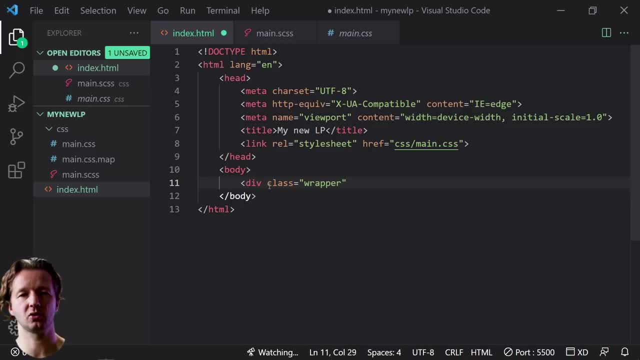 really, but you commonly see this as named- named for this sort of thing, This idea that we're we're wrapping everything around a central element- Uh, it'll be wrapper or container usually. Um, so you could do this, or, if you don't want to have to type out all those elements, 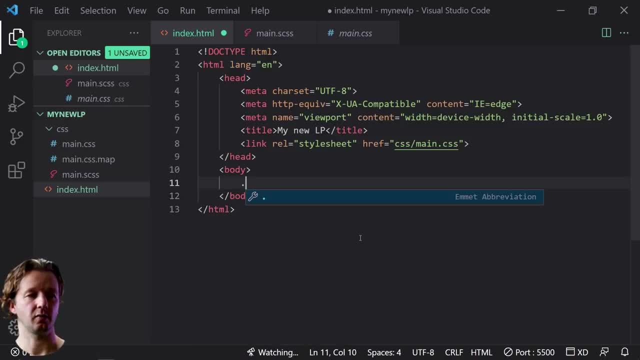 you can use the M abbreviation, So period for class and then the name of it and then hit enter. automatically it creates a div element. So div element is probably the one element that you will use the most when writing HTML And it's just kind of like a generic element, that's. 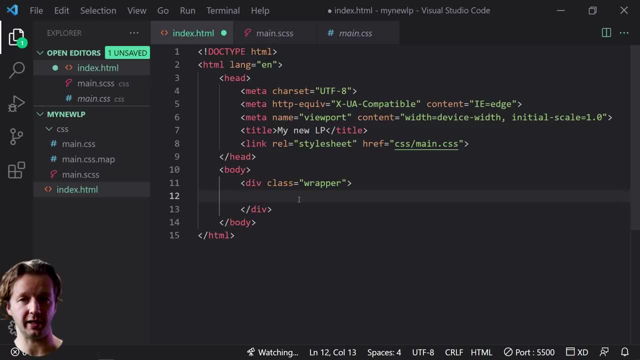 created for defining the structure of your layout. All right, So you'll see plenty of div elements and their attributes Primarily you'll see as just being class or or ID, So you can also have multiple attributes, of course, in a given element. ID equals, you know. 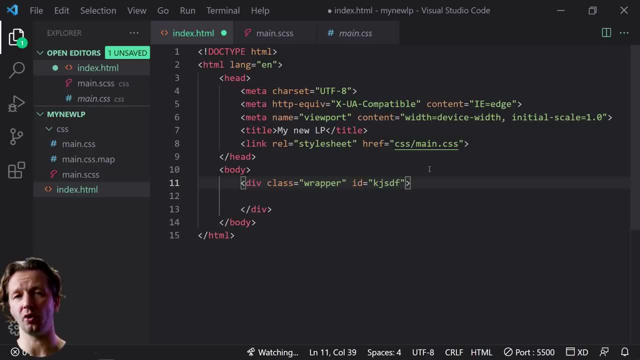 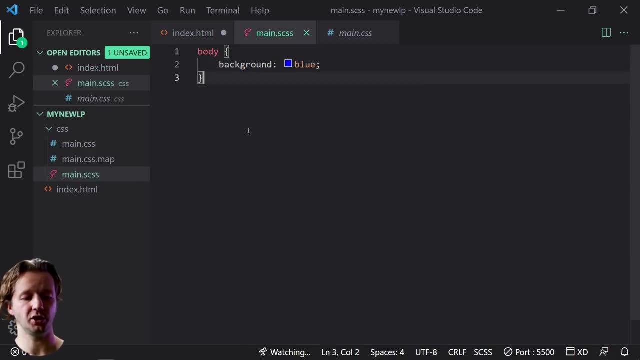 some unique ID, and ID is primarily used for JavaScript, though You typically don't see people referencing uh IDs and CSS. Now, if you wanted to, you would just put, instead of a period, you would put a hashtag and then the name of the value that you gave it. Essentially, I think I. 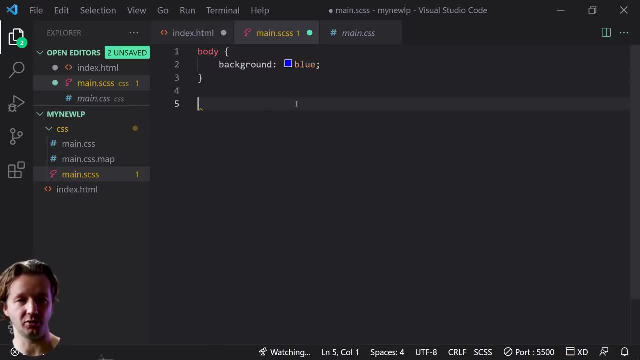 hit the keyboard, something like that, but you don't really don't see people do that anymore. So you can also have multiple attributes, of course, in a given element. So you can also have multiple attributes, of course, in a given element. So you can also have multiple attributes. 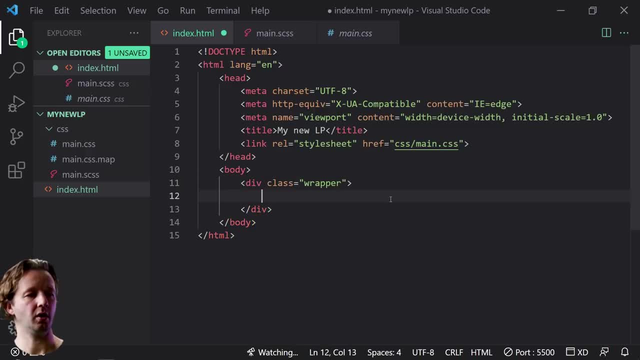 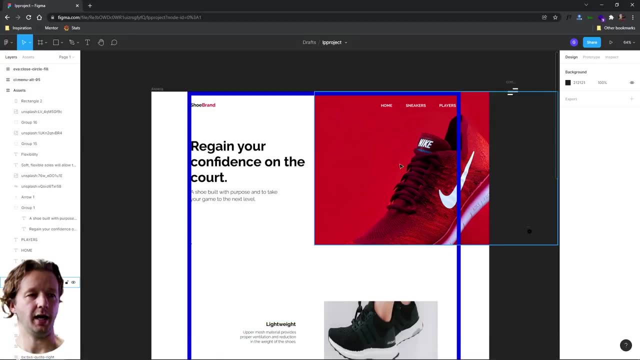 so we'll leave off ID, All right. So now we have that overall element. One thing I do want to consider is this photograph right here. I notice how- let me hide this real quick- Notice how I we have the menu on top of it. So how do we show a photograph like this picture of a Nike shoe? 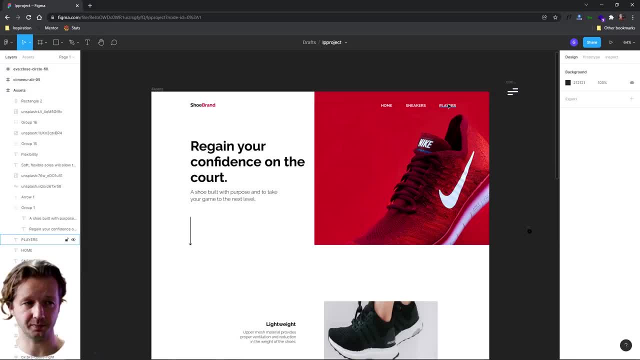 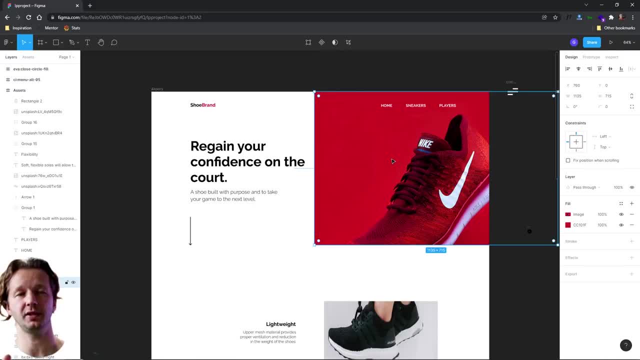 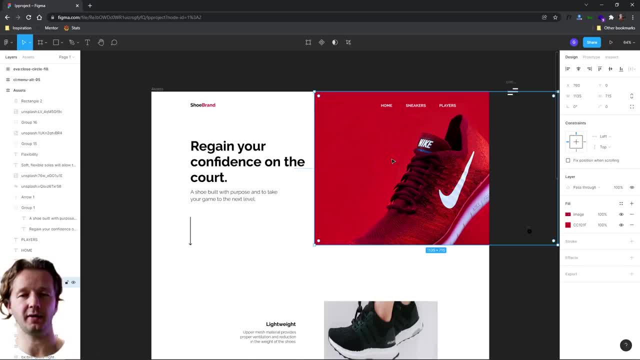 can kind of just break outside of the box model, as it's called- And you can position and stack it by like way in the background and you can have things on top of it like this element right here, And so when we do that, we can really position or place the HTML for this image anywhere in the 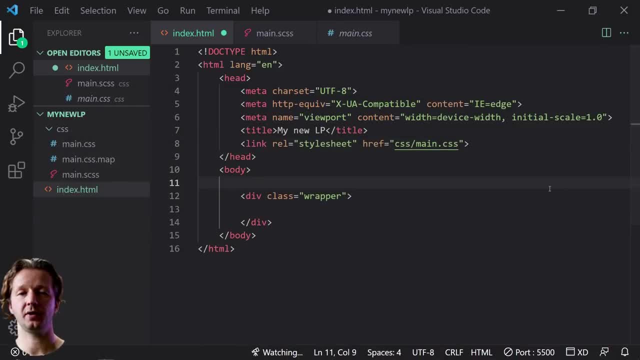 HTML element, So I prefer just put it at the top. Now there's two different ways. you can actually show photographs or imagery in a sense that are from like JPG files or PNG files, And the first way would be an image tag. So if we type image, source equals this is where the source goes. 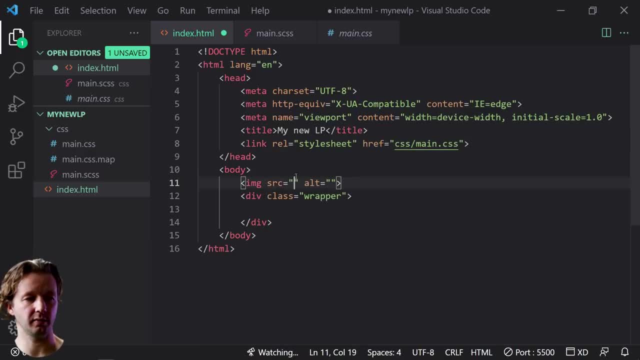 kind of like HREF. right here, Source is like where you know the actual file is located. Now, currently we don't have any image files in our my new LP folder, So we actually have to get that image And I'm going to link this image in the YouTube description. It's a free image that. 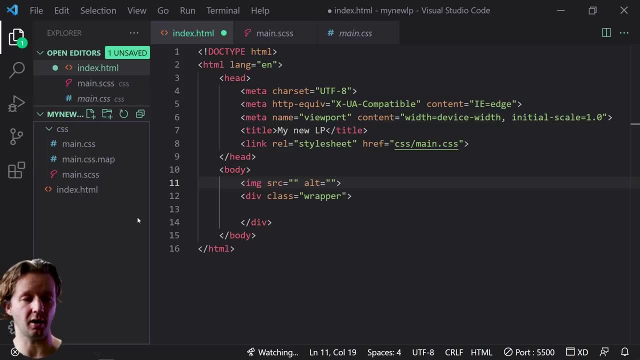 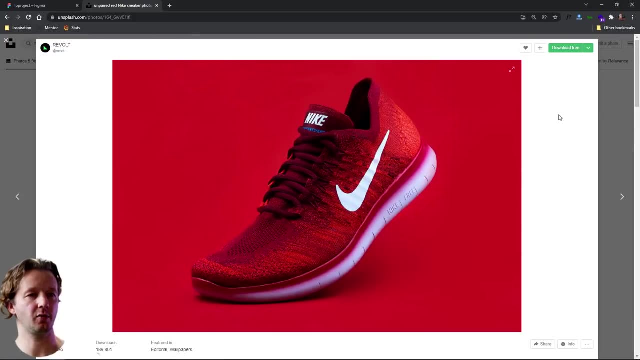 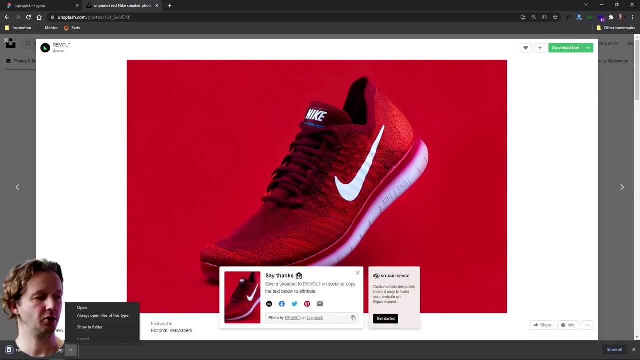 you can use from an awesome service called unsplashcom. So right here, if you type in shoes y'all, you will also find it. This is the graphic that we want, and we can just click over here and just choose medium And it will download that onto your computer here in Chrome. 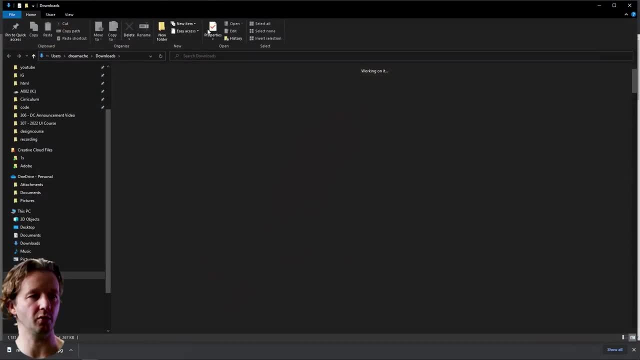 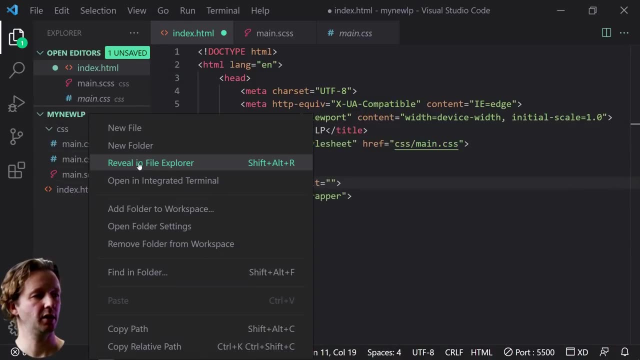 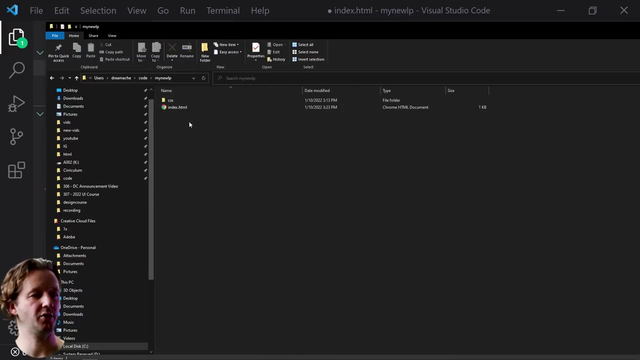 We have this little element. Firefox has the same thing. We'll click on show in folder, And then what we do is we come over here, right click, reveal in file explorer, and that opened up on my other monitor, And so we have my new LP Now we we double click into. 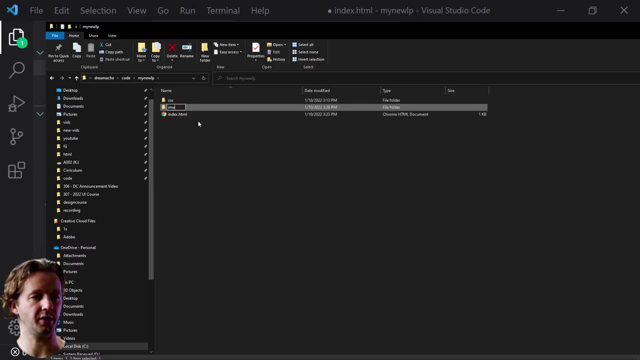 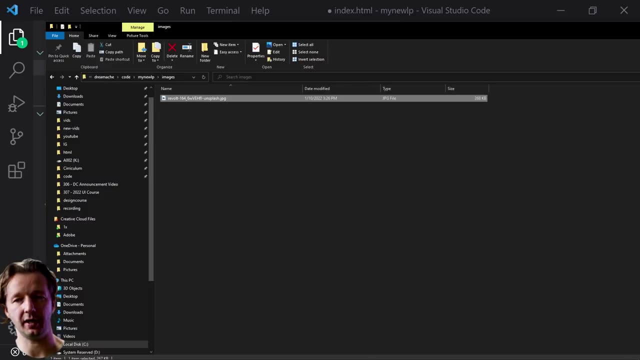 that folder And then now we can have a new folder called images, for instance, or assets- You can name it whatever you want- And we can drag from here the other element which is on my other monitor, that picture right there. So now we're just going. 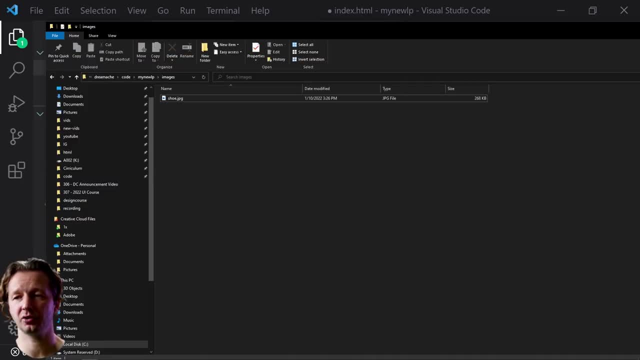 to call this shoe. Now we're also going to have three other pictures of shoes and I'm going to link those as well. You can use whatever you want from Unsplash and I'm going to drag them in here as well. All right, And there they are: shoe two, three and four. So now we can close this out. 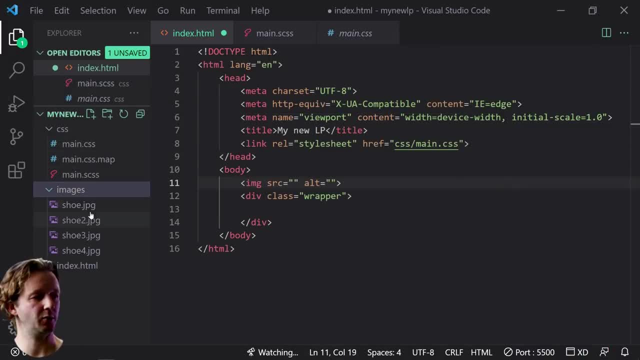 and you could see, we have our images with our- you know- different shoe pictures right here. All right, So let's close that out. And so now we have our image source, Now we could say: images forward, slash shoejpg. Now the alt attribute is a really important attribute. 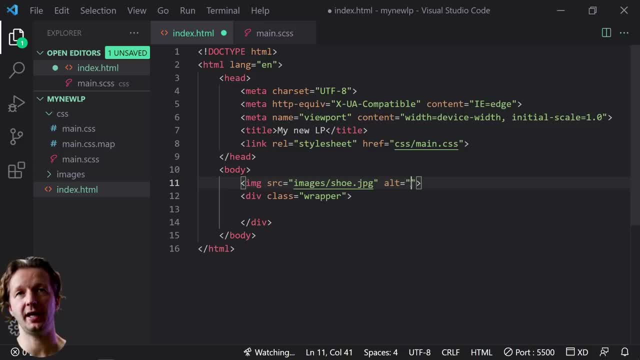 because whatever you put here, when somebody hovers over it, for instance, they'll be able to see a description of it, But also for people who are using screen readers, who are visually impaired, when they're navigating through the website, they're going to see a description of it. 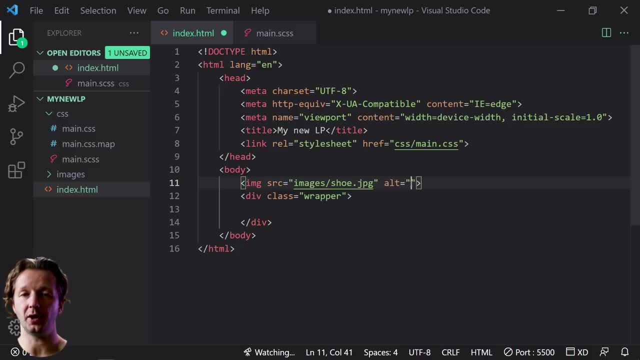 So if they're on a website with their keyboard, it will actually give them an audible reading so they can hear what's happening essentially on this website. So we can just say red Nike shoe, not shoe, not show shoe, rather. So we'll save that and we'll come back here, and here is our. 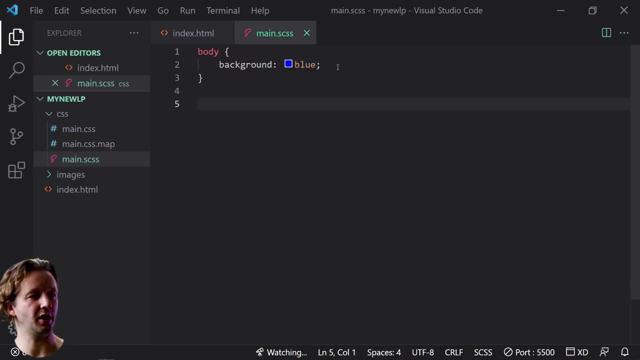 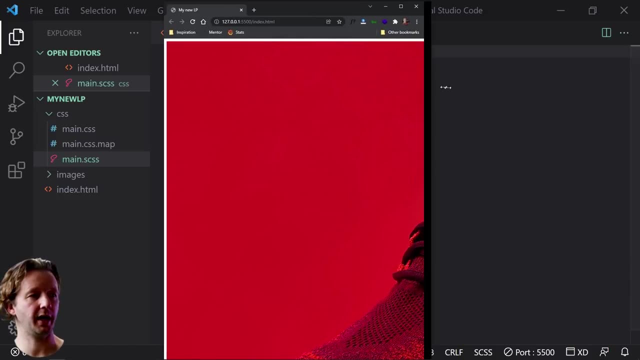 document. Oh, there's that big blue border which we do not want. Let's just delete that right now. And here is the shoe. Now notice, when I drag this in and out, it doesn't change. And also, if I were to bring this up, 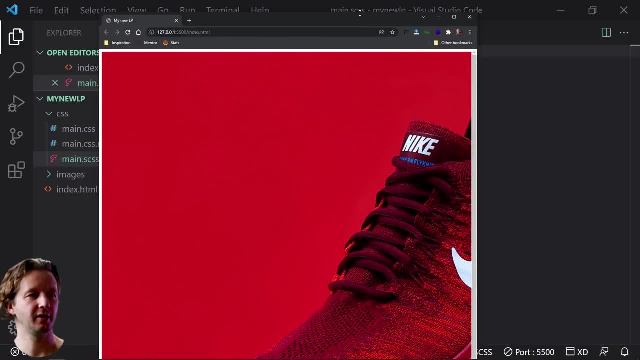 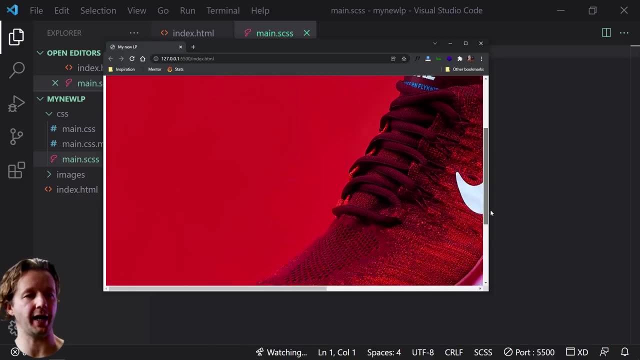 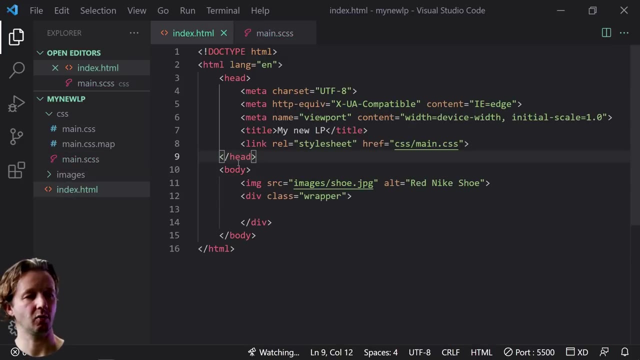 let me try to find the bottom of my browser here. Wow, It's really large. There we go. We could see that it has scroll bars, So we could solve for that and remove these scroll bars and make this image responsive. The way we could do that is, we can reference this image element by: 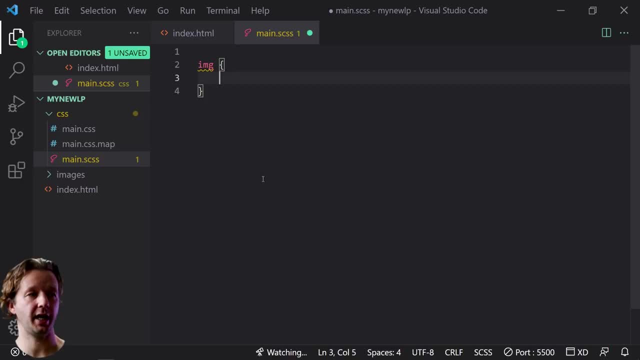 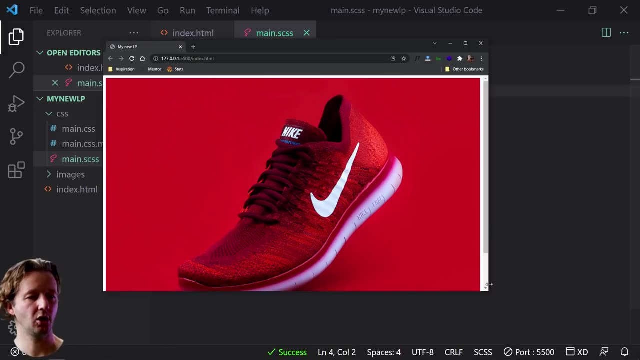 putting IMG here, opening that, And then we can come back to our image itself and we can go back and do some more work on this. So now, if we go back, we will see it responds kind of how we want it to. So that's the first way. 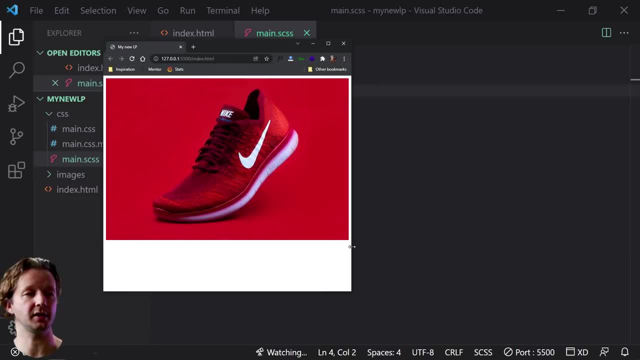 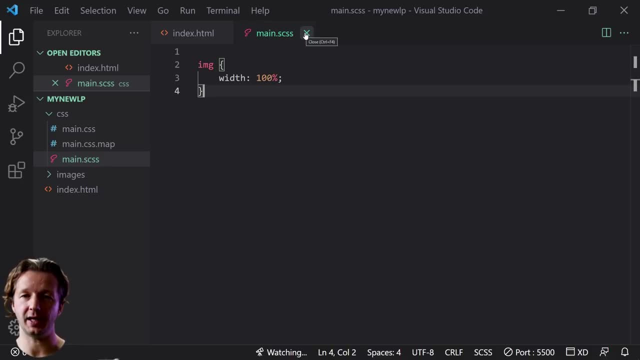 that you can display a photograph here, essentially in CSS. Now the second way, which is the way we're going to do it, because it gives us more control over the image itself, is we're going to make it as a background image in CSS. So let's say we're going to do a background. 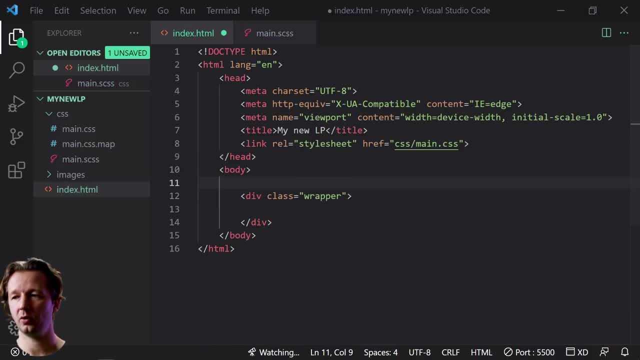 image here And we're going to go ahead and do a background image here And we're going to do a let's. let me show you that real quickly. so the way we'll reference that is: we're going to make another div element. let's give it a class of hero hyphen img for image. and, by the way, hero means i. 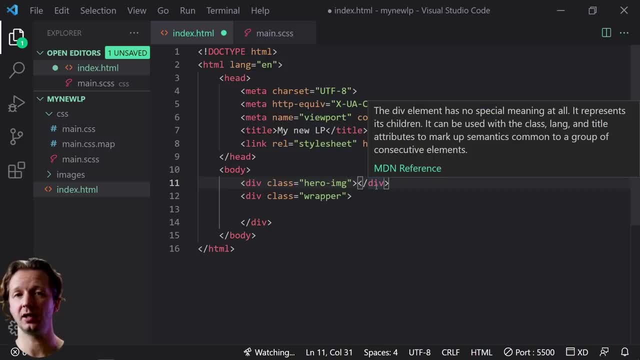 the hero section of a website is usually the first thing people see, so it's like the top of the website. and so now, inside of here, we just leave it like this. we don't put anything, any content, in between these, this closing tags and the opening tag. we just leave it as is, and then. 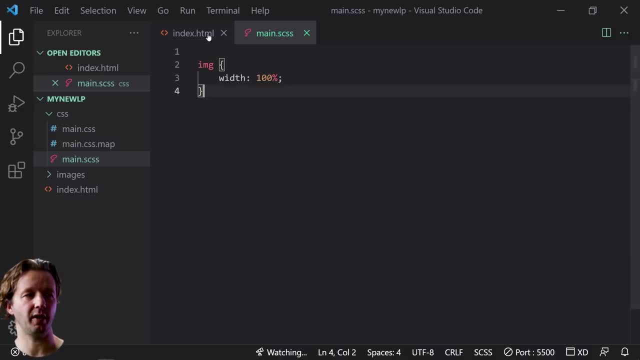 when we get to css portion, you'll see that we will reference- uh, this hero image class right here and create a rule set in css, and we'll define the image there. we're not going to get to the css portion yet, though, but i wanted to kind of describe, you know, my reasoning behind not using 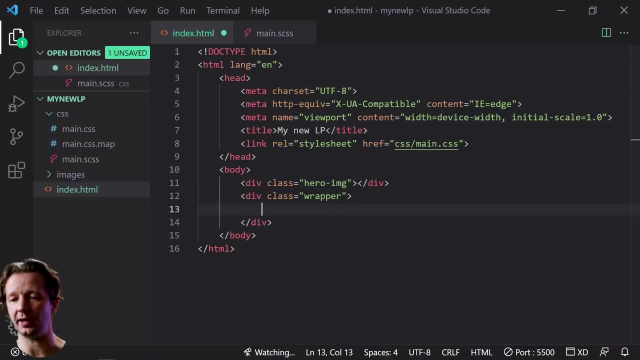 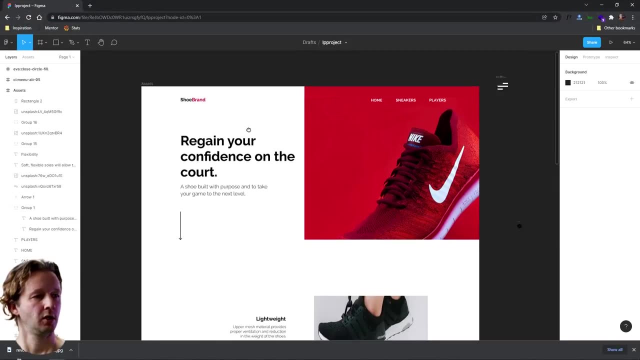 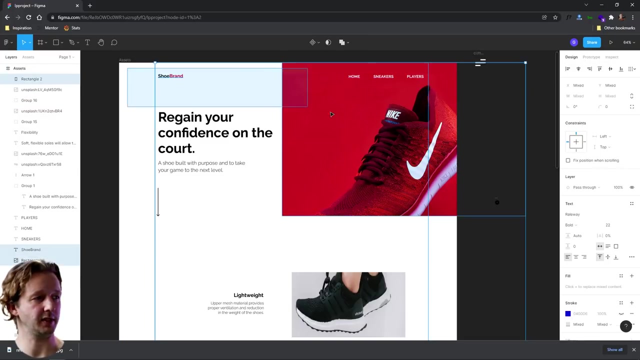 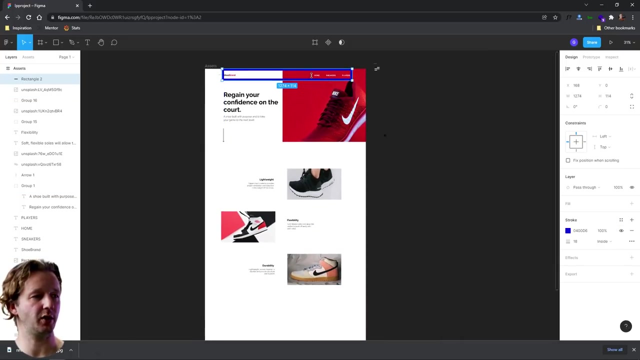 just an image tag. okay, let's continue on. so, referring back to our design, which is right here, the next thing we have is this portion right up here. so if i bring back our um, let's get it over here, rectangle 2, and we review it. i can go ahead and get this situated. 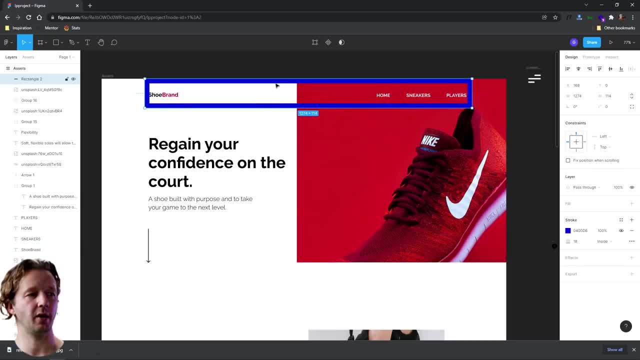 right here. this is what i'm going to look at next. so this is our, our header, which has a brand like a logo, left line, very typical pattern that you'll see that ui designers i create. you see that your logo on the left and then usually to the right, sometimes in the middle, sometimes close to the. 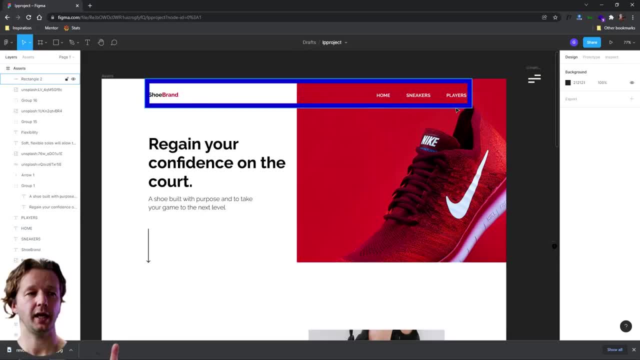 actual brand is the navigation. so we have two elements, and notice how they're in two they're: they're in a column one's. this is in a left column, this is in a right column. so they're not rows where they're stacked up on top of each other, they're columns, and that's important distinction to make. 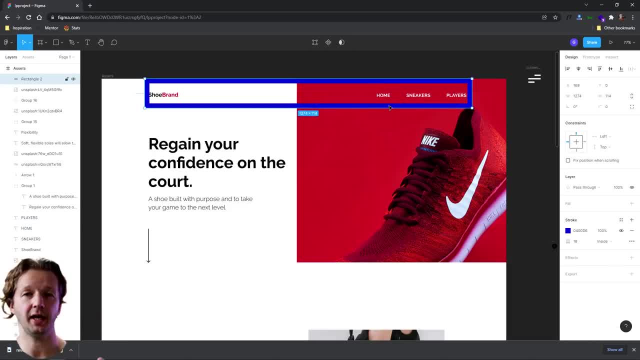 because that will. that will influence how you structure your html. so, in order to have two columns, you typically need to have a parent container. all right, so this is this blue element is a parent container and, if i duplicate this again, we have another element in our html for this, right here, the logo. i know that looks kind of. 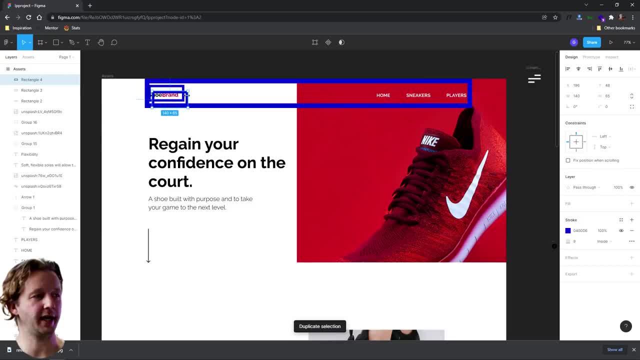 bad, and then i will duplicate that and we'll drag this one over here. we're gonna have another element that contains these individual elements. so when you're structuring your html, think about it like blocks, like rectangles all over the place, because that's essential. that's just essentially what it is. that's how the browser interprets it, but then we can style it up. 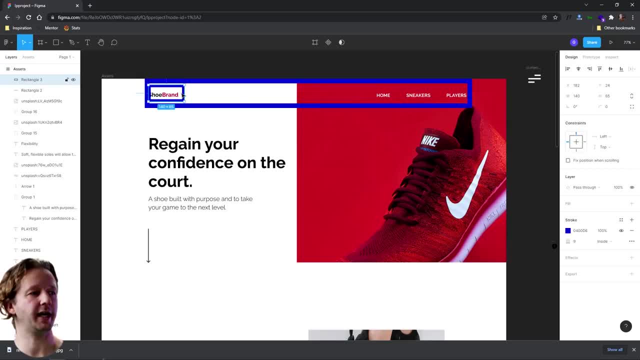 with css and make it not look blocky like that. all right, so let's close that out. and there's also something called semantic html, and it simply means use the html tags that are relevant given the context of what's happening happening in your html document. so for here we're going to give. 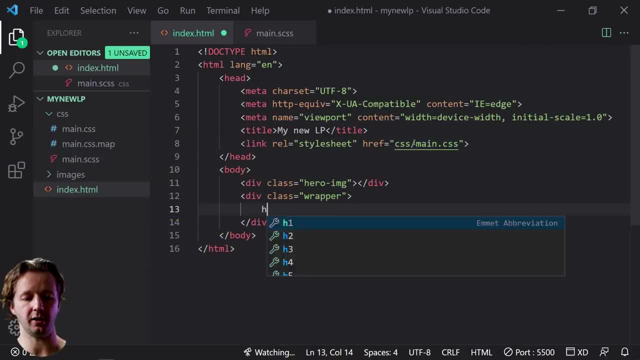 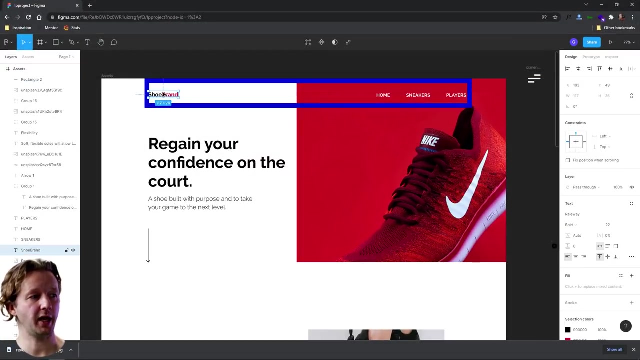 this what's called a header tag, and it's very simple. we simply put in header, enter, inside of here we put the two columns, so the first thing inside, so this, think of this header as we revert back to here, this rectangle. right here now we have, starting from left to right, the first. 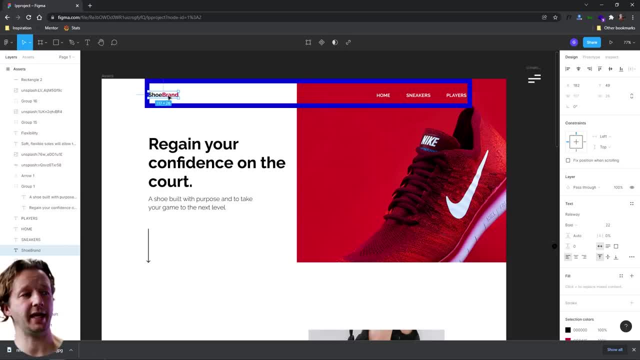 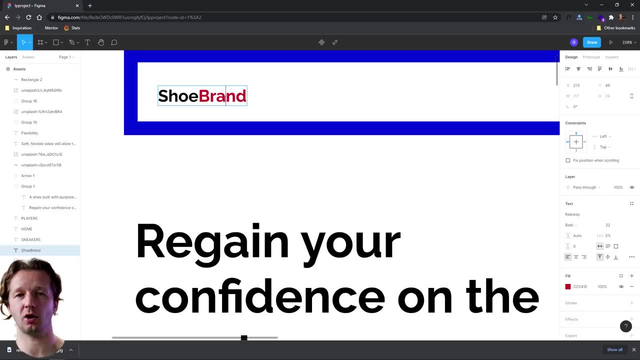 thing that shows up is going to be this logo. now, this is a logo that is purely a wordmark logo. so an identity and logo design- a word mark is just type. now, the reason I know that is because I'm also an identity designer. once upon a time I did over 2 000 logos, but this, typically, you're not. 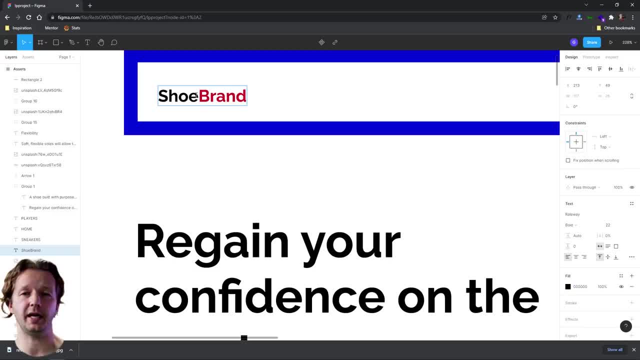 going to have a logo like this, though: usually you're going to have an svg file, which is a scalable, scalable vector graphic file, like an asset that you put in that folder. it's an individual graphic file that hopefully the company will provide you with, and that is their logo. that. 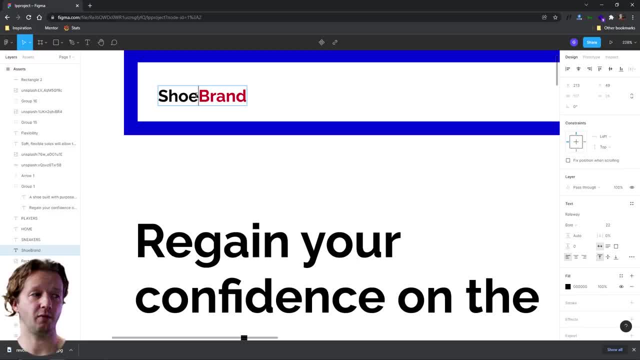 they want you to use. so typically you would use an image tag for this, but for us, because it's just purely wordmark based and it's going to be based on the, the font that's used, used here already in the document, we can just use and make it a link I, and so we'll use the a tag. 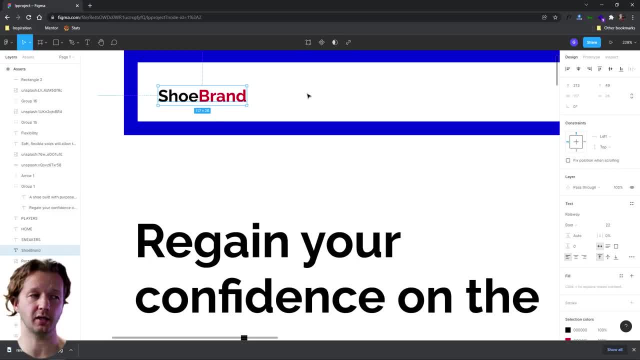 all right, and that's how you create hyperlinks or people, the things that people can click, because another typical pattern is the logo should be clickable and it should take you to the home page or the dashboard or whatever it's associated with. so we're going to put in a enter. 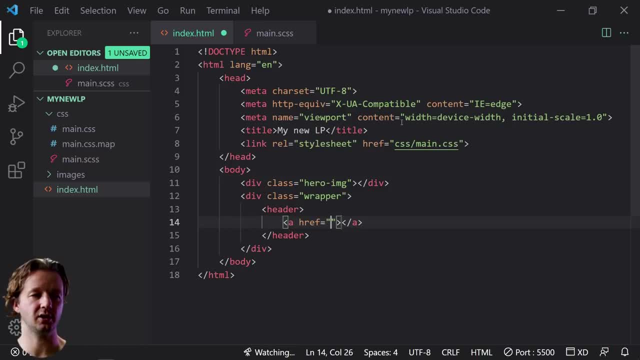 so remember, get used to that using those end abbreviations it makes writing HTML a lot faster. so the href is the location of where I'm. you want somebody to go when they click on it. this could be to an entirely different website, like websitecom, whatever, or it could be into a I, a different page. 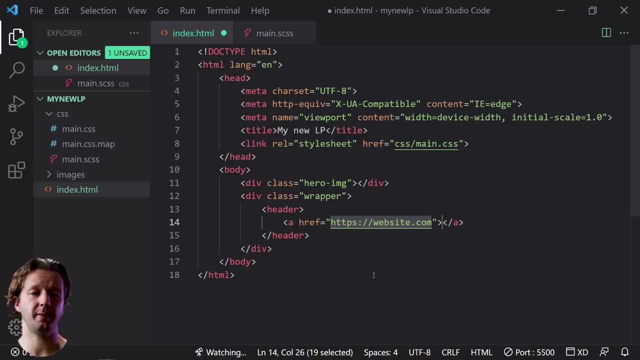 on the website. so in our case this would just be. in most cases it would just be um the actualcom of the website. so if this website for designcoursecom, I'm putting designcoursecom right here for the other navigation links that that show up. we have three of them. you could also. 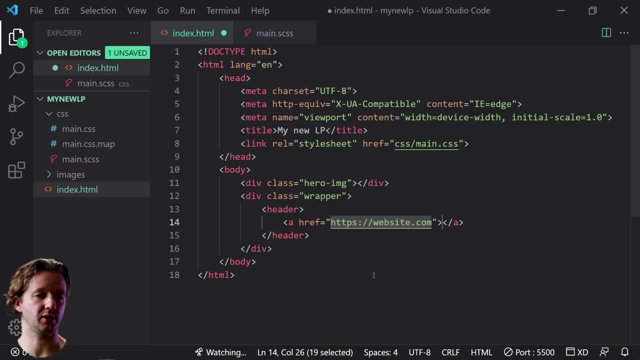 put this to a different folder on the website, so something like about. you could do that, or can go to individual HTML files like abouthtml. you have different uh types, like you could do PHP, although that's old school, but anyhow, that's just for taking you people to different websites or 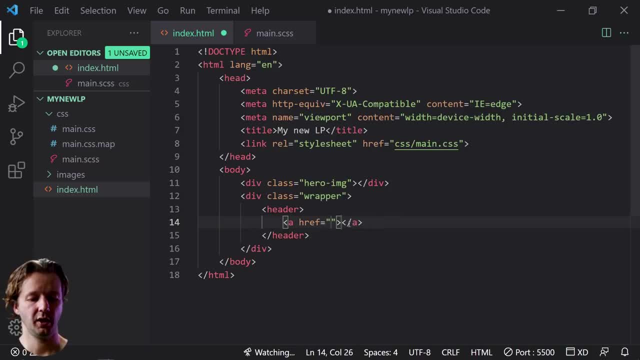 different pages on uh on the the same website. so if you don't want to go anywhere, just put a hashtag, or there's also ways to take people to different parts of the same HTML document. it'll scroll down automatically. you've probably seen that and you do that through tags, so we just put in like section. 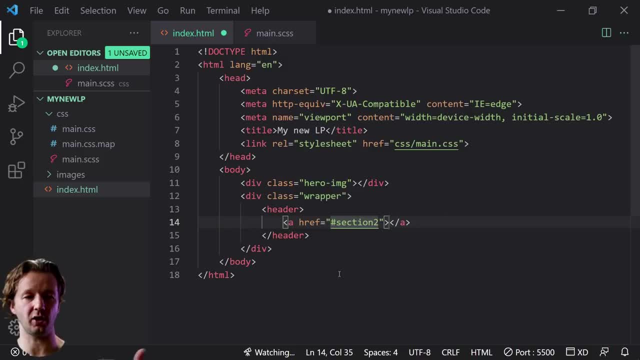 two or something like that, and then you'd have to create a reference to section two somewhere else in your HTML document. all right, I know this is a lot. it's a crash course. so we're just going to leave this empty. that means nothing's going to happen, not empty. we're gonna put a hashtag that. 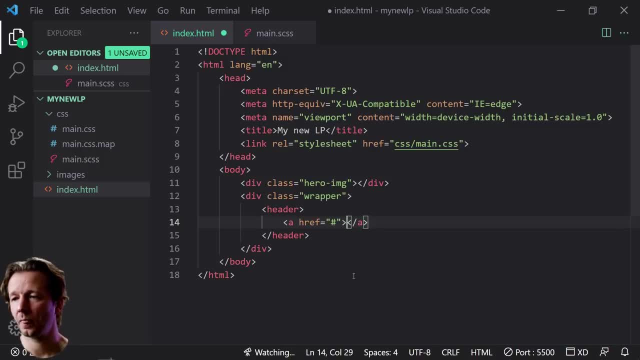 means nothing's going to happen when somebody clicks on it, because this isn't a real website. so now we're going to also have a class attribute: class equals logo. this class attribute will allow us to reference it in CSS to style up to make it look like it does in the figma prototype that we've been looking at now. 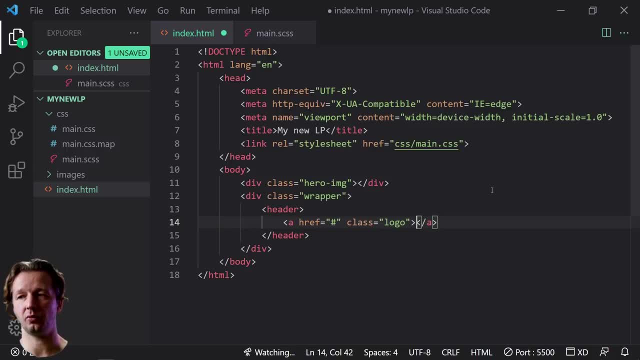 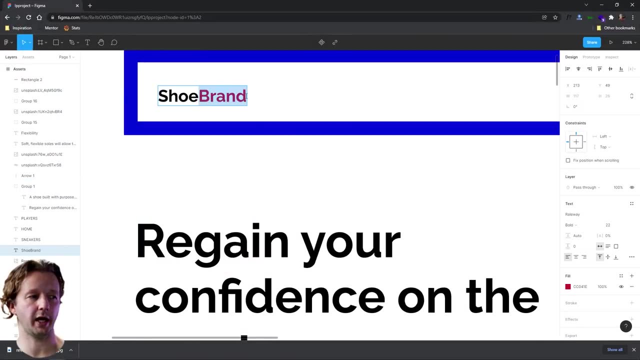 inside of here we have the content section, and so inside of it we're going to put shoe and then notice for a second: if I come out here, notice how one word is red and the other is black. well, we need a way to make this red, just brand right. 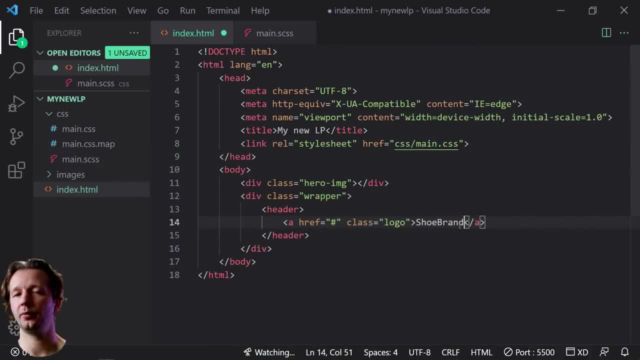 so to do that, we can't just put shoe brand. we want to be able to do that. maybe with JavaScript we could, but that would be silly. what we would do is wrap brand in its own element as well, and a great element for that use case is span. so we take our span, make sure we put brand inside of it. 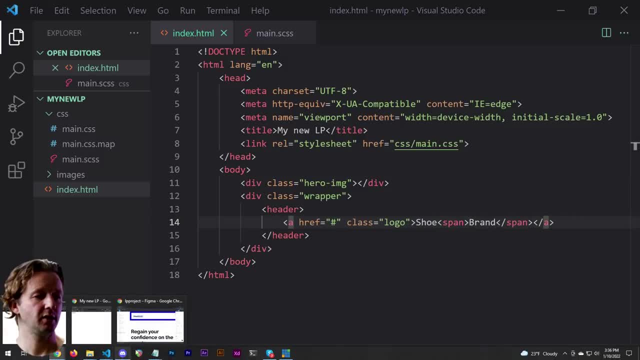 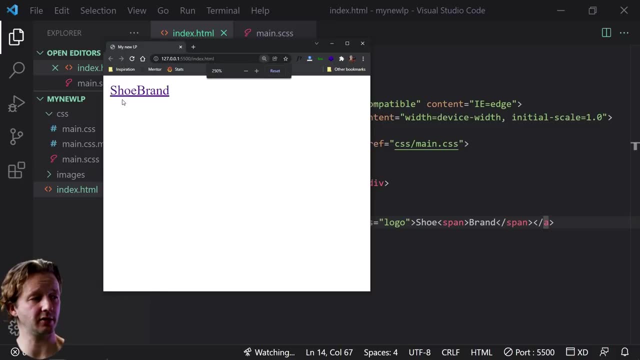 there we go shoe brand and by default, if we look at the result it'll say shoe brand. it styled exactly same, as you can see if I zoom up a little bit. but that's because we haven't styled it differently yet and span doesn't have any inherent browser styling. that's applied to it. That's something. 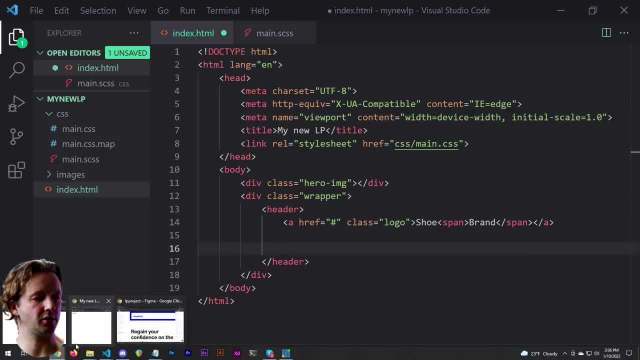 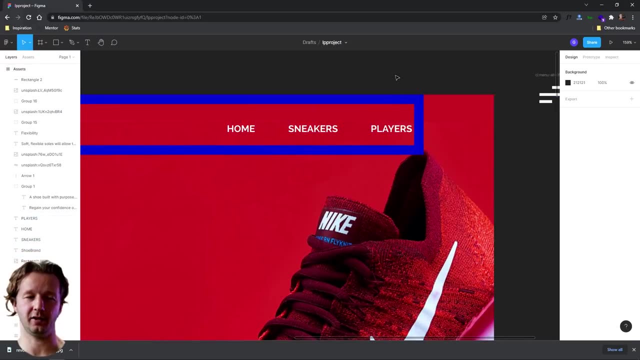 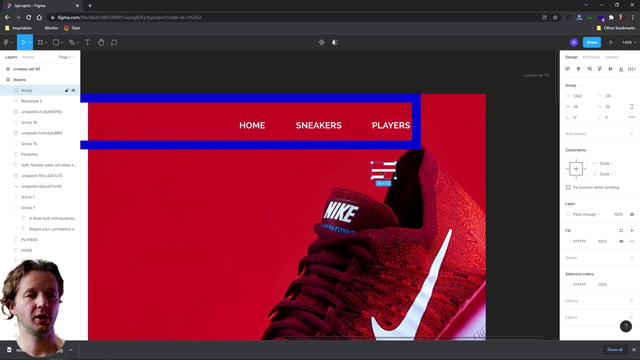 that we'll have to do Next up. if we refer back to our document here we have this element: home, sneakers and players, All right. So we also have to account for the HTML that will inevitably show up right here for mobile. See this little icon, which you've probably seen. 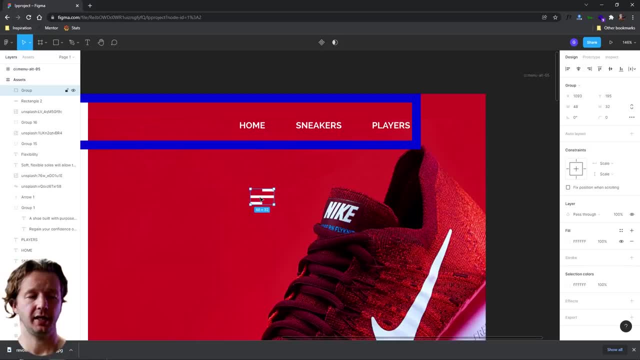 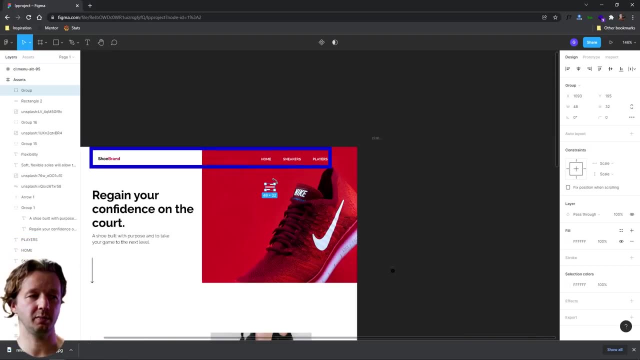 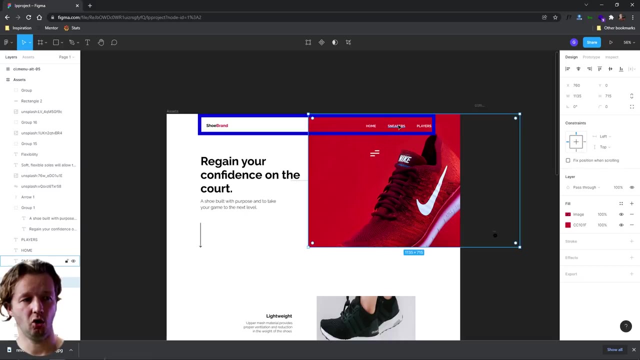 versions of like. when you're using your phone and you visit a website, you tap on it and then it reveals a mobile-based navigation of these elements. Well, that's because you simply just don't have, in many cases, enough width or space on a small phone to show home sneakers players. 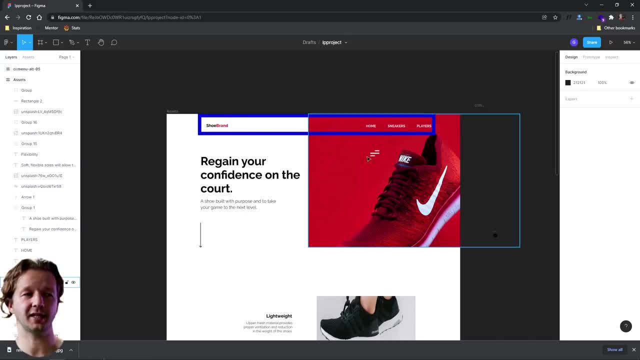 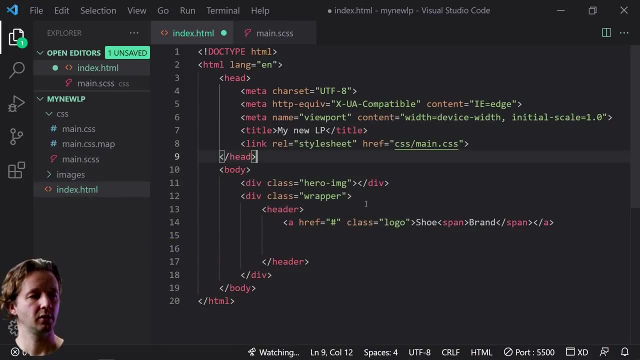 and maybe even more, along with the logo. So that's why we have to account for the HTML, that we have to account for This. it's kind of like making the navigation dynamic, So we have to create an element for an HTML for this and also for these. So let's do that right now. So what we'll do is we will specify. 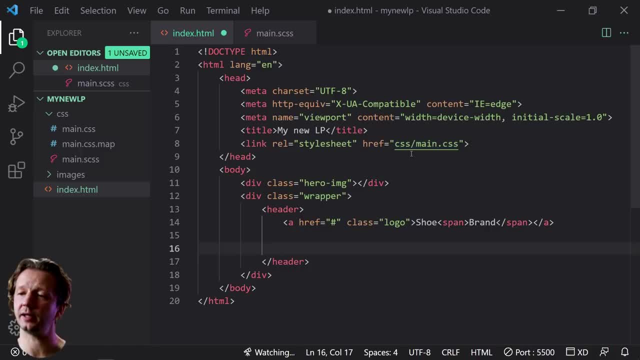 the first element. Actually, it doesn't really matter which we make first, that hamburger menu or the actual navigation, So let's do the navigation first. So for a navigation like this you're going to wrap it. those elements, those three elements which are: 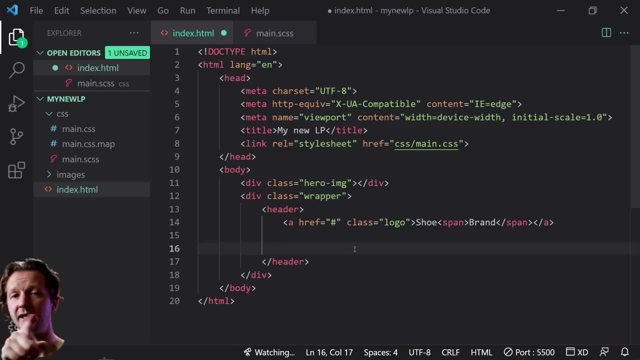 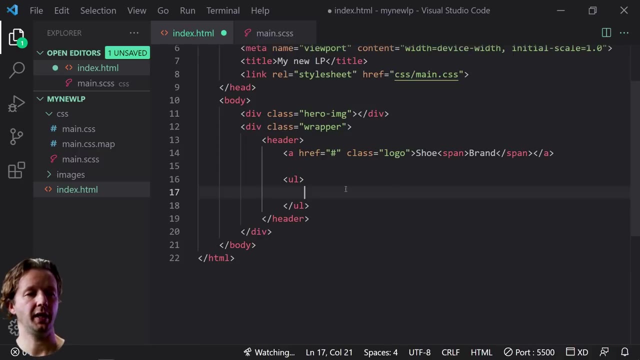 currently on a desktop in three columns. So remember, we need to give it a parent container. We're going to wrap it in an element called unordered list, All right, So that's an acronym, obviously, UL for unordered list, And then we're going to put three elements inside of there. 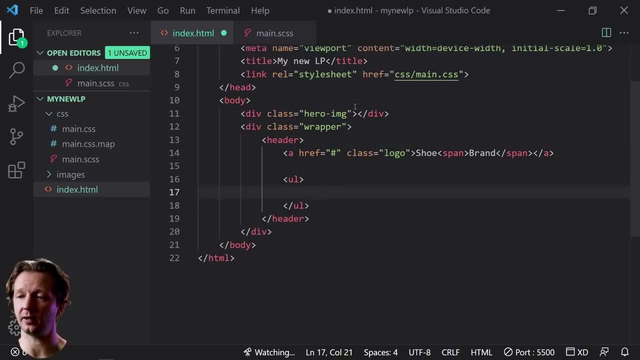 And so because we have three links, we have home, sneakers and players. So an unordered list excepts sibling or nested HTML elements that have to be denoted as LI, list items because it's a list. So list item one, we just hit LI, hit enter And then we put a link. So remember, 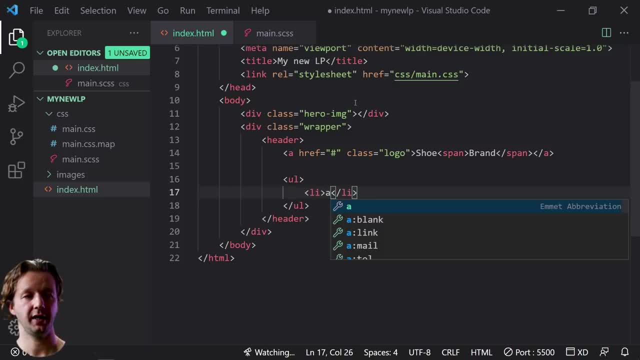 to create a hyperlink. we put an, A element, hit A hit, enter inside of there And then we're just going to put the empty hashtag because it's not a page, It's not real. Typically you might put something like: you know the actual website address because this is going to be a page. 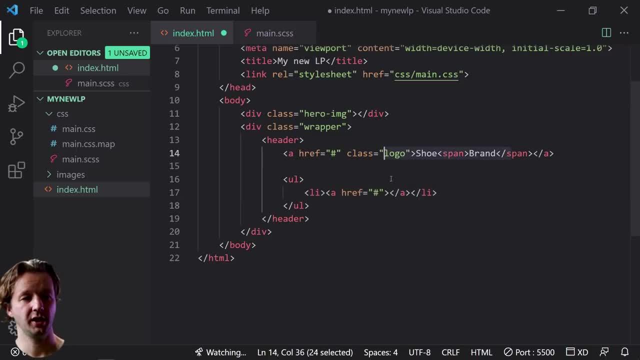 This is going to be a home link as well. So we link the logo and we put a discreet home link as well. And there's been usability studies about this. People expect to see a home link and they also expect to be able to click on the logo to get to the homepage. So inside of here, we just put: 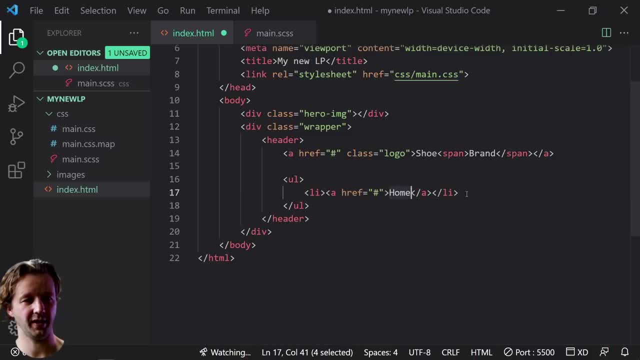 home for the content. So hopefully that makes sense. Now, typically you could, if you wanted to, you could kind of separate these out. I don't like to do that. I just put these elements with links on the same line, just to save space. Now another big handy feature here. 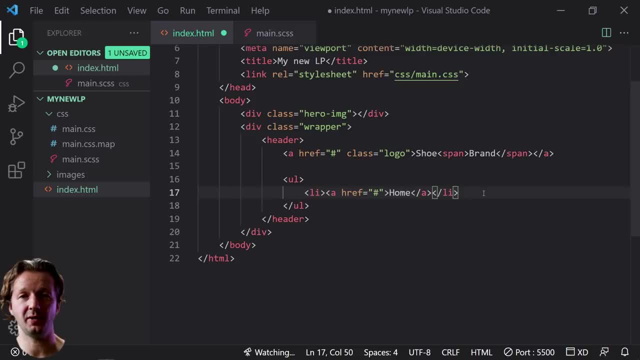 in visual studio code. if you want to replicate or copy and paste elements quickly, we could take everything left, click, hold it, hit control C and then control V. But a better way is shift alt and down arrow key So fast once you get it into your muscle memory. So now we have three of 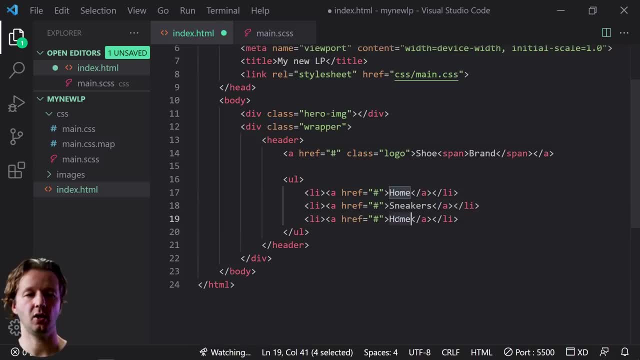 these and we can specify sneakers here and then also All right. So there's one thing that I forgot. I forgot a certain element that I should not have forgotten. I remember how I said: we need to wrap these elements. I, we do have these wrapped up in. 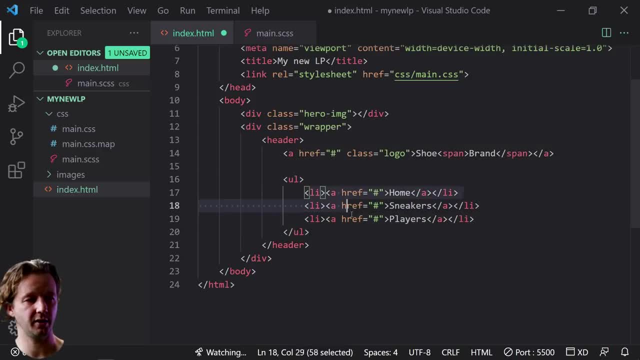 a parent container or a parent element of UL, these three, but I also want to wrap- and this is for semantic purposes purposes- this entire element right here and our um navigation or or I'd call it, a little menu icon within a nav element, which is a semantic element that will help screen. 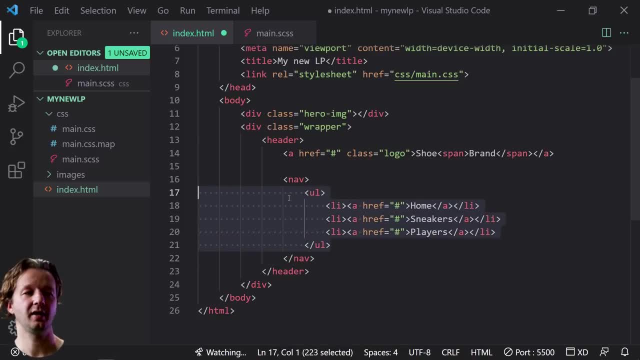 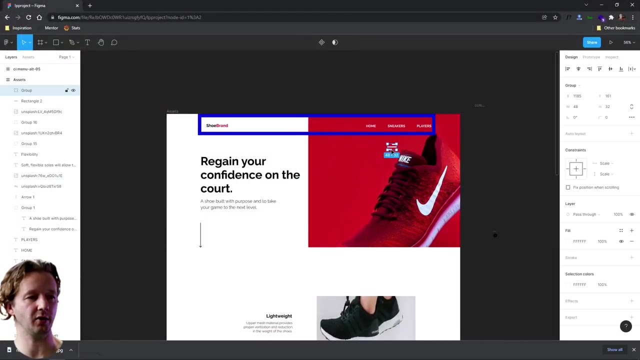 readers understand that this is a navigation and it will say: you know, audibly to the person who's using a screen reader that this is a navigation right here. So we've wrapped that up and we could also put in that menu, And so that menu is an illustration. It's an SVG file, right here. 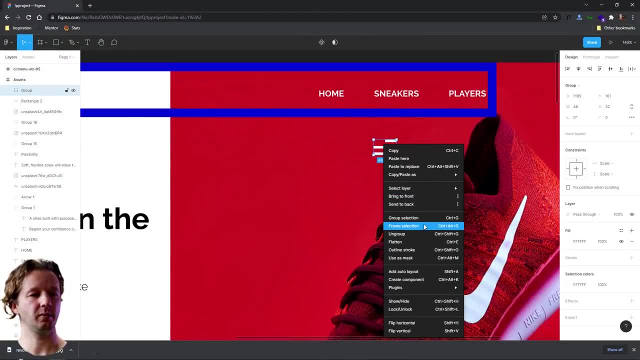 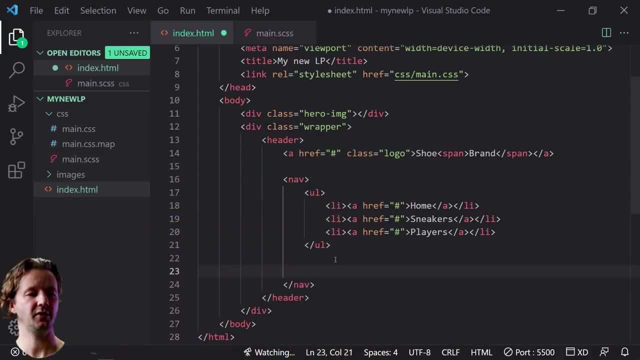 So if we click on it, all we have to do is right click And then we'll Copy, slash, paste as SVG. SVG is short for scalable vector graphics and it's not rastered. So when you're you're, you're considering, you're talking about graphics in general. they fall under two. 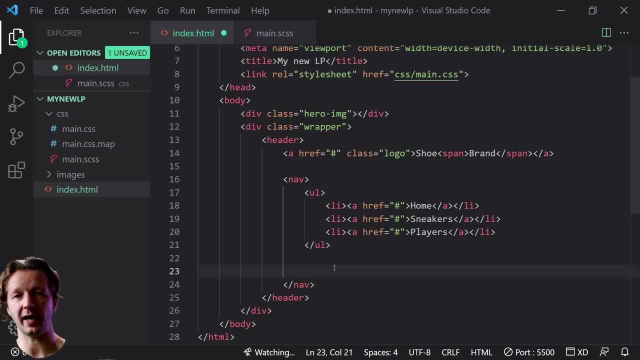 categories: It's it's scalable or it's vector or it's rastered. rastered is like when you've seen photographs sometimes are really pixelated and they look horrible. but photographs can only be rastered. but this is an illustration, So 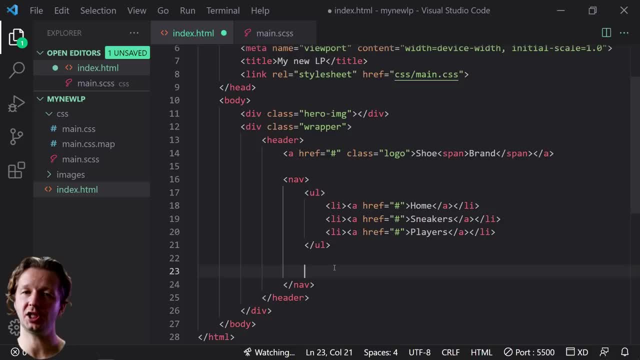 It doesn't make sense to make that a rastered image, because an SVG is code And so we can scale up the size and SVG however large we want and we'll never see blurriness or pixels. So we're going to paste that control V right there. So that's what it looks like. SVG is just code. 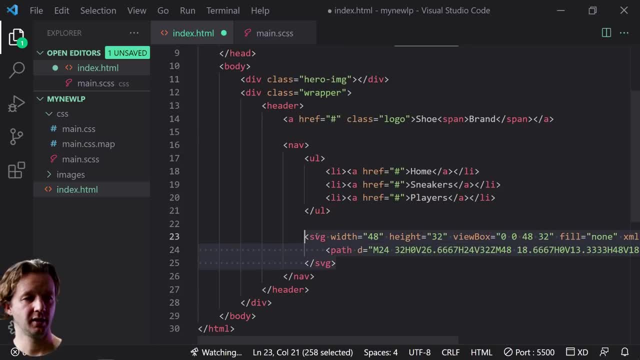 All right That we can actually paste into our HTML document. So that's right. There is looking good. Let's give it a class two of close so that we can reference and style And then scale it in CSS in the future, And let's also get rid of width and height, because we can. 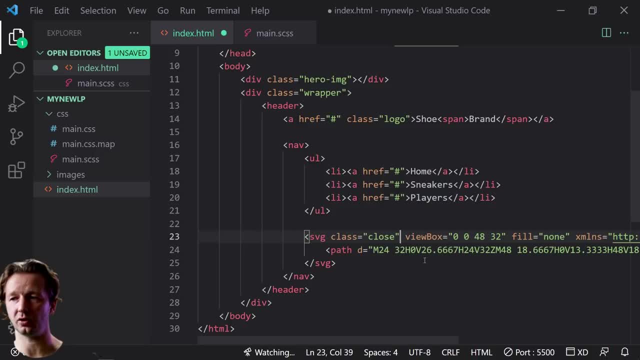 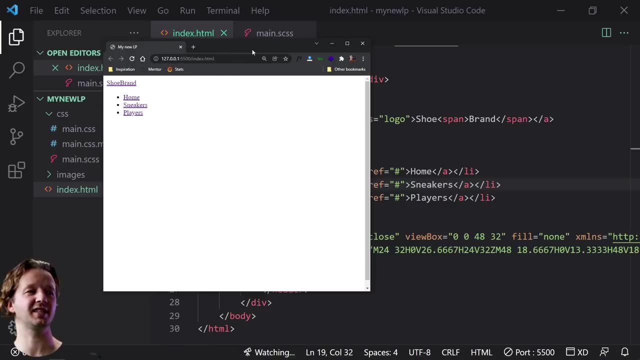 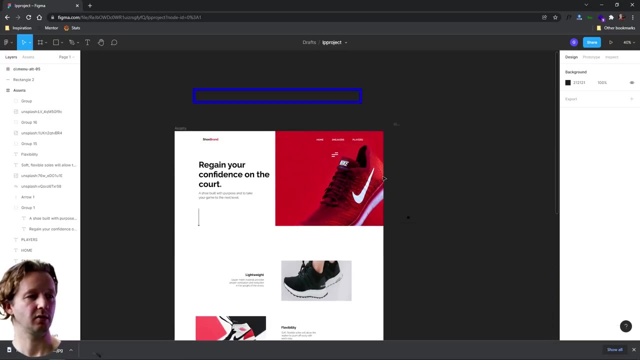 set that in CSS as well going forward in the future. All right, So that's looking pretty good right there by hit save. When we look at our HTML document at this point, it looks but ugly. it looks nothing like what we have going on here, right? Yeah, That's the beauty of CSS, because 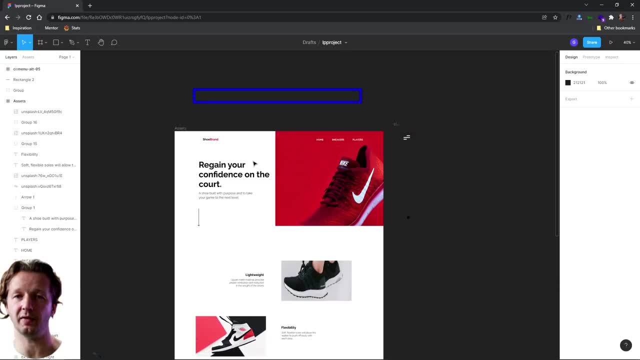 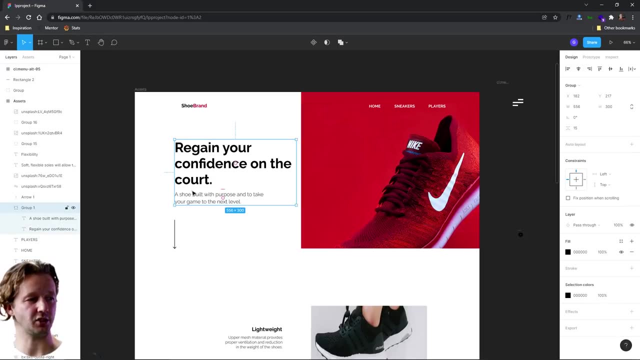 we're going to be able to transform it into looking like this Once we get all the HTML ready and we start writing our CSS. All right, Next up is going to be this section right here. So this is a part of our hero section, especially on desktop. This: 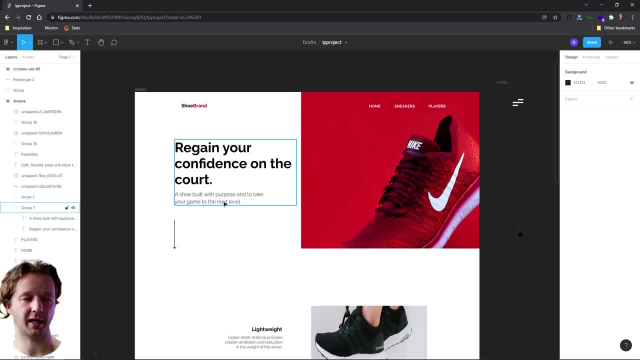 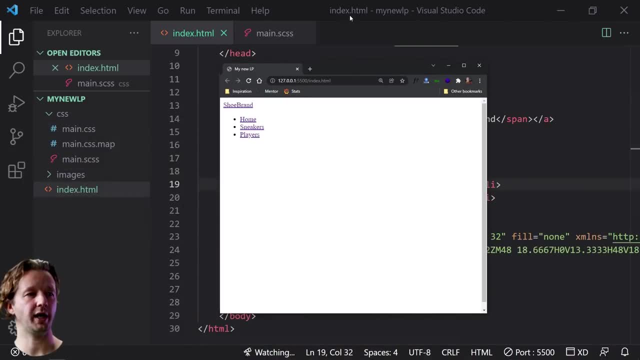 is the main part. we see, and we have a headline, a sub headline, slash, description, and this little down arrow which again is an SVG element as well. So let's go ahead and write the necessary markup for that. So, outside of header, we're going to put in a section. 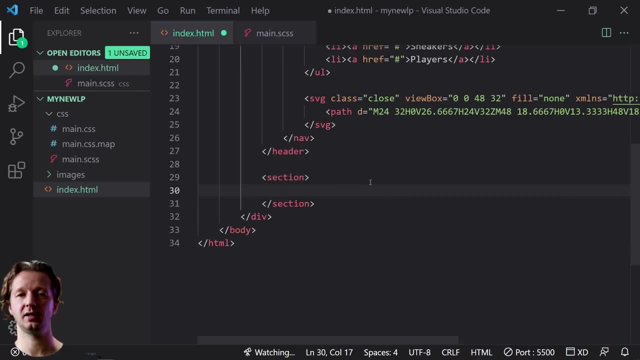 Element. So this is just basically a section of content and this helps structure and organize your entire sections, essentially, And we can reference this section in our CSS to give it white space away from other sections and things like that. So we're also going to give this a 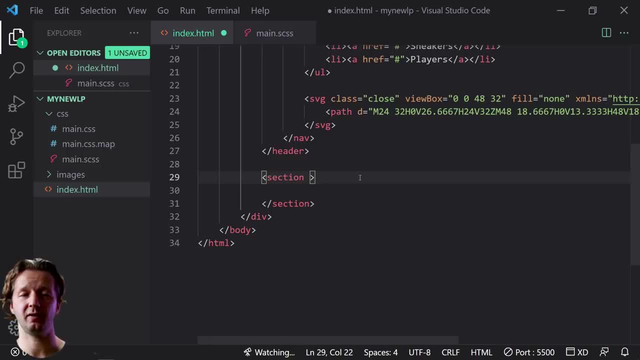 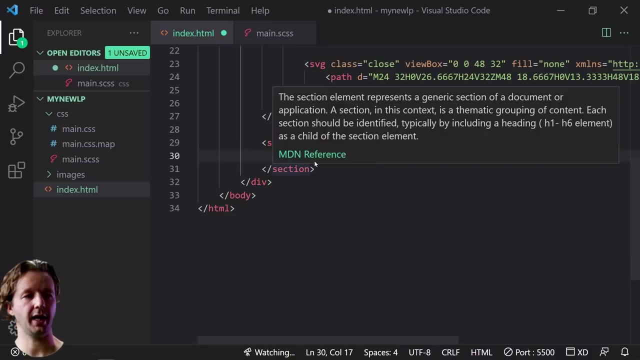 class and we're going to give it a class because we're going to have two sections. We have that top section and then we have the bottom section down there. So we're going to do class equals hero. And inside of here, what falls next is that headline that we have. So we're a headline. 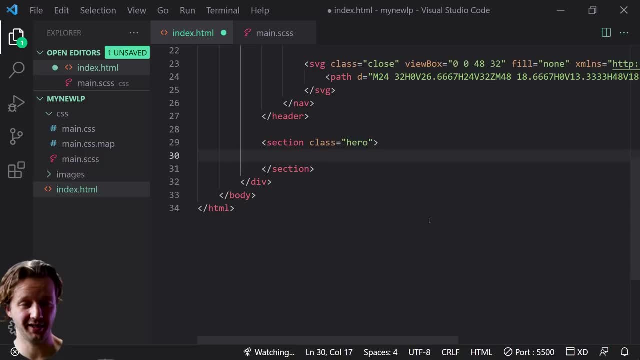 specified, usually million times out of a million times at H1. And you have H1 heading one all the way through. heading six- H1 is the most important And usually that's in your hero section- is the big bold text that grabs the user's attention, essentially. So we're going to put regain. 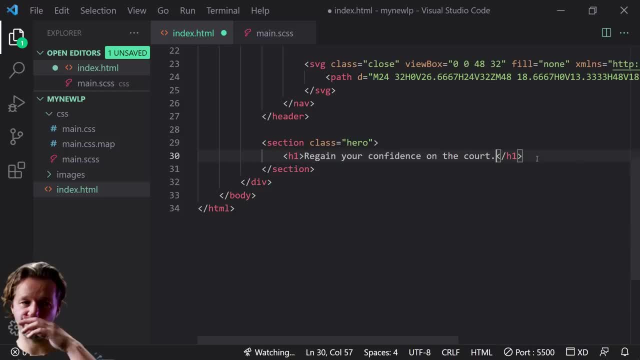 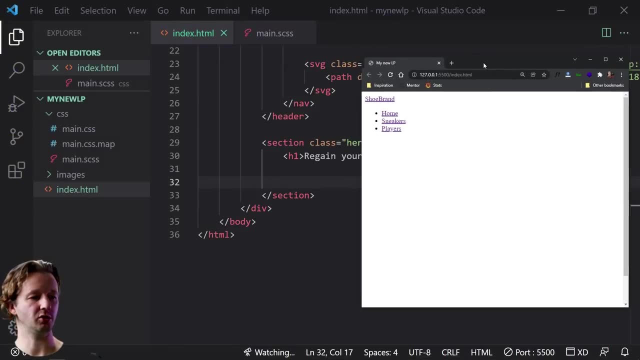 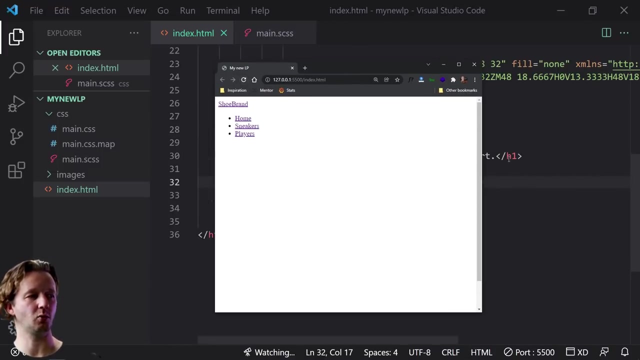 your confidence on the court. There we go Very solid. So now if we hit save and we go back, we don't see it. What is happening here? All right, That's a little bit strange. So sometimes weird things like this happen. It's not actually showing up in my browser, because we should. 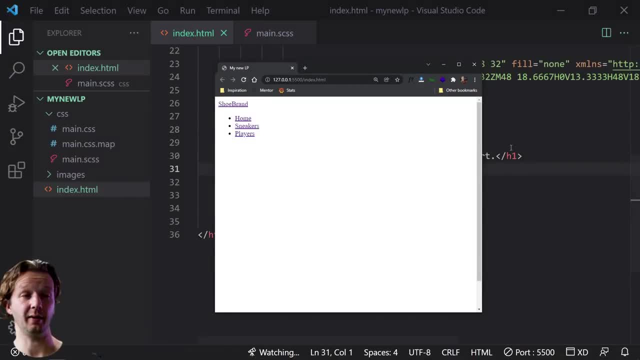 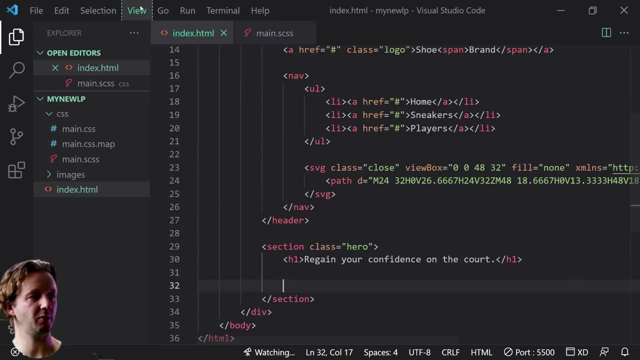 certainly see that type, And I'm actually confused at this point, And so I'm going to sit here a little bit and figure out why It is not showing me. Maybe we can go to view terminal. All right, It's not running in the terminal If I right click, open with live server. 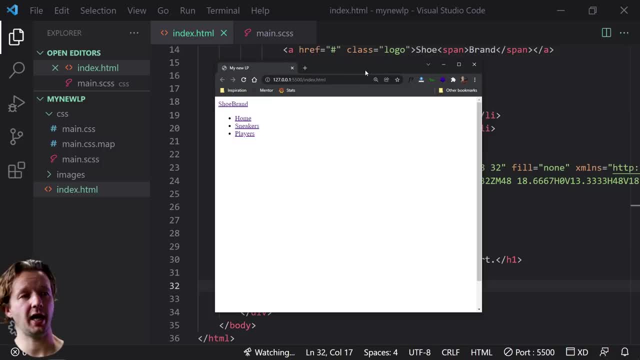 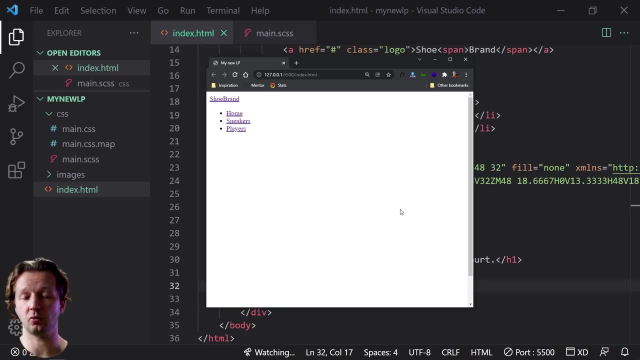 it's not showing up there. Now, what we could do when you have Firefox or Chrome, which I advise using when you're working with web development- hit control, shift I or F12.. And this will get up this little dev console. up There it is. It was way down there. 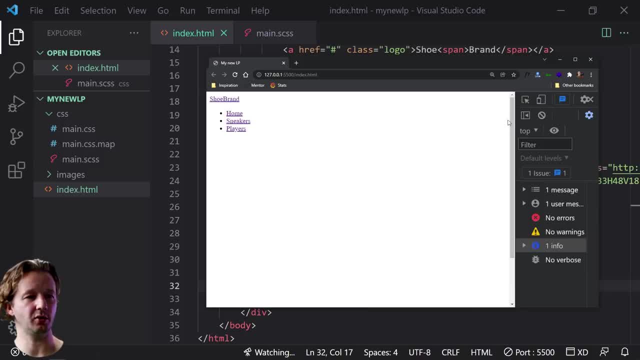 Now, why is that? Well, what we can do is we can use this little element right here, and this will help us see, when we hover over different things and notice this big area, Why is that there? I can tell you why it's there. Now I understand, because I didn't know. 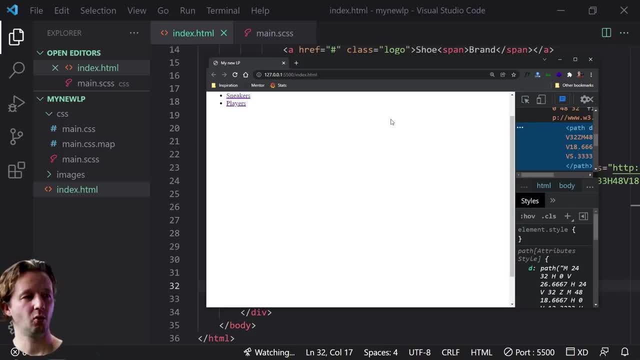 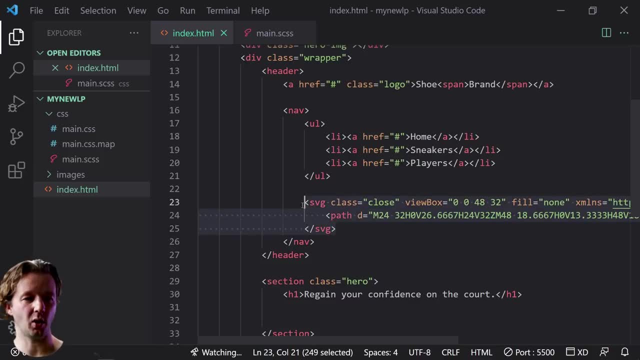 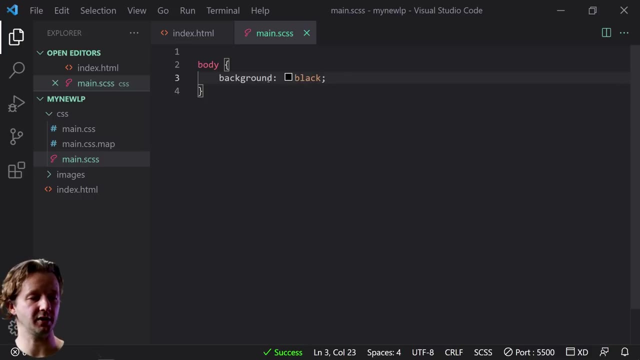 what was happening. See where it says SVG close. Well, that is actually because of this. We don't see it because it's white on white, All right, So that was a white little hamburger menu. Now, if we change this background, so to take our body background, let's say black, for instance- 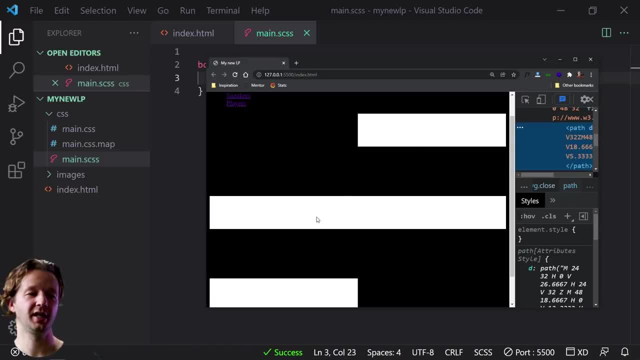 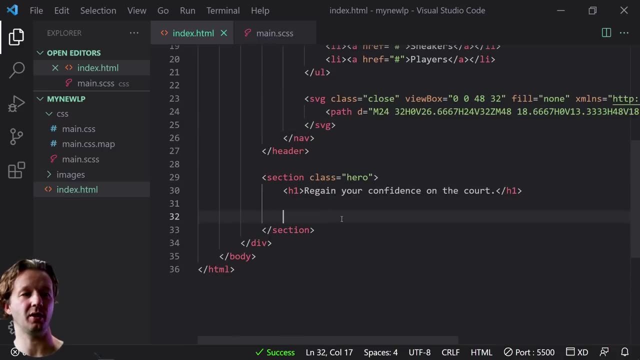 and we save it, we will now see this huge, And that's because we remove the width and the height attribute, So it's just making it really large by default, And so that's what was happening there. So nothing to worry about. We can delete that, come back here and just keep on writing our 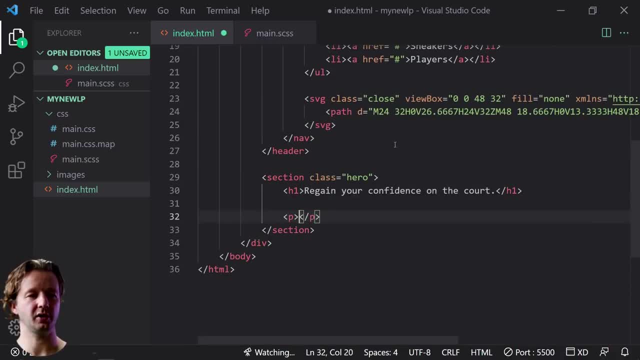 HTML at this point. So now we're going to have a paragraph, because we had a paragraph underneath subhead, as it's called Sometimes. we're going to give this a class as well, because I want to style this individual paragraph as well. I, and we're going to call it subhead for subheading and I'm 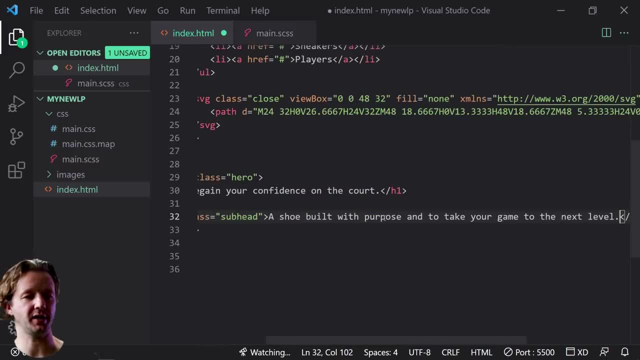 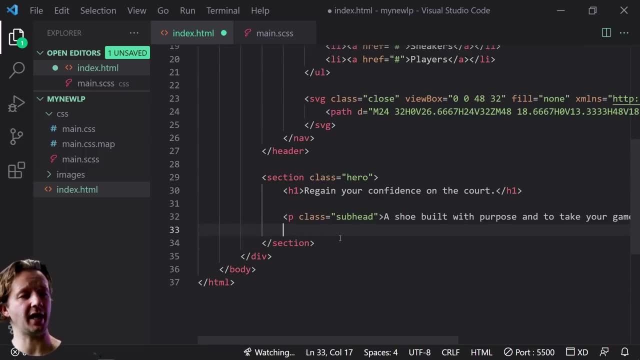 going to simply copy and paste this, So you don't see, you're not sitting watching me type this out. It says: the shoe built with purpose to take your game to the next level. blah, blah, blah. And then, finally, we have third element, which is that little down arrow icon. So what do we do? We 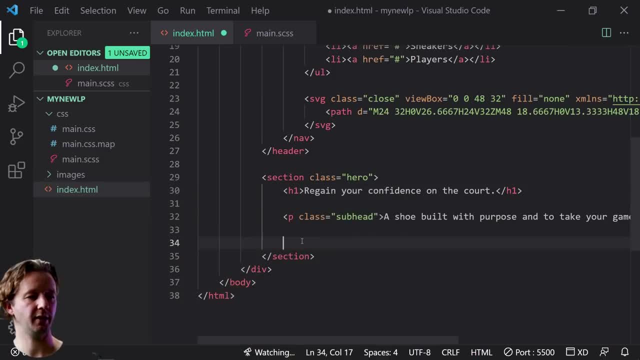 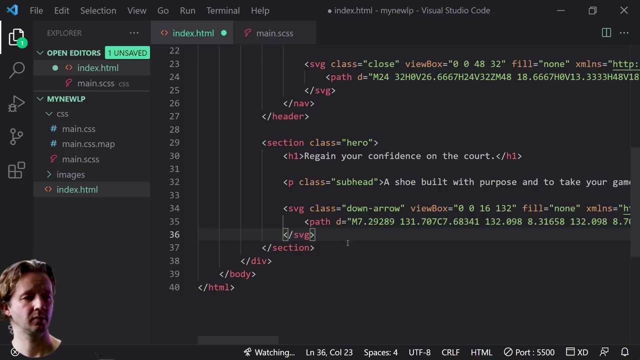 right click, copy and paste as svg and paste it in right here. Now, once again, we can go ahead and get rid of the width and height type in class equals, and this will be down hyphen arrow. We're going to make this actually animate as well. next up, And, by the way, 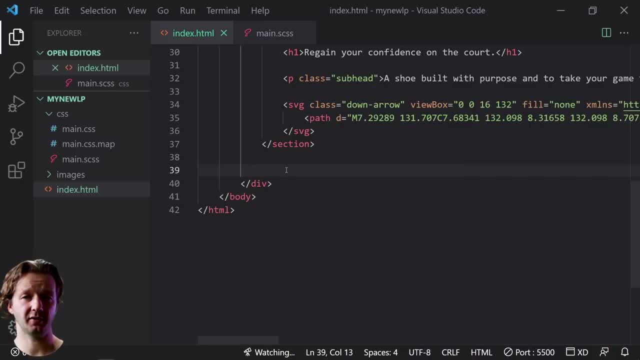 we're almost done with our HTML, So we're going to have another section And then that section is going to be based on this design that you see down here. All right, we'll do section. We're going to reference that class equals. we'll just say more info, or. 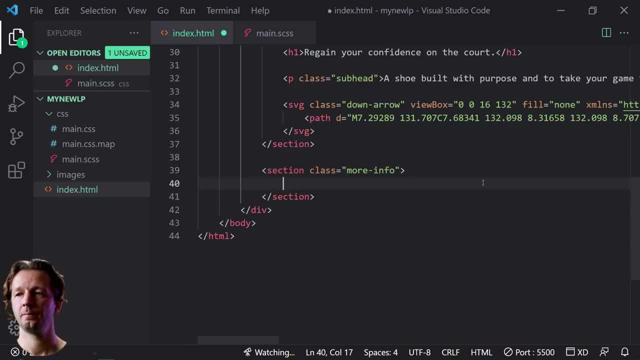 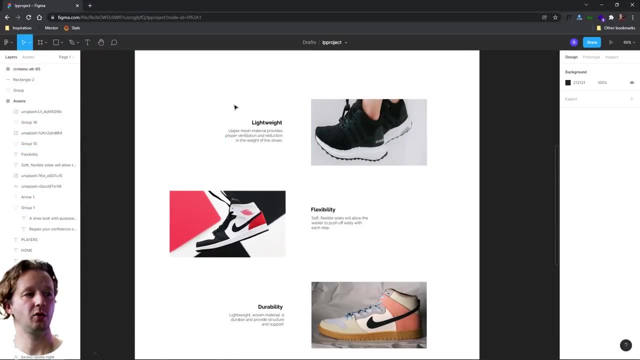 something like that, So you can put hyphens as well, And we have three elements occurring here. So again, let's get some muscle memory here. We have two columns per row. We have three rows and we have two columns, So we have a column here. Let's get rid of that. 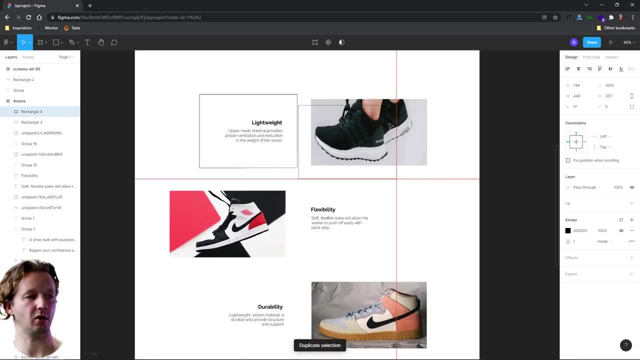 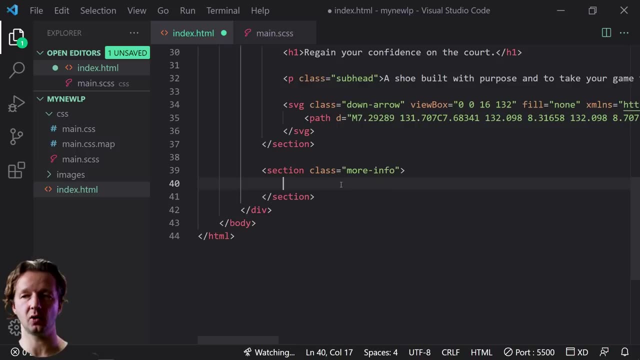 And then we also have a column right here, So we need a parent overall, parent container that contains both of these elements in HTML. Think about them as blocks or rectangles. So to do that, we're going to wrap each one in a div called feature, All right Inside of there. 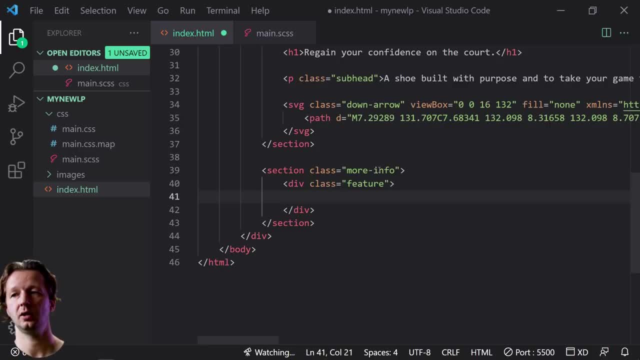 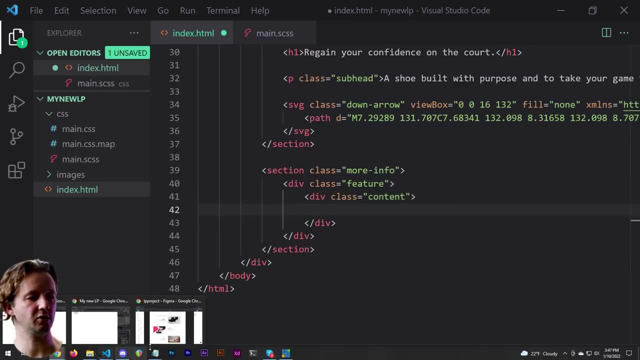 we're going to have two elements for column one and column two. That is going to be content and content. Because we're going to have two elements for column one and column two, Because, remember, look at our first one And this one's getting a little bit tricky. 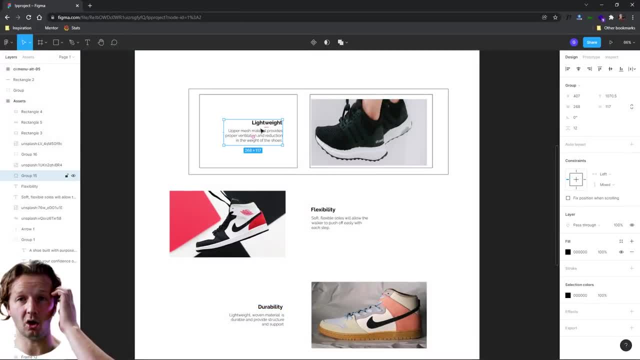 because the first element of the first column is our content- a title and a description, But then the next one. we're reversing it And then we're going to have this here and that there, But we're going to style it in our HTML so that all three of them, including the middle one, 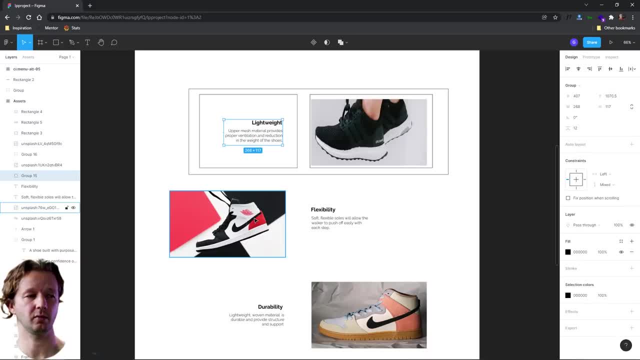 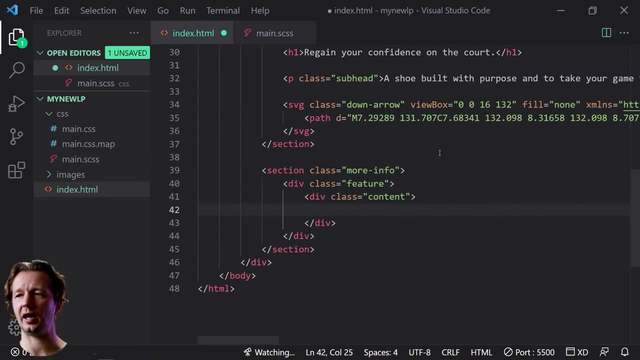 start with our content in the first column. But we can use CSS, something called the CSS grid, to take just this second row right here and reverse them with CSS- Very cool stuff, Exciting. So to create that title we could use like an H3 element. You can use multiple H2, H3, H4, whatever. 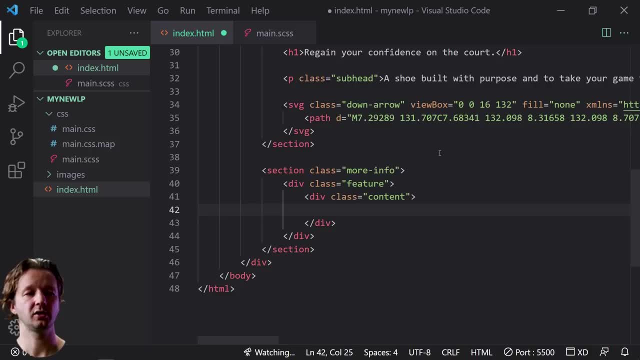 But we can also just use a paragraph element as well, which is what I'm going to do, So the Emmett way of doing this. we want a P element or paragraph element with a class We name of the class or the value. 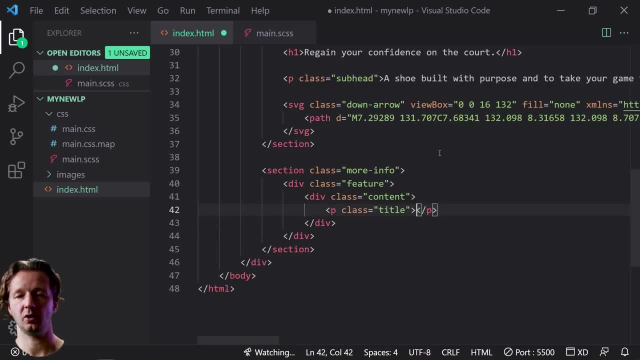 So we're just going to say title: All right. So inside of there we're going to say light weight. That was the copy for the first one. Now let's go ahead, shift alt down, and then let's go ahead and put in here. You can copy and paste this. I'm just making all three of them the same. 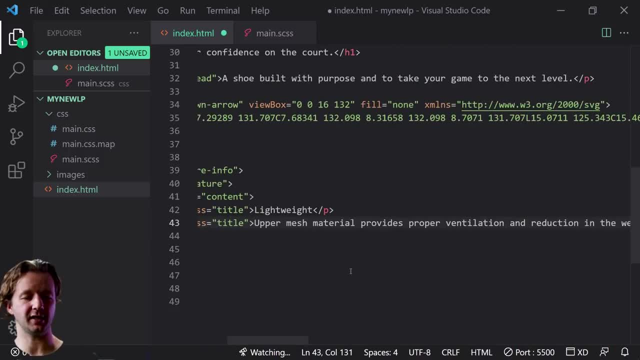 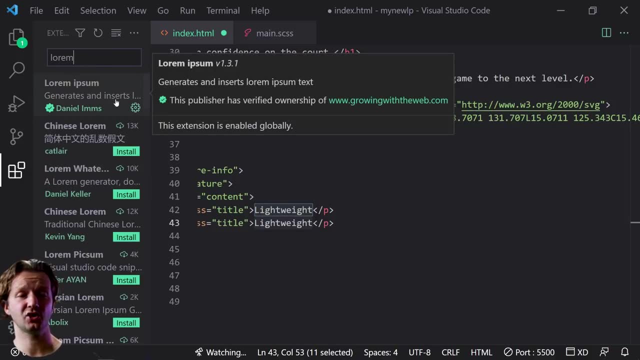 We just paste that right there Now real quickly, as an aside. you can go to extensions and you can type in L-O-R-E-M for lorem or lorem ipsum. I've already installed it. but what it allows you to do if you don't have actual, real text? 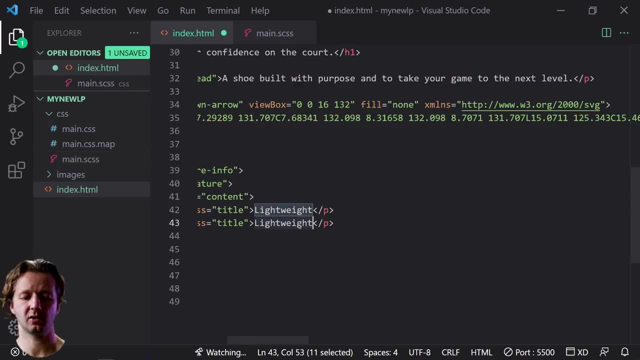 you just want filler Latin fake text, as sometimes you'll see it's called lorem ipsum. You type lorem and then how many words you want. So if I want 15, lorem 15, no spaces, And then we automatically get all of this gibberish that you cannot understand. 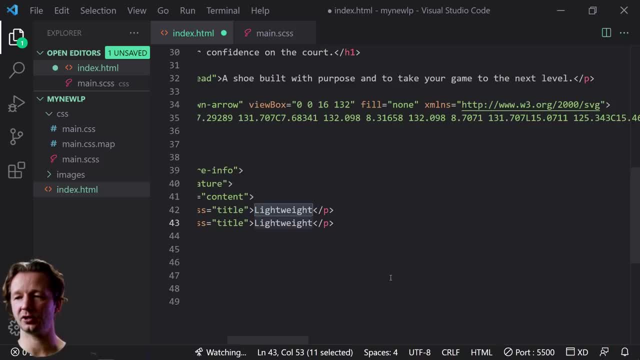 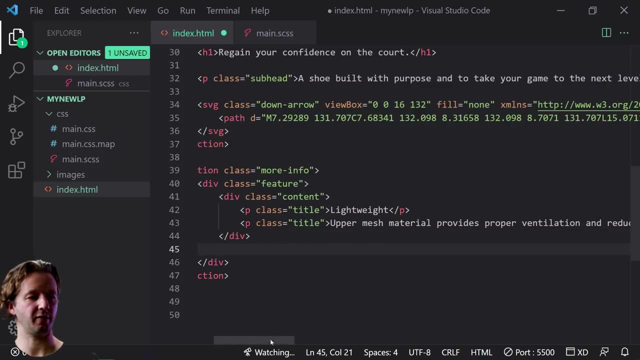 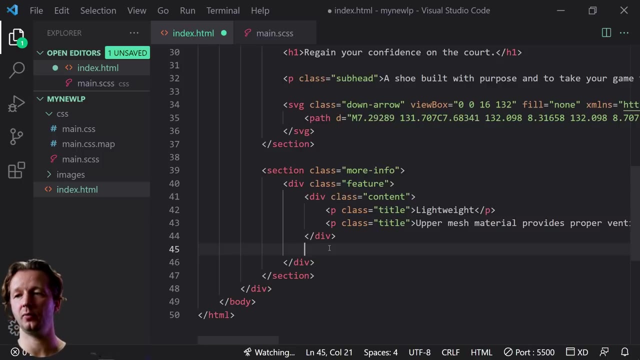 All right, So they have lightweight. So yeah, we have that, And then we have the image next to it. So we have our first element for our first column already defined within feature. Now we have to have the image, And this time we will use an image tag. So image. 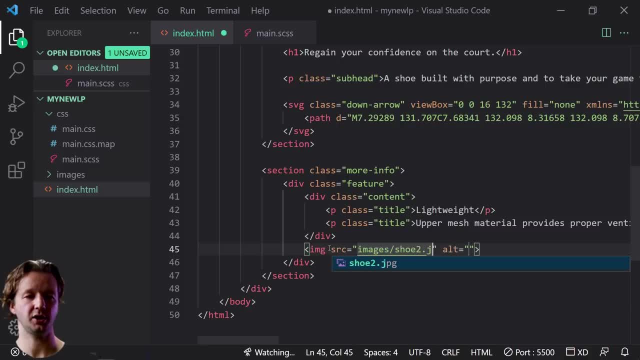 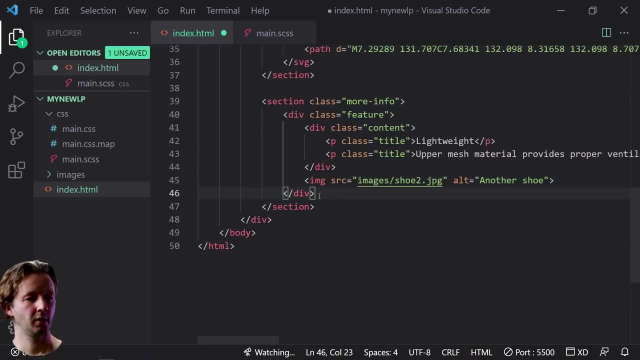 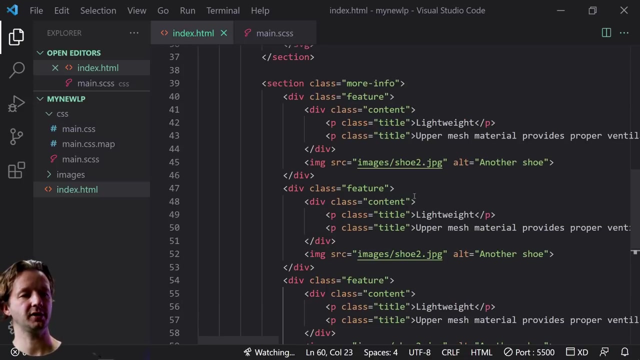 source equals images forward, shoe2.jpg And alt. you can just describe the shoe whatever it looks like, And that's it. So we copy all of that, the whole feature area, And then we paste it two more times. Now let's say that we need a way, though, for us to reference. 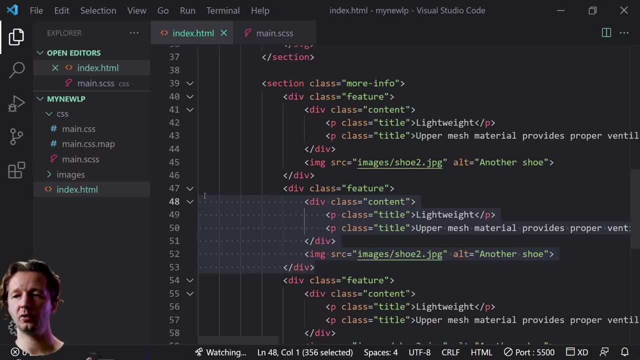 this middle column to flip those two columns. And the way we'll do that is, on the feature element we're going to put a space and we're going to add another class name So you can put multiple class names in the same class attribute. So this will this particular div element. 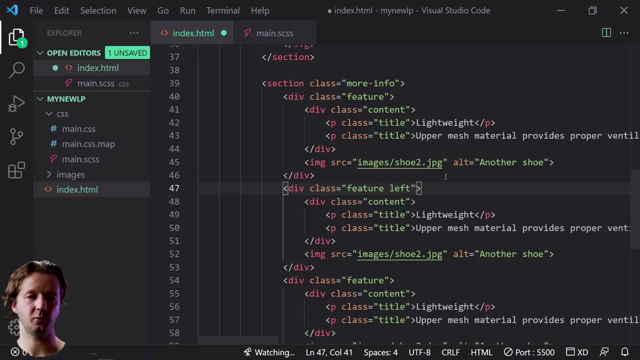 will have two classes feature, and also left. we can just name it left. you can name it whatever you want. you can call it flip, because we're trying to reverse, or you can go reverse whatever you want. so that's all we need to do there. and guess what? that is our html. that is the full html. 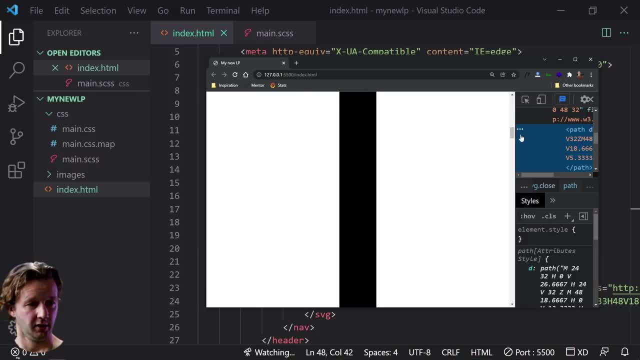 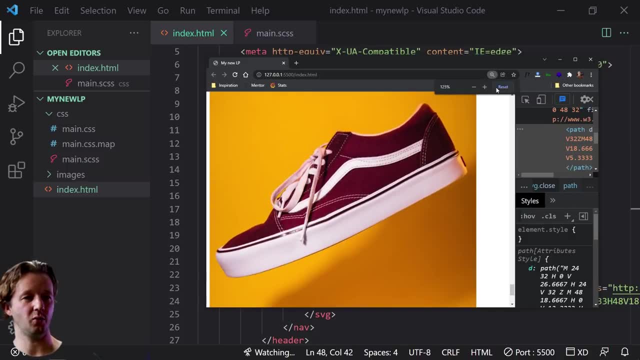 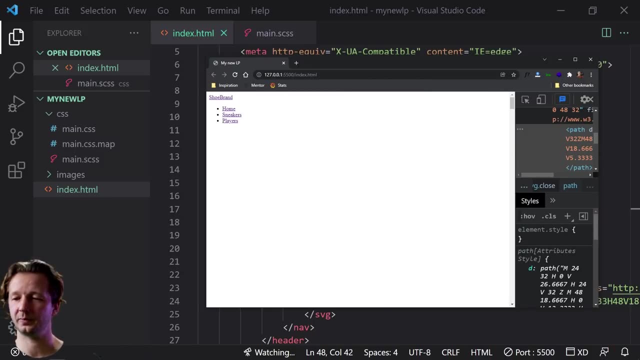 document and, of course, if we go look at it here, it looks really bad. look how big that down arrow is. so that that's why, essentially, you know, we want to use css to make our website actually usable, which is what we're going to do now. all right, so for the css portion of this video, which is: 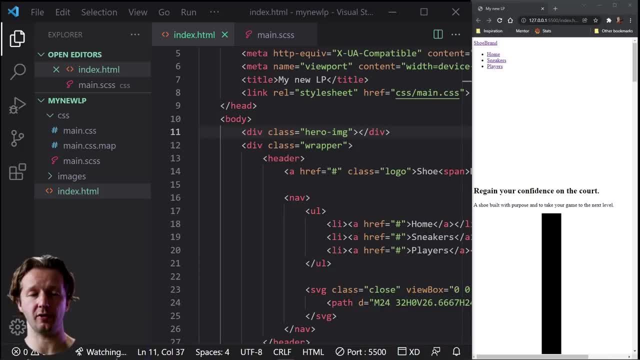 what we're going to be focusing on here. throughout almost the remainder of the video, i we, as you can see, my my format here for this layout of the the desktop. you can see i have my browser window right here, kind of like in a phone orientation, and then you have my 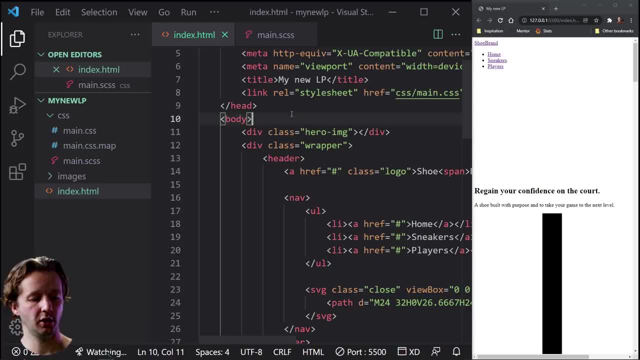 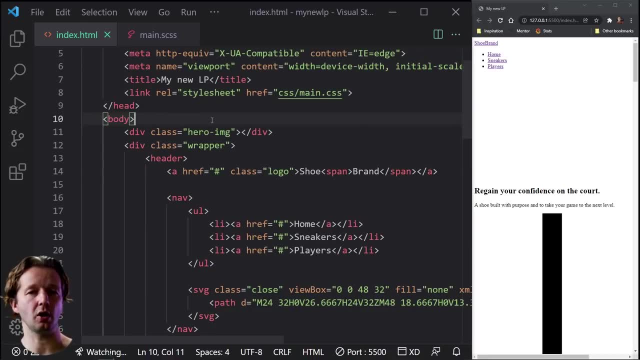 editor right here. and, by the way, to have more room to actually code, we can hit control b to hide that file area right here. all right, so you can always just toggle it on and off with the control b. now, the reason i have this over here in a phone orientation is because we're 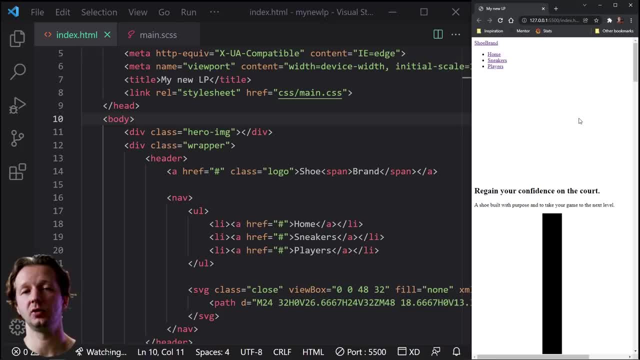 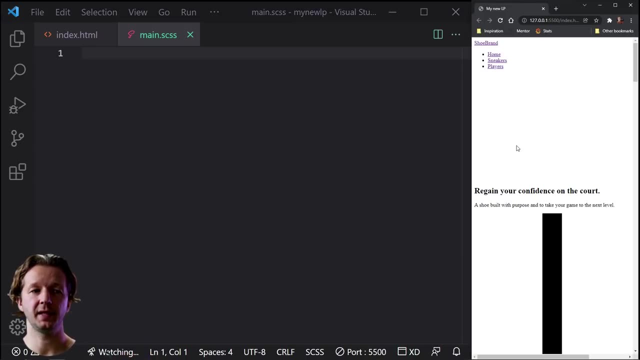 going to do something. we're going to write our css, which which is in a format called mobile first, so mobile first css. what does that mean? that means that all of this initial css, the initial CSS rule sets that we write, are going to be geared towards what this particular website or app. 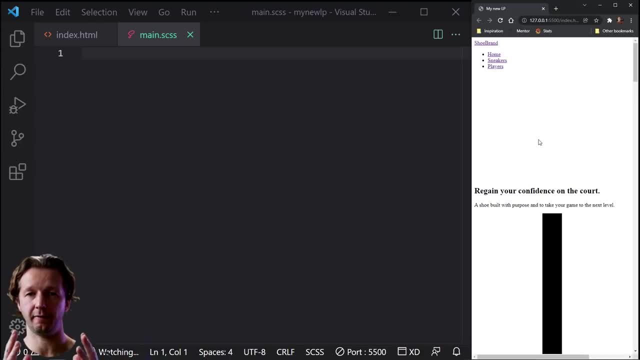 looks like and how it behaves and looks like on a phone or a device that you know has a little amount of width. Now for our actual Figma documentation, the link, the prototype that we're looking at. there is no actual design for the mobile view Now. typically you would have 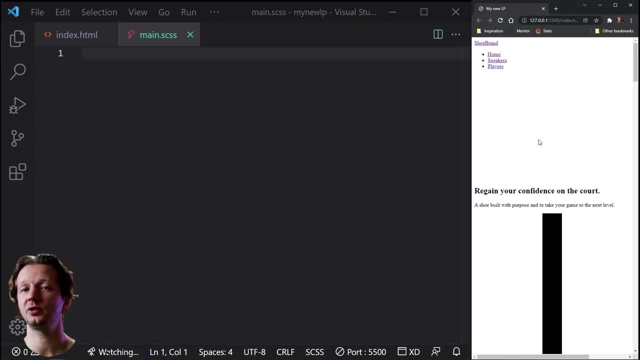 that. but we only have a desktop, So we can make some design decisions on our own in order to adjust things with CSS so that it works and looks well on a phone. All right Now. the reason we do mobile first CSS as opposed to desktop first CSS is because, when it comes to your CSS in your 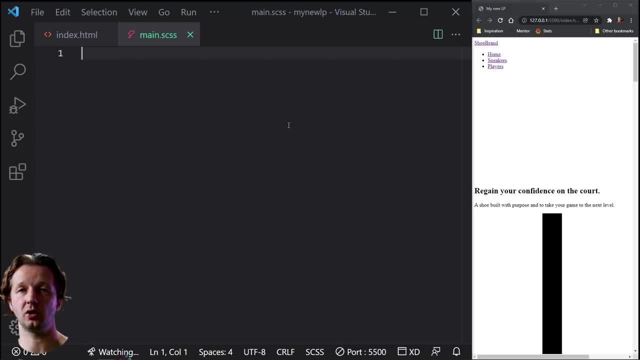 initial rule sets that you write that aren't a part of what's called responsive design or media queries. I know I'm confusing you right now, but I still have to plant the seed is because you're starting off in a more simple manner, because typically, when you're working with and you're looking at a website, 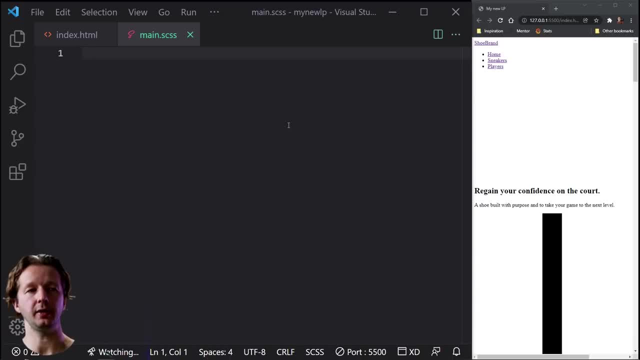 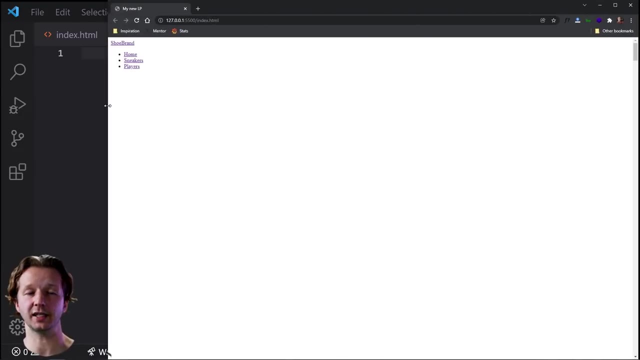 that's on a phone like this, for instance, it's stripped down there. It doesn't have to be as complex. So when we start to expand out this browser window which can help us mimic going through the browser, you're adding in more features and such, and we can do that in the media query. 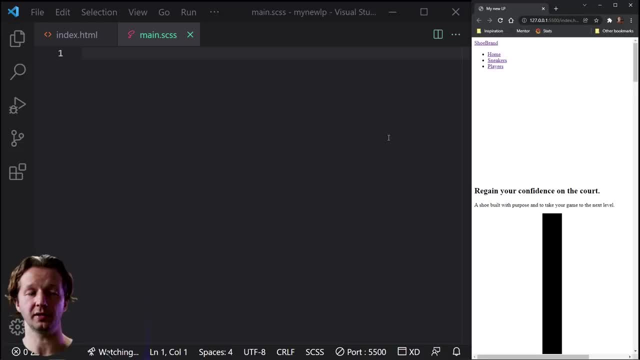 So it's just a practice that makes sense for me. Now some people still do desktop first and I'll show you what that kind of means in code going forward, But for now we're just going to try to get this thing looking good on a phone, and just taking your browser and pushing it in is one way. 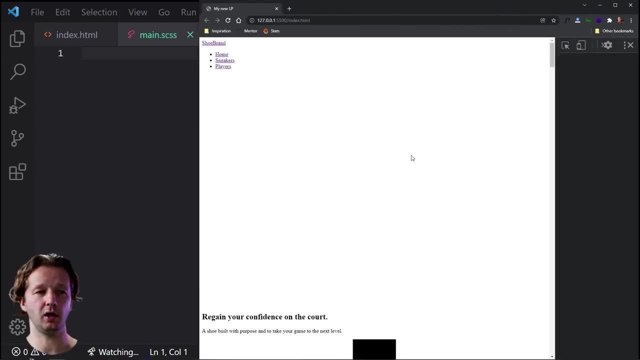 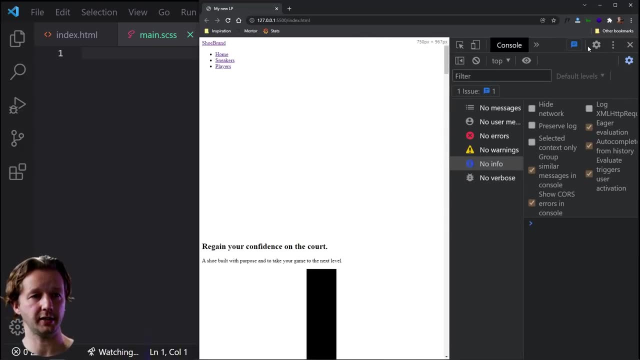 to do that. Another way to do that control shift I or F12 is we can take this right here And let's also click on this little cog. Wait, it's not the cog, I'm sorry, It's these little three dot menus. We could dock this thing wherever we want. We can also completely just detach it. 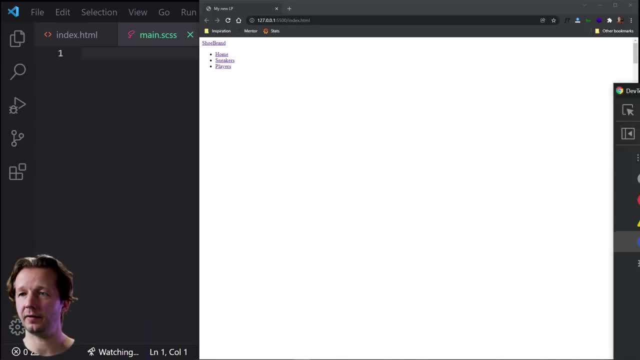 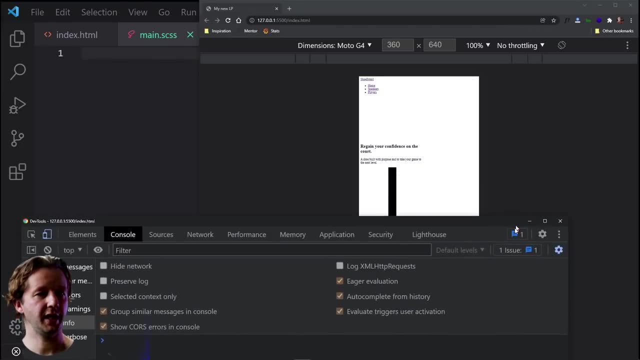 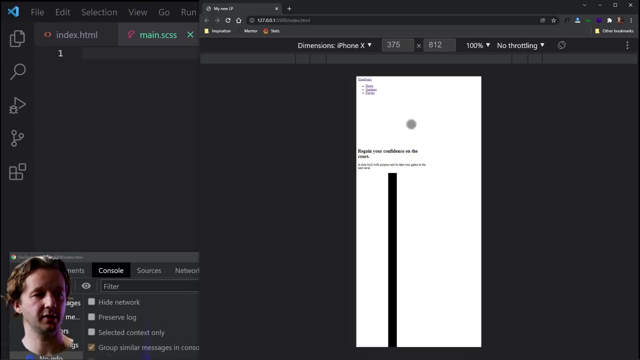 You can unlock it. So if I click that, for instance, now, I have a separate window right here. If you click this element right here, you could see now it's kind of allowing us to present it by default, like in an iPhone X, for instance. 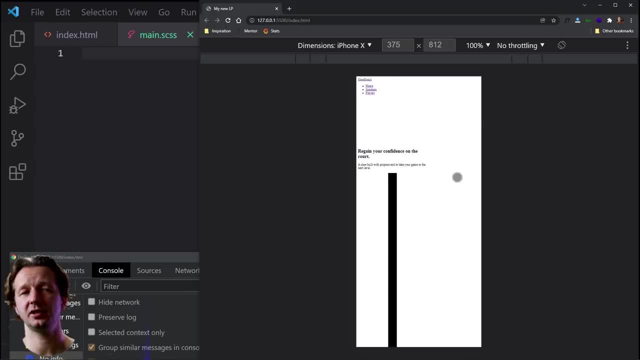 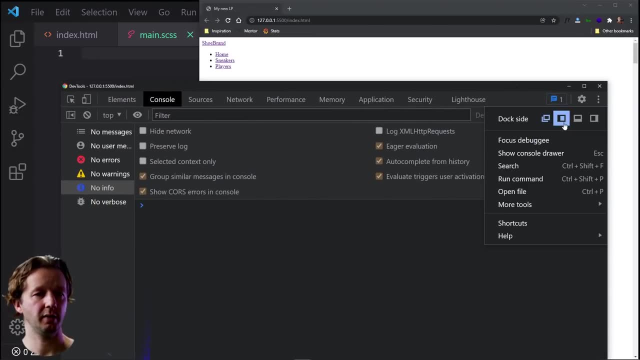 And we can kind of see what it looks like. You don't have to use this way, but it's still. it's just, it's an option. So I'm going to redock this back. So, coming over here and I'm just going. 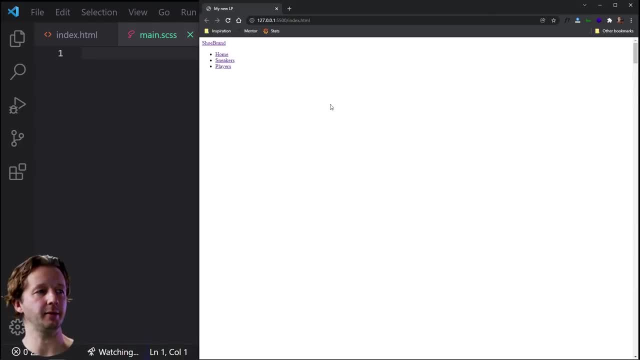 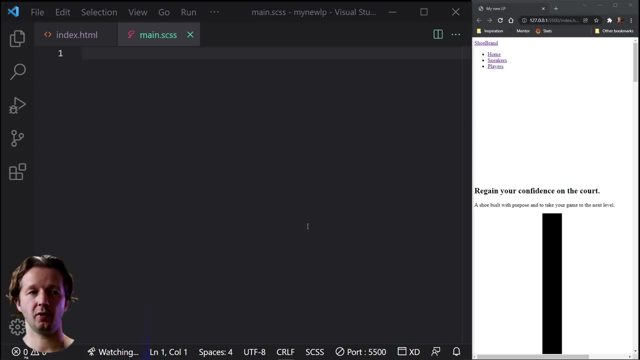 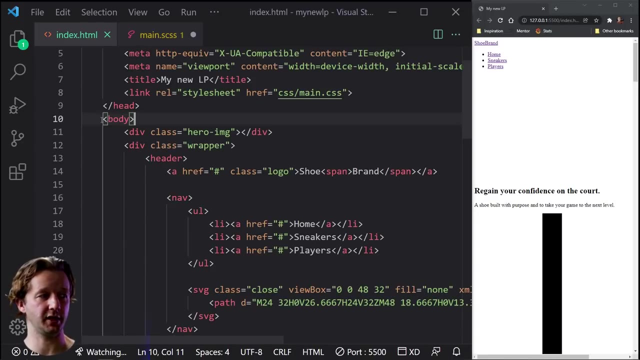 to put it. maybe I'll put it at the bottom and now I can just exit out of it. All right, So here's our mobile view, essentially. So, the first thing I typically will start off with is the body element. Now, the body element is the very first element in this. 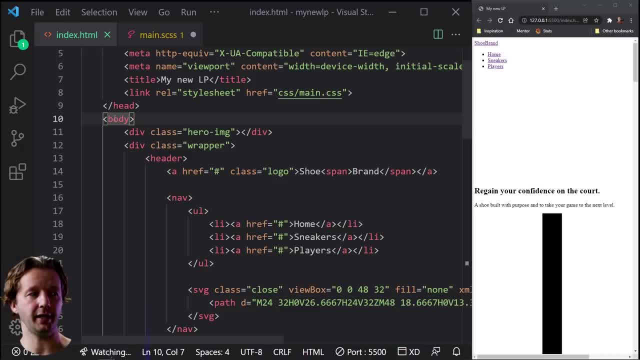 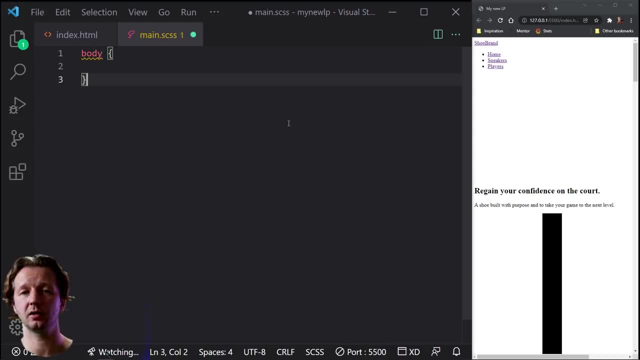 tree, so to speak. You can actually go ahead and start styling. So it's the body element. What would we want to change about the body element? right? Well, it might be a background color. It could be a lot of things. We could set in a font family, if you want to use a custom font. 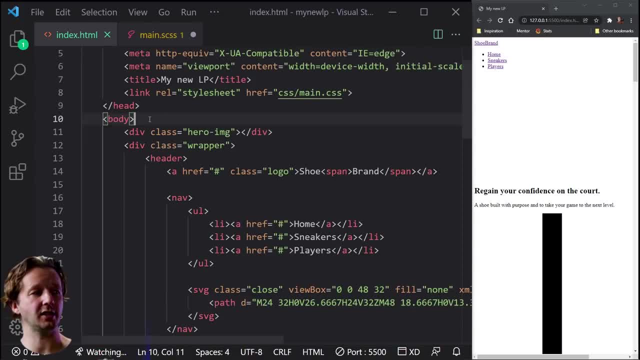 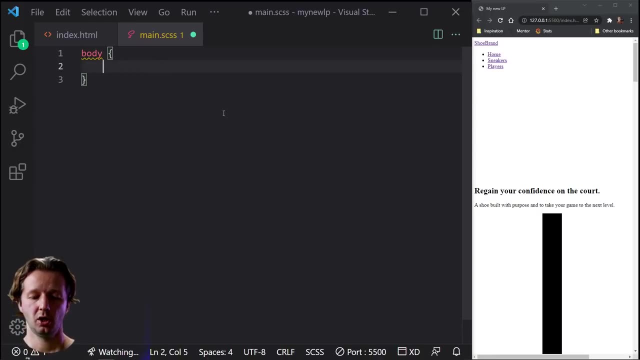 for everything Now, because, remember, if we set certain rule sets here in body, it can affect all the elements that show up within it, that are nested in it as well. So setting your font family in the body element makes a lot of sense for most cases. All right, So another thing that we'll also do is we're 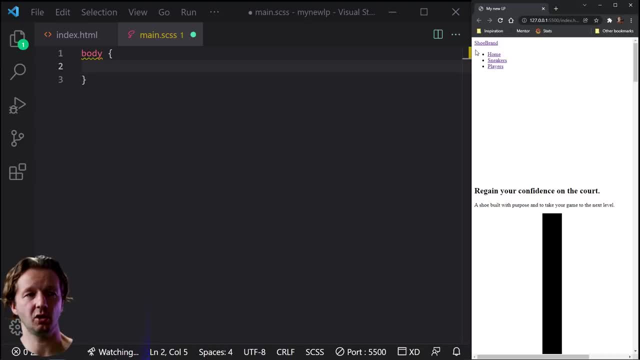 going to reset the margin, So by default, the browser will apply margins. Now your margins. you have margin and padding and that's a way to define white space. White space is just the empty areas We can see. there's a little bit of white space up here, but it's. 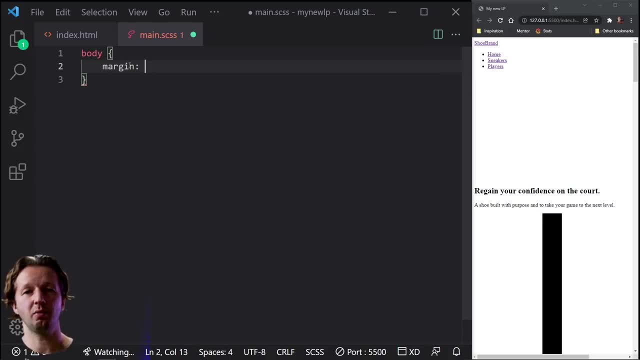 for me it's not enough, So I want to put margin. Now, that's our property, And then I'm going to put a value of 1.5 M units, Okay, And we're going to end it with a semicolon. That's how you end a declaration within a 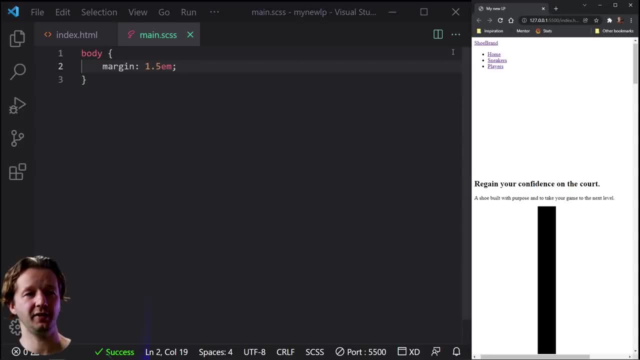 rule: set: Hit, save. Not much has changed. obviously It actually looks almost exactly the same, but if we change it to like 10 M units now, you can see that it doesn't look like there's much space here on the left. but if we scroll all the way to the top there, 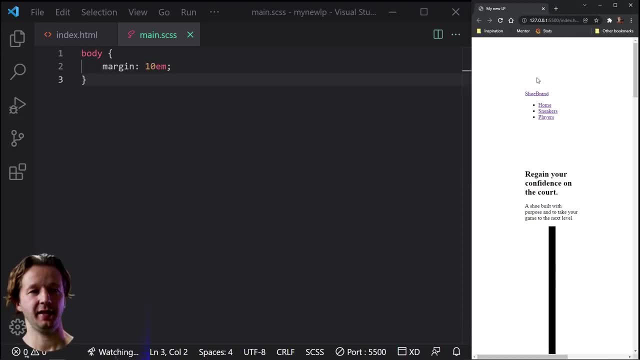 is a lot. but also there's a scroll bar at the bottom. That's 10 M units. That is a lot. So if we change this to 1.5, we can now see we have much more Compared to what was default. So if we remove this, that's all we had. That's not a lot. 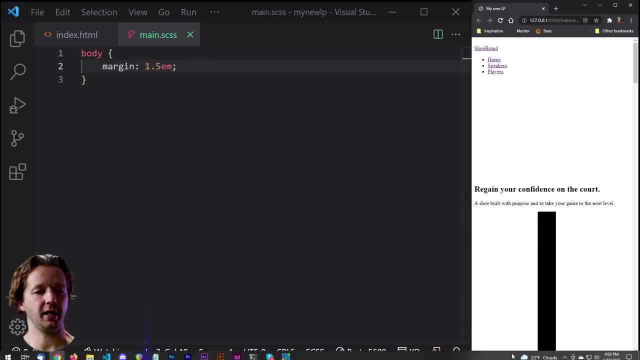 of what's called white space. So, going back here and scrolling over here, the reason is creating scroll bars sometimes is because we have issues with our images. They're not responsive yet, So but don't worry about that. So what is an M unit? You're probably. 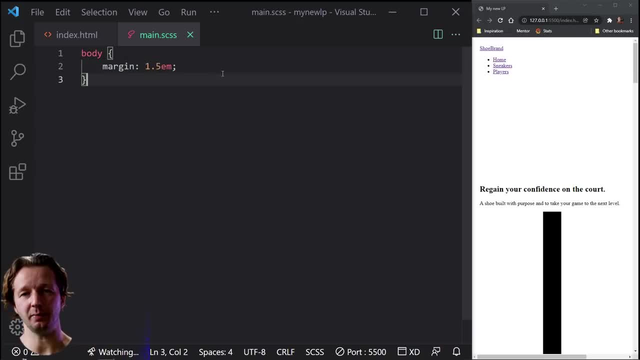 wondering what is M? Well, there are many different unit types that allow you to scale things or define widths in just lengths Units, and they fall under two categories: absolute units and also relative units. An M unit is a relative unit and I'm not going to get into a full description because I could. 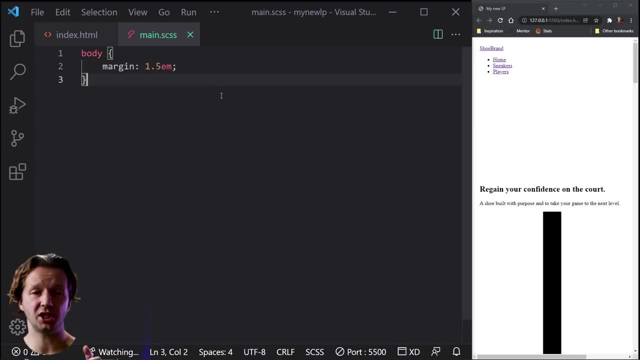 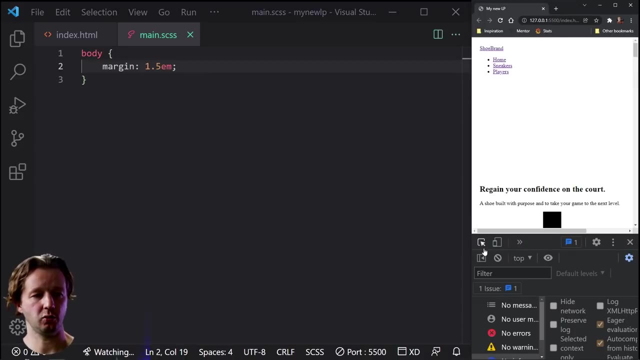 do long videos just on this topic alone. But generally speaking, when you're dealing with margin and padding, you want to use M units and the M unit is simply meaning I. if we take a look at the default font size again, if we have control shift I or F12, and we 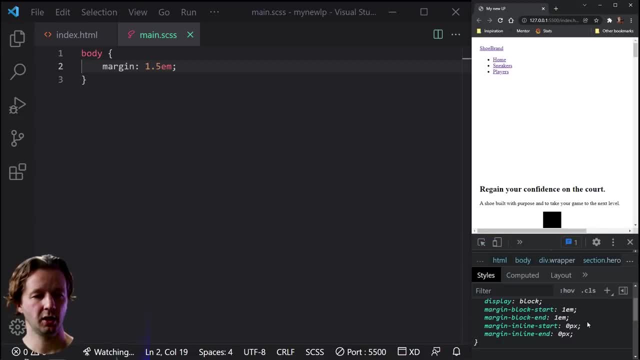 take a look at our paragraph, for instance. we could see by default, which I'm not sure if it's going to show up here, but by default browsers will apply 16 pixels or PX, which is another unit that we could use to things like type like, for it's set on the body. 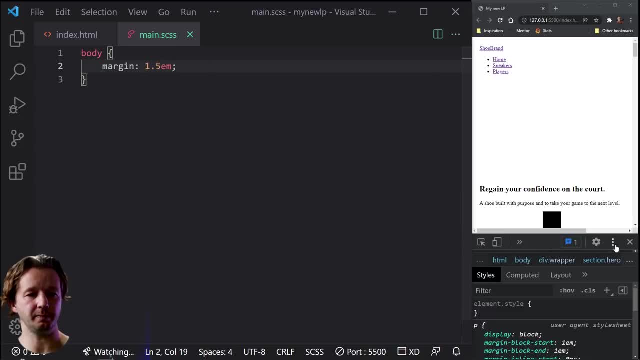 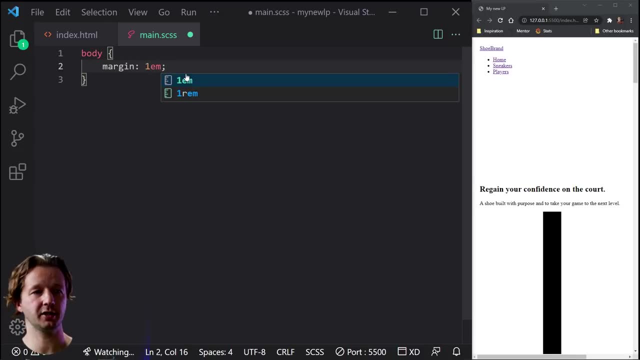 element essentially, And so our body element. if the default size is 16 pixels, one M unit is equal to 16 pixels. Speaker 1.. All right, Now, if I change it to 1.5, that means it's going to be 16 times 1.5. So hopefully. 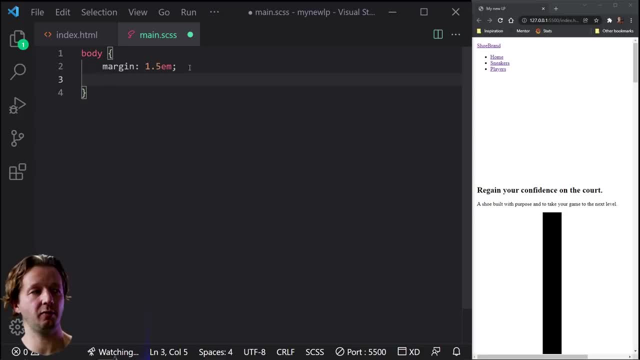 that makes sense. Now that would change if we changed font size, for instance the font size property from we overrode the default value that the browser gives it from 16 to something like 25 pixels, And then that case we could see it increases this even more. 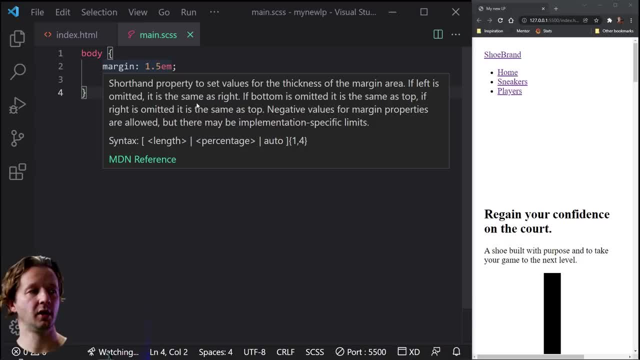 So that's a little bit of a difference. Speaker 2.. Yeah, Speaker 1.. So that's a little bit of a difference. So if we change it to 1.5, it's going to be less than 1.5. And then we can see that it's going to be less than 1.5.. So we can see that. 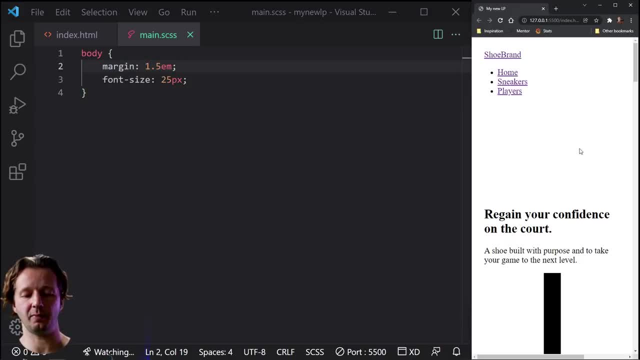 it's going to be less than 1.5.. So it's relative. The reason you want to use M units for this sort of thing is because if people want to zoom up their browser, or if they've changed their operating system so that things are larger, everything in your user interface. 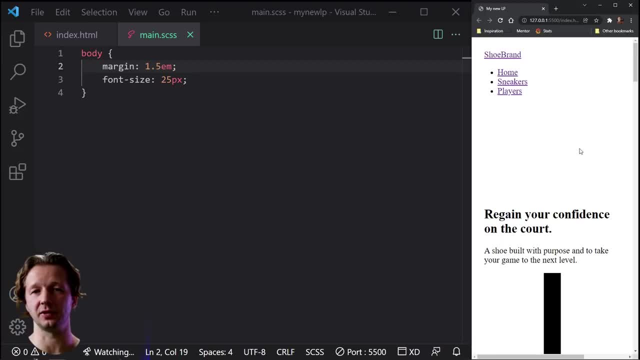 will scale well If you leave it at pixels, it won't an absolute value like PX, for instance. So that's just a quick rundown there. I know it's confusing and this is a crash course. like I said, You're taking in a lot here. I don't expect you to fully internalize all. 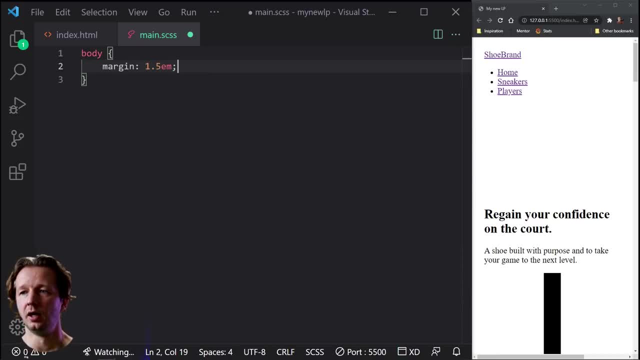 this at this point, but I'm planting seeds here, like I said. All right, So remember I'm talking about wanting to use a font. Well, if we go back to our prototype- which I think is right here- and we click here, we choose here, we can see this one's called Railway. 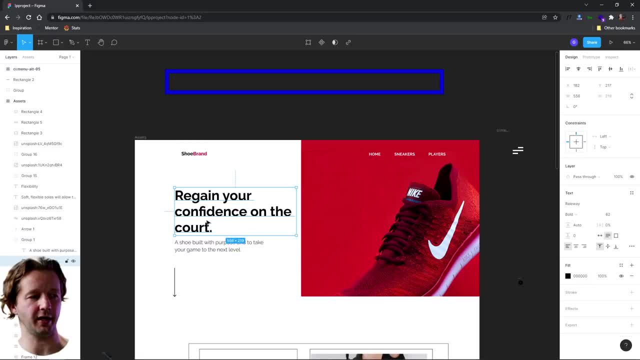 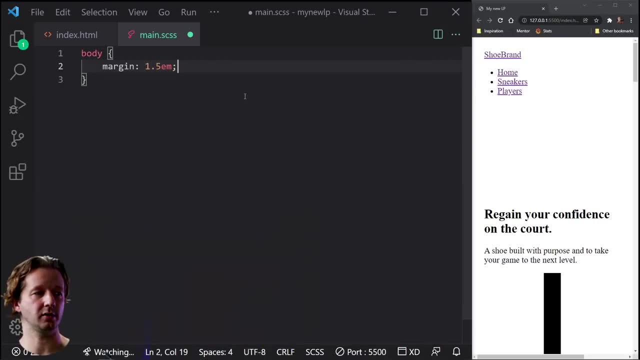 actually- Actually, I wasn't even planning on using Railway- We're going to use a different one called Poppins, which I really like. Speaker 1.. So how do you specify Speaker? 2. How do you define a font? Well, we type in font-family and then the name of it: Poppins. 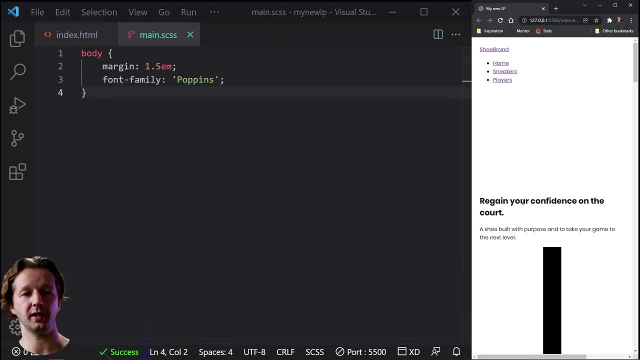 There you go. Problem with this, though, however- and it's going to work for me because I saved it, You can see. it changed the font clearly from the default Times New Roman, which is a serif font, to the sans serif font of Poppins. Now, if you don't personally have this, or 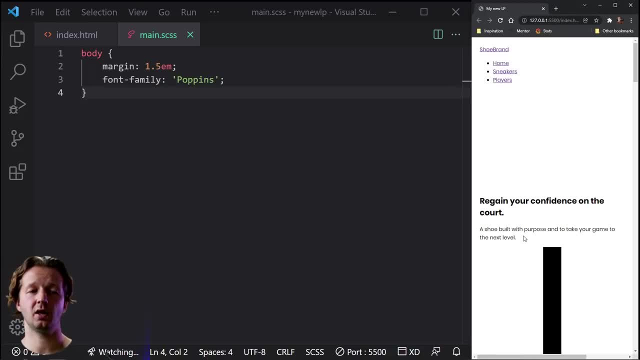 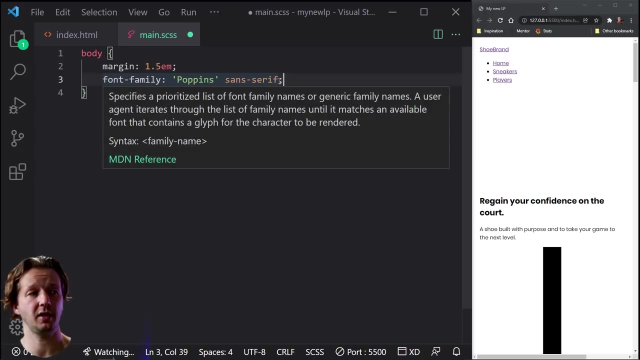 the person visiting your website doesn't have this font installed, they're not going to see it. Speaker 1. So what you can do is you can provide a fallback here in this value and just say sans-serif, So it'll choose the closest sans-serif font. Sans-serif simply means without serif, and 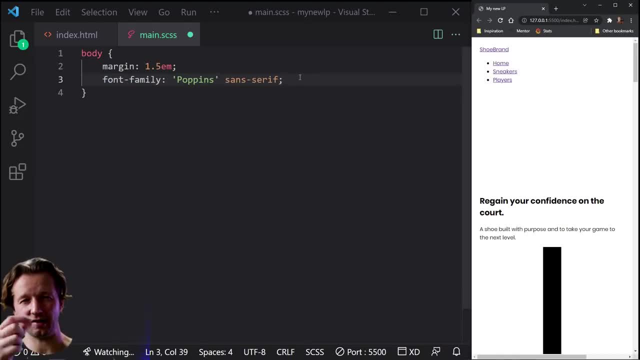 a serif is like Times New Roman. It has all those things hanging off the letters. Sans-serif is usually a cleaner font. It's much more simplistic like this. Now, the way you force them to be able to download this font is we actually import this font We're going to. 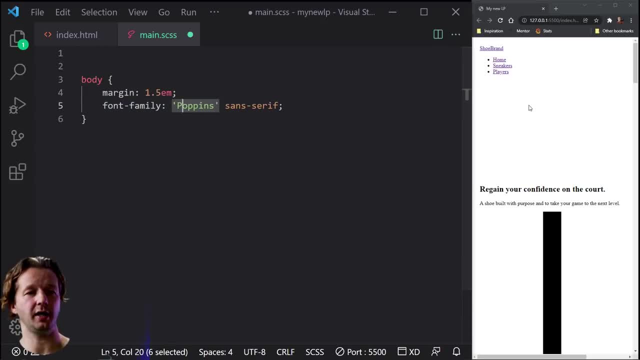 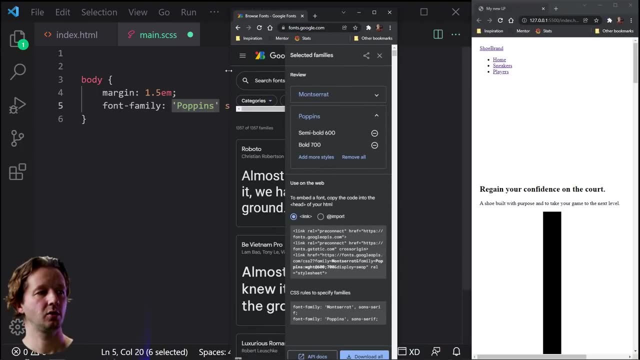 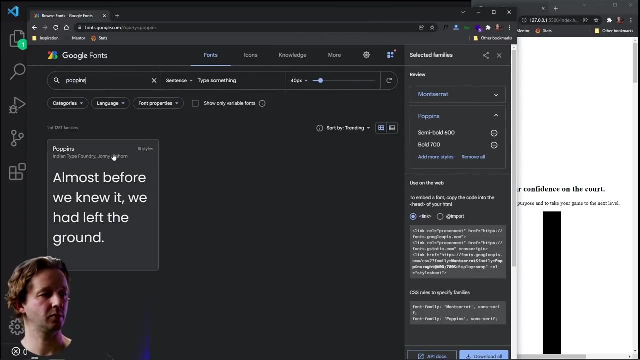 import the font. Now, this happens to be a font that's available on Google, So if we go and get our browser fontsgooglecom, this is a resource in which you have all these cool fonts that you can use. So let's type in to search for a font called Poppins We. 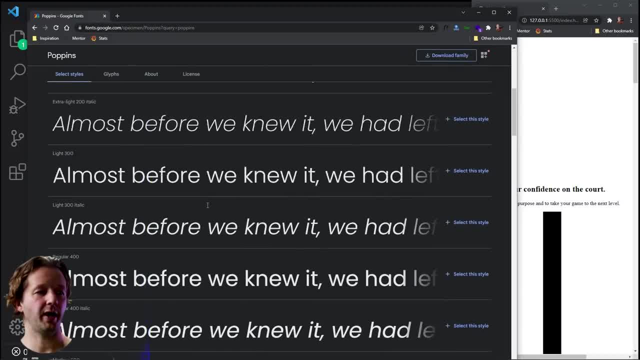 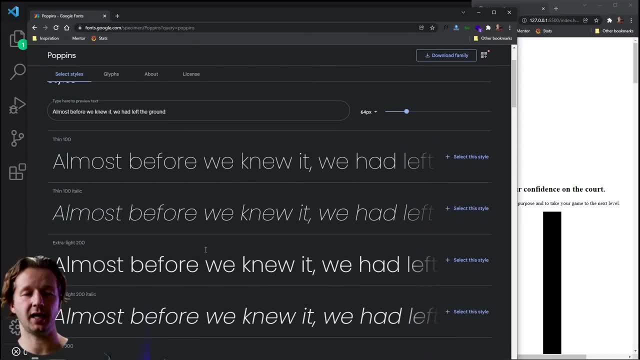 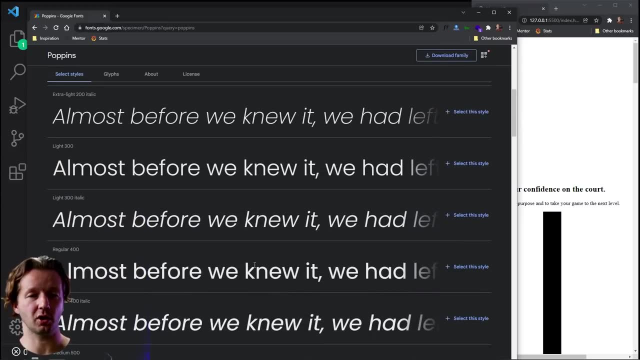 click on it and then we choose our weight. We want it really bold. Do you want all of them? No, you don't want all of them. Why? Because it takes time for these to download. So if somebody's on a phone and they have a poor connection, 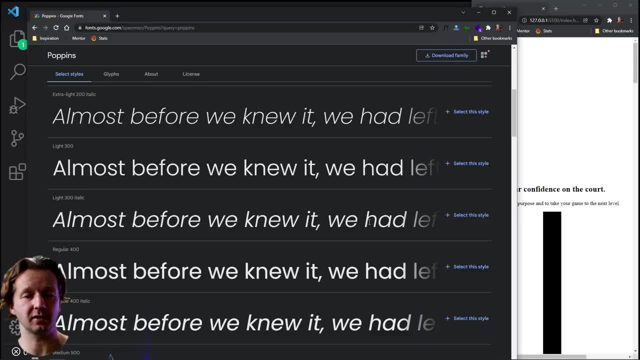 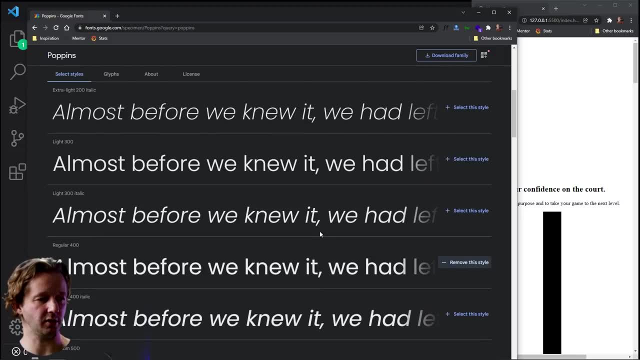 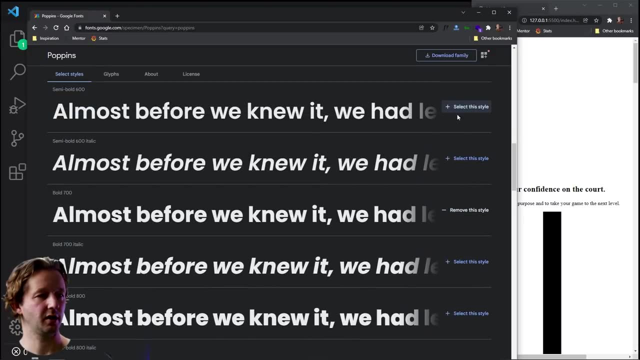 the fonts won't load right away. So you only want three max. I'm just going to choose two. So I'm going to use Lite 300.. Actually, you know what? I'm going to use regular 300, or 400 rather, And then also not 600, I want, Yeah, Yeah, I want 700.. All right, So when? 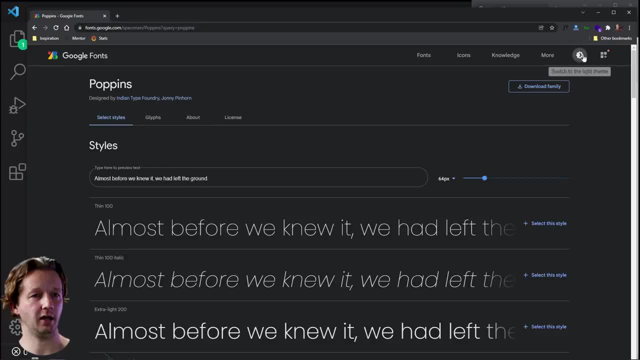 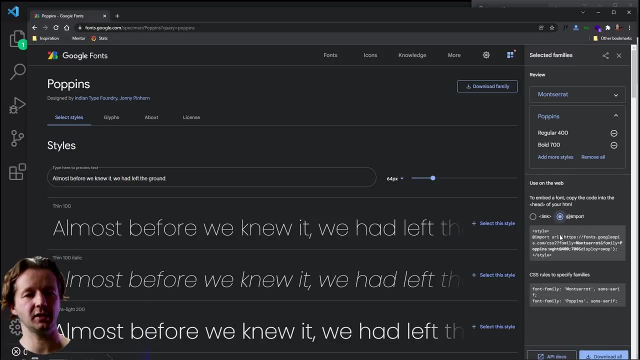 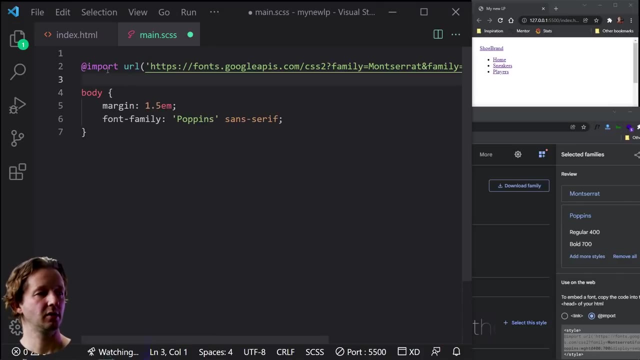 we do that. I think I clicked off of that little element right there. There we go. So we click this to get this up and we can choose to either import it. If you copy this right here, you can just simply paste it in your HTML document, But typically speaking, you 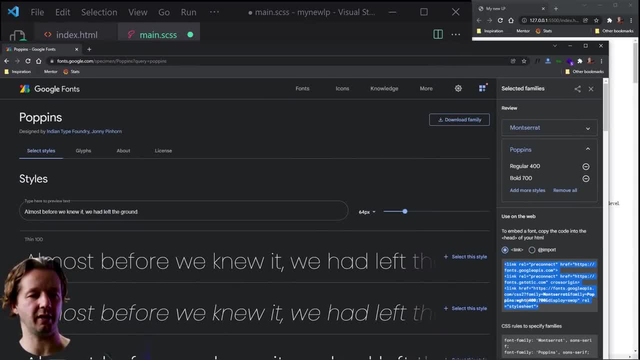 want to link it in your HTML document. So you take all this stuff, copy it, and then, above your maincsv file, you're going to have a link to your maincsv file, And then you're going to have a link to your maincsv file, And then you're going to have a link. 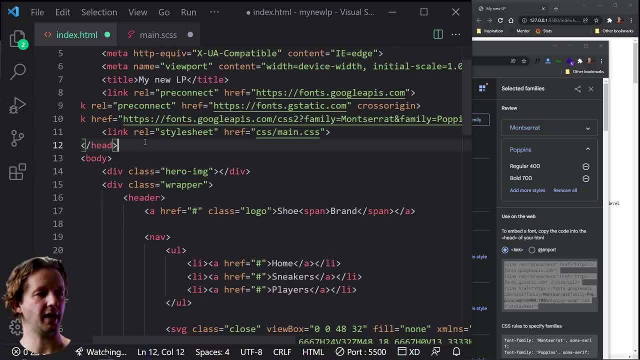 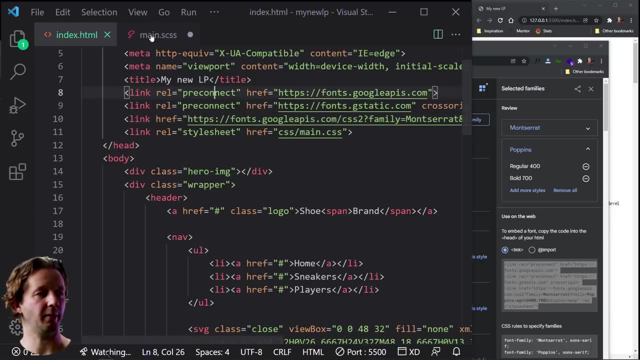 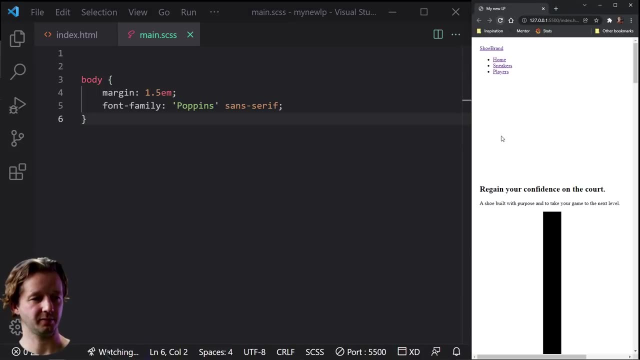 to your CSS this link element. we just paste it And then that way it's going to download automatically from your HTML element and it'll be available automatically here as well. So for me, Ooh, interesting, This is no longer working And it's showing that serif. 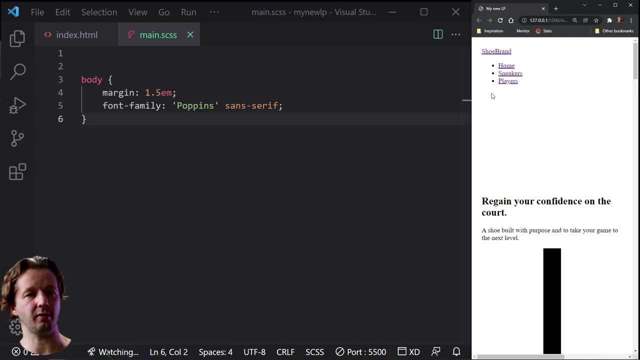 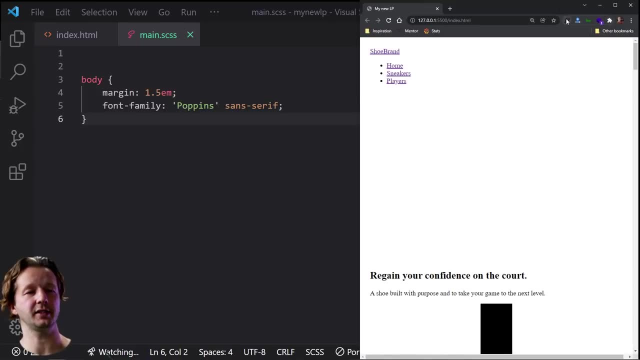 font. It's a serif font, So I have this cool browser extension. Let me extend this out, out, and unfortunately i don't. oh, there it is, it's black. that's why i can. it's called what font. so if i hover over this, times new roman, times new roman. why is this no longer working? uh, it's not loading. 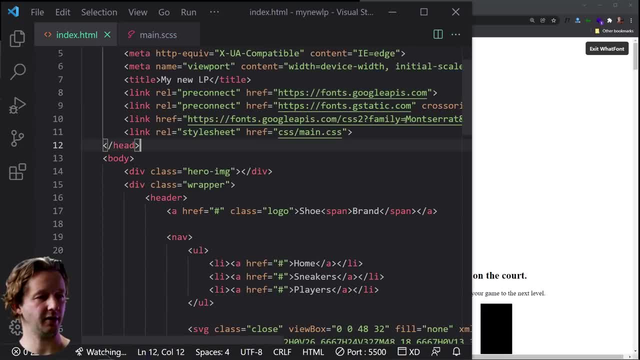 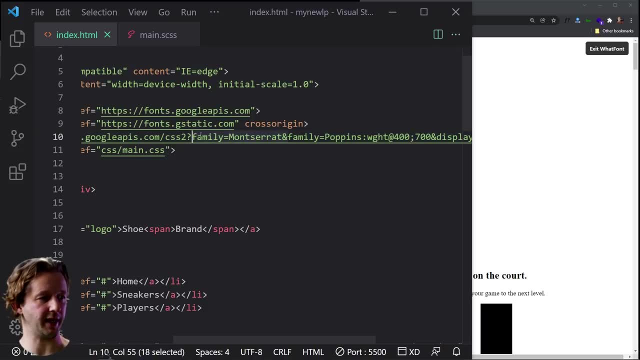 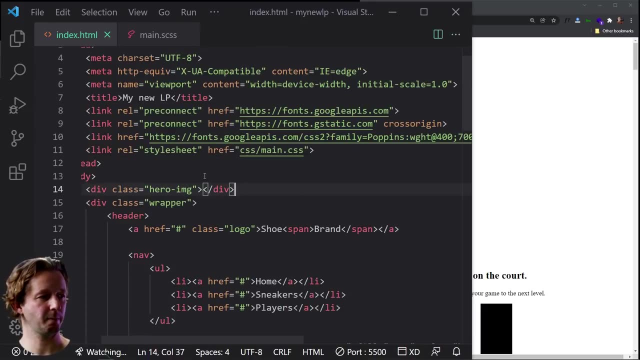 our poppins font, despite having- oh wait. it says want surat. what is that? oh, it's selecting two families. all right, let's get rid of that. family equals poppins. that probably didn't happen for you, but let's just save that anyways. all right, and it's still happening for me. so what you want? 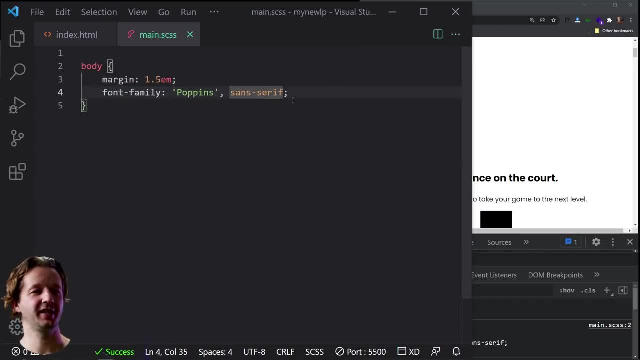 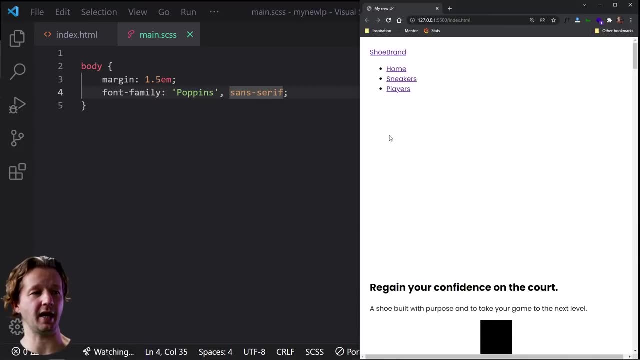 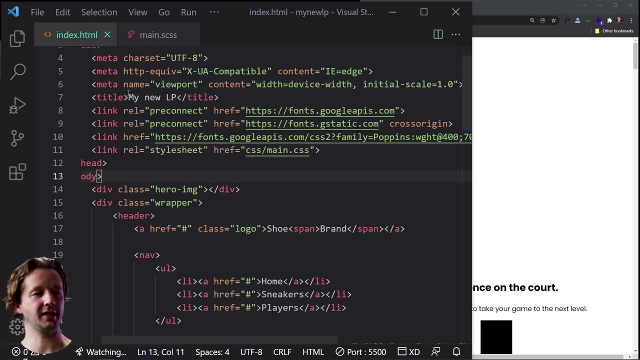 to do is put a comma right here. oopsie, i'm going to save that, and now it's coming back. so that's how you debug your html: with the help of the help of the dev inspector, all right, or the chrome tools, it depends on whatever you want to call it. okay. so we got that done and let's continue on with our 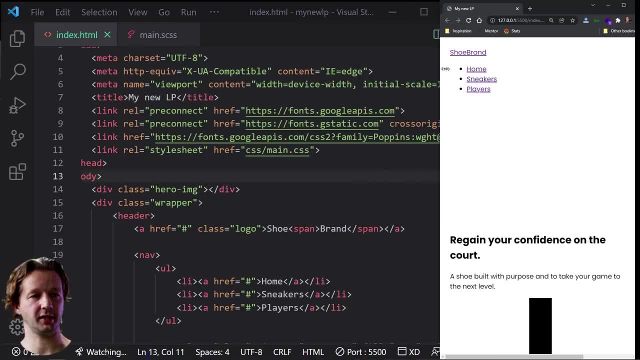 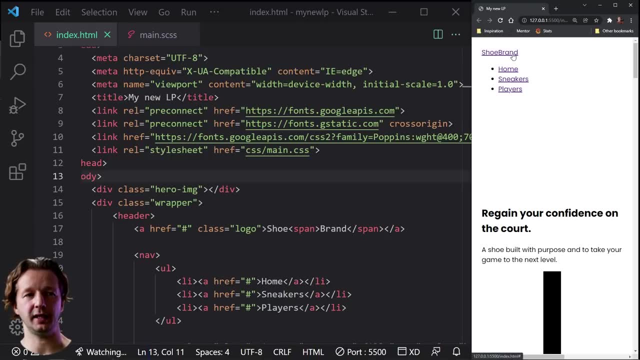 next rule set, all right. so let's drag this back in and the next thing we're going to do is we're going to get rid of the underlines. nowhere in our design, in figma, do we have links that are hyperlinks that are underlined. so how do we influence all links and remove the links from all you know existing? 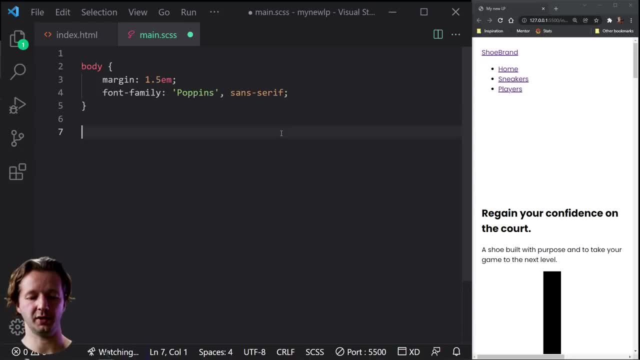 elements here on the document. well, we simply reference, we create a selector based on the tag name a, which is the name of the document, and then we create a selector based on the tag name a, which is all links. we open it up and we give it text decoration. 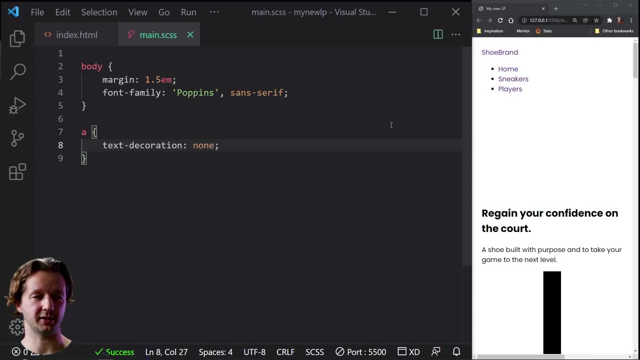 none save it, they go away. awesome, now we can also choose to style all links and make them even larger. so let's say 1.3 rem units. now, what is a rem unit? we're using m units up there, rem units over here. so, typically speaking, for font sizes, you want to use rem units or relative m units. 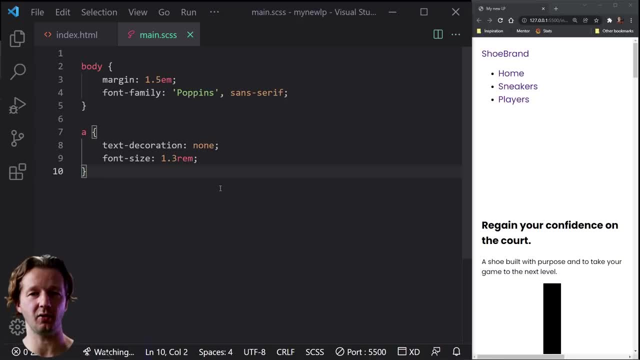 if you want to use m and okra even harder to broadcast the type of font size that you're gonna have to do. is you want to use this umbrella? that's the best way to describe this file of m. yes, and then you always have to do the same language over here. over here, you're. 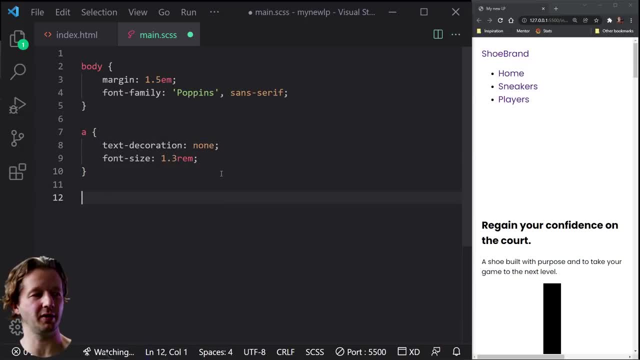 going to have to also think about the font size as a reference of any range of font. are you gonna design and edit the font size? so if you want to go ahead and edit the value side of each text size- verse M- or Google REM verse M, and you'll get a better explanation that way. But just as you 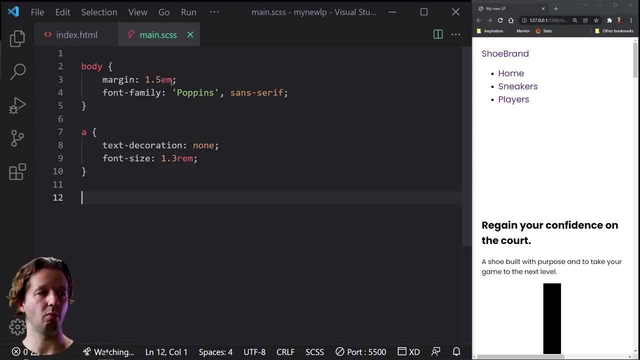 understand it. for now, font sizes use REM, margin and padding use M. All right, So next up we're going to have nav And nav. if we look to our HTML structure, we have header up here, We have. 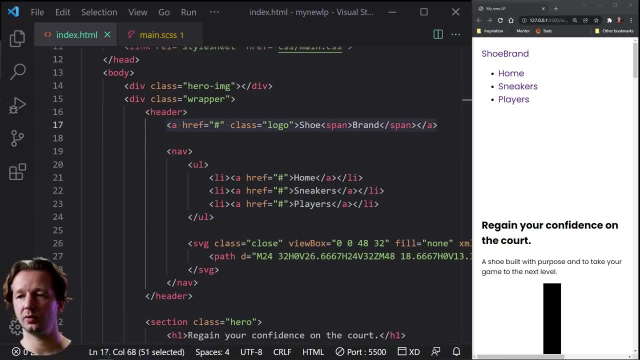 our A element, which is the logo. In fact, let's style the logo up. Let's style the logo up a little bit later until we get our image actually up, our hero image, that big red image of the shoe. So I think what we'll do is, yeah, let's do the actual image. So notice, the image is right. 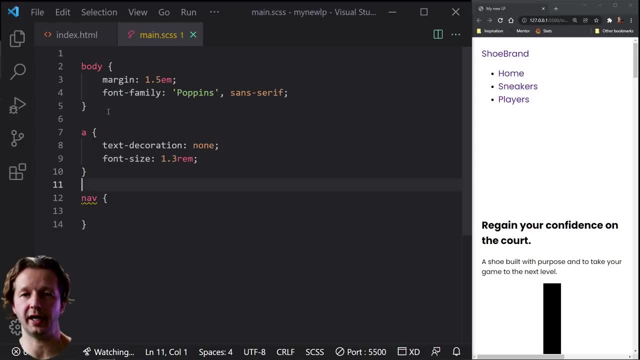 here. It's our first element. This doesn't have to be our first rule set either. So we can put these rule sets wherever we want. So we can put these rule sets wherever we want. So we can put these rule sets wherever we want in relation to each other. So let's actually get rid of nav. 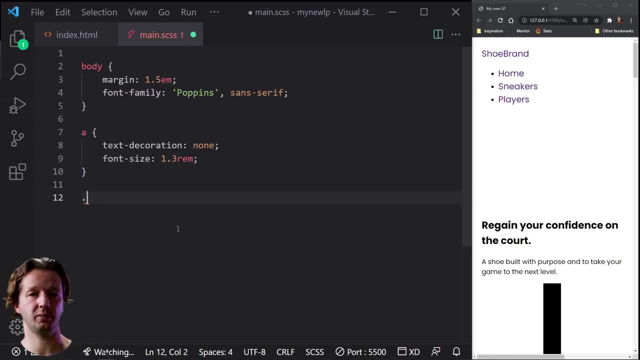 and let's work on our hero image. So we're going to put period because it's a class called hero hyphen image. All right, So this one has a lot of declarations. It's almost- it looks like it's- over 12.. So the first thing, remember I mentioned at the beginning of the video, there's a CSS. 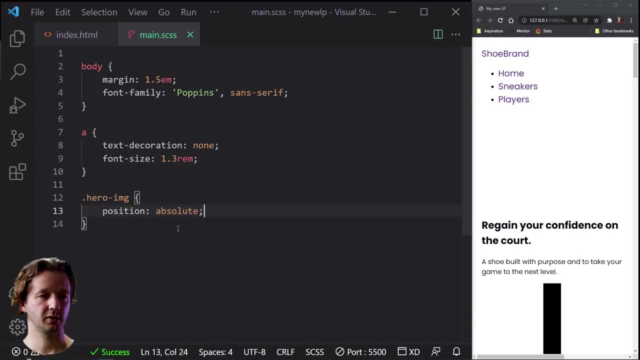 property called position, and we're going to make it absolute. So we're going to save that And we're also going to put top zero And top zero is going to be the top zero. So we're going to put top zero And top zero is going to be the top zero And top zero is going to be the top zero, And 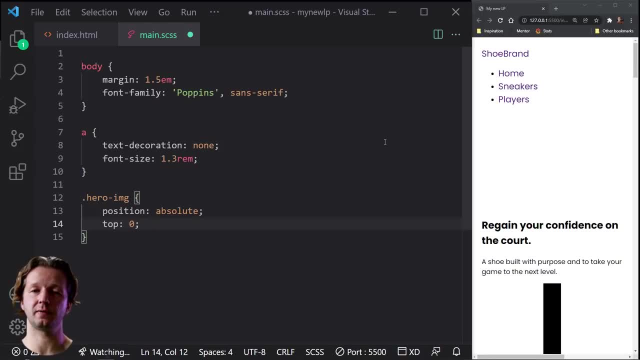 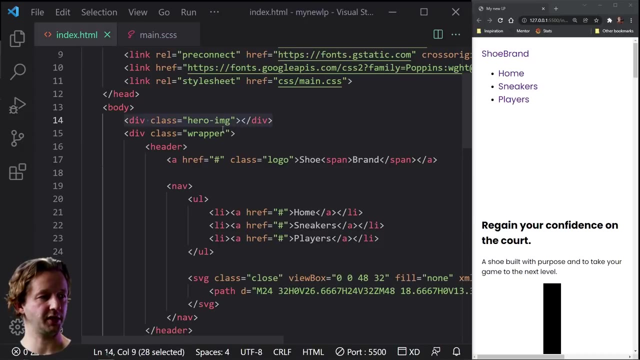 top, left, right and bottom are elements that you can use for position absolute, So you have to have position absolute in order for those to work, And it's this way for us to position it. So top zero, left zero, All right. So let's make sure we are referencing everything. So class hero. 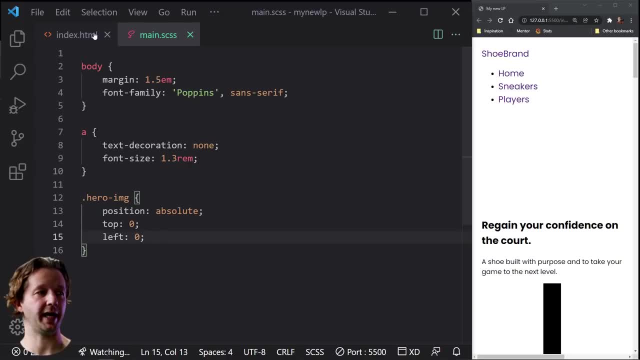 image, And the reason we don't see the image yet is because we haven't specified the background here. So let's put that in. So to create in a photograph or an image based on your CSS, we type in background URL and then we put in the location of the images. So if I hit control B, we'll see. 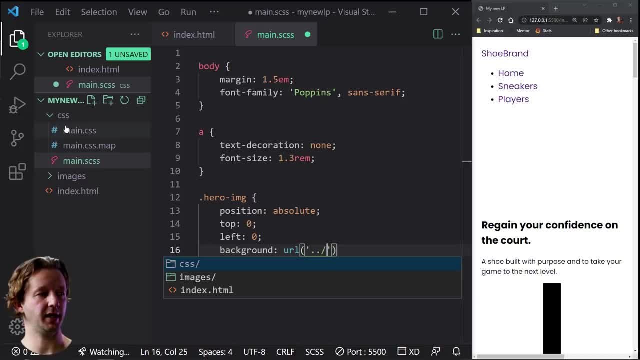 that we have our CSS folder that this file is in, but then in a different folder adjacent to it is images. So we get out of our folder by putting two periods and a forward slash. and then into what folder? Images, Forward slash, shoejpg. All right, So that image is there now, but we still don't see it. 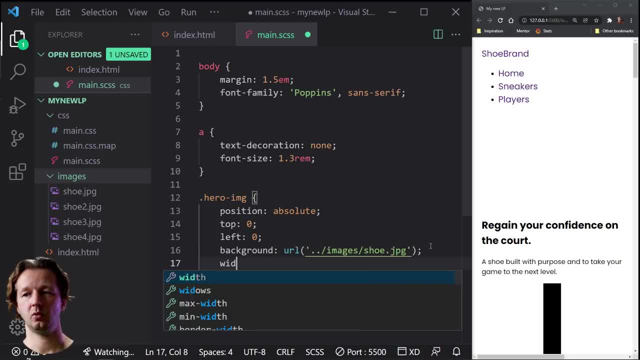 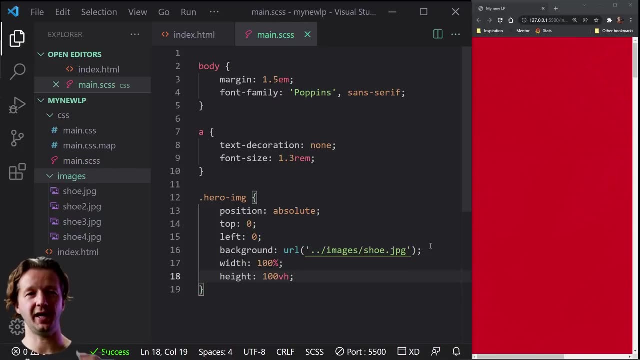 because we haven't specified a width or a height. So width, we'll just say a hundred percent of the browser. Now, height, we're going to use a new element. It's called hundred, or it's called viewport height or VH. So hundred, VH. There it is. Finally, we see part of this image which 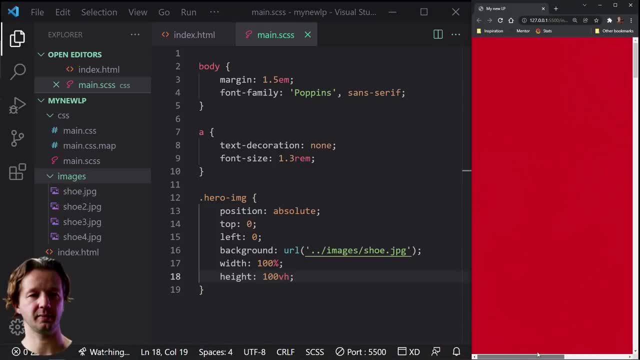 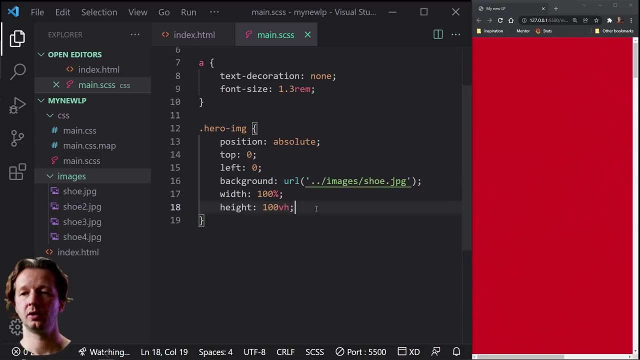 clearly is Quite large. All right, In fact, we don't even see most of it anyway, And so we still have some other elements to write. So viewport height simply means the height of what's viewable here currently in this browser. All right, Now we're also going to specify a property called Z, hyphen index or Z. 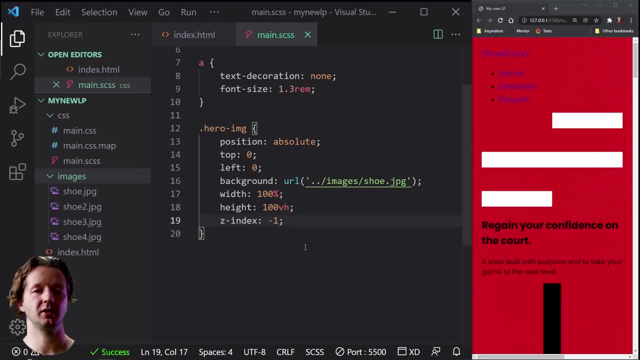 index, negative one. Now, what that does is that the Z index, based on the value you choose, which you put negatives, will make it Fall on top of or behind other elements that I may show up, And you can only use the index with. 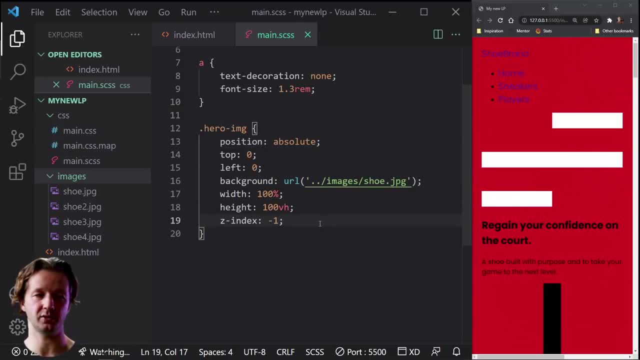 position absolute or position fixed, which you'll see we will use in a little bit. Now we can also change and add some other properties to background, So for instance, background hyphen size. we can change this to cover. Now we can actually start to see a little bit of that shoe. All right, We can. 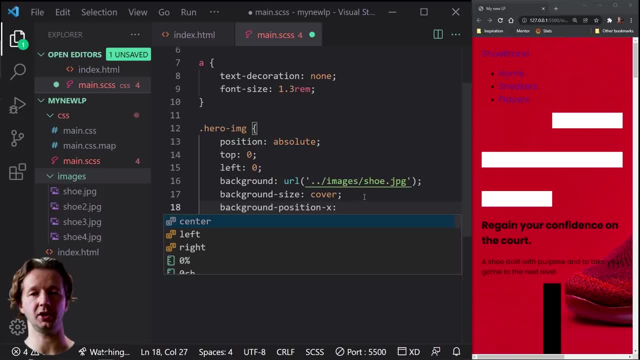 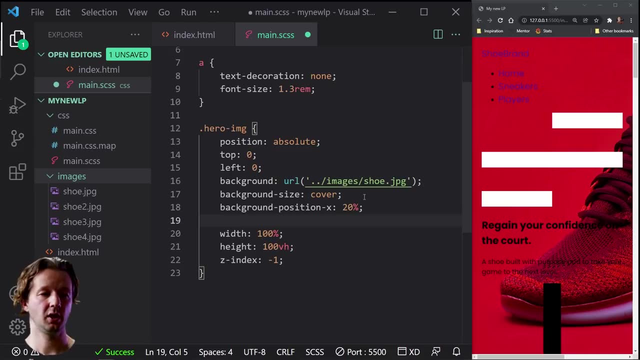 do position. hyphen X, for instance, which is left and right at 20%, So we can kind of move around what's viewable. Now we can see more of that shoe. We can replicate this as well: Shift, alt and down. 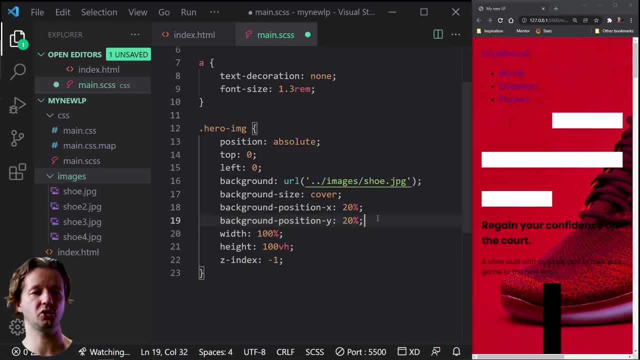 and we can do position Y Now for a lot of these values. you can have shorthand values as well, In fact background right here, if we can start to add some of these same values and just put cover here instead of explicitly stating it here. So know that you do have those. 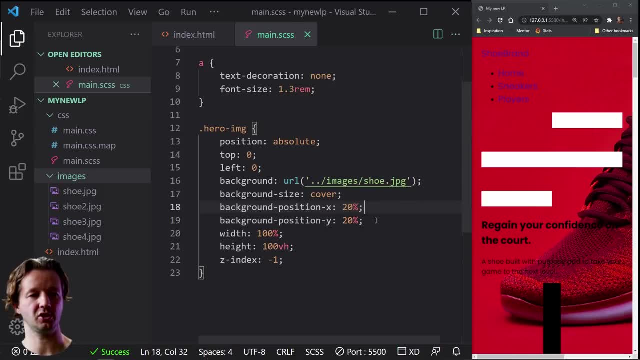 options. So Y, we'll put 20 as well, for instance, just to move it down a little bit. We can also specify, and I'm not sure if this is going to affect anything- overflow hidden. All right, So I had. 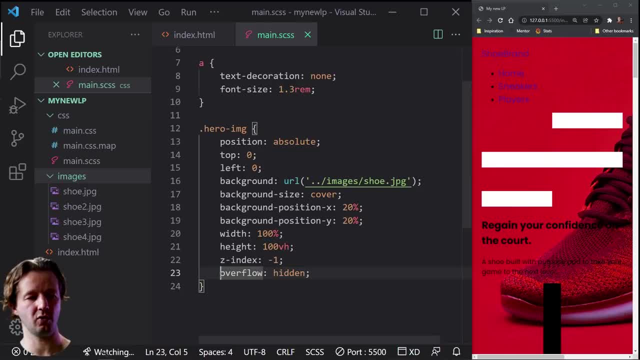 overflow hidden in my reference code. We may actually end up needing that, but for now I'm just going to comment that out. So to comment a property out so that it doesn't actually work. yet it's still there for your own reference point. put two forward slashes. 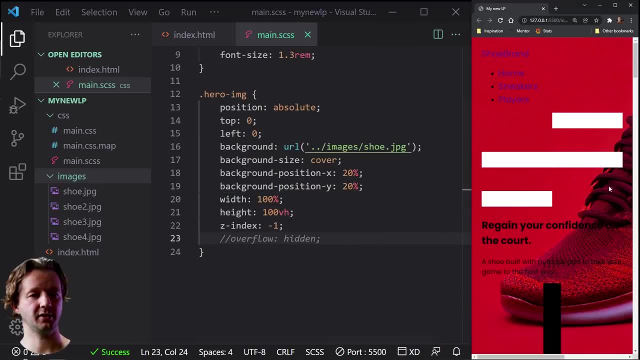 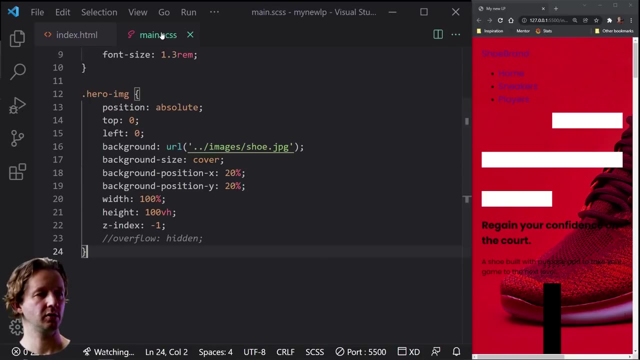 All right, So that's good for now, And now let's get back focused on this navigation up here. So let's take a look at our logo, And that logo hit control B is right here. It has a class of logo, So we want to reference just that. So we put the class logo And inside of there, 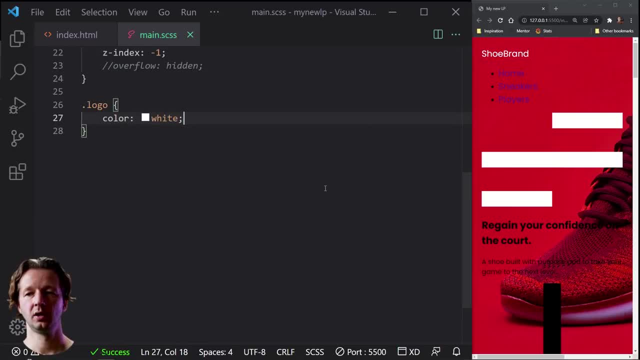 we're going to put color white. That's the way you change a font color. Font weight: bold: We'll use that bolder. the 700 value of that font that we imported. All right, So that's looking good there. Next up, looking at our situation: here we have our header element, So what do we? 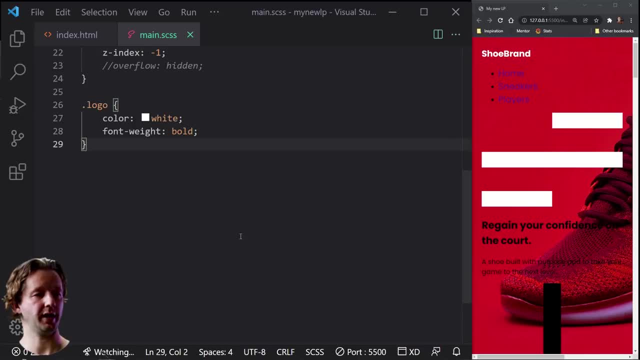 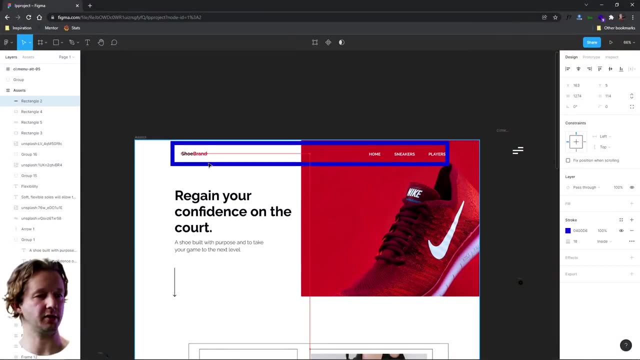 need to do with the actual header element, All right. So if we look back to our design, this whole thing is the header element, this invisible blue square which we don't see, obviously, in HTML. But we have two elements, We have two columns, rather, 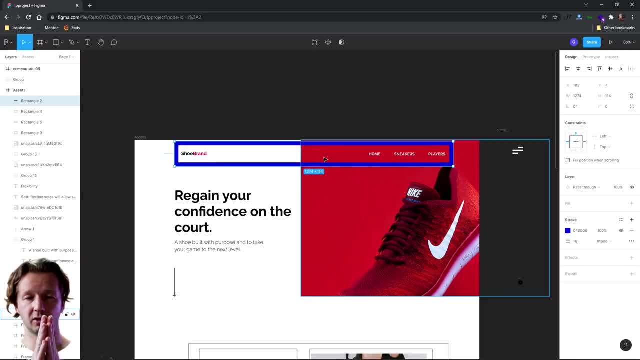 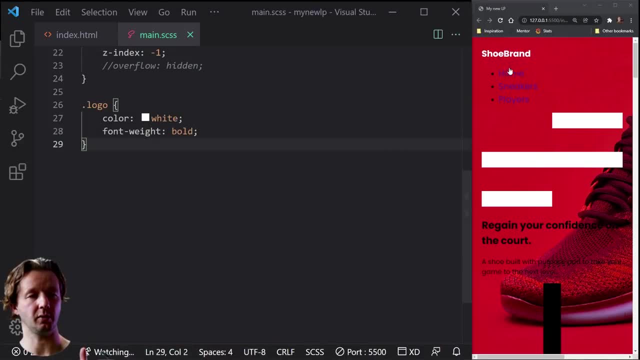 this and the nav element. We had to make it so that those are not underneath each other, like they currently are in the browser, but side by side. We don't want rows, We want columns for these two elements. So the way we do that is we say header and we say display flex. 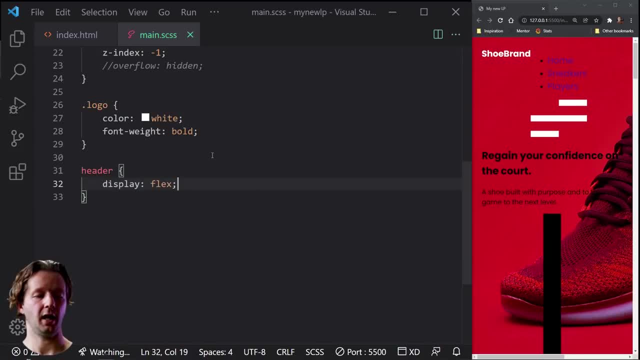 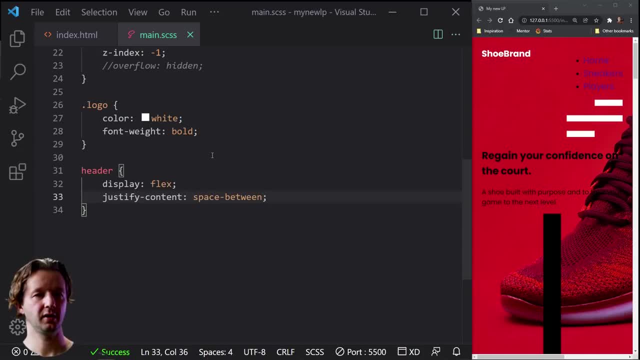 going to do that, We're going to do that. So now we have a way to do this too. So we say: content space between now, that pushes it out All right, So we're getting somewhere. So display flex is a way to structure your layout. There's also one, a value called grid, which we- oops. 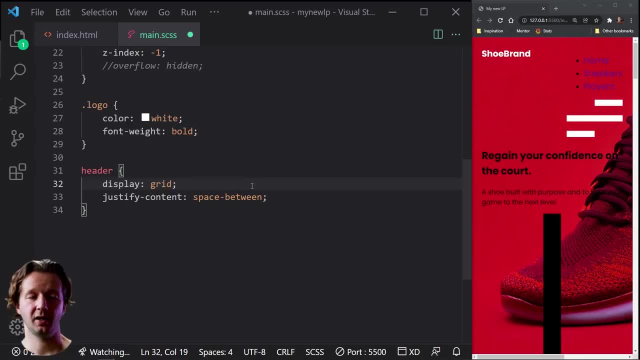 not gird grid, which we will also use Now they're. they each have advantages, but the grid is pretty, pretty powerful. But for just quick, simple things like this, put two columns. I like to use the grid or the flex rather. 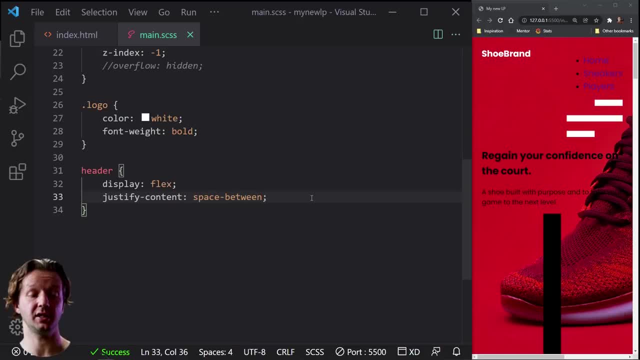 Flexbox, as it's called. If you want to learn more about both of those things, there's entire courses on them. So again, Crash Course. this is All right. so that's pretty good, right there. And now what we want to do is, by default, we don't want this, right here. 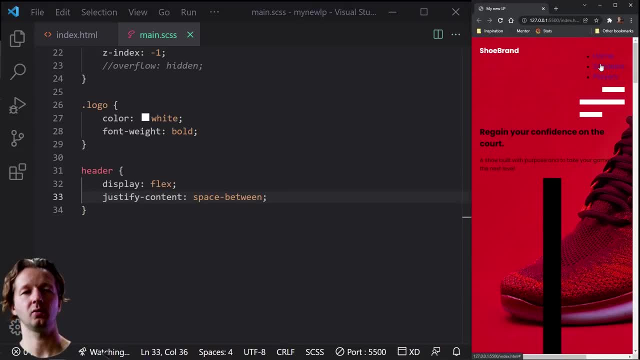 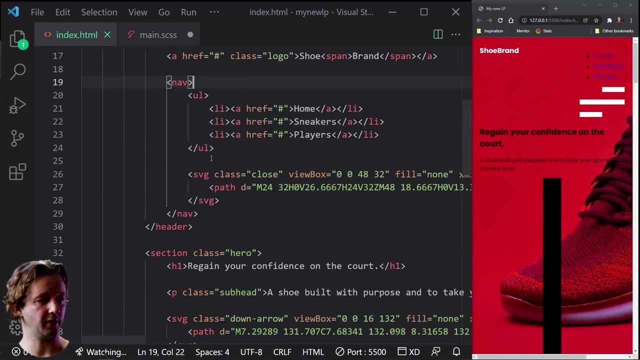 Let me reset this browser zoom. We don't want that right there. We want just this little hamburger menu. We need to hide this element right here. So how would we do that? Well, let's go in and let's specify, and let's first reference this: Where is this at? Okay, these are both inside. 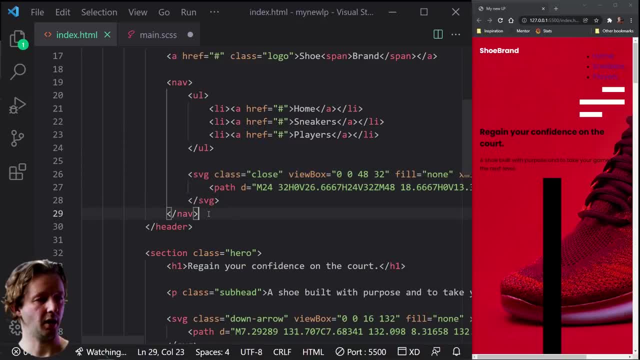 here We have a close button. Oh, I don't think I actually. let me see. here I want to make sure I structure my HTML correctly, because maybe I actually didn't- Yeah, I didn't Okay. and so actually, what we want to do is take this menu element and we want it outside of nav, My 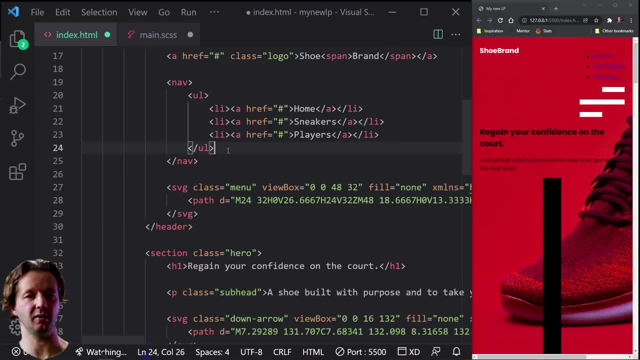 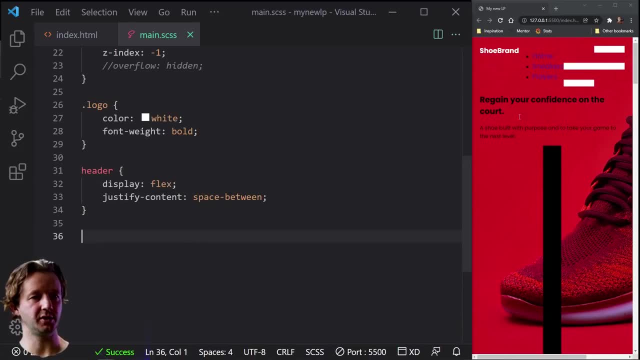 bad. We're going to have the close SVG element a little bit later, inside of the actual nav, but for now we're just going to leave it like this. Okay, so now these are all stack three, because we have three elements that are in here- One, two and three- and it's created. 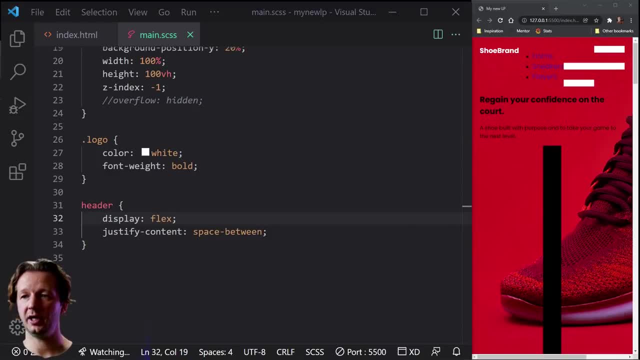 the display. flex has created three elements, essentially. Now we need to hide this navigation in a second, but for now, let's, let's, let's go ahead and get this style up, because it's way too large, clearly, so to do that. we're going to take in, uh, and take a look. 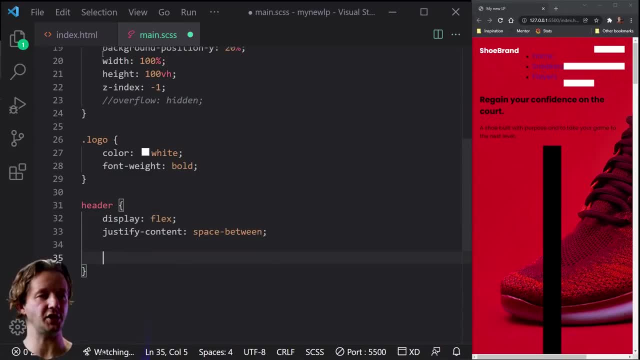 at the elements we need to. there we go. yeah, it's going to be svg. so if we look at our header right here, we have a single svg inside of here. all right, so what we'll do is we'll say: svg. now. this is where we're nesting for the first time, i believe yep, which is the feature of sas. so this means uh. 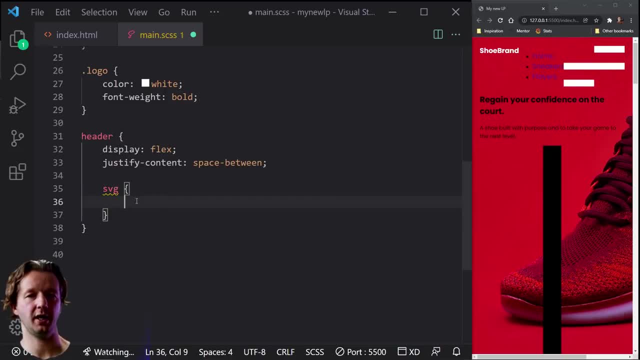 any svg elements inside of header this- this right here- this rule set will only apply to them. if there was an svg outside a header, like down here somewhere, this rule set that we're about to create would not apply to it. so we're going to say: with 3m units, save that and that's a good size, right. 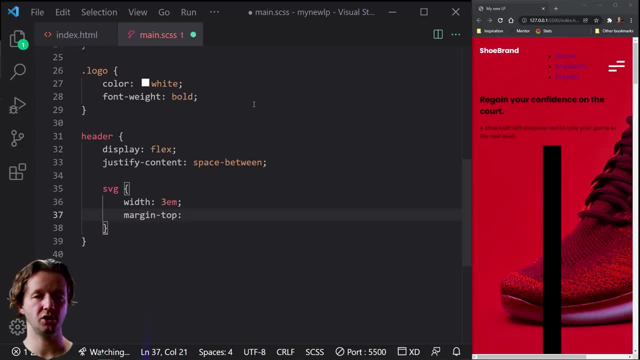 there margin top. so margin you can. there's a shorthand for margin, so you can do margin alone and just say you know, and specify the four different values if you want. so top right, bottom left, like a clock. or you could say margin top, we'll say negative 0.6 m units, so you can actually. 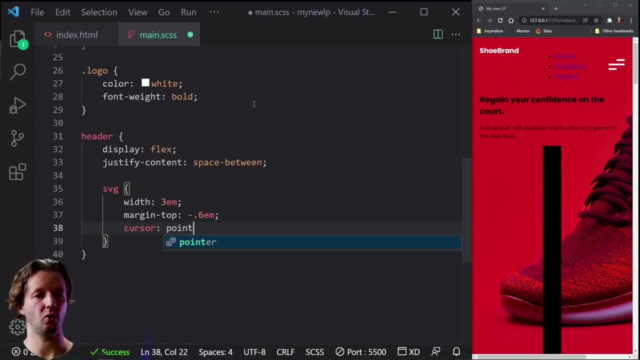 do negative values and we could do cursor pointer here. now that doesn't look like it's right location, right, that's because of this element and we need to try to hide that. so what we're going to do is we're going to choose, maybe just above here, we're going to put in nav. now we could just do display none. 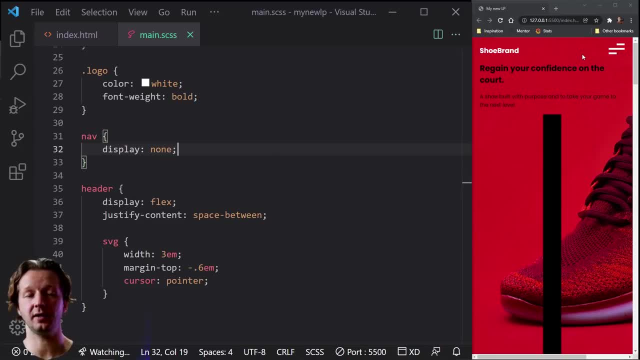 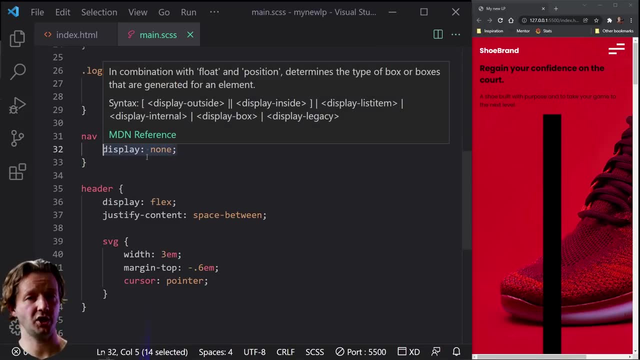 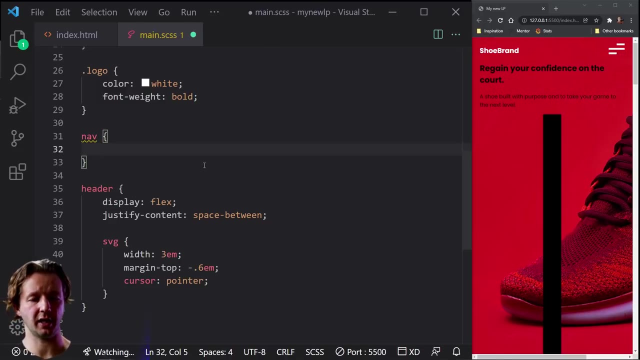 and that you know almost this pretty much. that gets rid of it, right? uh, and that's what we want, and we could do that. but there's another way to hide this situation here, um, and the way to do that is we can use the transform property and kind. 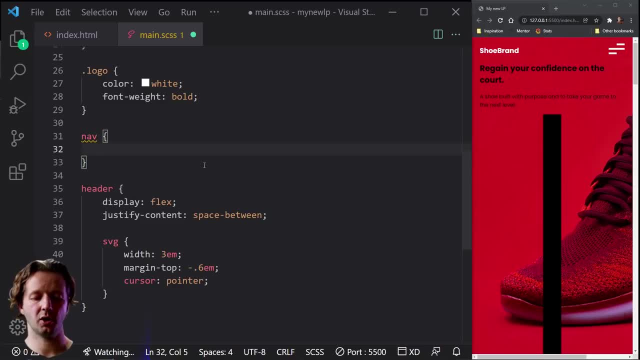 of just push it off the side of the page. for now, we're going to leave this at display. none though i- and you'll see why in a little bit- but we want to get things structured up just um a bit more here. i. i want to at least finish this portion, all right, so? 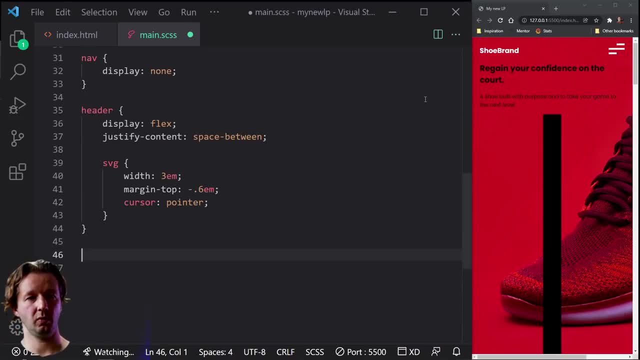 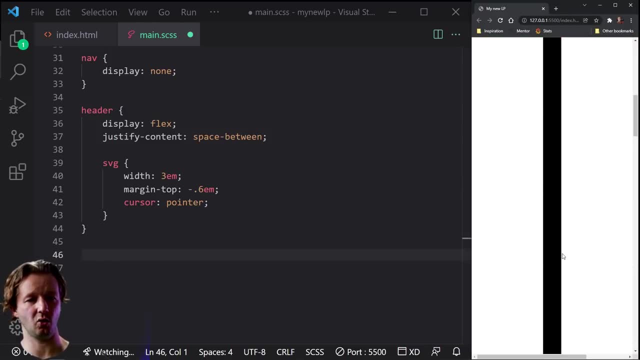 then we'll work on that navigation. all right, so if we want to get this all structured up- because clearly this is way too close to the logo, i think it needs to be larger and this big old thing that needs fixed as well- so what we'll do is reference here. so we have. 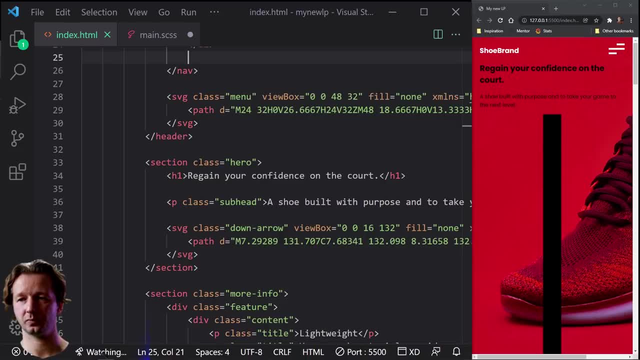 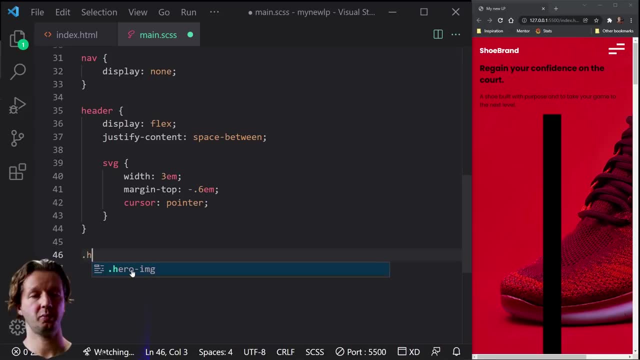 a i, a section called hero and let's reference this section alone. so what we do is we could put hero or we could do section dot hero, which means i, it's in real, it's. it's also specifying the html element and the hero element in there, and i like to do that just as a reference point. 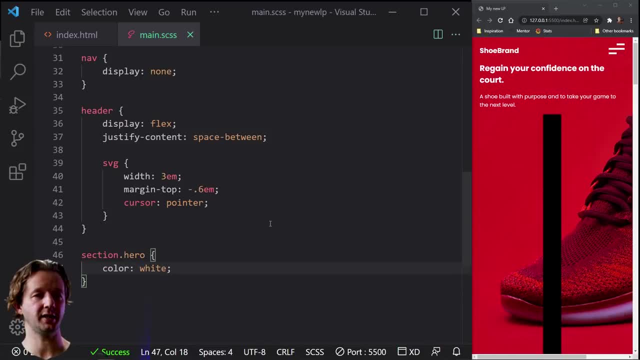 sometimes it gives it more context. essentially so color white. that means any type elements inside of that element is going to be white. we can do also- i let's do, let's do- a height here of 90 viewport height, and this will become important when it comes to scaling this svg element and positioning. 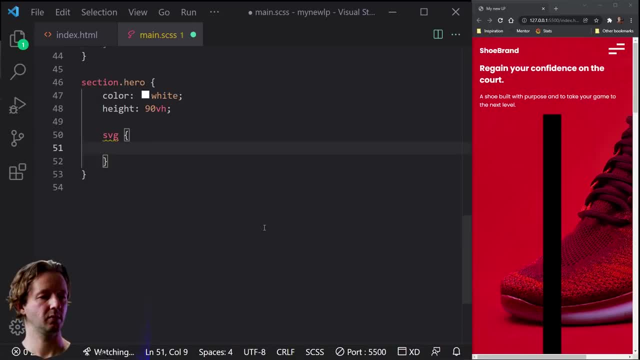 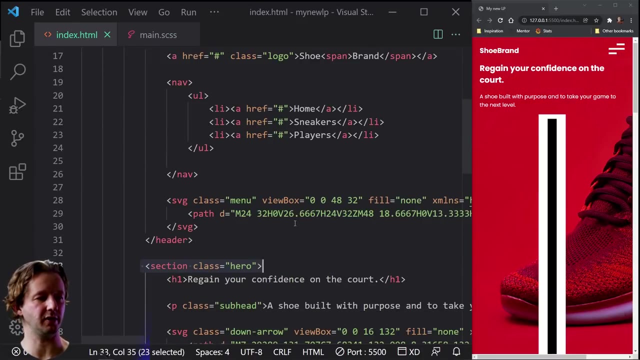 it. so let's take that svg element inside of there and let's make the stroke white, and then we could also make the fill white as well. or is it fill, let's see here? because, svg, you have to specify the background a little bit differently. so if we look at our down arrow, right, 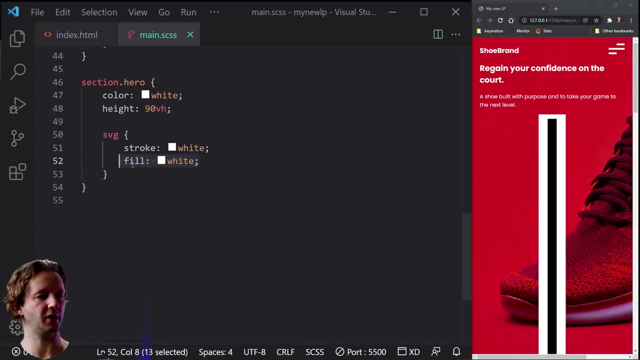 here. ah, that's because the way we change the fill here it's specified in the path attribute. so path fill white, there we go all right. so we've done that and also we did give it a class of down arrow. so technically, what we could do is we could say: 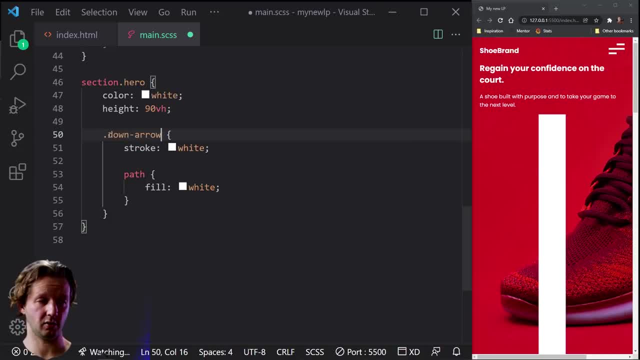 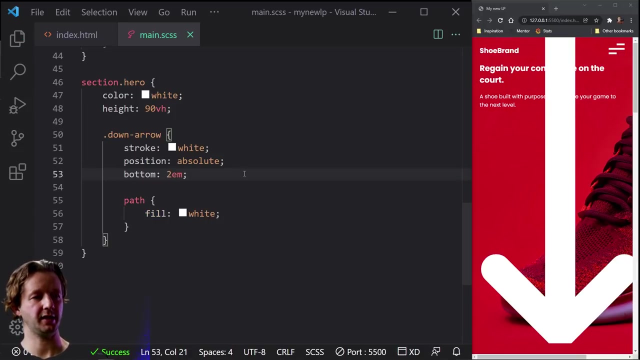 right here: changes from svg to down hyphen arrow. notice: if i save it, it works just the same and we can also size it a little bit or adjust the width. so what we could say is we could say position absolute and also bottom 2em, and we need to get this scale down big time. 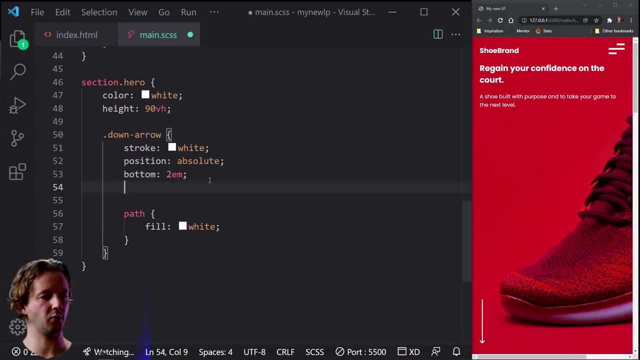 so to do that, what we'll do is just put in a width right here and we'll just put one m unit, and there it is way much smaller, all right, and i think that's pretty good right there. so now next up, let's also focus on this element, this type element. 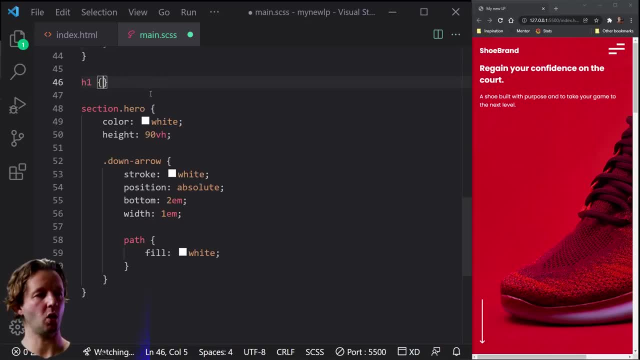 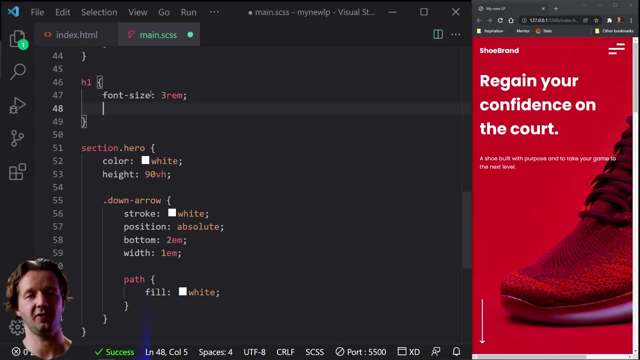 so we're going to put in h1 and we're going to say font size: 3 rem units, which would be 3 times 16, which i'm not sure what it is off the top of my head. i'm terrible. um, we're also going: 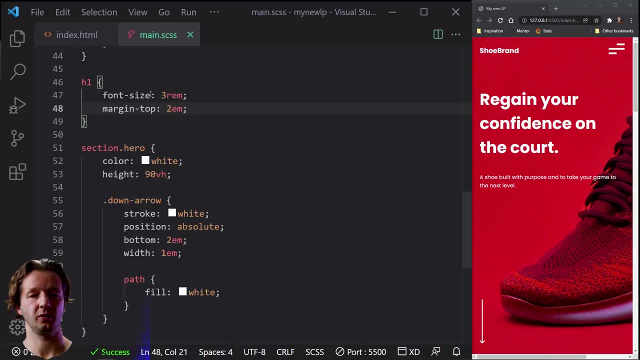 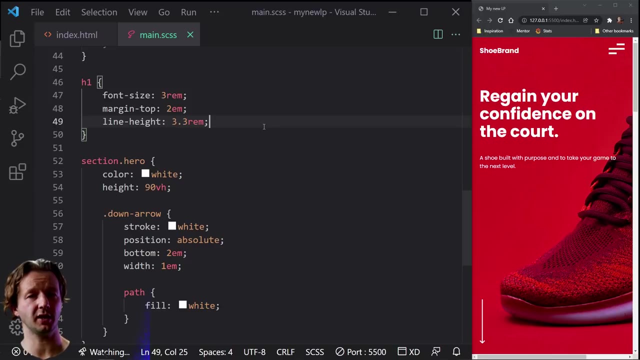 to do margin top 2m units really push it down. and then also we can adjust the leading or the line height. with the line height property we'll say 3.3 rem units. now you may be wondering: how do i know all these values offhand? Well, sometimes you can refer back to your Figma document. 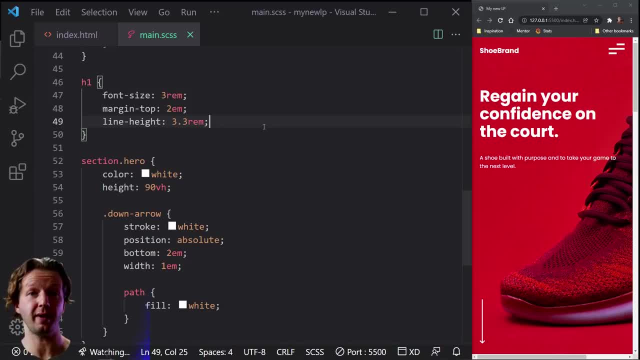 and then click on it and then it'll kind of give you the pixel values and you can do some math to convert it to MRM, or you can just eyeball it. Sometimes it's all about eyeballing things and just adjusting these values as is. So I already prepared this document before. 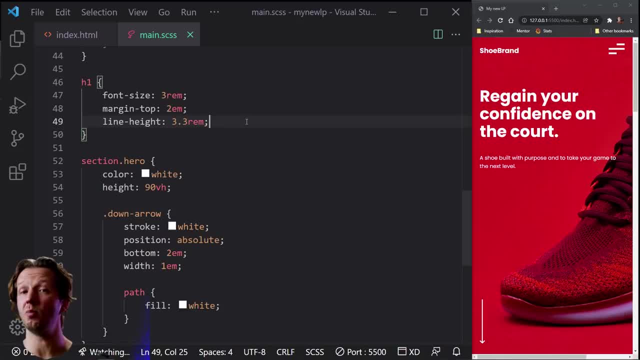 I have a reference code on a reference monitor. It makes the tutorial go much smoother than rather you sitting here watching me fumble around and adjusting values. Sometimes people get mad to like: why are you not doing that? So that's the answer: because it's not clean. 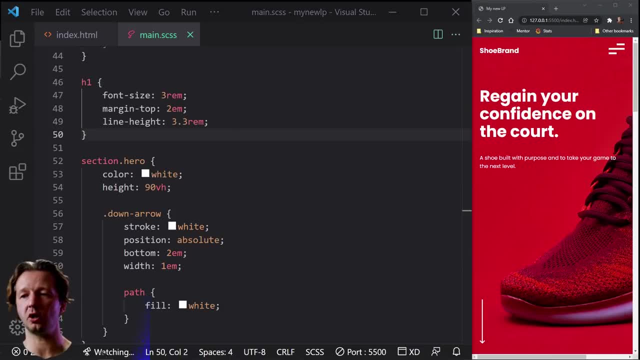 watching me. It's already difficult doing this as is. Now. let's also reference our subhead, which is, right here, a subhead class, because that needs to be a little bit larger. So subhead will be font size: 1.4 rem units, And I think that's looking pretty good right there All. 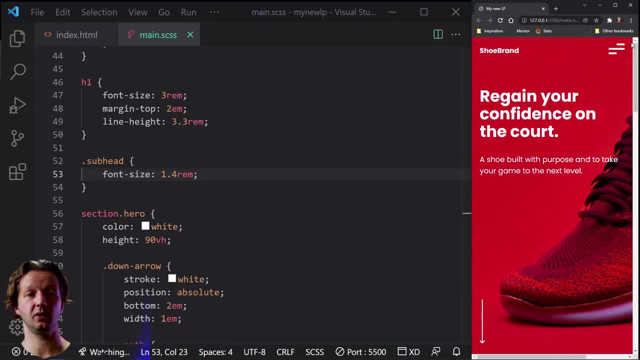 right. So right now, all this doesn't look good, but this looks a lot better than what we had before, clearly, Okay, Okay. So now let's get this menu up, And when we click on this, a menu is supposed to show. 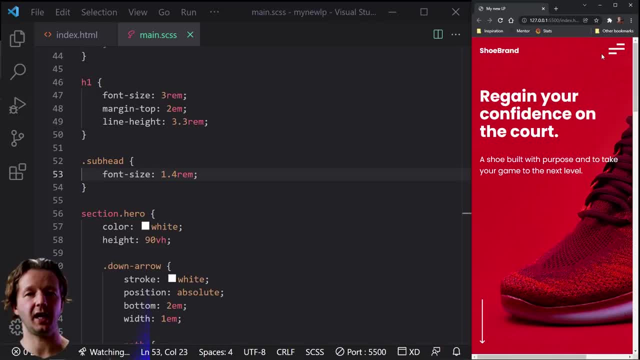 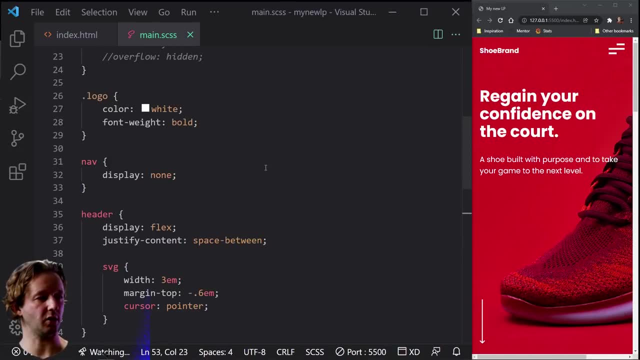 up. What does that menu look like? So we need to style that menu right now, And that menu is defined within our nav element. So that's why we're going to go back to our nav element and take off display none. Now let's just pretend somebody clicked on this element and 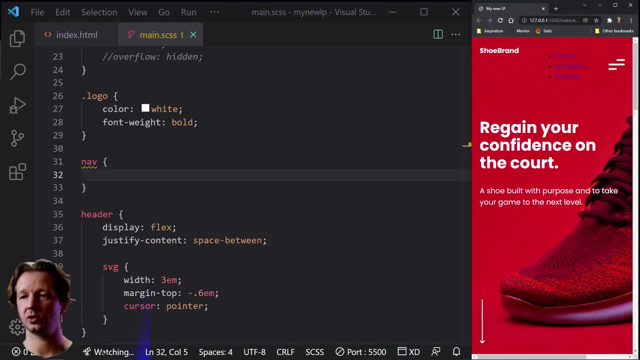 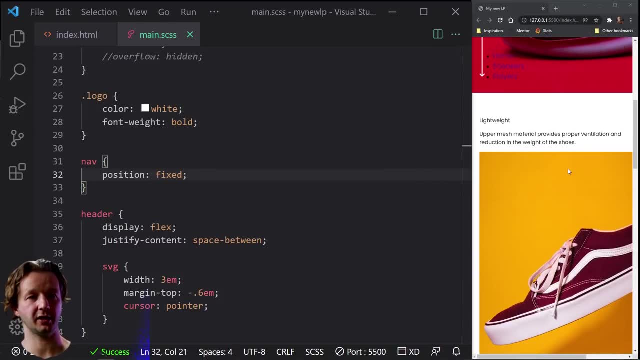 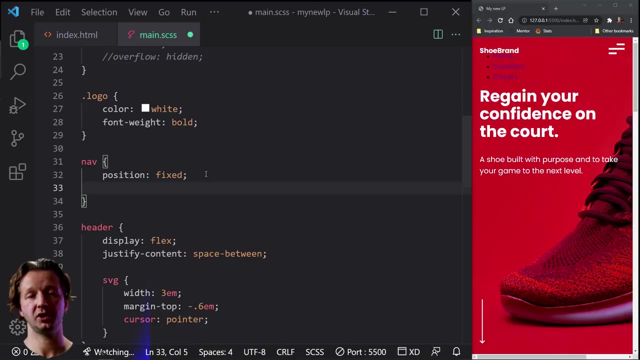 it shows up a nav, a navigation somewhere. So what we'll do is we were going to use position fixed. Fixed means: when I scroll down, guess what, It doesn't go away, It stays right there, which is what you want with this type of navigation on mobile. Well, we want to position this: 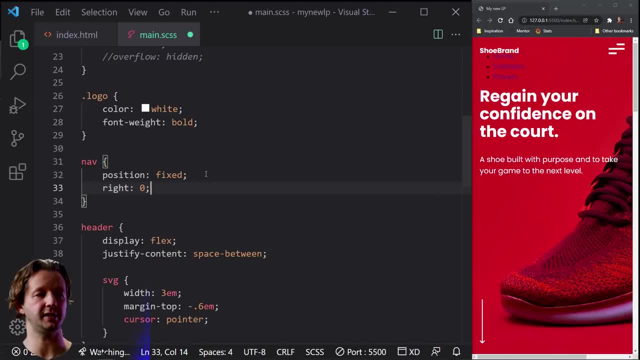 to the right. It's going to slide in. actually, from the right We're going to say right, zero, All right, And then we're going to say top zero, And then we're going to go ahead and give it height a hundred viewport height. Now we can't really see the difference there. 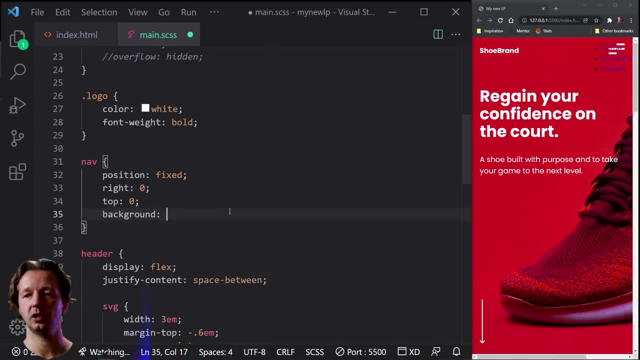 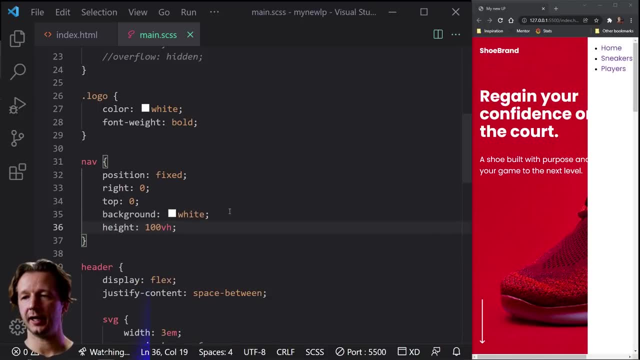 until we give it a background. So I'm going to remove that and I'll show you. background is white. Now we're going to say height: a hundred viewport height. There you go. Next up, we're going to make the width about half, oops, or 50%, because you can use percentage values. 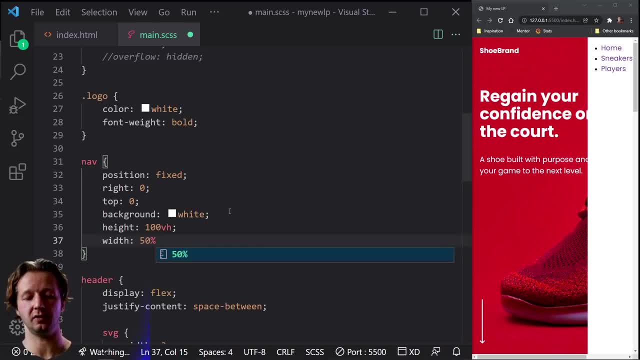 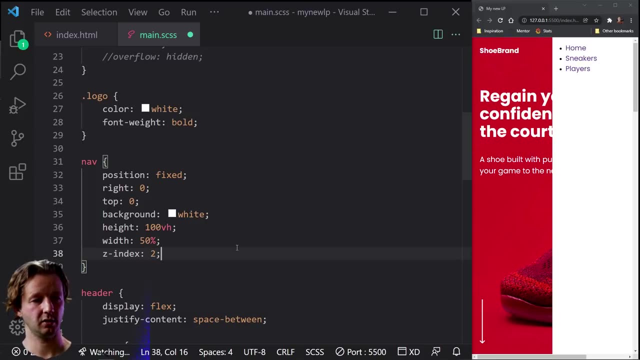 as a unit which is relative to the size of the browser, the device that you're viewing it on, And save it like there. Now we can see it's given us enough space for a navigation, And then we'll also do Z index two to make sure it is sitting on top of this white text. 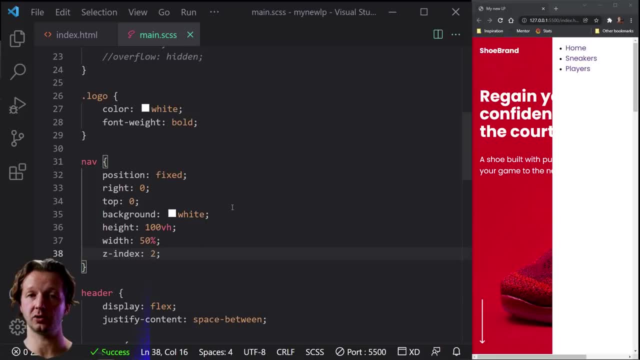 Okay, Because you want this navigation to make sure it goes all for everything. So you might actually want to make this a really high value, like nine, nine, nine, just to be careful. So then also, text transform uppercase allows us to take all this type and make it uppercase. 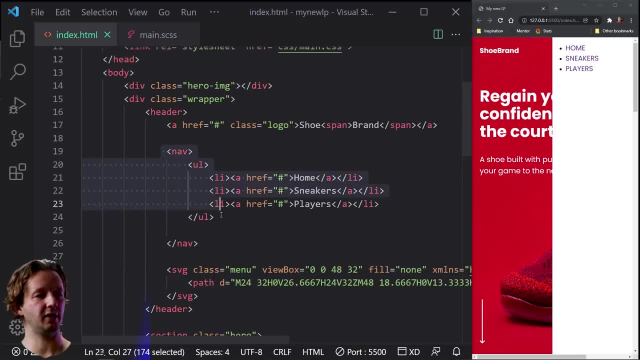 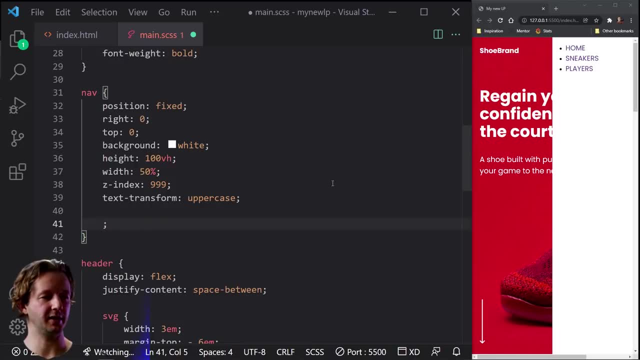 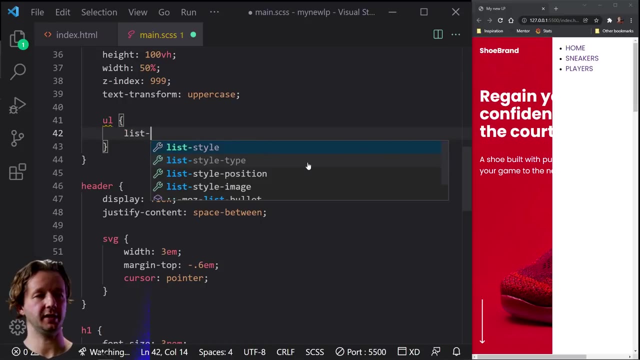 All right, So now, inside, nested inside of an ad element, is the unordered list element. So let's do that. You will enter- uh, sometimes the abbreviations don't work like you want to, So ul for unordered list, we're going to say list. style type is none. That gets rid of these. 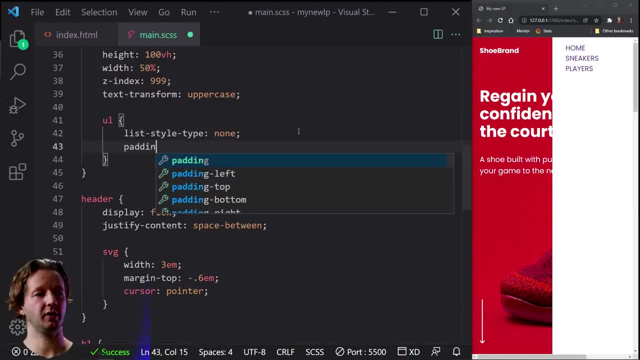 little black circles. We're also going to get rid of default padding because browsers will add a little bit of padding on the left side of these list items. So if we save, that pushes it all the way over here to the left, And then we're also going to push it away from the top by about. 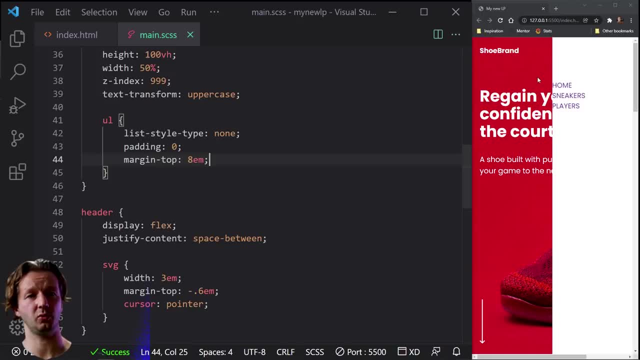 eight M units, So eight times 16, it's really pushing it away because we are going to have a little close button up here Now. then we want to style these right here because these look bad. Purple default color is bad and they're also too small and too close together. So we're going to 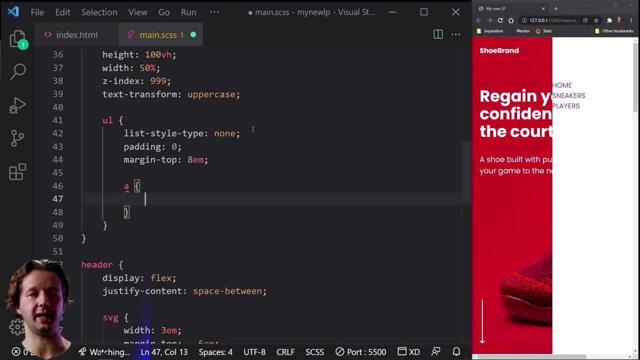 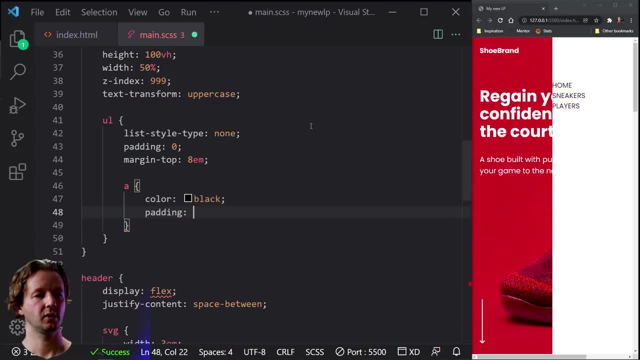 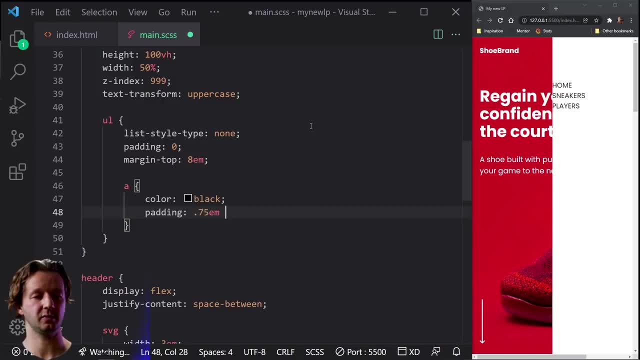 and bottom values by put seven, five Emmy units, And then the right and left values can be two M units. All right, Then we're going to display block and watch what happens to them. So padding on a link element won't work unless it is display block, All right. So hopefully that makes sense. 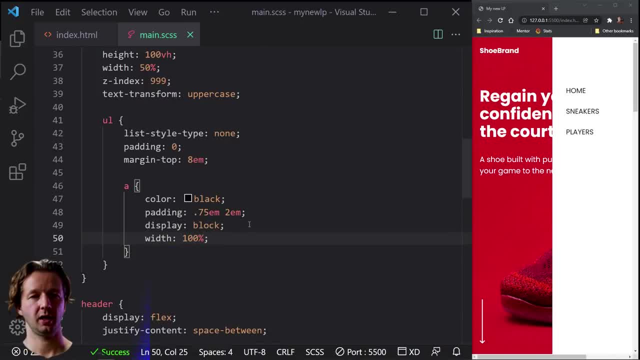 Now we're also going to do width of a hundred percent, And now that doesn't seem to change anything. but if we also add a hover state, which we can do through SAS by putting an colon hover, that means on this a element, we're going to have a hover rule set, just for when the 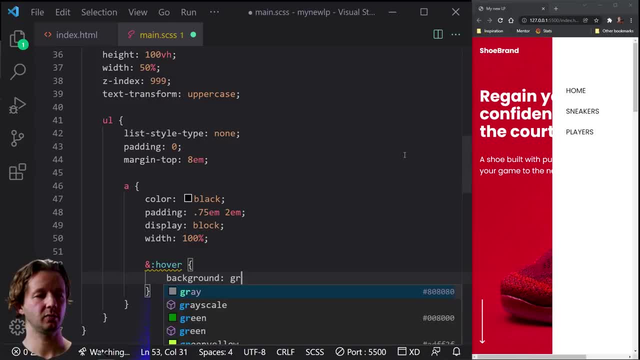 the cursor hovers over it, We can say background gray, We're not actually going to leave it gray, but I'm going to hit save Now. look at that Now. if I remove, remove width a hundred percent, oh, it actually still works. I thought it was not going to work. I think display block will. 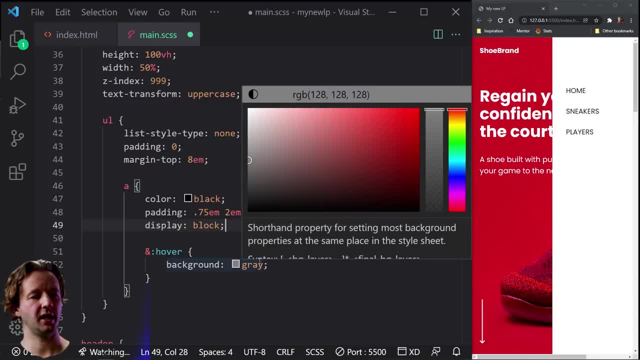 automatically make it that. So so okay, Now we could take this. I think that's too much gray. We want it to be really light. So if we just hover over that black value, we can just use this here to choose a value with our cursor. So if we hit save, look at that. that's a lot better to have. 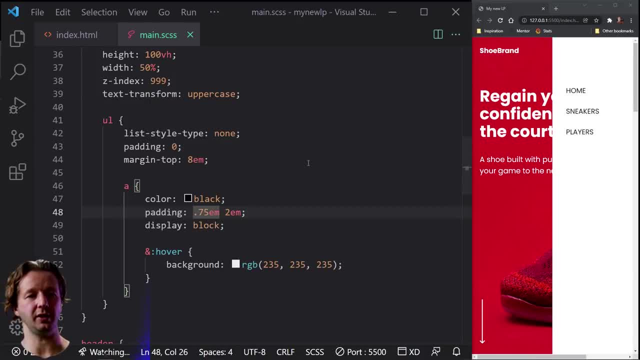 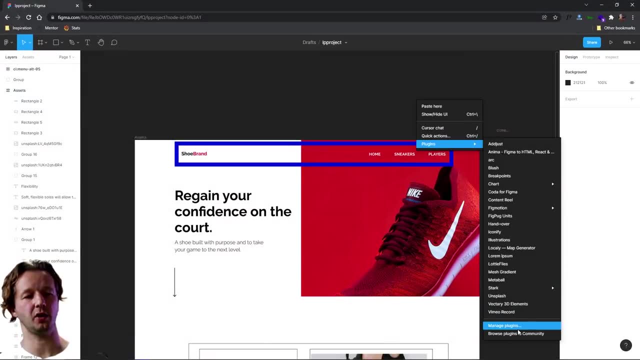 a nice little hover effect. Now let's get that, that close button, working here. So in Figma I'm going to right click and I'm going to use a plugin that I've installed. If you go to bandage plugins or 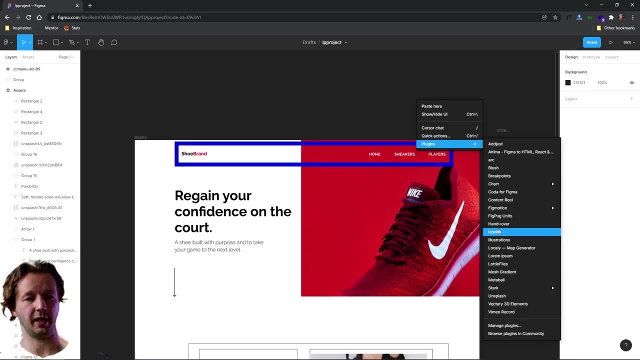 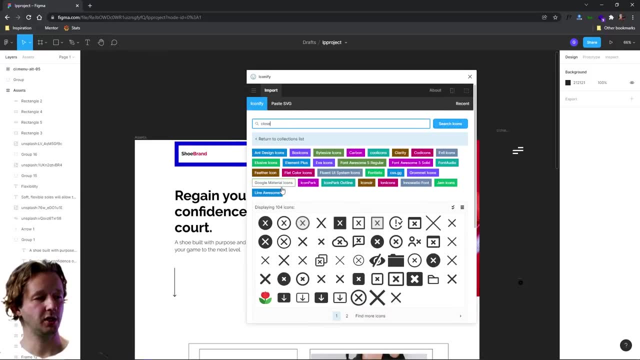 browse plugins in community. you can use an actual plugin called Iconify, So Iconify after you get that installed. if you want to follow along, type in close and you'll see all of these. So I like this one. Let's go ahead and just drag that, And we want it to be black already. 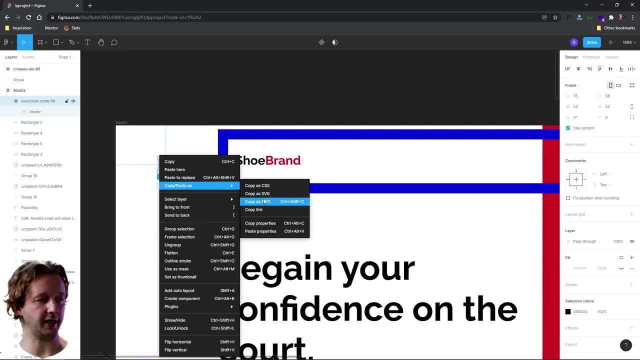 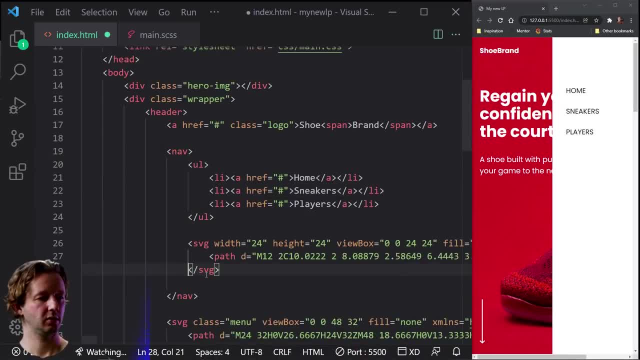 So we right click and we do this copy as SVG. All right, So we go back to our HTML and we're going to put it right here. Now we're going to get rid of width and height. class equals close, And I believe that is what I did in my reference code. It is just to make sure this is all working. 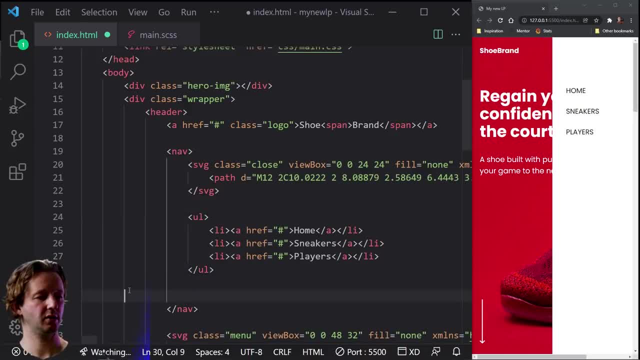 I think it won't matter. I'm going to put it at the top because that's how it is in my reference code. All right, We're going to save that, And now you can see it's showing up. but we have to. 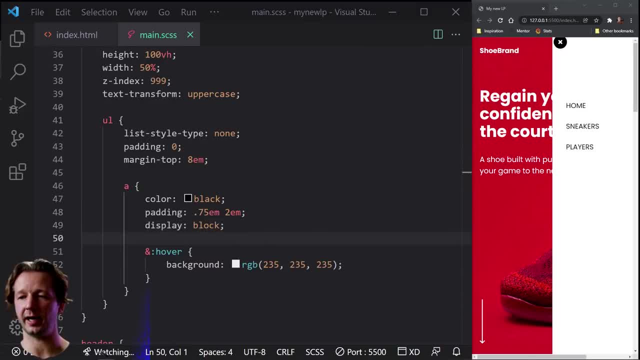 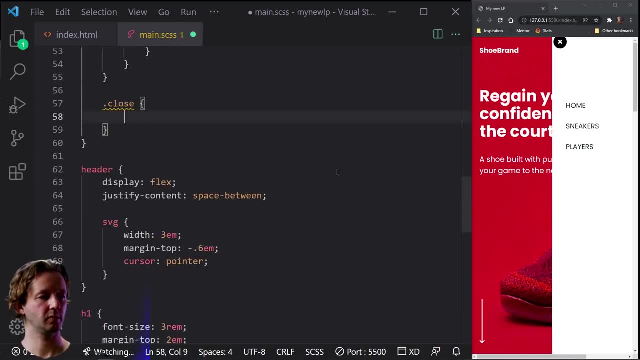 actually be able to do that. So we're going to save that. And now you can see it's showing up, but we have to actually be able to position it now, because it's not in the right area. So underneath here I'm going to put in close And in close we're going to put float right. 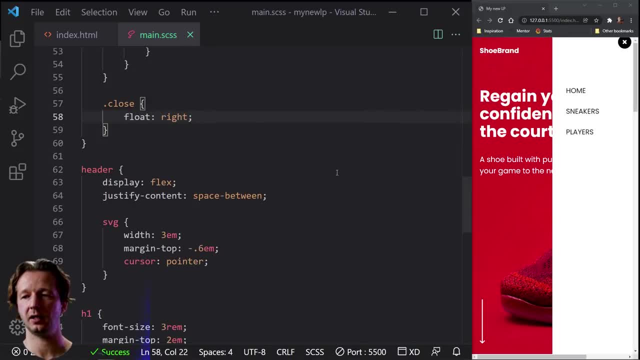 which is a way just to kind of push something over on the right side, And we can also do margin, 2M units, and then also width, 2.5M units, And I think that's good right there. So this is our mobile navigation when a person clicks on it. So now we need to hide it. So remember I didn't. 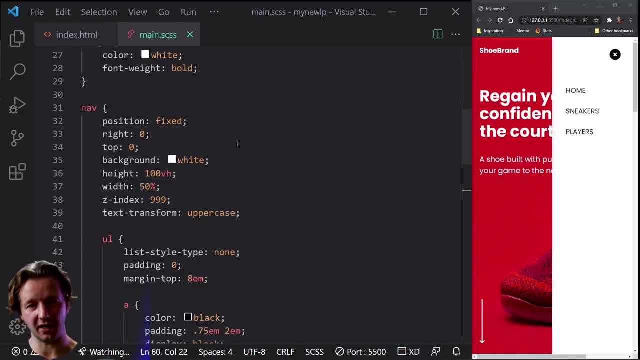 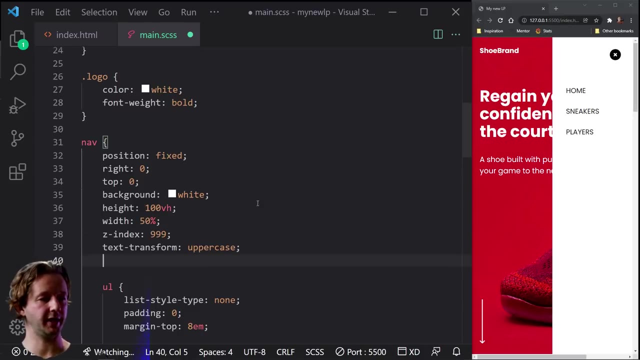 want to hide it through display, none because I want to be able to animate it and kind of have it come in when we get to that portion in a bit near the end of this video. So what we'll do is we're going to use transform to hide it. So what we can do is put on the nav element transform. 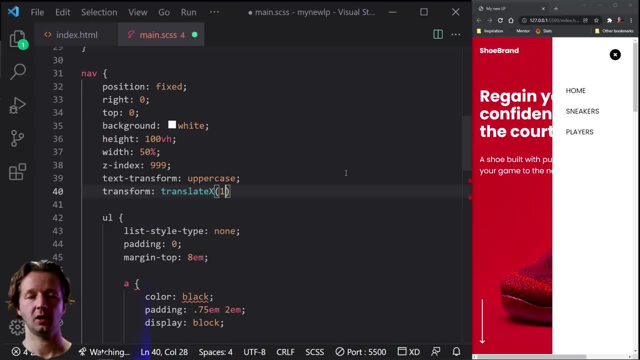 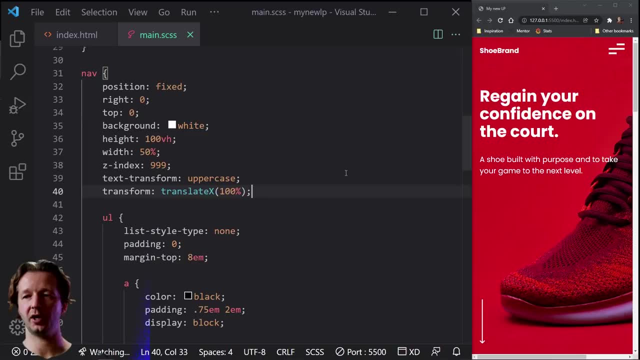 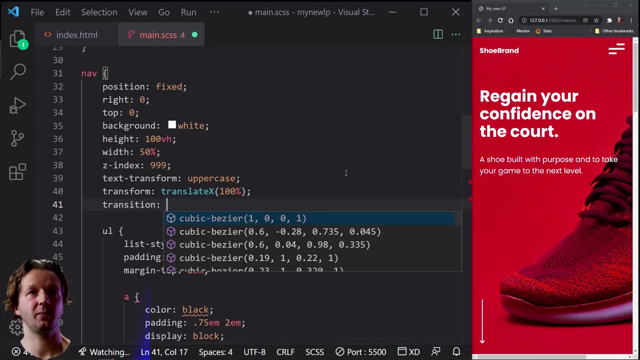 translate X 100%. It's gone, We no longer see it. And then what we can also do, just for future reference, is transition. Transition is a way to specify what type of property should animate from one point to another. So when we create a little bit of JavaScript, when a person clicks this: 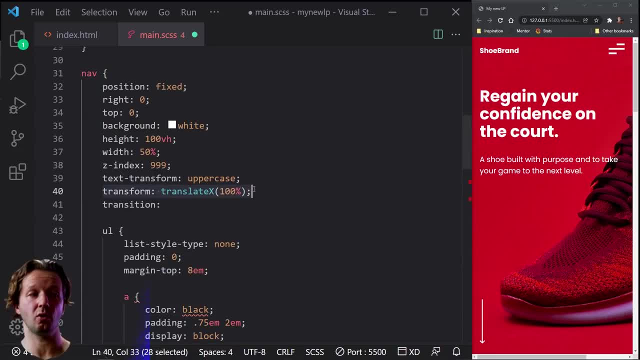 element. we're going to change this transform property from translate X 100% to zero. All right, So we want this to animate, So we put transition and we put in transform. We'll say for a duration of 0.5 seconds, half a second, and we'll have some ease. 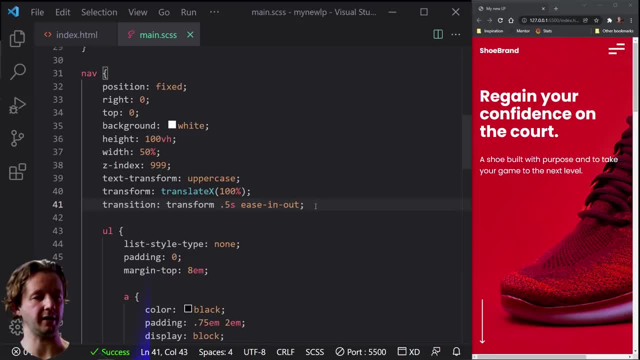 in out which can affect how the animation looks. For now we're not going to see that. For now we can't click on it. It doesn't work. We'll get that working later on because we need to finish up the rest of this, which we're actually pretty close to doing that already. All right, 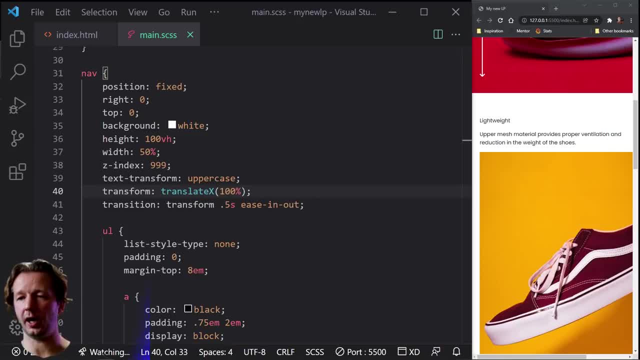 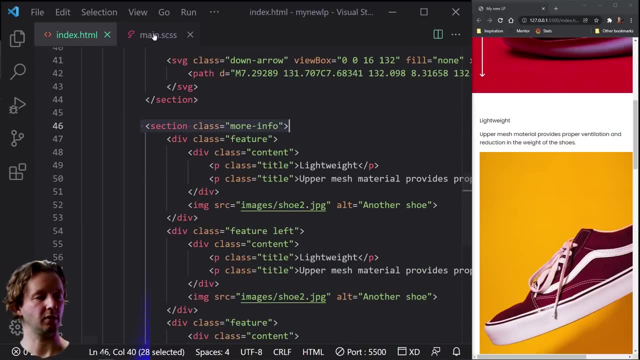 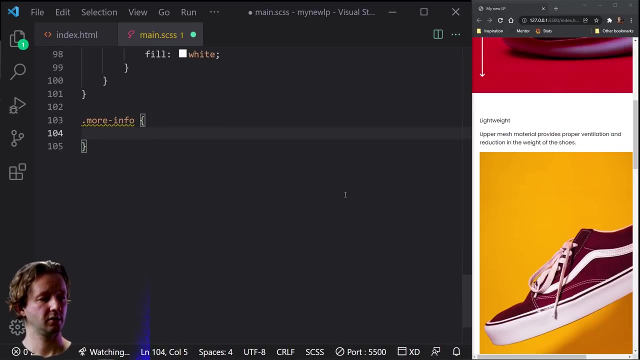 So next up, we're going to focus on our more info section, which is right here, All right, So let's reference that It's coming all the way down here. We're actually getting close to having this part finished, or at least the mobile CSS, the mobile first CSS. So more info, actually we don't. 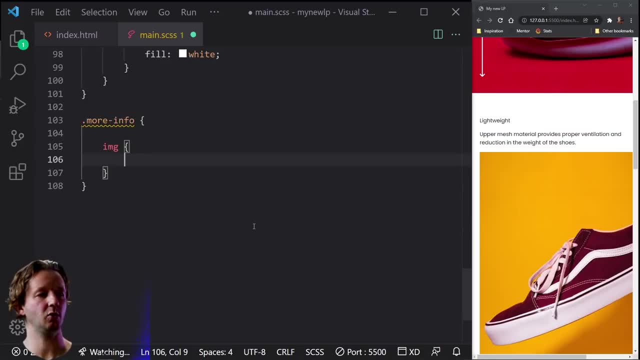 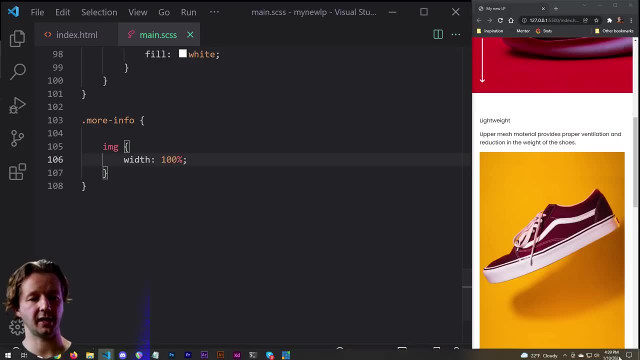 necessarily even have a rule set for that, but we can just reference this stuff inside of here. We can say image. So all of our images, we're going to say we're going to make them responsive with a hundred percent. Notice that that got rid of. 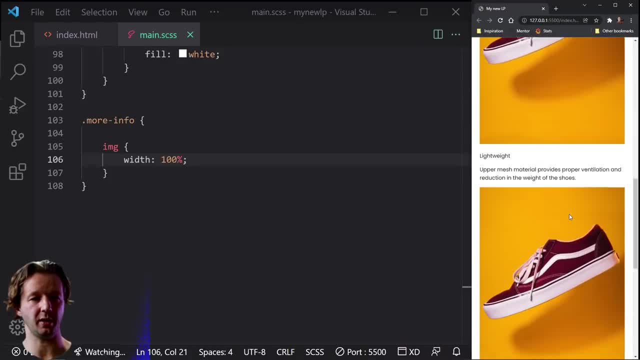 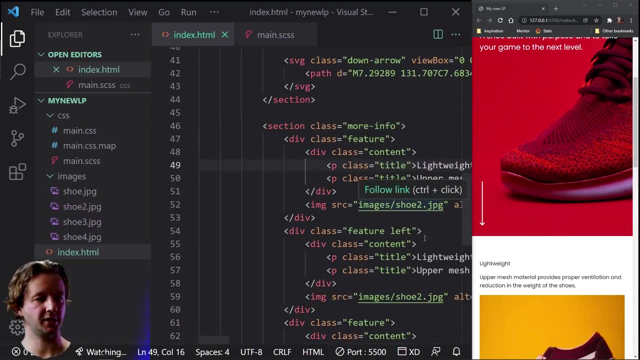 that horizontal scroll bar, So we don't have that scroll issue anymore showing up. Oh, and also control B. I do want to change these. That's two, This is going to be three and this is going to be four. That way, we have different shoes showing up. 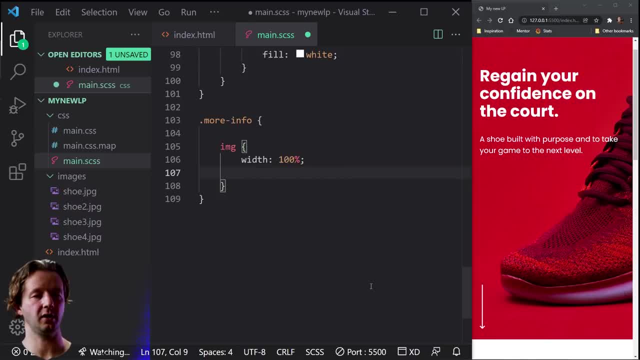 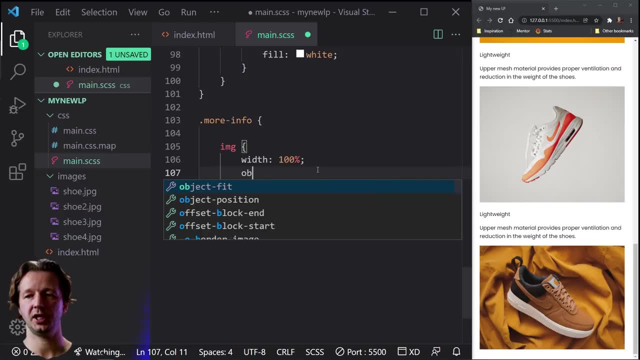 And I'm also going to change another thing. Notice how there are different proportions right now. This is real tall, This is kind of like a. you know like a. you know like a, you know like a square, And so is that one. If we change the object, fit hyphen cover and also give it. 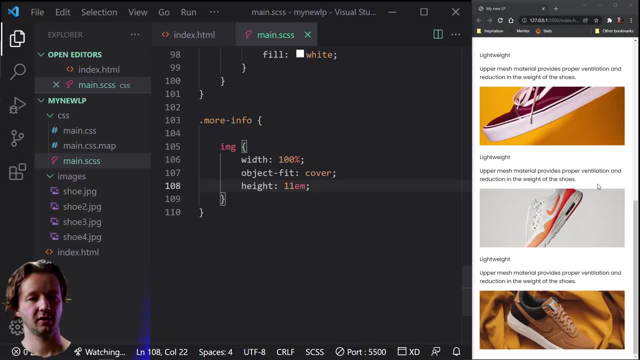 an explicit height of like 11 M units. guess what It changes the? it changes the element, the images, this object fit cover. For instance, if I change, if I remove object fit cover, it kind of distorts them. right. If we add that, it keeps them there. Very, very cool. 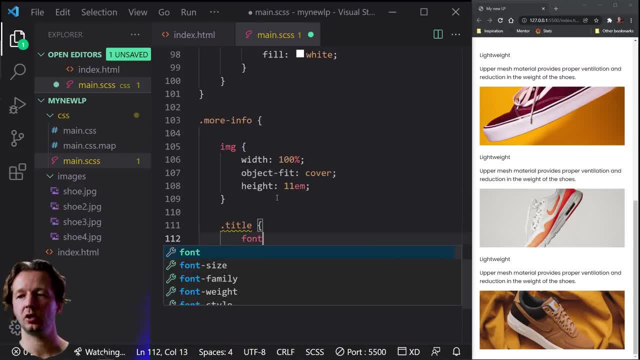 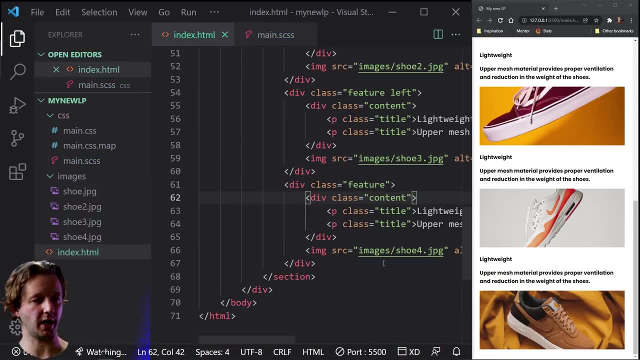 Next up is our titles, which is a class of title. Font weight is going to be bold, bold. And why is that affecting there as well? Oh, it's because we forgot to- I rather forgot to change- that This should be description or DESC for description. There we go, And also. 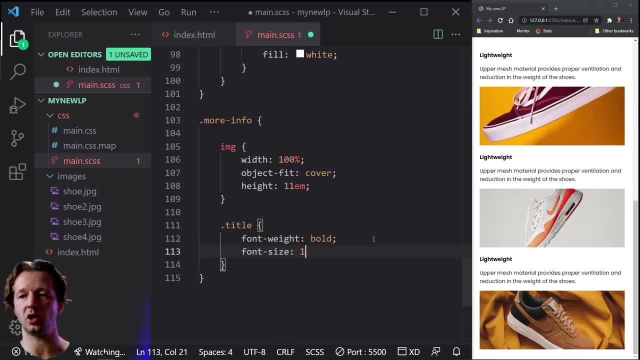 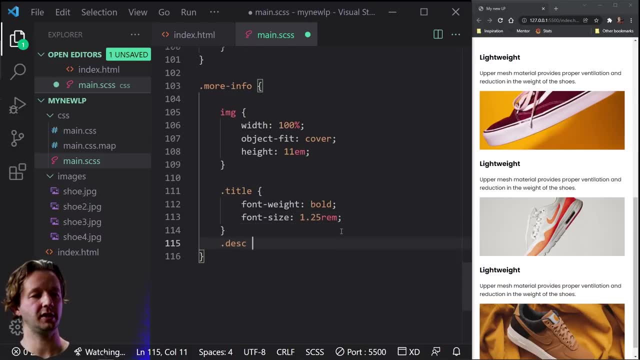 we'll change the font size, make it a little bit larger to reinforce what's called visual hierarchy. That's a, that's a UI design idea, or design idea in general, actually, And then also our DESC, or descriptions, line height. We're going to adjust the leading or the line height, And then also. 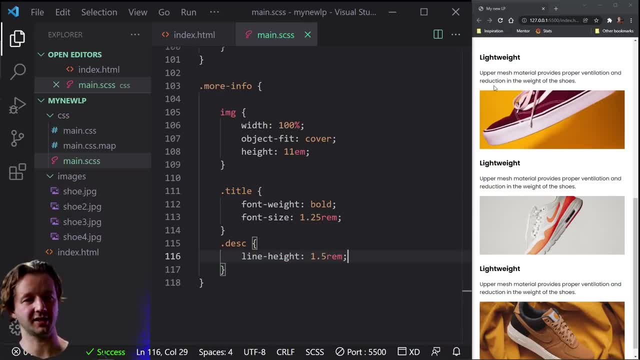 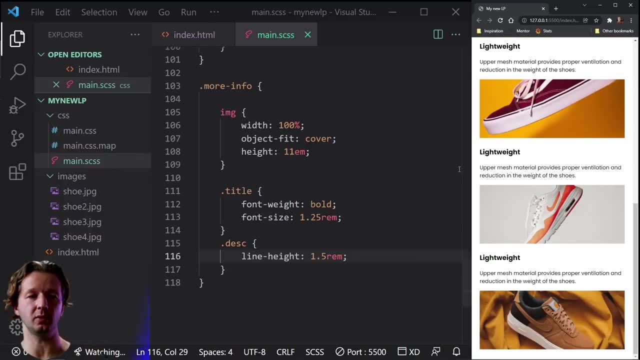 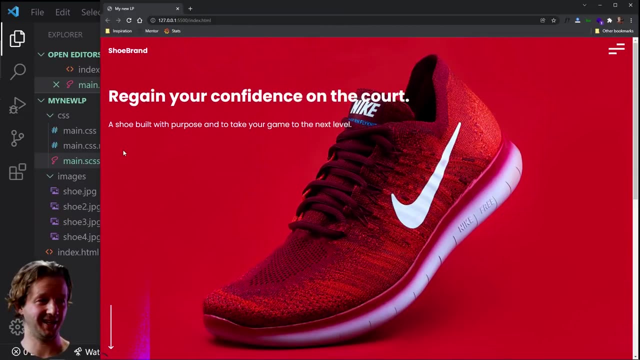 line height to 1.5 REM units, And that kind of just slightly tidies it up a little bit. And there we go. This is the actual mobile design. Now here's the problem. If we review this on a tablet or even a desktop, this is what the design looks like. It looks like garbage. That's why 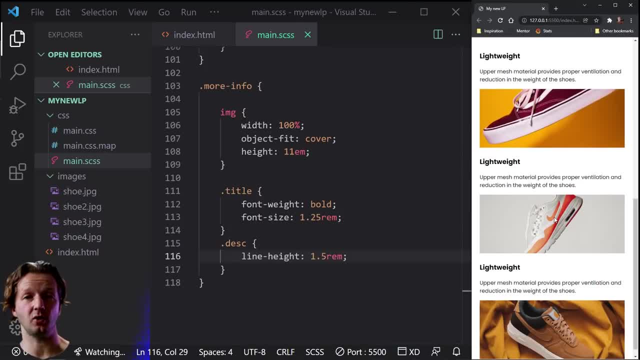 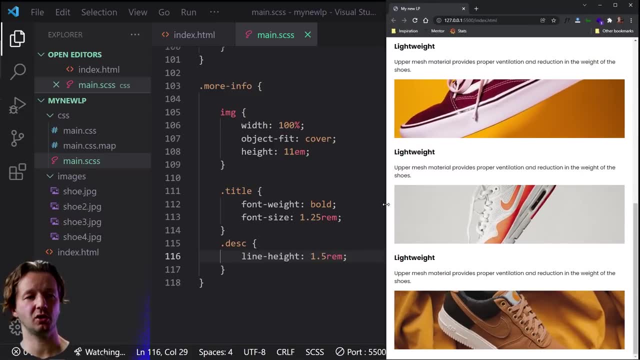 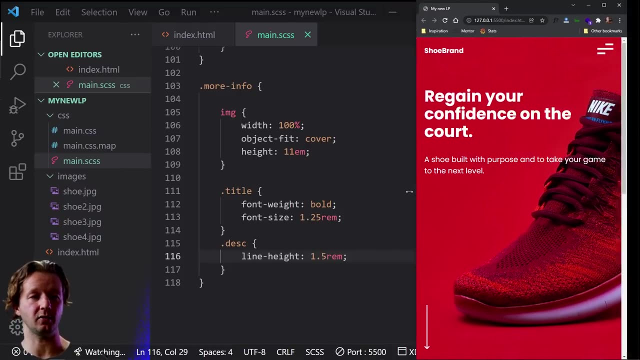 we have media queries or responsive design. So now what we do is we ask ourselves what should, at what point should we start to readjust this layout so that it looks good on a tablet or something like that? Or so many times? 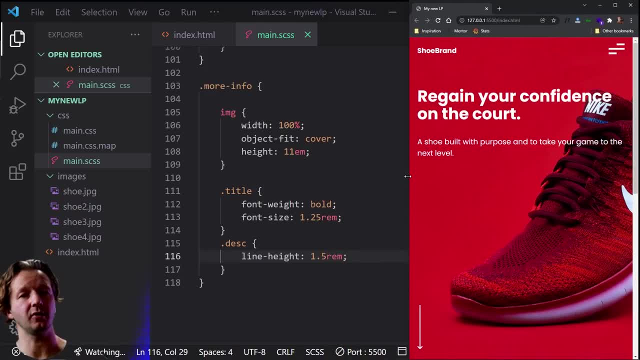 if you're a front end developer, a UI designer will have thought of this already- or a UI UX designer, I mean, they might provide you with a prototype to say: Hey, this is what this looks like here on a tablet. code it for us to make it work. Here's what it looks like on desktop. 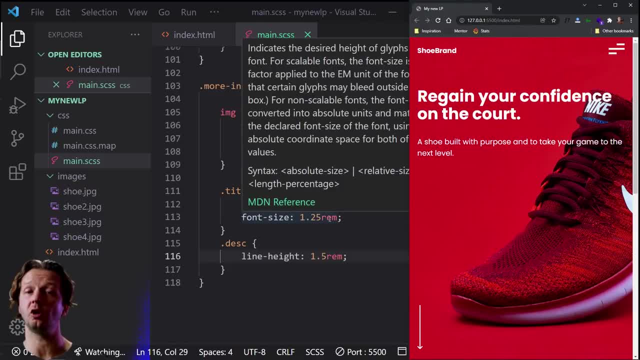 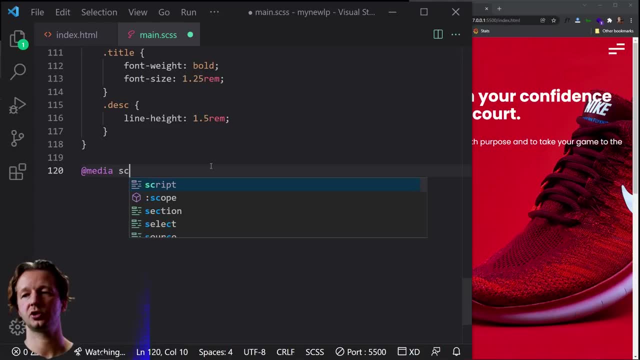 So the way we start to adjust this is through what's called media query. Here's what a media query looks like. Control B: to get rid of that, We're going to do at media only screen and, and then parentheses, minimum width or min width, And we'll say 680 pixels. 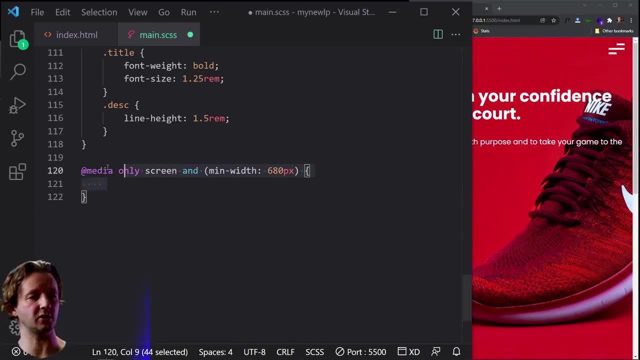 Now that's confusing as all hell, but basically what this means, this whole rule set. what this means is that, once we get to 680 pixels, only the rule sets that are going to be defined inside of here, that are necessary, are going to be defined inside of here. So that's. 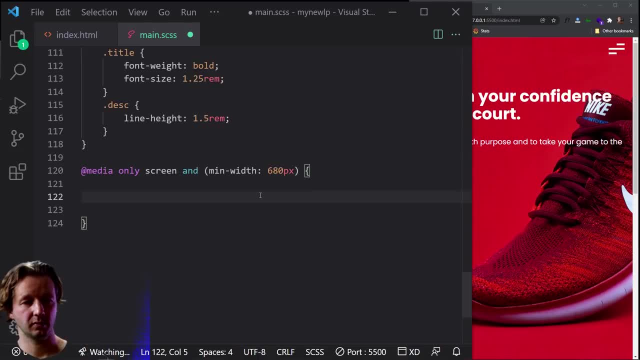 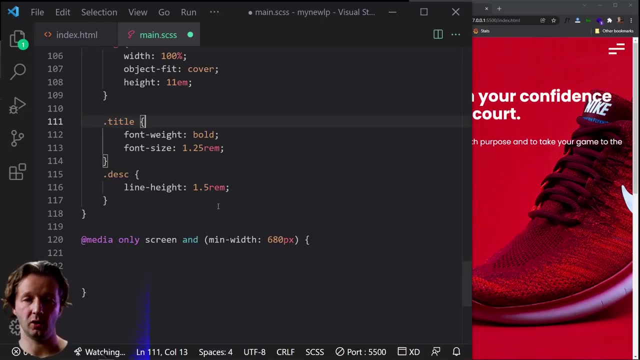 me. So these little numbers here, all of them- I've messed it in there- are going to count. So at minimum width, All right. So anything underneath that which is like this stuff over here, you know we'll get counted, All right. So if you were to do desktop first, you'd be changing. 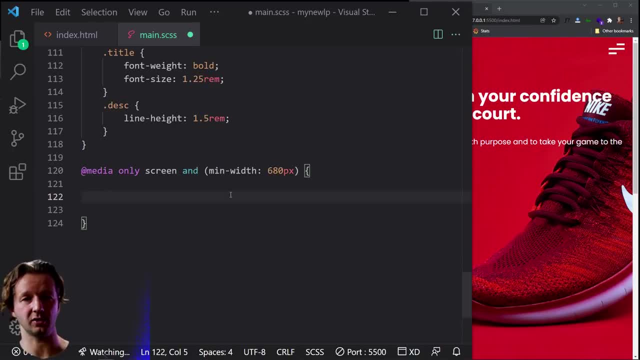 this to max width, but I like min width better. So do many other people. All right, So at how do you know what is? 600 pixels though 680 pixels? It's like: is it here, Is it there? Well, if you. 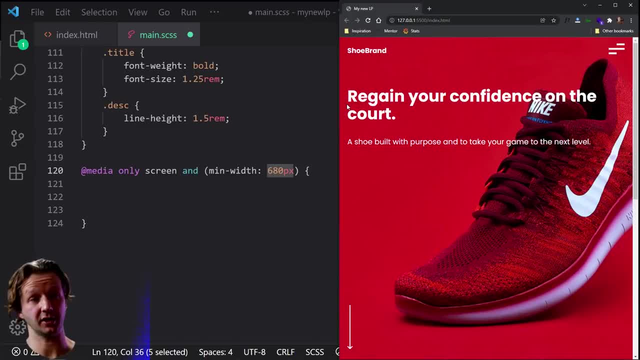 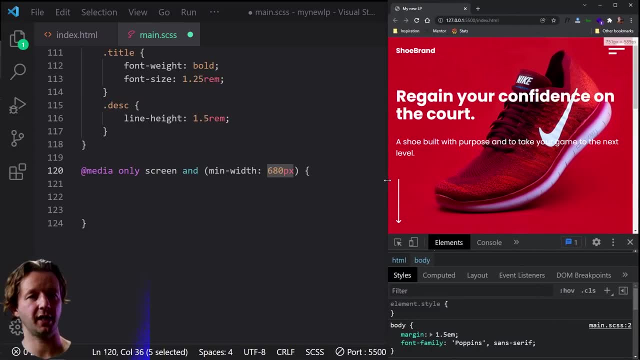 use your dev tools. I hit print screen by accident. I hit F12.. If we start to scale this in and out, you can see on the very upper right corner. it's probably hard to see in this video, but it'll show you the width. 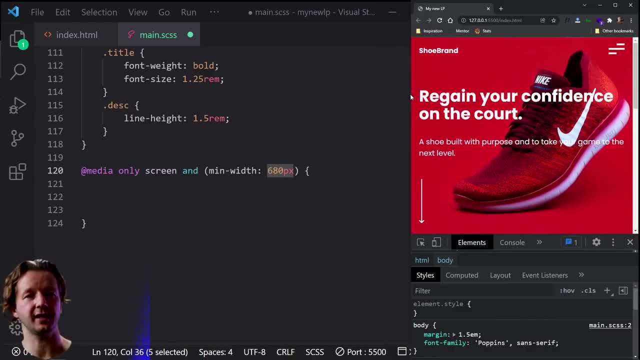 and height. So the width is changing, So 680 is like right around there. We're going to make some changes right around there. So, basically, this design is going to look like this only up until this point. So what are we going to change? Well, we're going to change something very simple. 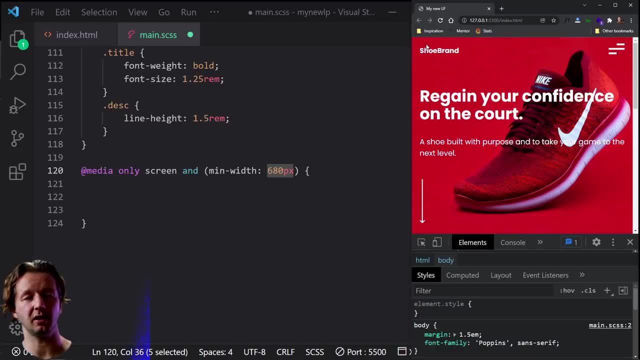 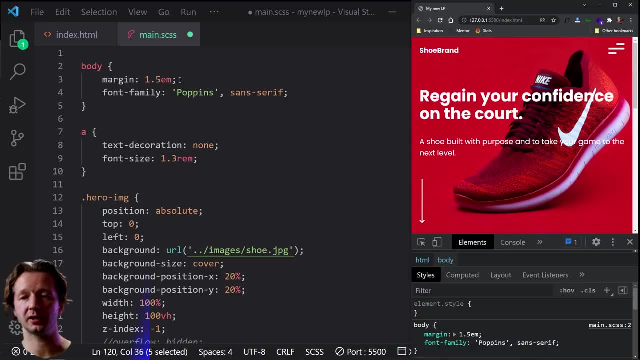 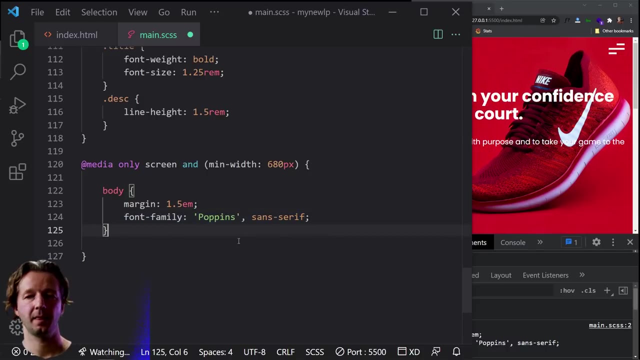 We're going to give ourselves more white space, which means, on the body element, we're going to take our margin element and we're going to grow this to something higher. All right, So let's just copy this real quick: We're going to come down, paste it in and we're going to leave 1.5. 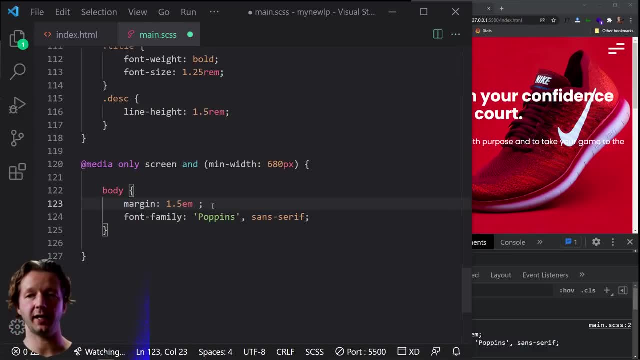 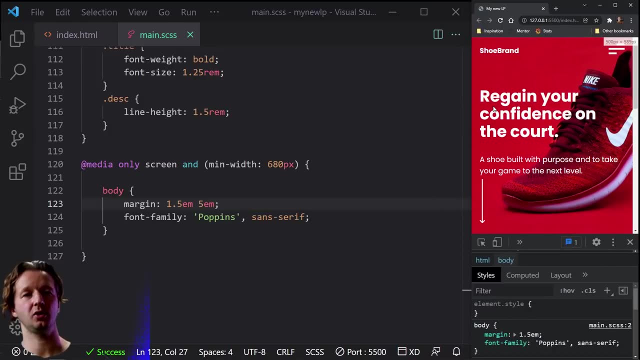 M units on the top and bottom, but on the left and right we're going to really bump that sucker up to 5 M units. So let's save that and look at that. So watch what's really cool. We're down down here. We're underneath 680.. This is not counted. 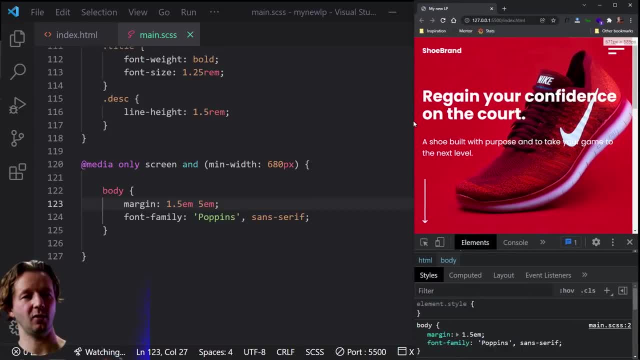 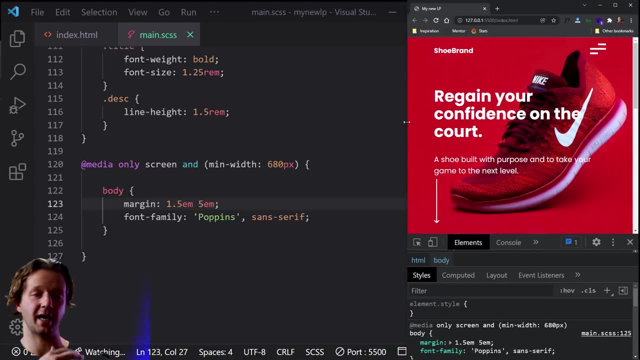 yet We're approaching 680 rapidly and watch just like that. It's magic And so it doesn't seem like much. but once you start adding more rule sets, you can drastically change the entire appearance of the layout through properties here, or rule sets rather. 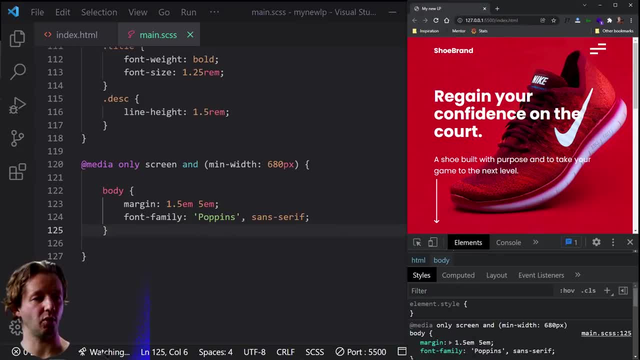 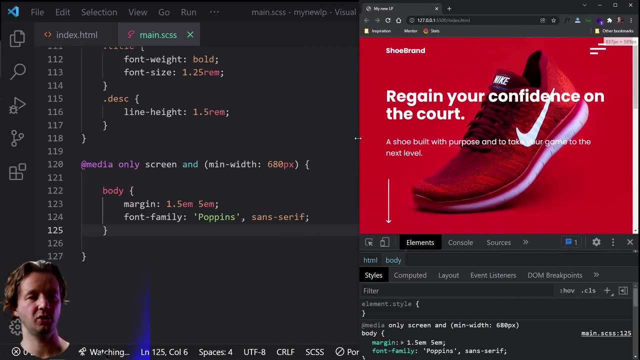 So that's the only change we're going to make there, at that breakpoint, as it's called with this media query. So they're called breakpoints, All right. So at what point next do we want to start adjusting things? Well, I'm going to say it's probably going to be around 920 pixels. One thing: 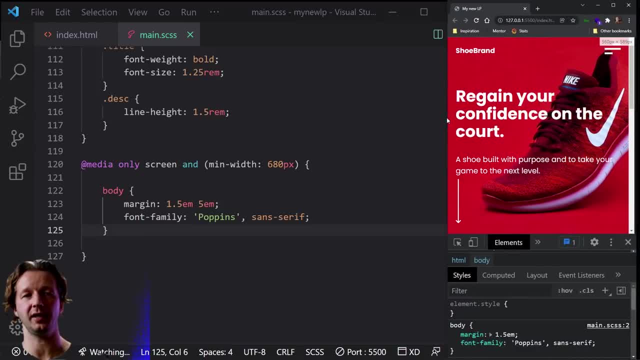 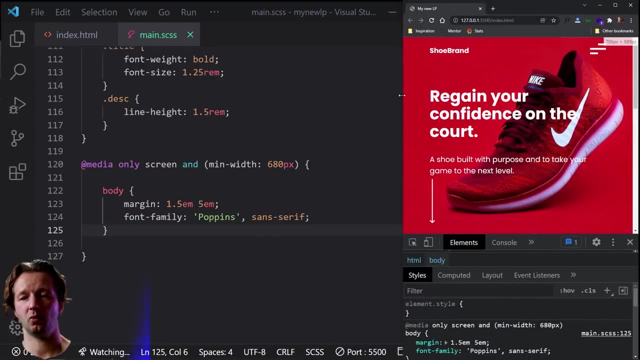 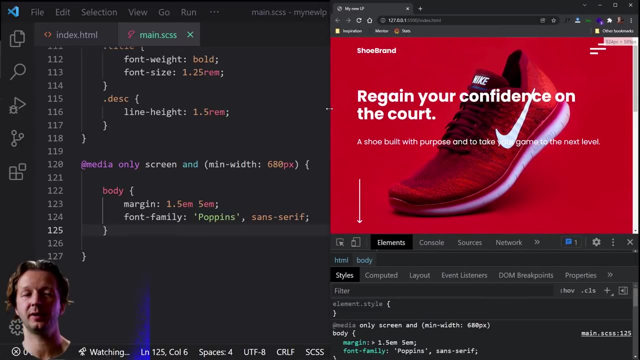 you have to ask yourself: at what point do we have enough room to put our three links and get rid of this hamburger menu, as it's called? Probably even right here we could put it, but we're just going to put it Right at 920 pixels, or right around here or so. Arguably we can go much lesser than that, but that's. 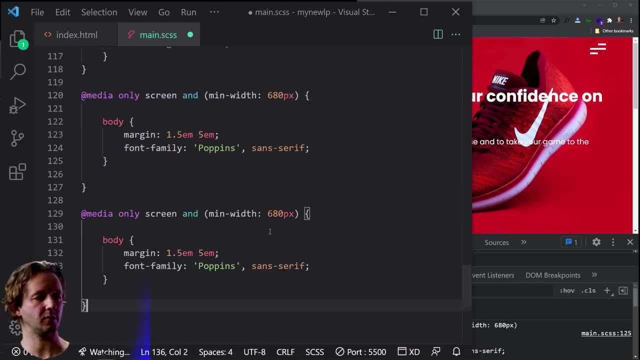 how I have my code structured, So it's just copy this stuff. So we have to rewrite it again. We're going to put 920 here and then we're going to get rid of this. So what we do is we take a look This: 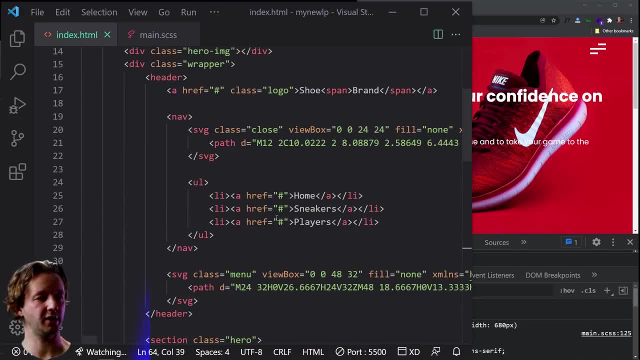 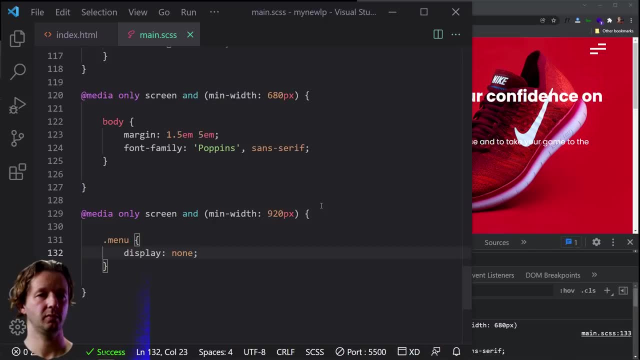 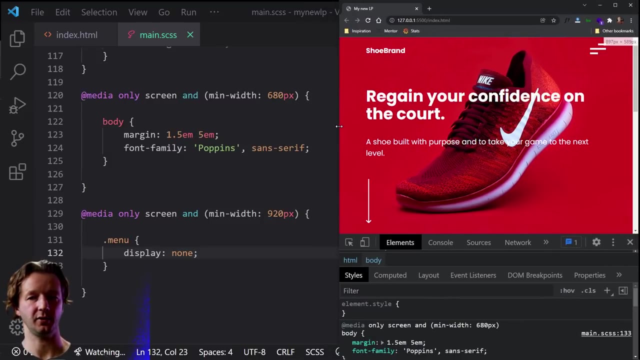 right here, has a class of it's SVG menu. So we hide it. So we say menu Display: none. Now we get out to 920.. Watch it hide. See how it hides. Very cool. Now we take our nav, which is currently pushed off to the side of the screen with 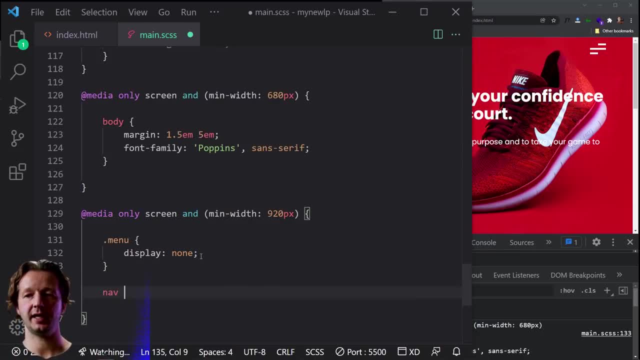 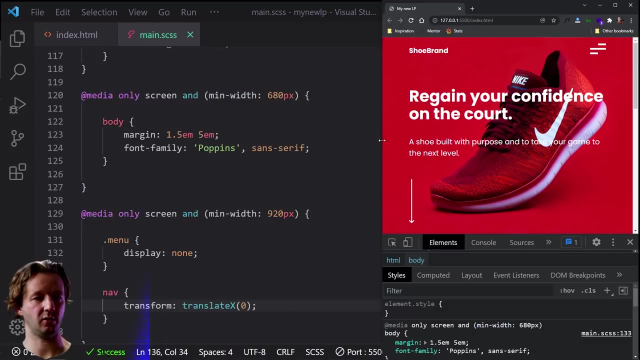 transform, translate X: a hundred percent. What we say is nav, We are going to transform and we're going to translate X: zero. All right, So let's pull this out Now. here's the problem. It's showing up, but it's showing our 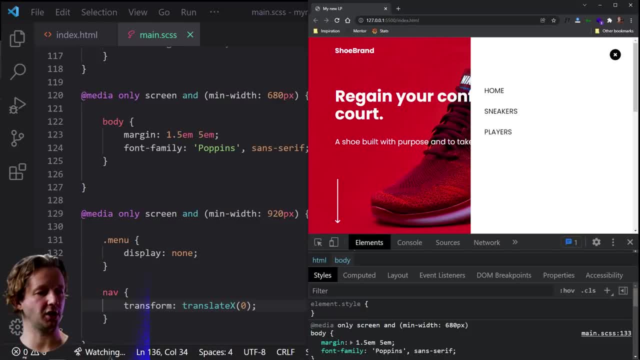 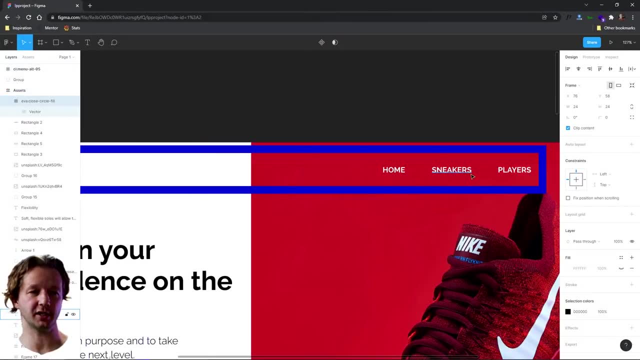 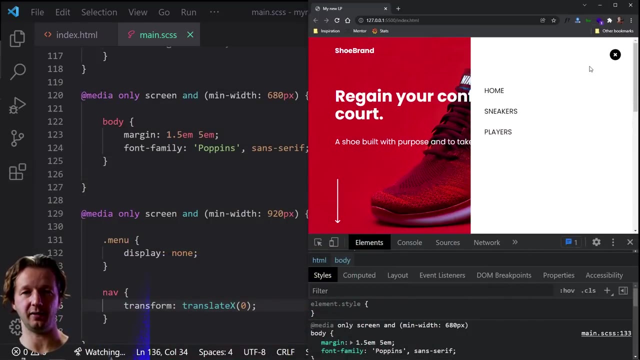 actual mobile version of the menu. It's not showing the menu, Right? If I can get it up. it's not showing this menu. It doesn't look like that, right? Well, that means we're going to have to rewrite some of this, the properties, to override this stuff and put and make it so that it looks. 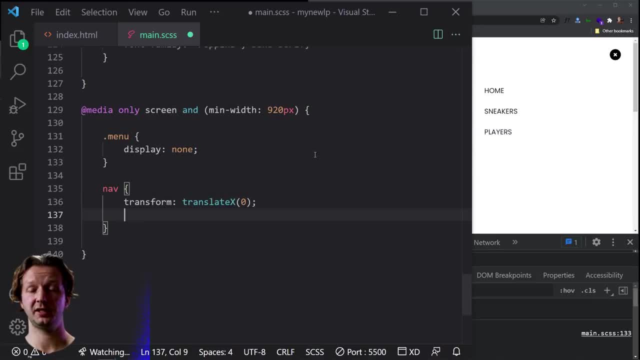 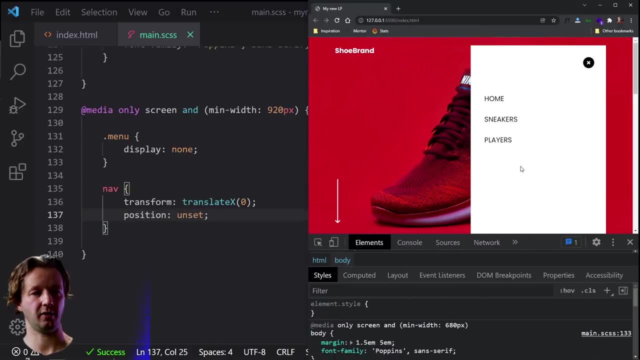 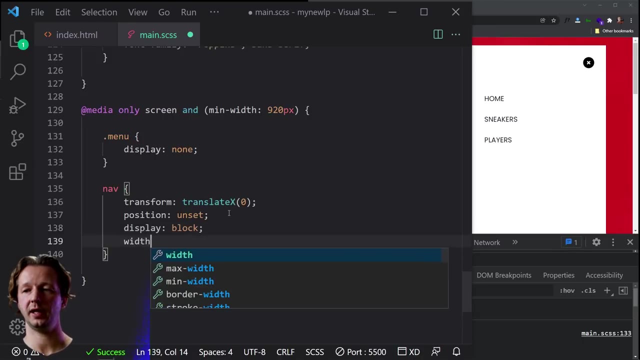 like that figment document. So here's how we do that. Remember, is position fixed. We weren't going to change that and override that by putting position on set. So now we're getting somewhere slightly. We're going to put display block, We're going to put width auto, We're going to put height auto and we're going. 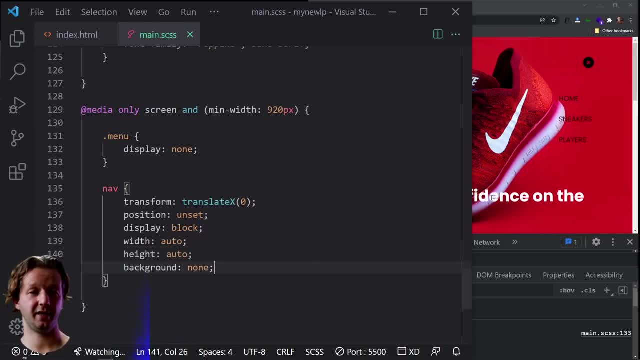 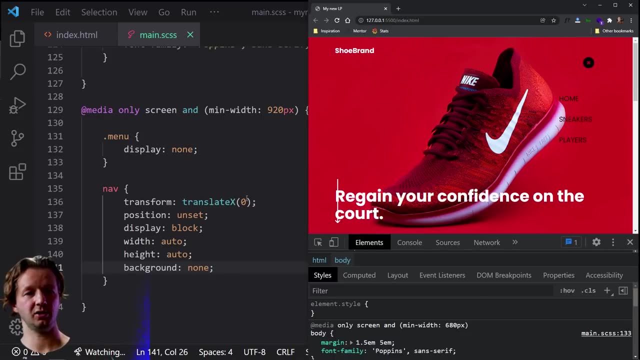 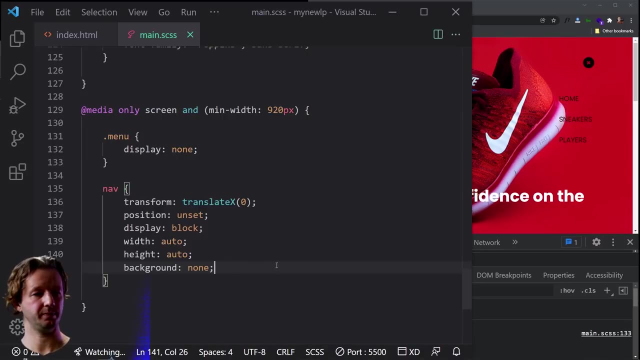 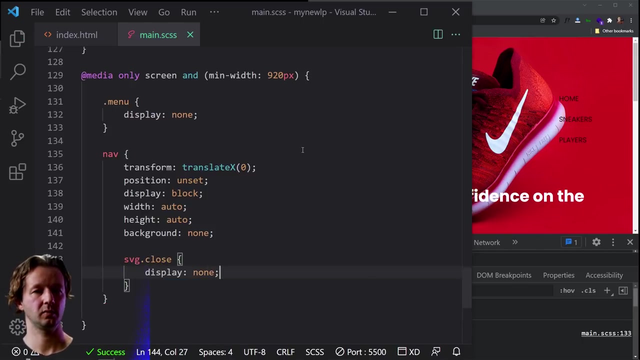 to put background: none, We're getting close. As you can see, we've overwritten a lot of stuff here. Now we are close. We don't need this close button, because this is always going to be there on desktop. So what we can do is we can come down here, svgclose. We can say display none. All right then. 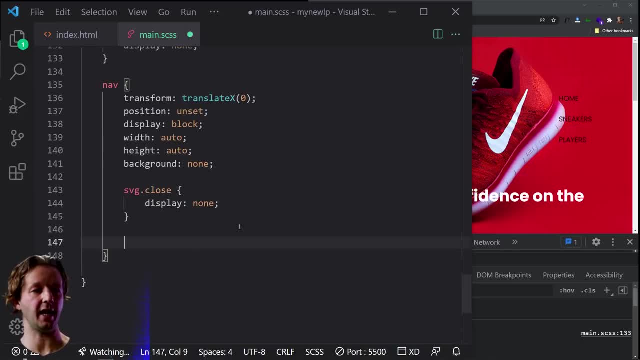 our unordered list, which is defined as an ul element, We're going to say display flex- Remember, display flex on a parent container. And then we're going to say display flex on a parent container. And then we're going to say display flex on a parent container. And then we're going to say display flex on a parent container. 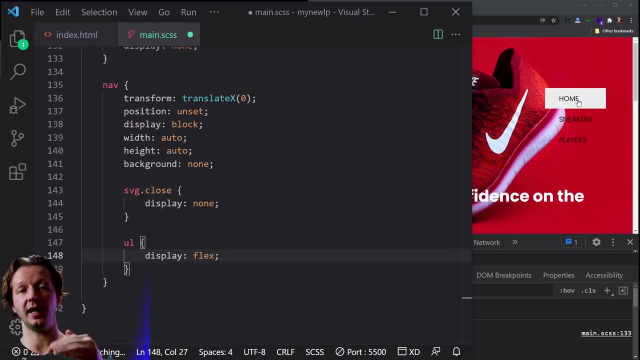 any else, any child elements inside of it that are nested in it will become columns, and we want them. like you know, we want them in three columns, so display flex, all right. and then I we're also going to put margin zero, so that gets rid of the default margin from the unordered list. 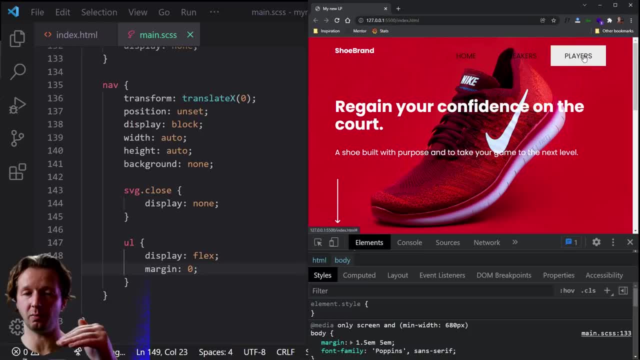 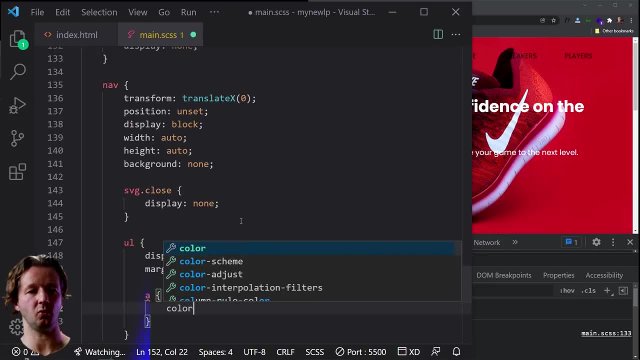 or the the. it actually wasn't default. we defined a margin to push it down in that mobile, so now we're just resetting it to zero. then we take our actual links. we say color white because we can't see them barely as they are, and then we also specify a padding. let me move this, get this out. 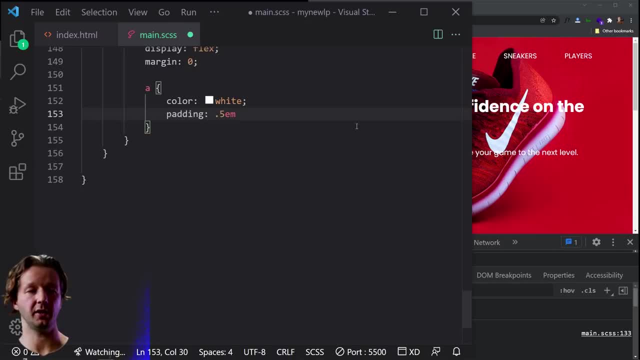 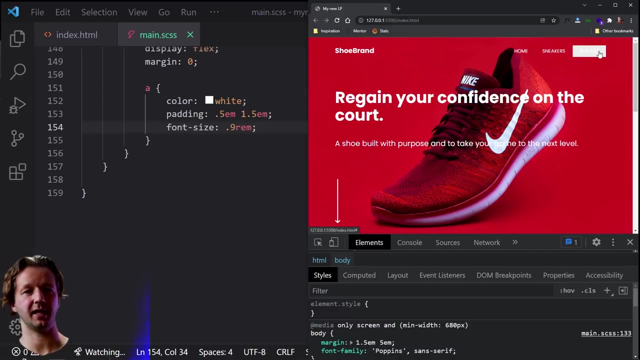 of the way. we'll put padding of 0.5 on the top and bottom and 1.5 on the left and right. then font size: we're going to make it a little bit smaller to 0.9 rem units. look at that now, the hovers. we don't want hovers like that because we can barely see the type when. 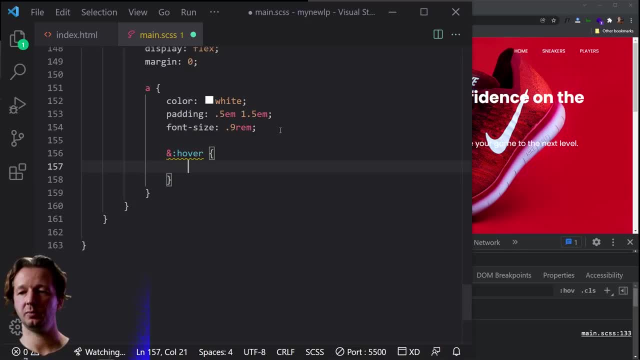 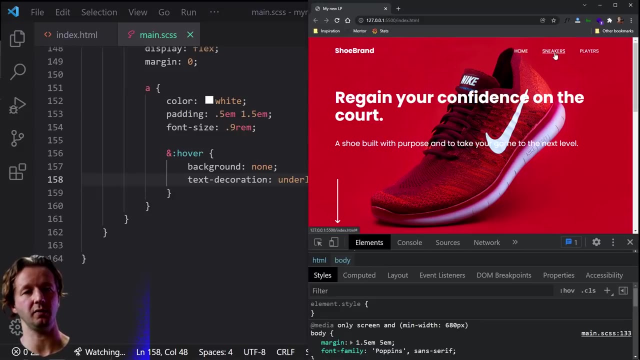 you hover, so and hover, and we simply say background none, and maybe we want a different type of hover, so we'll do text decoration: underline, which brings back the links. so when we underline it, there we go, we have a visual indicator that we're hovering over this particular element. all right, I know. 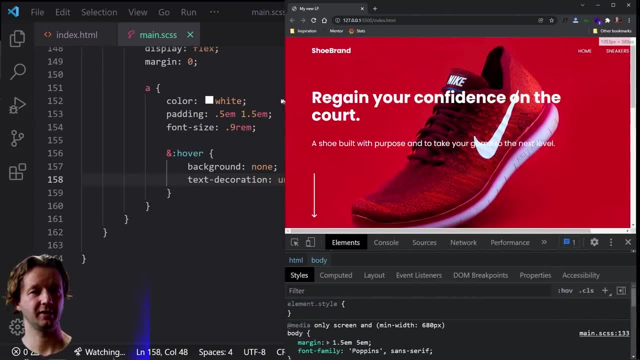 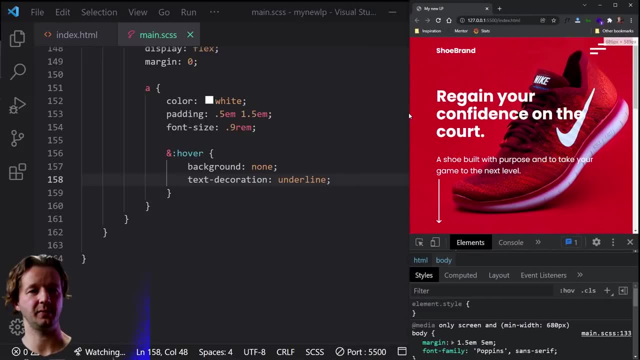 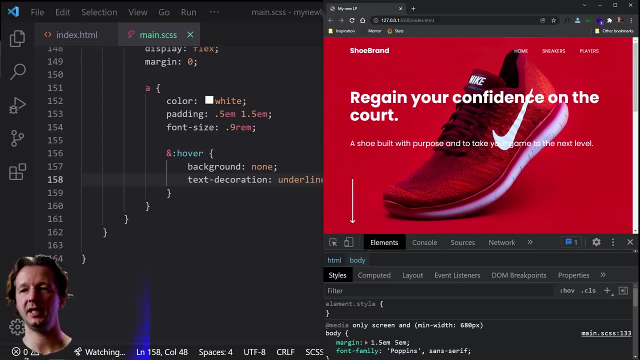 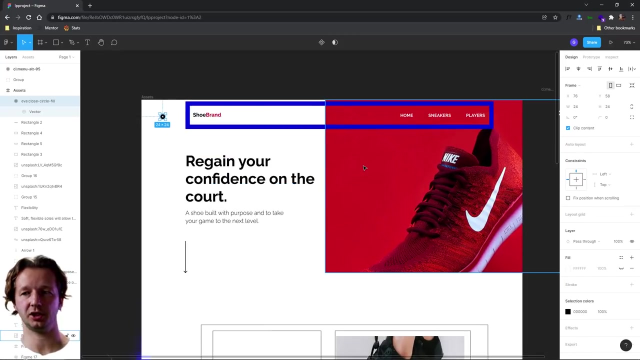 that was a lot just for that navigation. so weird things are happening now. but don't worry, we'll fix that once we I get this working and we start to work through things. all right, so next up, what about the hero image? if we refer back to our design, you'll see we have this desktop version showing up where it's. it's no. 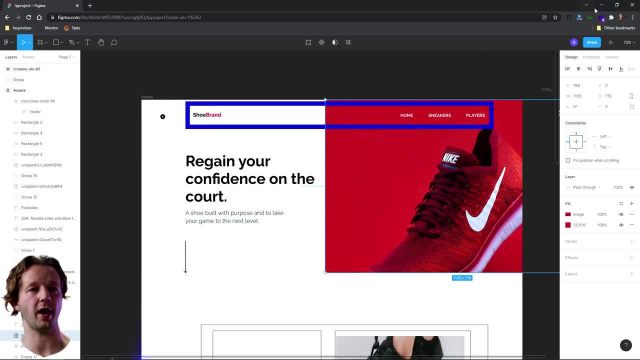 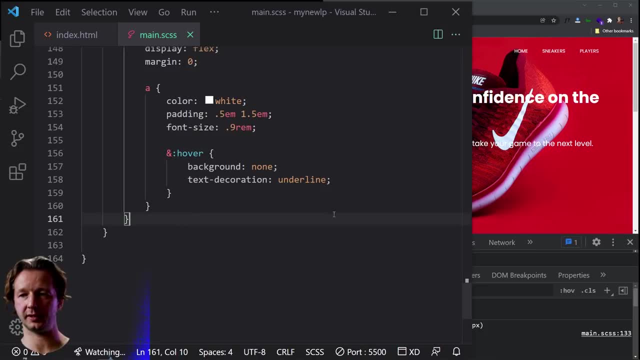 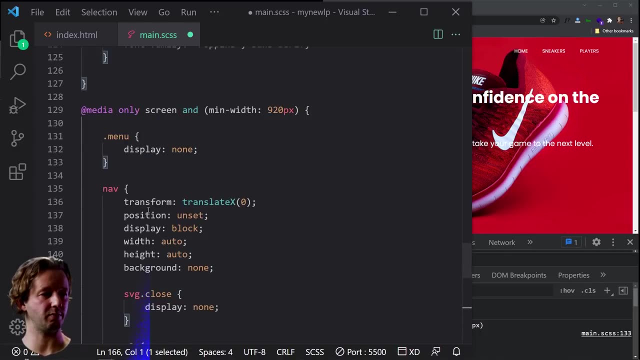 longer fully consuming the layout it's. it's basically halfway, so let's work on that. so after our, let's see here. I want to make sure I am doing everything correctly. yeah, coming out here, this right here, this final closing bracket is still within this media query, so we 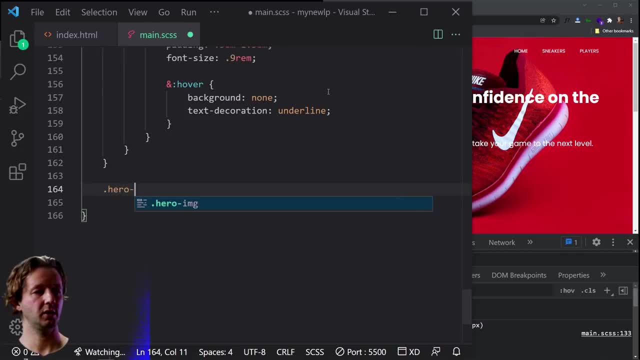 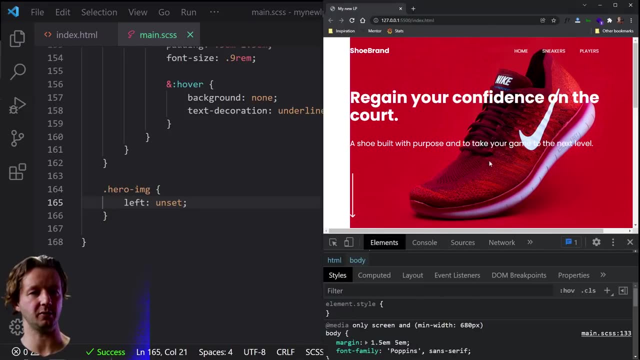 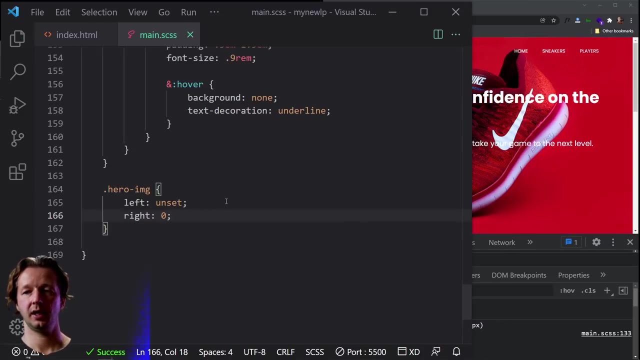 still want to stay in there, and so we'll say our hero hyphen IMG. we're going to say left is going to be unset, so we're just unsetting that value that was placed on there initially. we're also going to say right is zero, because we want to push this thing over to the right, and then the width will be. 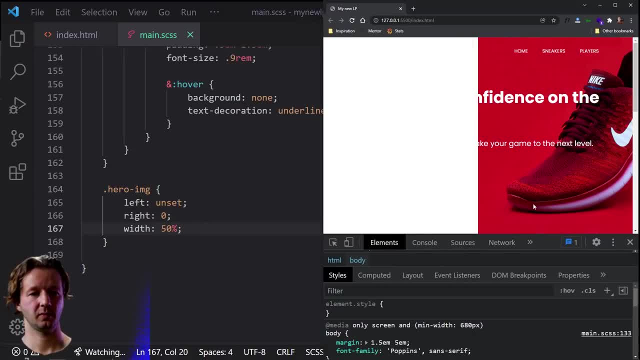 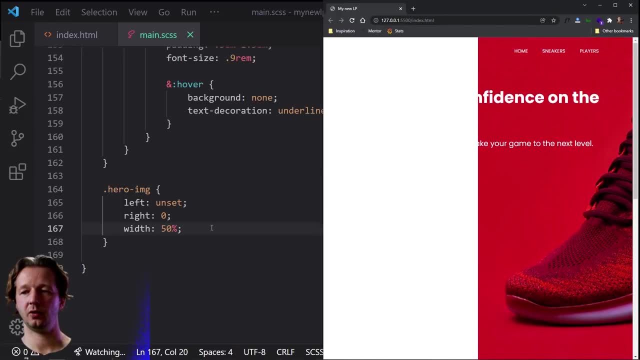 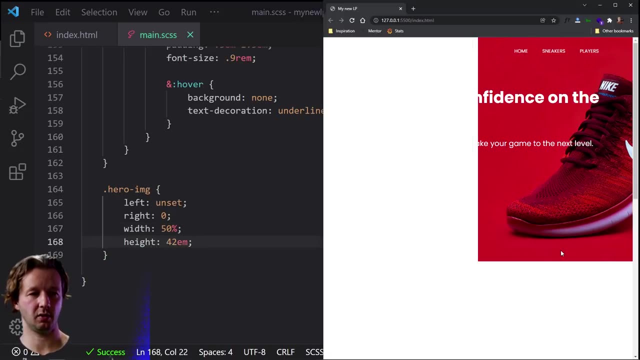 50 percent, all right. so let's hide this for a second. so we're getting close and we'll also give it an explicit height, and I've chosen 42 M units, so we're kind of just kind of writing it in. it's no longer going to be based on the height of the browser, all right, so that's looking pretty. 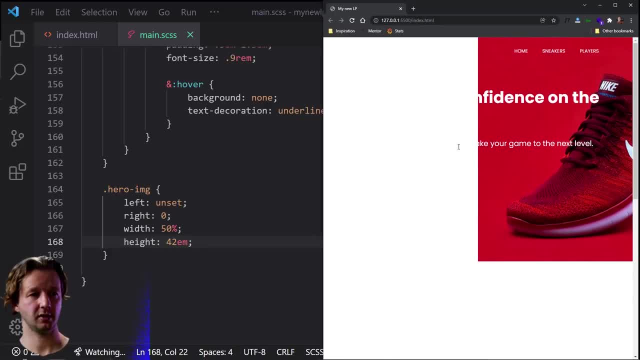 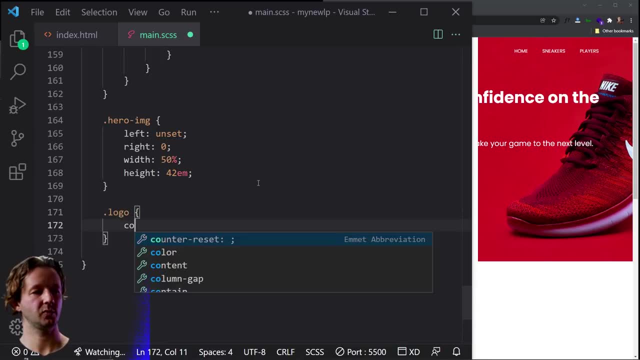 good to me for now, all right. next up is our logo. we lost it because it's white and it's currently white on white, so we're going to say logo color black. there it is, and remember we wanted to make brand red, so we can just put span because we use that span element and we'll say color red. so there's multiple ways. 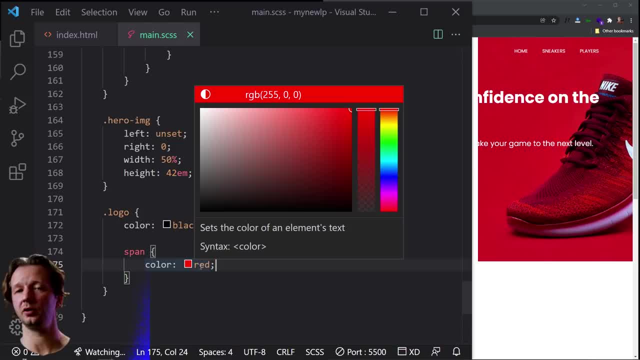 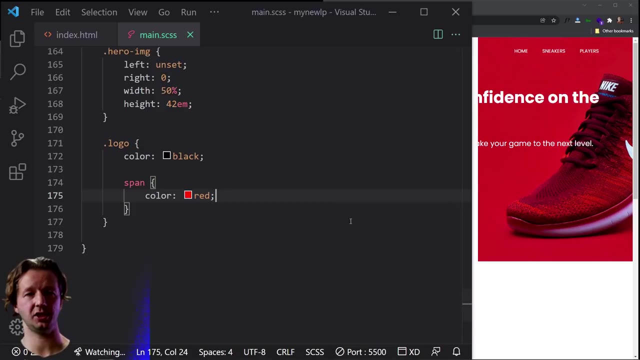 by the way, to specify the value of color, you can put red, white, blue and all these different colors. so I put in hex values with a hashtag. you can do RGB, you can do HSL. there's a lot of different ways, just so you know. all right, after that we're going to take our hero section and make all this stuff. 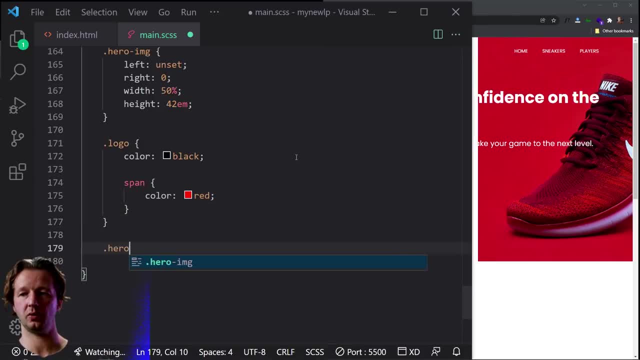 black text. so coming outside of here, we're going to do hero, we'll say color black, let's do sectionhero. that's because we specified that rule set as sectionhero above. so there was a specific specificity issue. I specify specific. okay, I'm not even going to try to say it. specificity is an. 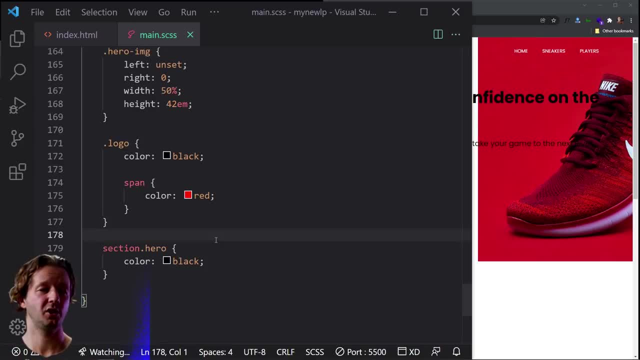 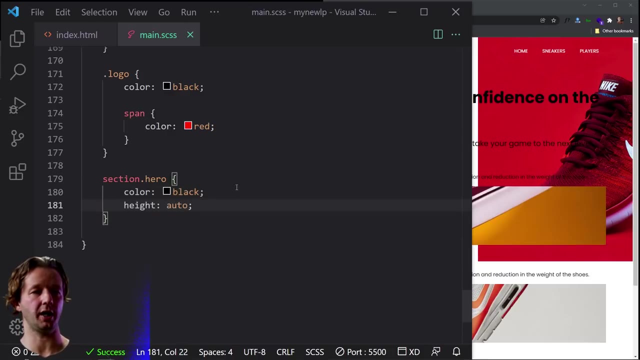 issue. I really screw people up. um, so you, I'm not even going to touch on that very much, but what we just experienced was an issue with that. uh, so, because I used section hero before and not just hero, that's why it wasn't working all right height. we're going to set this to auto and then also we're 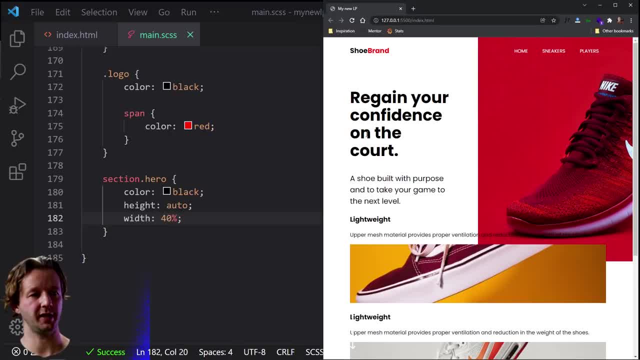 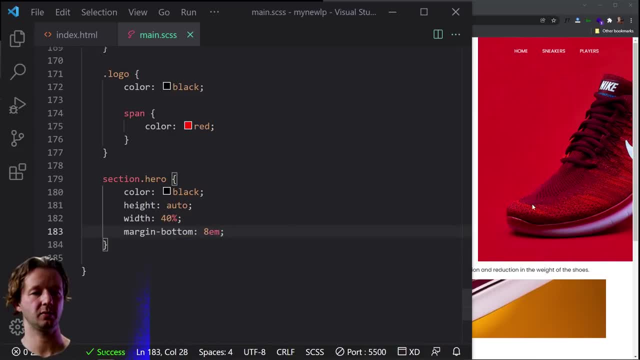 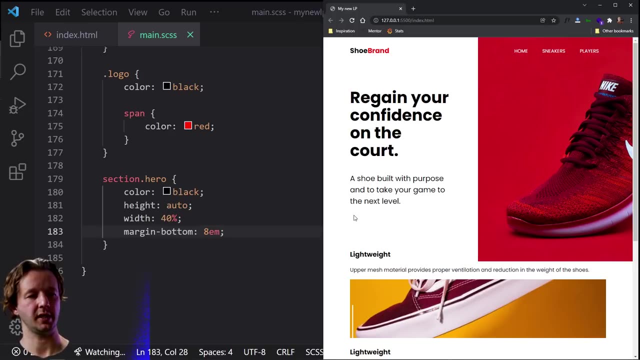 going to do a width of 40 percent just to kind of move this stuff in a little bit away from there, and then also a margin bottom to push that stuff down by 8m units. all right, next up is the we have this little um the down arrow, which is white on white, which is 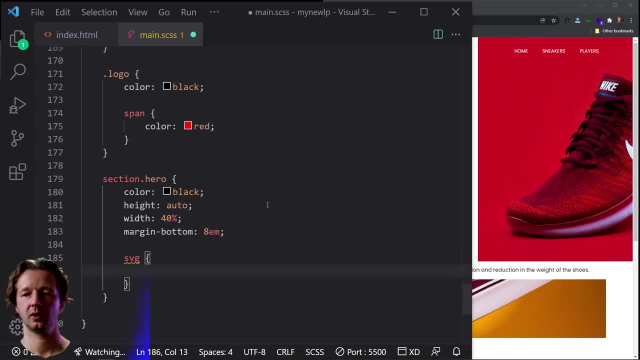 why we don't see it. so we're going to put in SVG, we're going to take, we're going to make stroke black this time instead of white. we're going to put position unset as well, because there was a position set there and then also also the path fill is black, so let's save that. 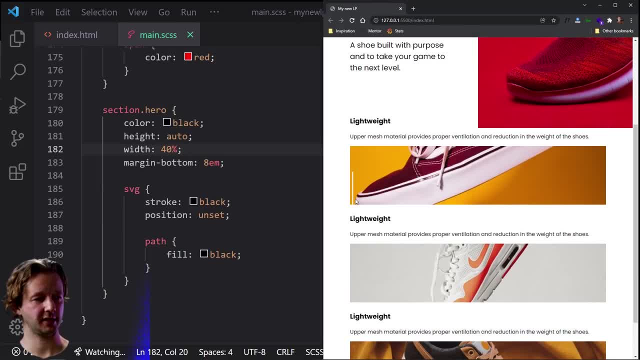 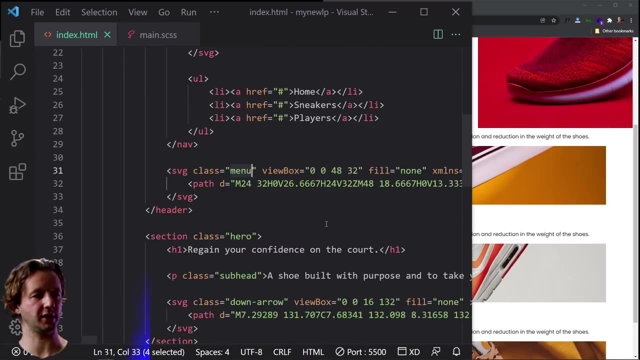 ah, and we don't see it still. why is that? all right? so that's a little bit strange because it's not aligning up with my reference code. so again, I'm not. I'm going to work through this just so you can show. this is inevitably, it's going to happen to you, a hundred percent of the time, even. if you've been doing this for 20 years. so I'm going to show you that it's going to happen to you 100 percent of the time, even if you've been doing this for 20 years, even if you've been doing this for 20 years, for 20 years. 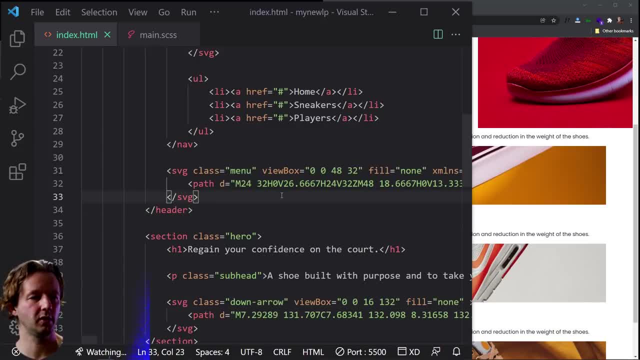 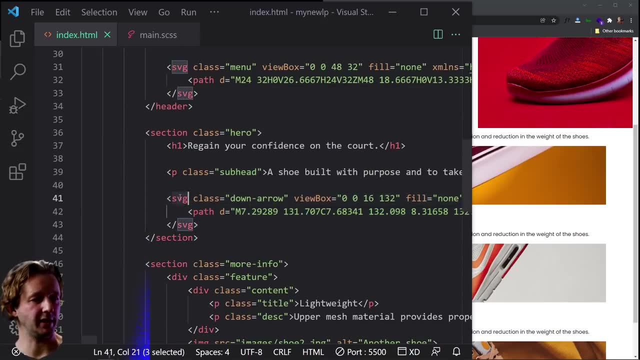 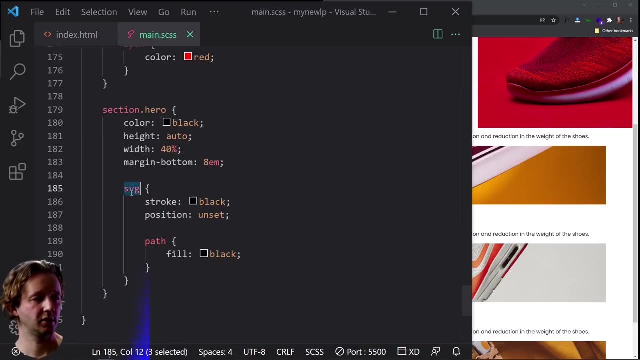 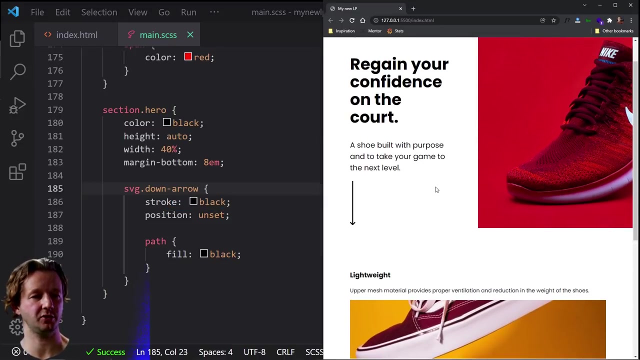 years. It's very rare to get something that goes smooth. So where is our down arrow? It is okay, so it's down arrow, it's SVG, it's in section class hero and it's not being overwritten. So SVGdown-arrow, there we go. So that was again one of those issues with being specific. 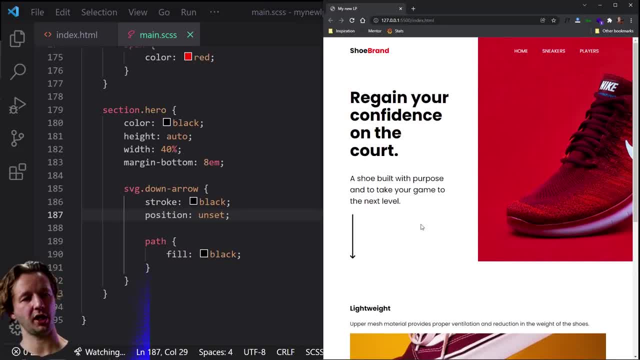 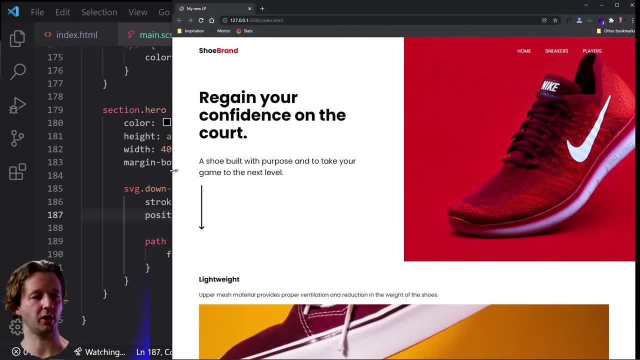 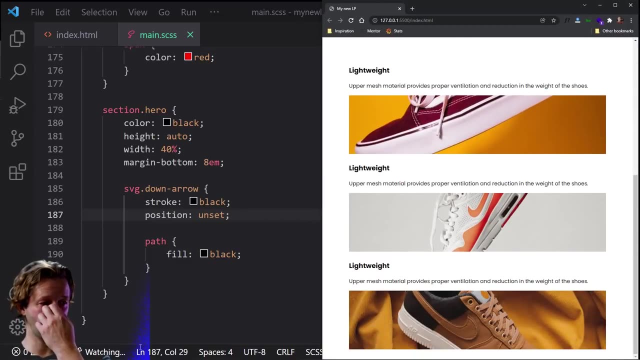 I'm going to try to say the name. There we go. Now that's working and everything's looking a lot better. Awesome, awesome, awesome, Okay. So now what we're going to do is we're going to style this area, and this is where we're going to put each one of those in two columns. So if we go, 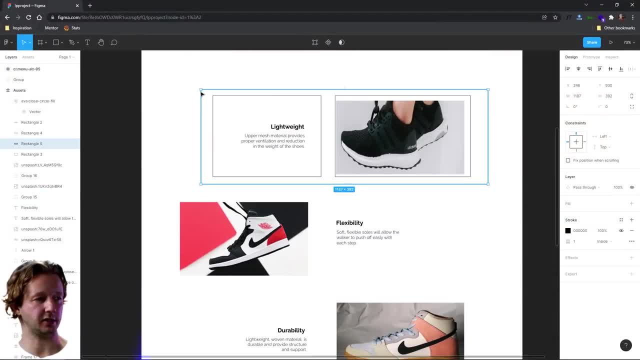 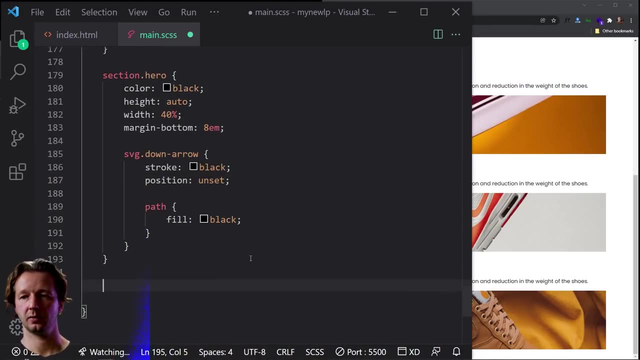 back to our reference design. we'll see each one has its own parent. We'll make that a display grid and these will be a column, and this will be a column, And then we'll use the grid to flip and reverse these. So, next up, what we'll do is we put in feature, which again is the parent container. 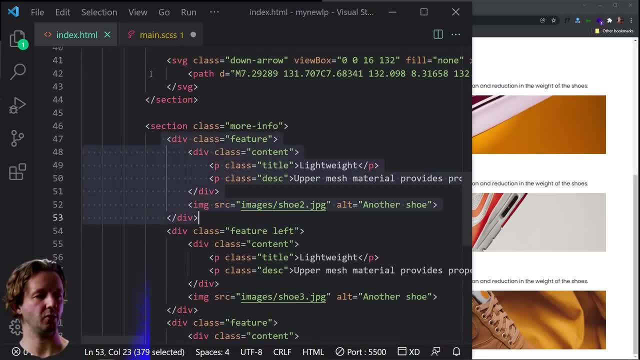 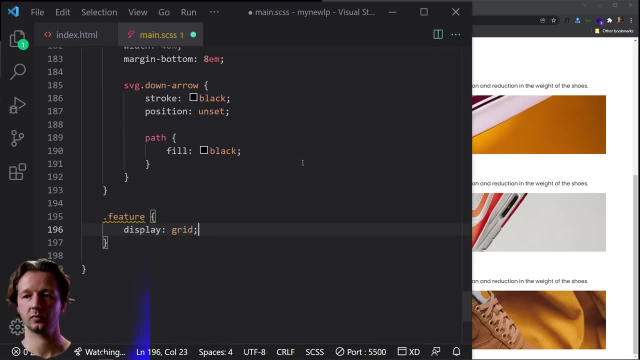 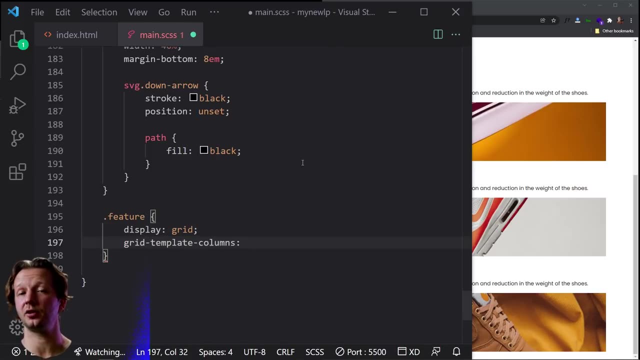 of each of these elements, Again, just to show you feature right there. So we're going to make it a display grid And then what we'll do is grid template columns, tire video and crash courses on the grid. I've done several of them. actually We're going to put repeat. 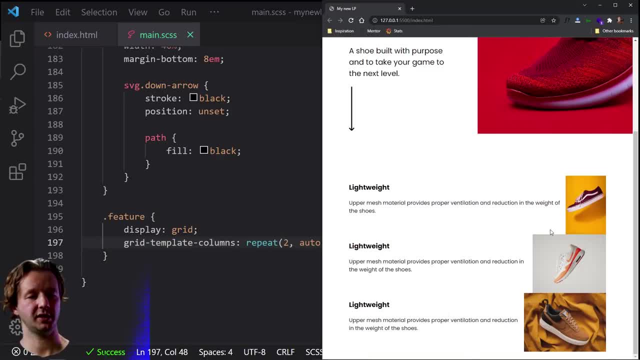 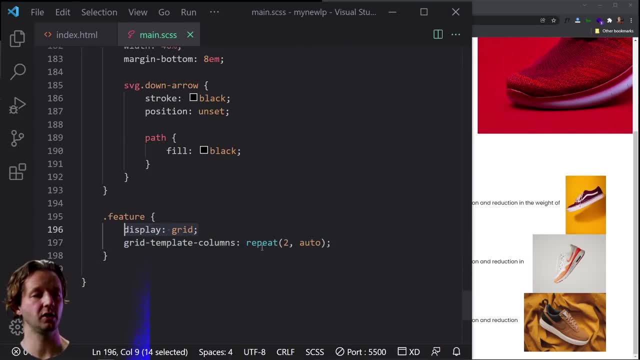 to auto. All this is saying is essentially that the grid template columns only works if you have this as a display grid, as the parent container, And then what we'll say is: we're going to use this repeat function. It says simply, just to repeat each of these columns with these values. 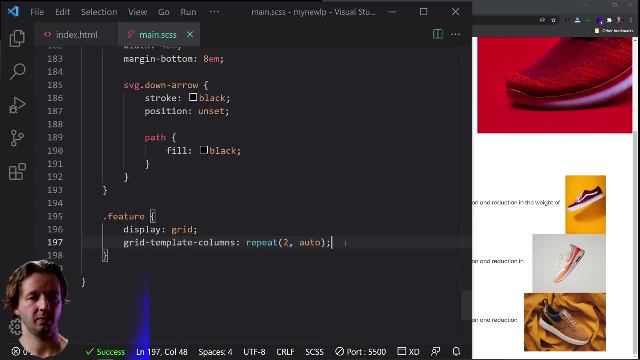 We want two of them and they're going to be situated as auto, All right. Next up we're going to say width: 25 units between them. You can see how it just basically puts white space between the columns themselves. And then also we'll put a margin bottom of 8M units to push. 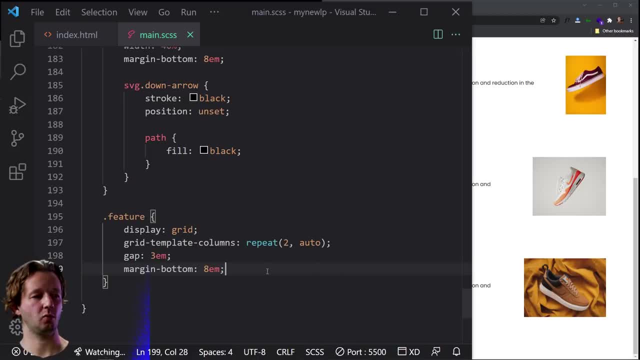 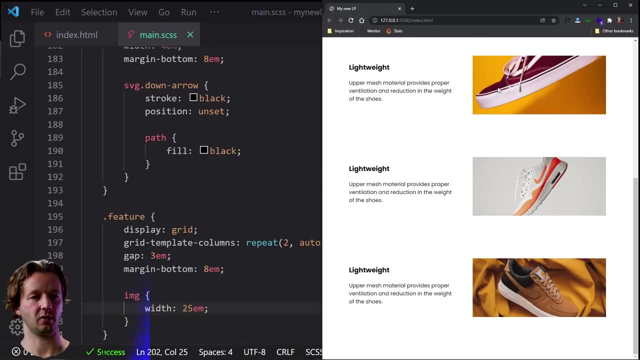 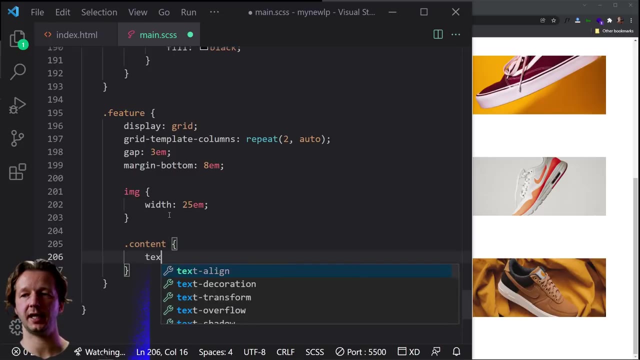 them away from each other. Now, next up, we have our image inside of them. those shoes, We're going to say width, 25 M units. So now they're all the same. All right, Now we're getting close. Next up, for the content, we're going to say: text align. 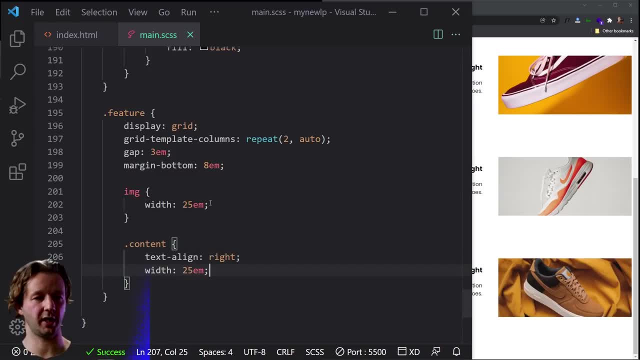 right with the width of 25 M units as well. so now they're all right aligned and this is fine. you could leave it like this, but we're going to do this flip floppy reverse thing the way we do. that is, we're gonna come outside of here. 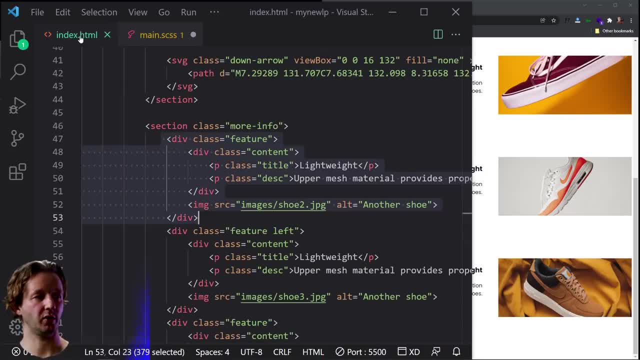 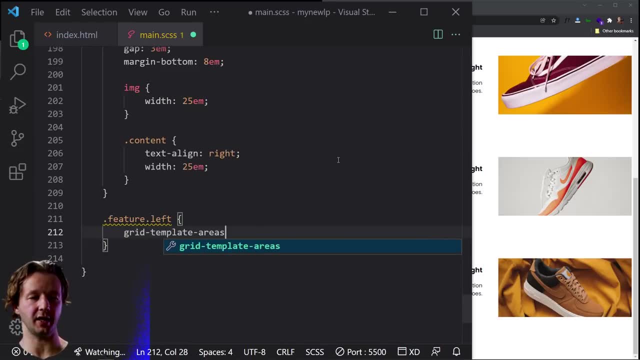 feature left, which is in relation to feature left here, and what we say is grid template areas. I know this is getting confusing, but this will all come to you eventually if you stick with it enough. we're gonna put left right, so we're basically naming our columns within the display grid, then we take our 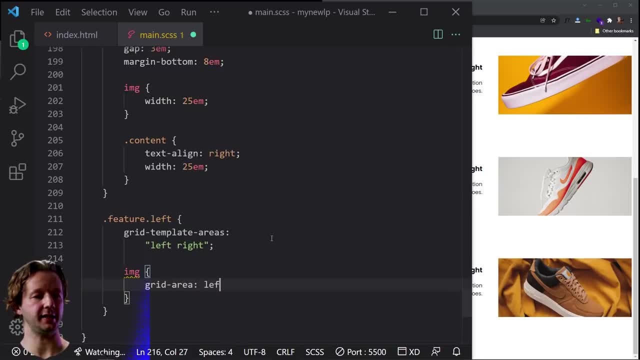 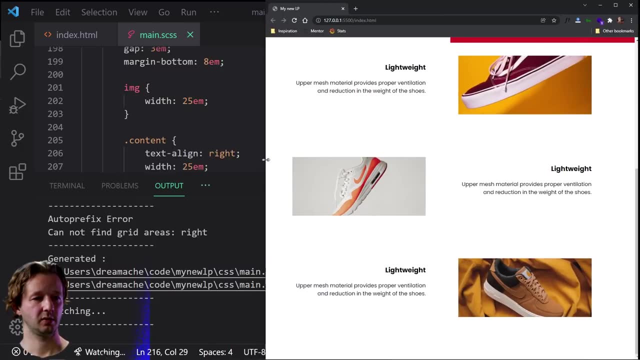 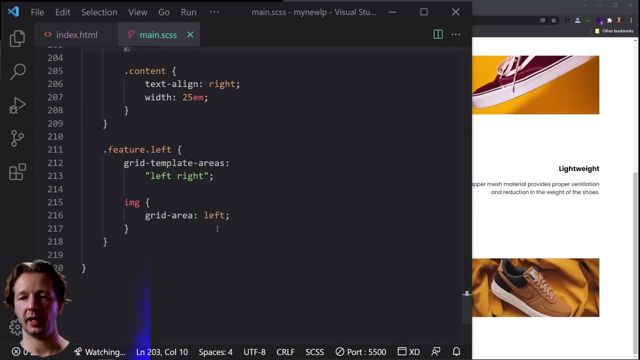 image and we say grid area is left. all right, now, it's just reverse those. now we also want to left align this type right here. so let's close this out and we're going to say the content inside of feature left- that's what that means is going to be- text align left. 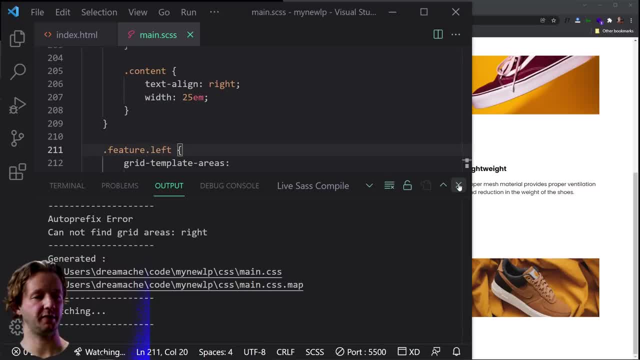 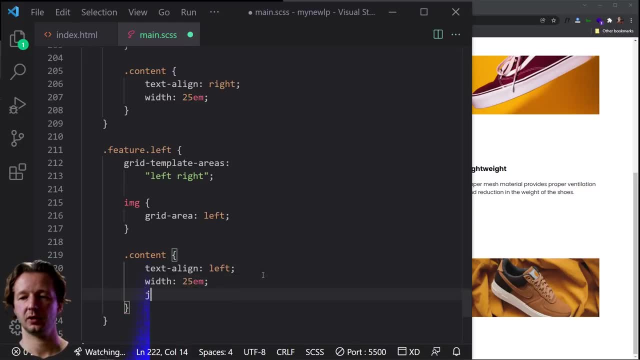 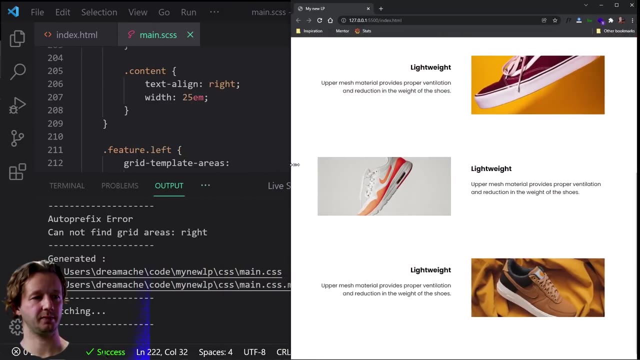 there we go, and then we're also going to give that a specific width as well. to make sure everything is evened up between all three columns, 25 M units and justify self will be left as well. so now, when we pull this up, everything is starting to look pretty good. 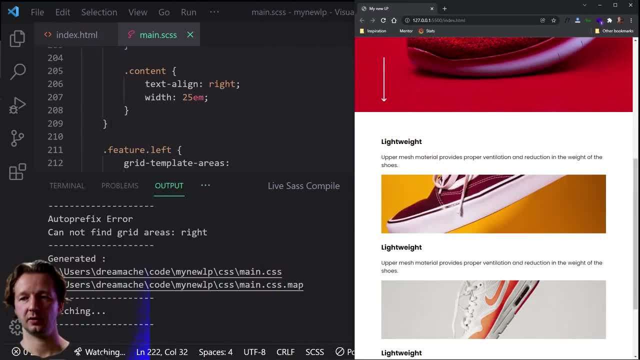 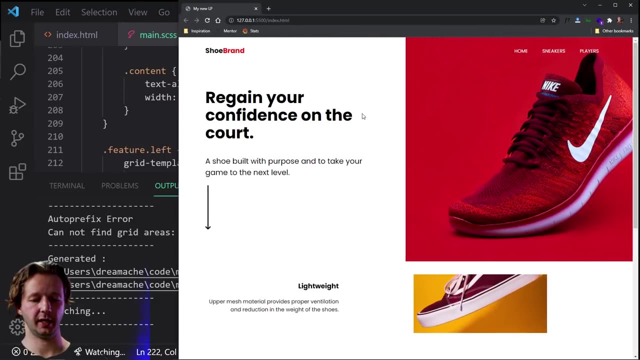 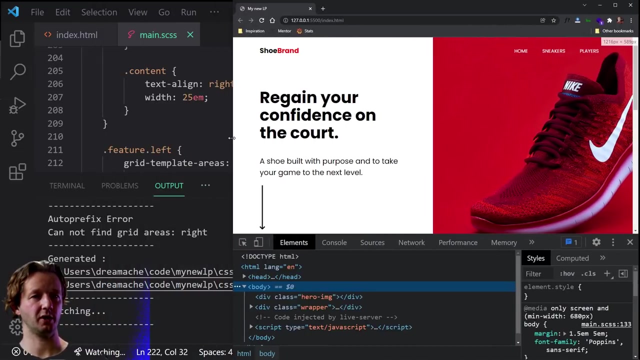 pretty decent. all right, okay. so at this point we're going to create, we're gonna make another adjustment here. so if I pull this out and I get f12 for our developer console, I think at about 1,200 pixels, I want to confine this design and make it centered. 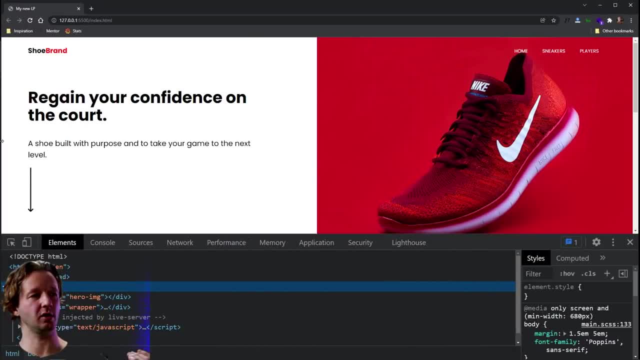 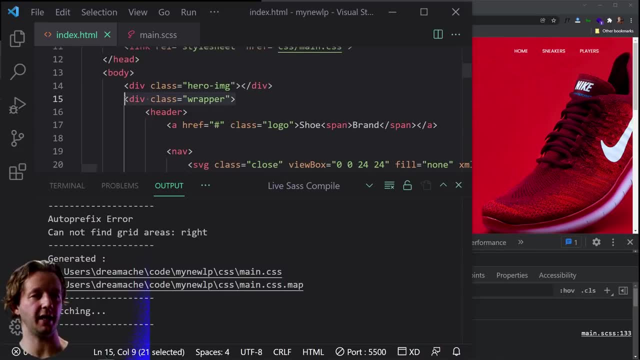 So what I mean by that? if we stretch this all the way out, I mean it is large. I don't really like the looks. So we're going to take that wrapper element which we haven't applied anything any styling to in our CSS yet. 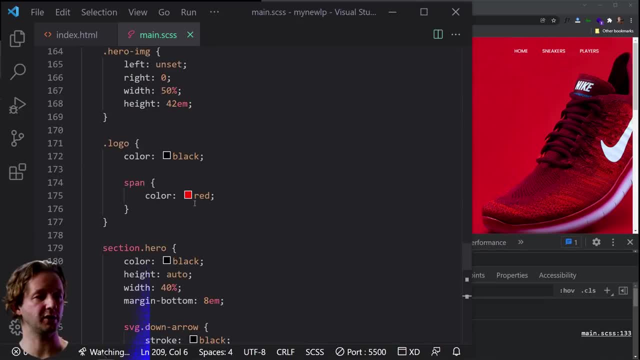 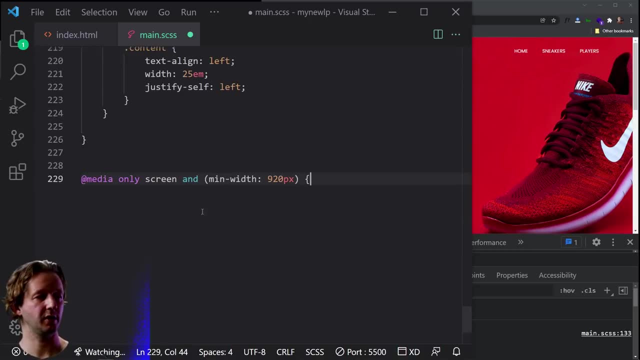 and we're going to apply it in yet a new media query. So let's go up here just to grab this code. So we're going to have a third breakpoint or a third media query, very bottom, and this is going to be for the size of 1,200 pixels. 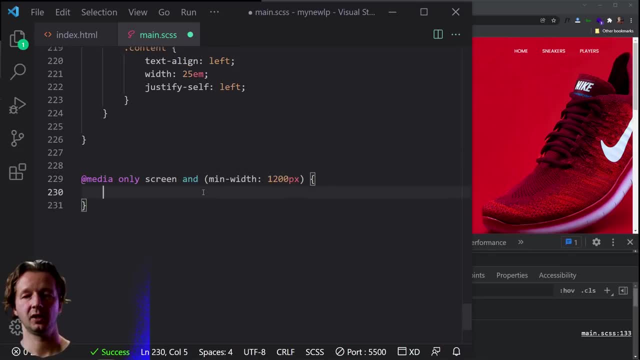 Now nothing happens because nothing's inside of it. So inside of it we're going to take a wrapper. We're going to say width is 1,200 pixels, so we're giving it an actual defined width and a margin of zero auto, which is a very quick way of centering elements. 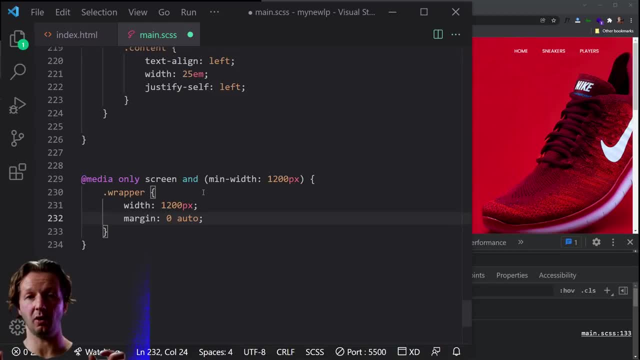 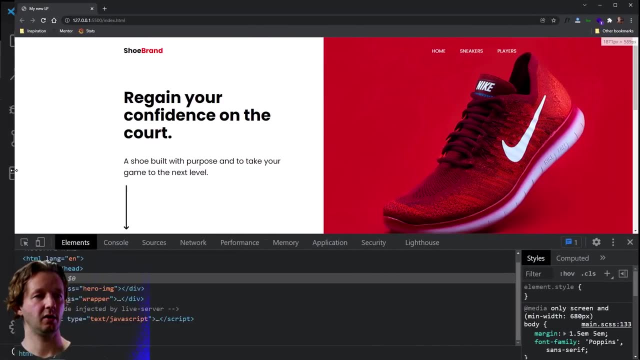 So you put margin zero at the top and bottom, left and right. You put auto and that just keeps it centered. So watch what happens now. So when we go beyond 1,200, look how this whole thing is stained. It's no longer resizing based on. it's no longer fluid based on the size of the browser. 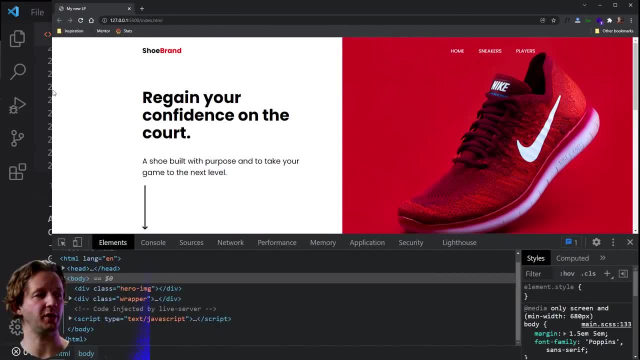 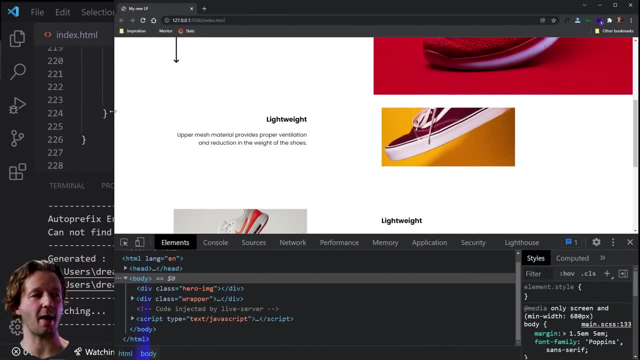 That way the layout just doesn't get too disconjointed, so to speak. Now also, I'm going to go ahead and change. look at all this white space here. That's because of the gap property. So what we can do is just say: feature gap zero. 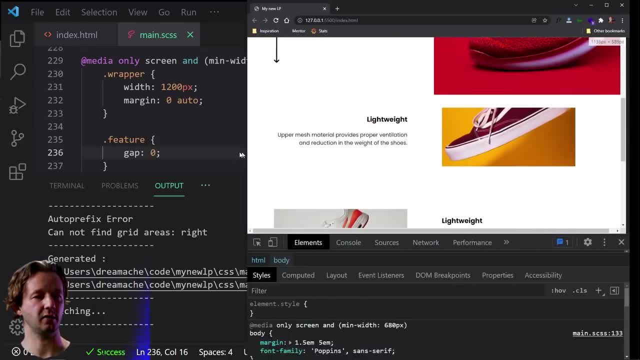 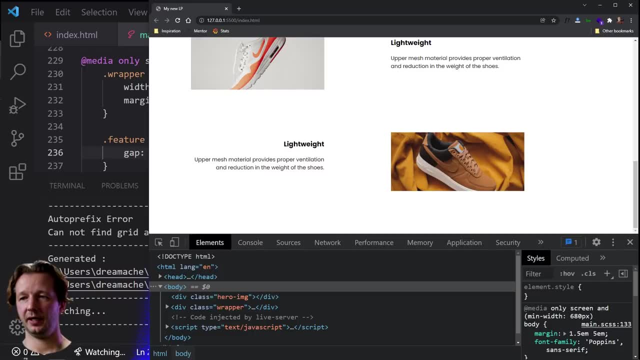 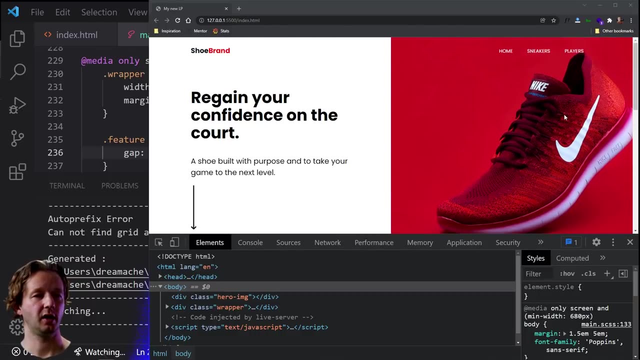 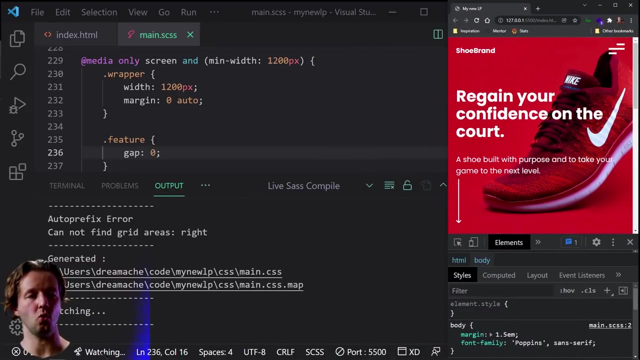 So now that just kind of brings them in closer together. All right, awesome, awesome stuff. Next up is the next section of this video. Now we're going to apply some animation to our design here, All right. so let's say, for instance, we want our image to animate in somehow. 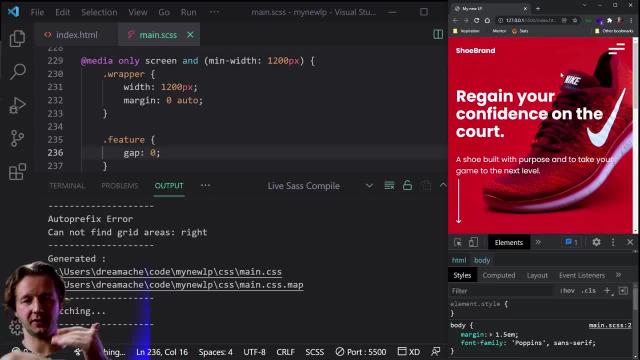 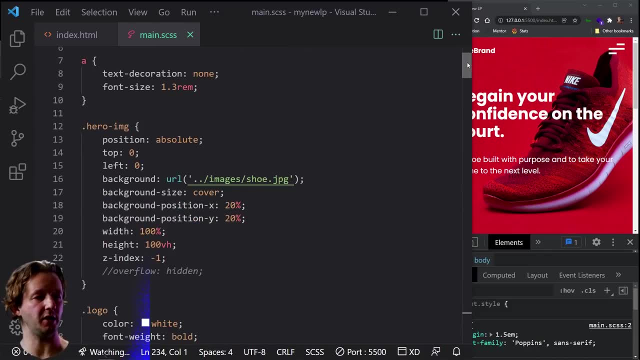 Maybe we want it to kind of just like fall down and like kind of just give us a cool sort of animation. So what we're going to do is we're going to visit our hero image all the way up here, outside of the media queries. 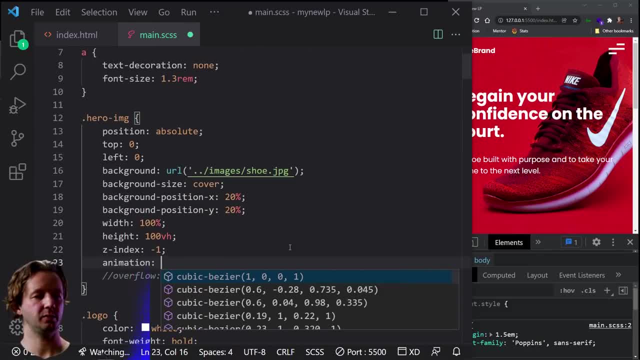 And we are going to add animation And we'll say intro load, So that's the name of the animation. We want it to be for two seconds long And we'll say forwards, because we only want it to run once, We don't want it to repeat. 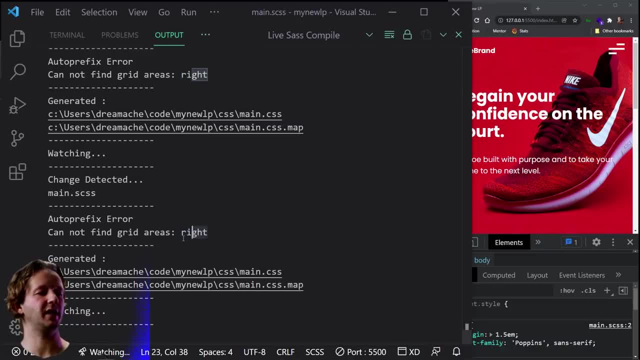 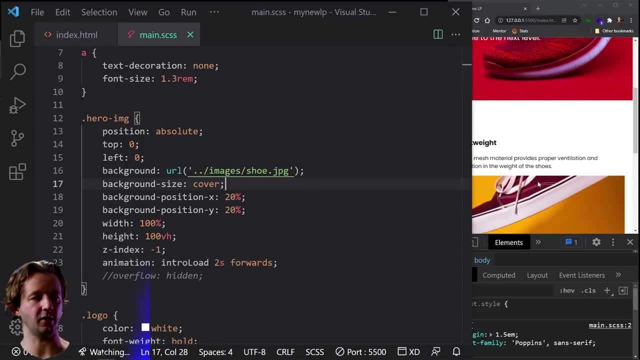 Oh, there's something. Oh, okay, It's because I never defined the, The grid area named for right. I was wondering why that kept popping up. You don't have to worry about that, though. All right, so we have an animation called intro load. 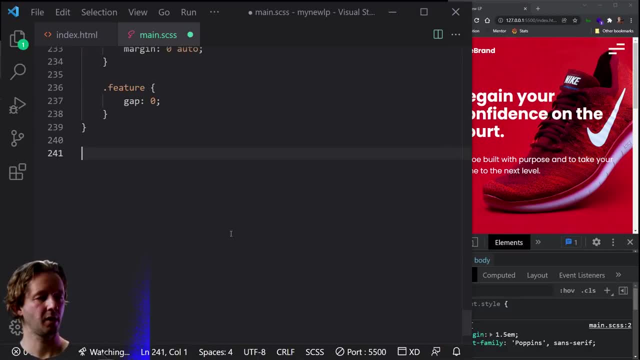 Now let's go define that animation way at the bottom, The way you define a keyframe animation you put at keyframes and the name in our case is intro load And we open it up like a regular rule set. So that rule set, what we'll do is we're going to say from: 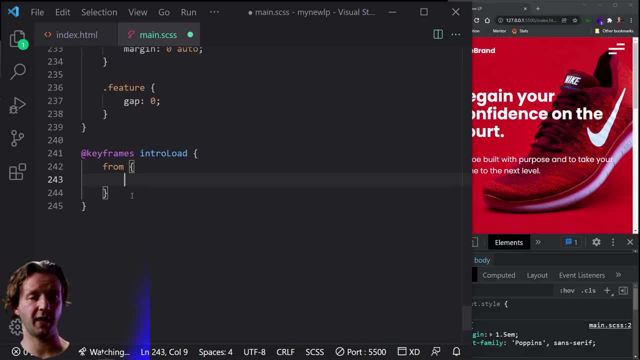 And there's multiple, There's multiple ways to put in these little keyframe rule sets. You can put percentage values So you can have multi-step animation, like maybe from zero to 10% it's going to do something, And then from 10% to 50% it'll do something, so on and so forth. 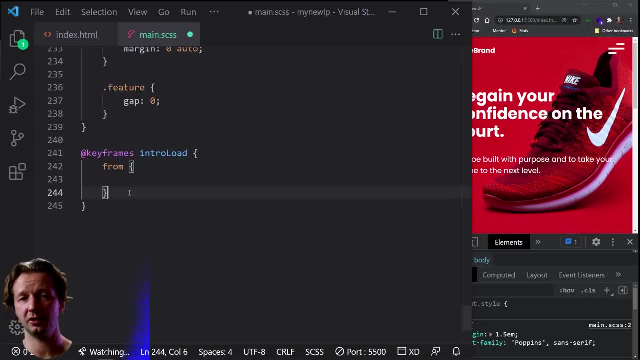 But if you just want a simple from and to, you can either use transition or you could use a keyframes as well. So we're going to say from clip path. Now, this is another property you've never messed with before, but there's a very cool tool called Clippy. 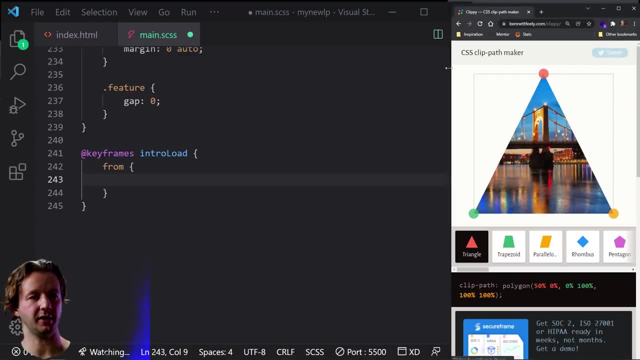 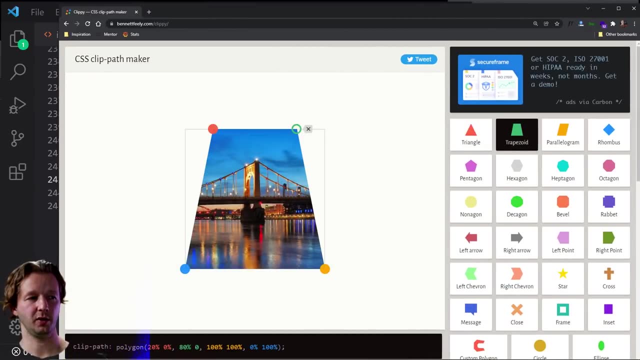 CSS Clippy. Just type that in Google and you'll find this result right here. I've shown it a lot on my channel, So we're going to choose trapezoid, which is just a square or rectangle. Let's move things out. 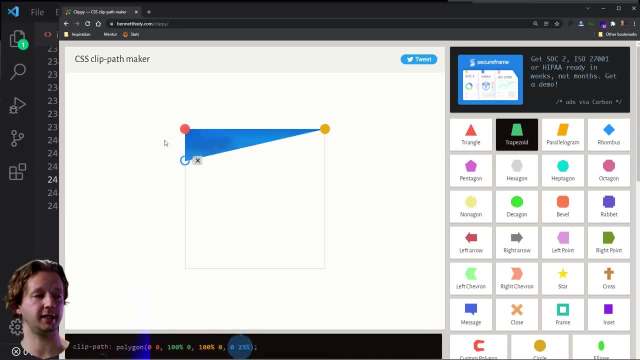 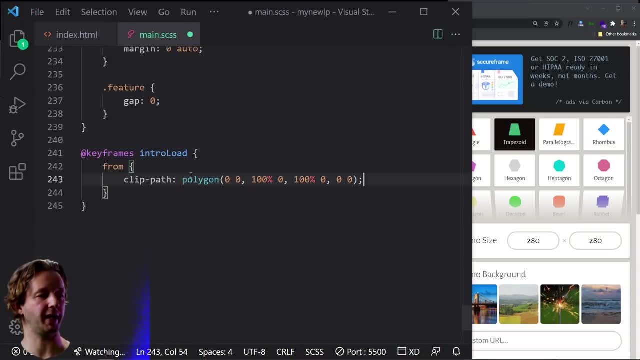 And our starting point for our image is going to be way up here. You're not going to see it, So we're going to copy this declaration right here and we're going to go back here and we're going to paste it in. 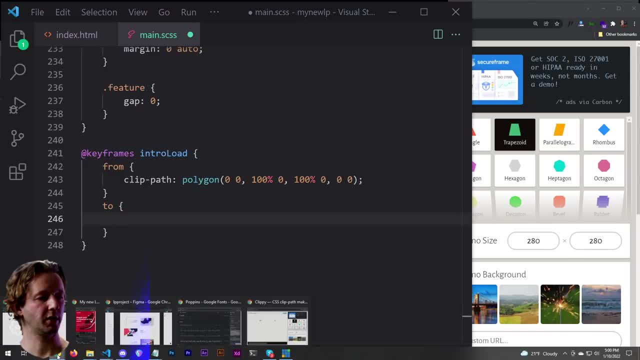 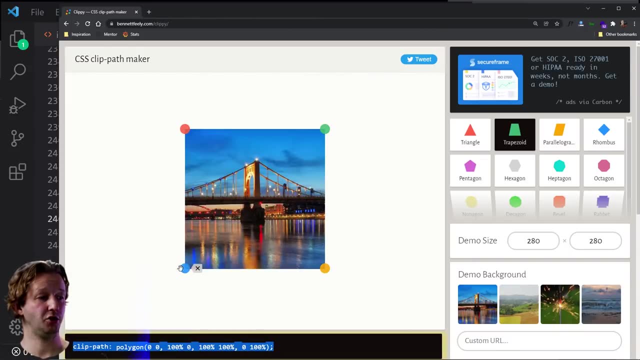 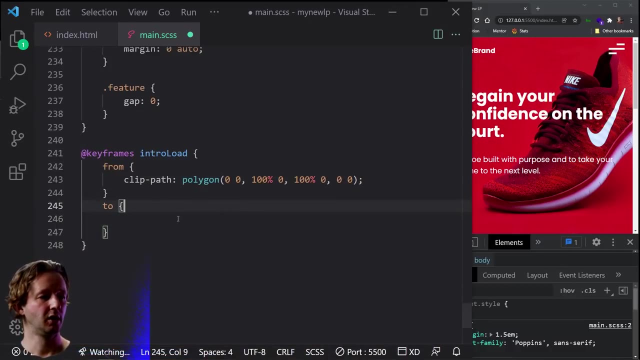 And then we're going to say to: We're going to go back to our Browser, pull these back down. we'll copy that. you could make it, make it interesting, maybe just do something like that or that or whatever. you can do a ton of stuff. as you can see, we're going to paste that in right there. 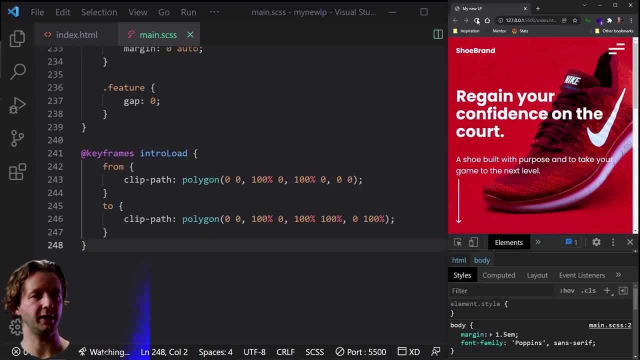 Look at that Once we save. how cool is that. That's how you can create animations on one of many ways. Now, what about this arrow right here? What if we wanted to Bob up and down, for instance, Just to kind of? 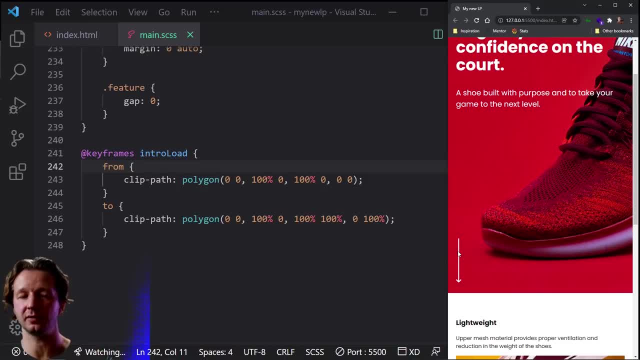 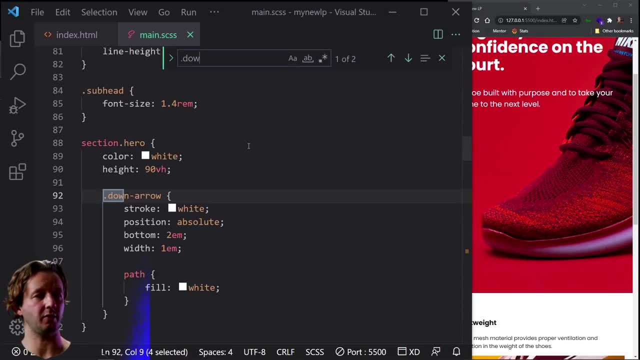 Give a like the eye like to, to bring it attention All right to the eye. So what we can do is- I will find this is called down arrow control F, By the way- if you have a big document, You just type it in and you can find it pretty quickly. 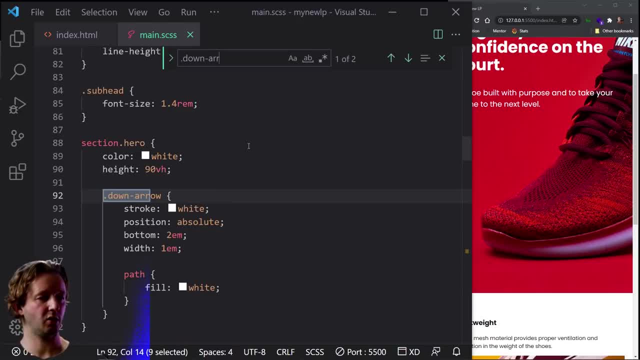 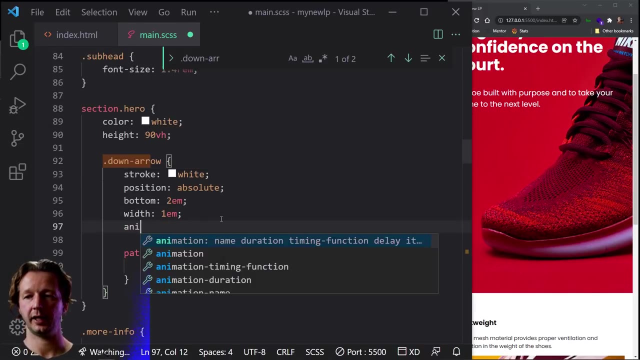 Down arrow, down arrow. here, That's in a media query. This one is not. So I'm going to do the same thing in my reference code And we're going to add another animation. So what we'll do is say: animation, move, arrow, one second, alternate, reverse. 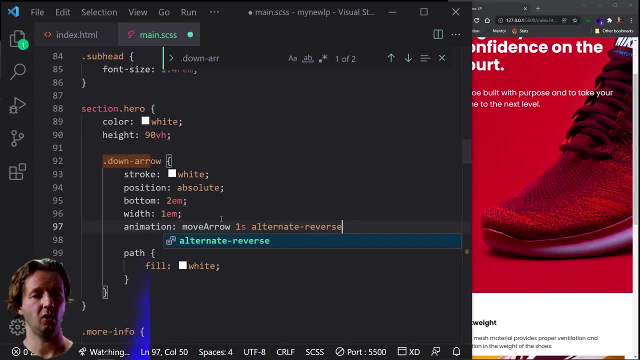 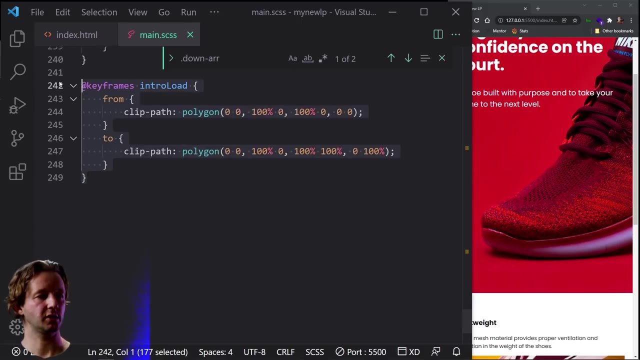 So that's, instead of putting forwards or infinite alternate, reverse. We're going to go back and forth between the two states and then we also want it to be infinite. It will just loop on forever and ever. so move arrow, let's come down. let's copy this, just so we can save ourselves some typing. 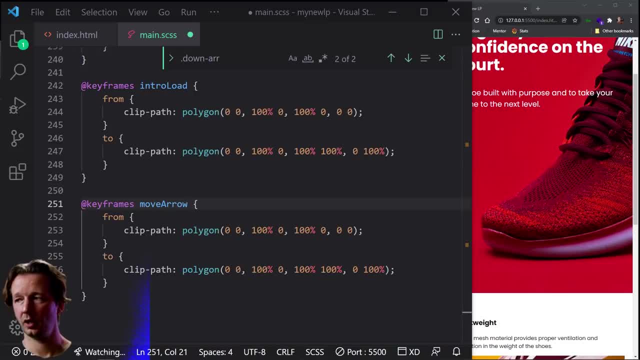 Move arrow And then, inside of their Same from and to, we can just do transform, translate. why negative 30 pixels? We're going to move it up 30 pixels and then we'll copy this And then just put zero, Save it. 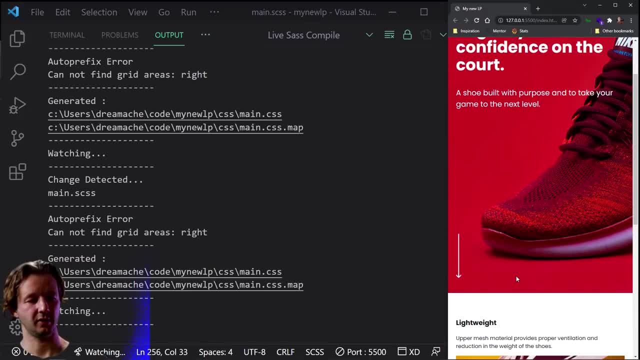 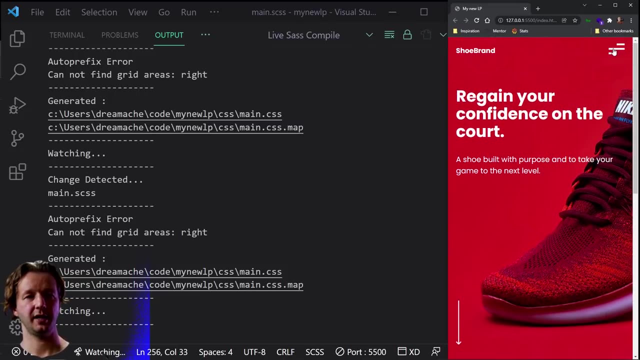 And look at that, It's bobbing up and down All nicely. so if you change the duration stuff and go really fast or really slow, all right, very, very, very cool, all right. also, we also want to get our navigation working. I believe, before we get to that point, let's make this stuff fall in and like fade in, all right. so what we'll do in order to do that is we're going to create another animation called 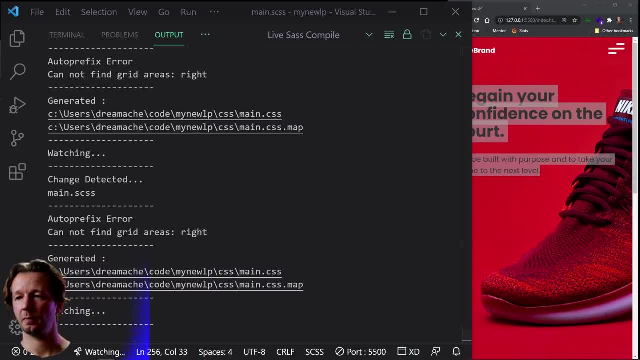 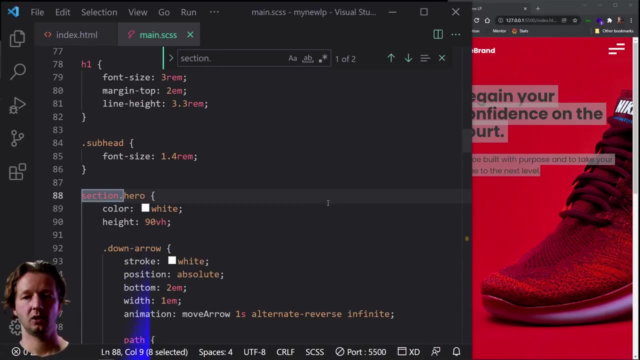 We're going to create another animation called Move arrow, Not not move arrow, I'm sorry, it's called I Move down, rather, so I'm going to search for that on my reference code. so on section hero, There we go. we're going to put in animation. 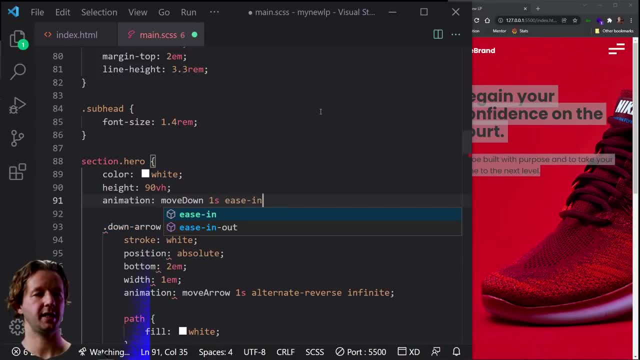 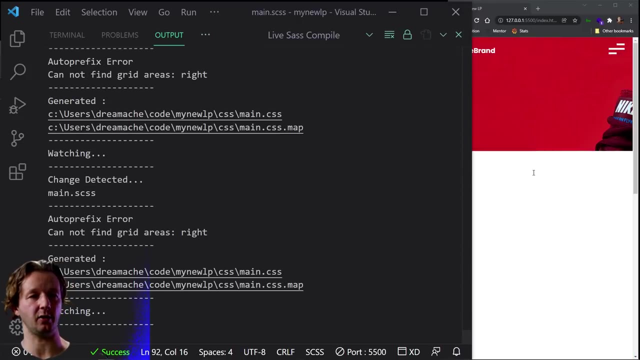 Move down One second ease in and out, so you can create custom easings which affect the flow of the actual Design Or the the animation rather, and then forwards. we only want that to happen once. and then let's also change the opacity zero. it's going to hide it right now. we're not going to see it anymore. opacity is how you can just hide things. 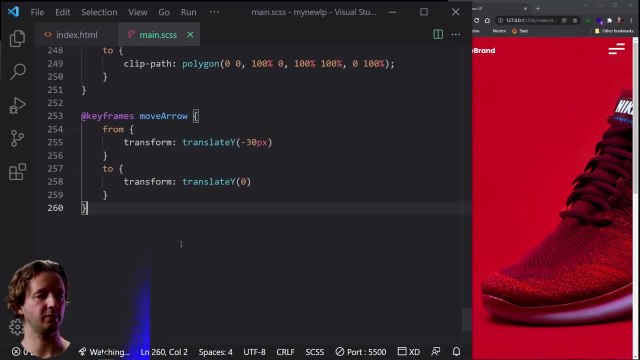 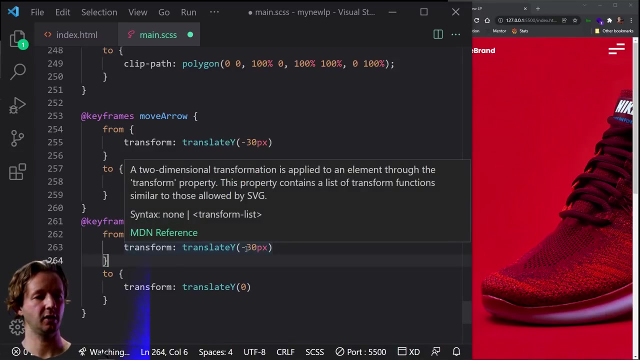 So then we come all the way down, We create, move down And then and move down. what we'll do is simply say, Translate, I Are transformed, Translate, translate why. And then we'll leave it at zero here. And then opacity: one member, we hit it. so now we're going to bring back the oops. we have an issue. 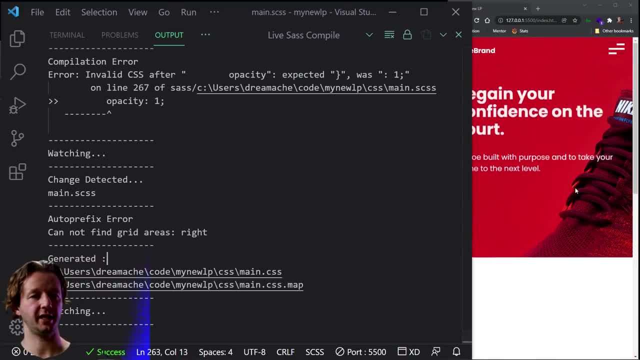 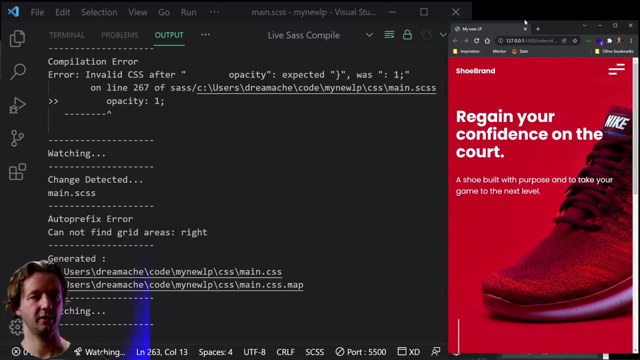 Make sure you have your semi colon there if you have more than one declaration, so we'll save it and look at that Now isn't that very cool? so let's get this up here. Put this up here Now. it's also cool is, if I bring this out, if I refresh. 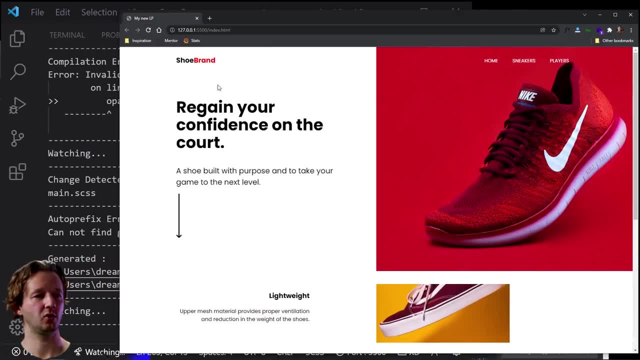 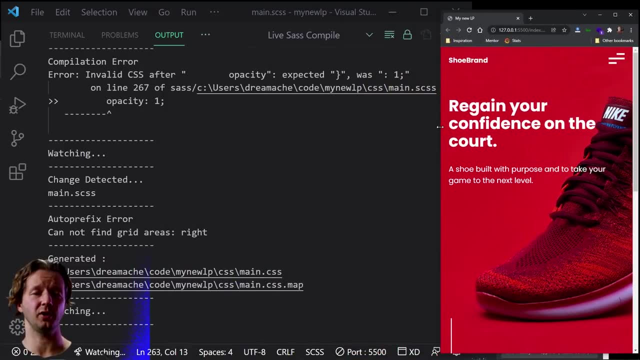 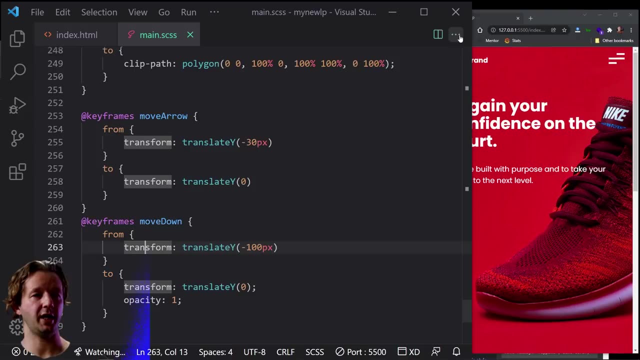 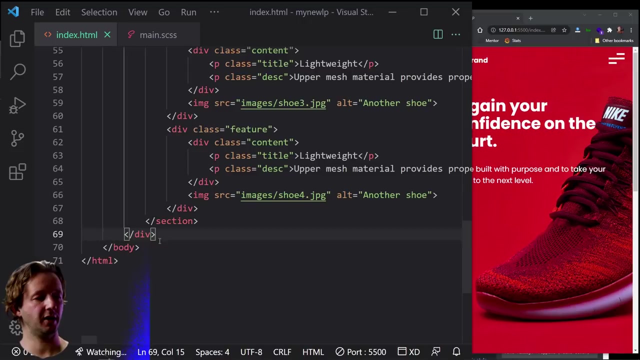 It still works on desktop as well. How cool is that? It's very cool. The final thing we need to do is some javascript And we'll do a little bit of animation to get that thing to slide in. so we click this, nothing happens. so this is how we create. interactivity is with javascript. now, this isn't a javascript crash course, but we still have to write some of it. so, at the very just, typically, if you're going to do what's called inline javascript, which means writing javascript inside of your html file, 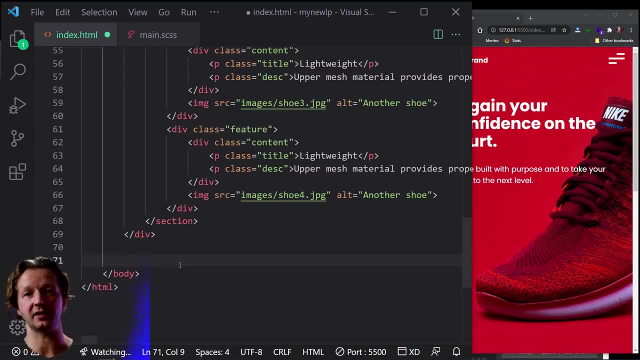 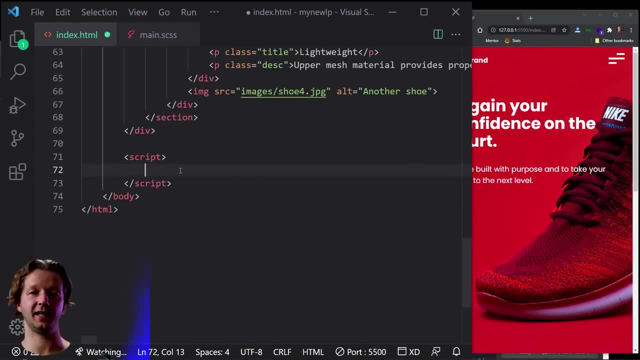 You don't have to. you can also link an extra file call a dot js file. but we're going to do here so we can type in script in there. Javascript goes in here, html, and all css does not go in there. css in javascript is a thing, but that's different. as another topic. 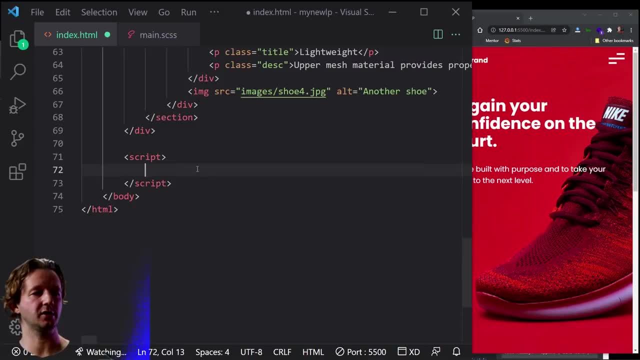 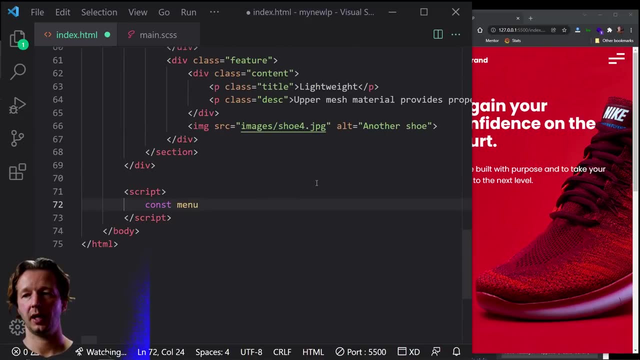 I. so what we're going to do here is just create some variables, or constants as they're called. We're going to say const menu And we're going to say document dot, query selector, And what we're trying to do is just create a reference or a variable by that will allow us to determine when this is clicked. so this has a class of menu, so we put in menu. 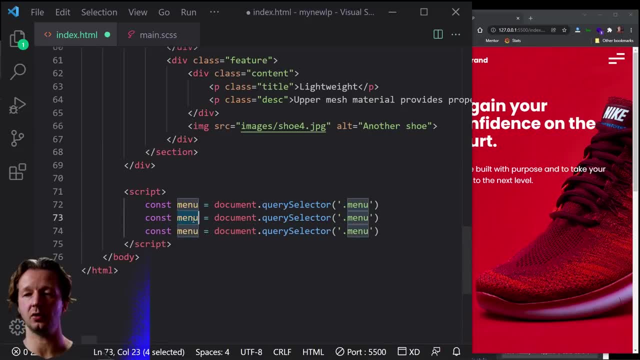 Now we're going to replicate this two more times because we also need access to the close button. so we double click that and we change that to close. and then also the nav element, which is currently hidden off that big white long I element. so we're going to change that to nav. 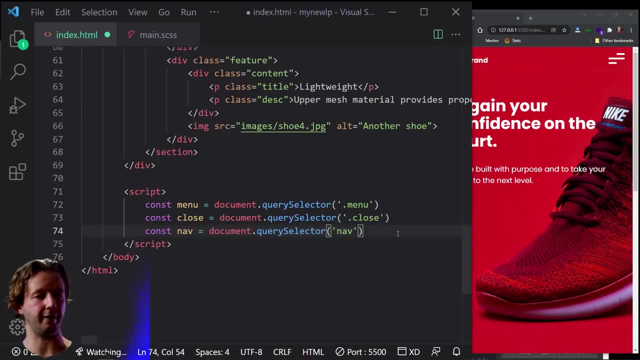 And this one is not a class, so we remove the period, just put nav. So first thing, when somebody clicks this, which is our menu, we say menu dot- add event listener. So there's a bunch of different types of events that can occur. one of them is click. so we open up in parentheses and a semi quote in the first parameter as click. 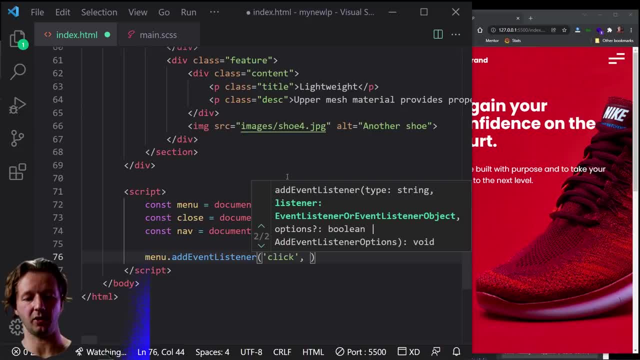 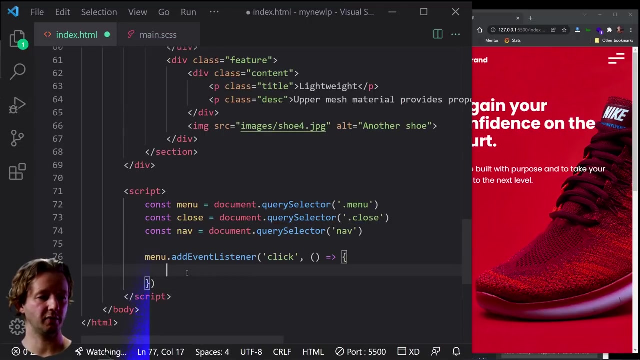 Then we put a comma which separates your parameters. we're going to put empty an argument here, we're not going to pass anything in- And then we put in what's called an arrow function and then we open that up into the squiggly brackets there and then what we say, what this essentially means, kind of like the in CSS, it's kind of like our media queries right here. this, what's ever in here only happens is, if you know, this element is clicked. so what we do is we say nav, which is defined right here, now that we have access to it, nav dot. and, by the way, we could have just done that. 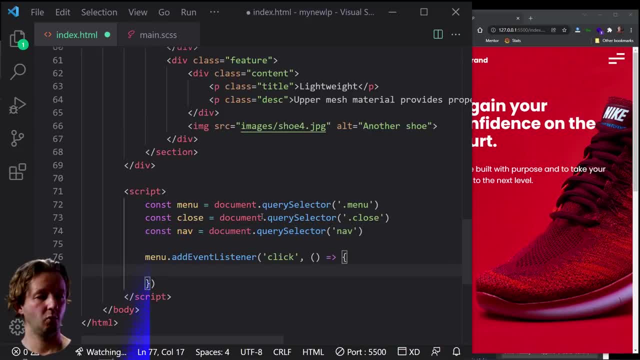 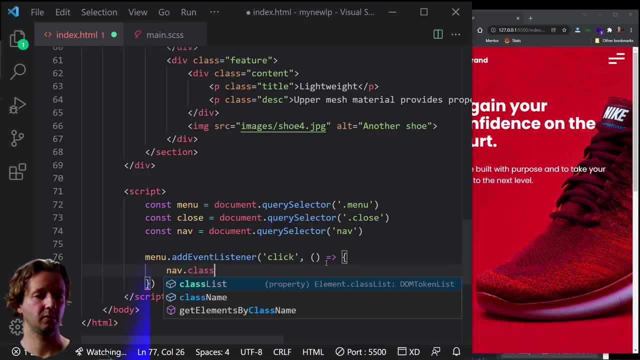 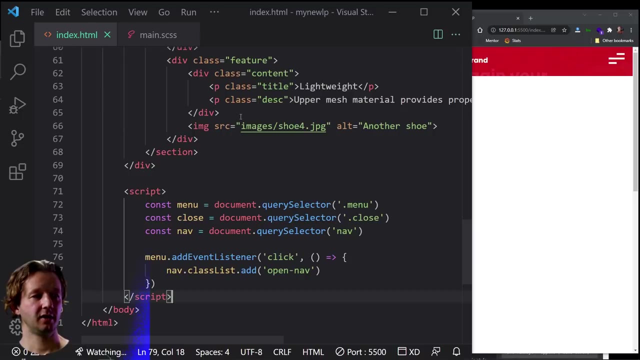 So we're going to say nav dot class, list, dot add, so we're adding a CSS class to it. when it's clicked, All right, We add A class that we have not yet created, called open hyphen nav. All right, So let's create that. 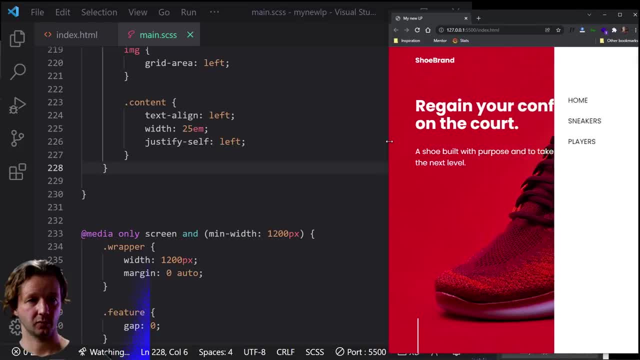 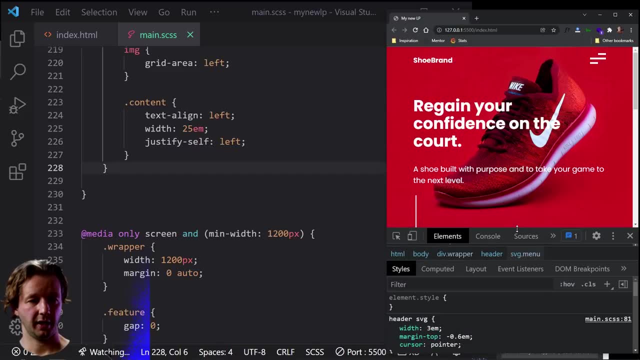 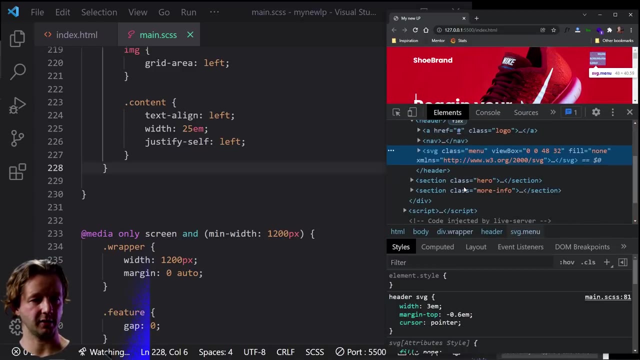 Now, if I show you real quickly with the dev tools And we get to a point where we're here and I hit F12. And I click on this And we view this. Let's, let's find our nav element. It's somewhere. 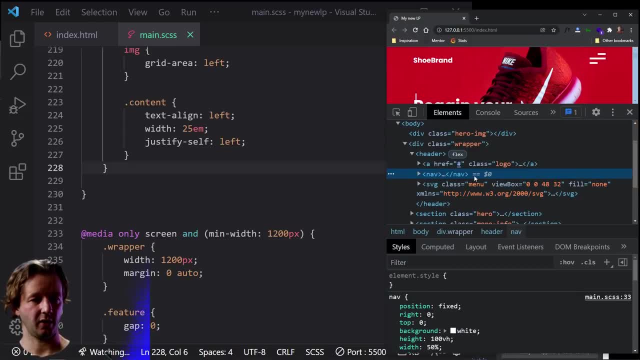 In here. It's in The header nav right there. Now, if we look And I click that, there we go. we click it. class open app has been added to it as an attribute, So that's what happens, Just to show you again. 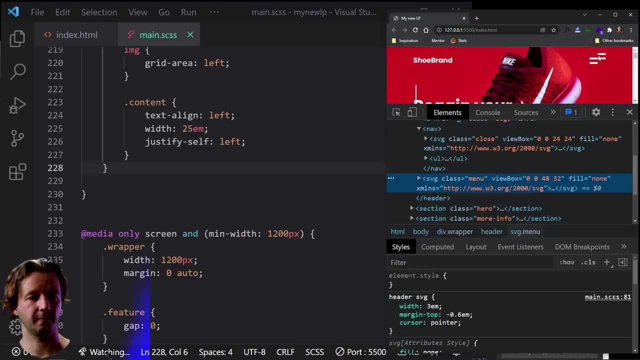 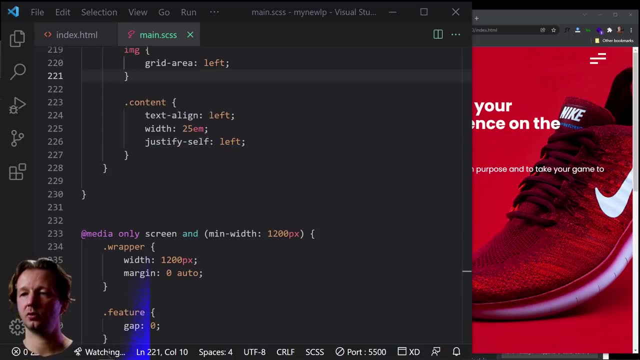 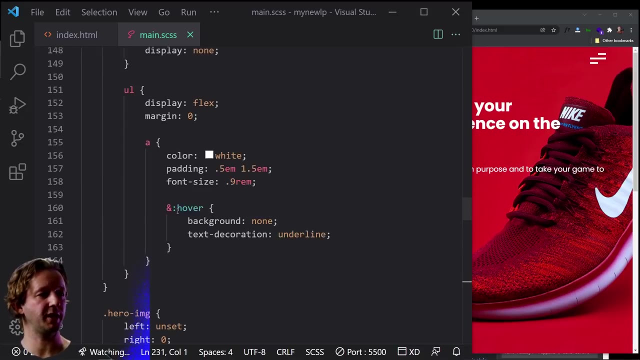 If I click this There, it goes as that, but nothing happens because it's not defined in our CSS yet. So to do that, we're going to go Back over I Right here, above our first media query, And we're going to say: 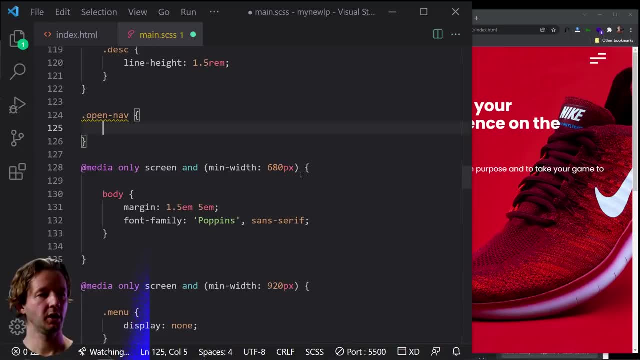 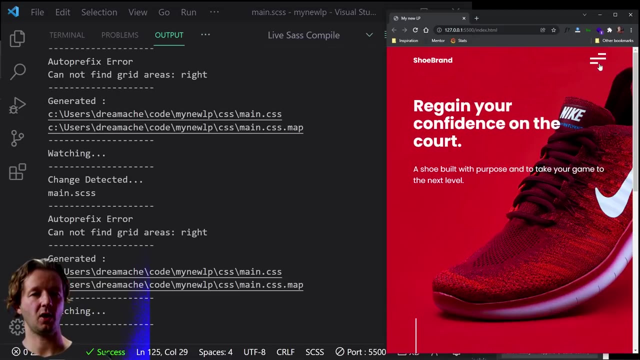 Open nav. We say: transform Translate, Oops, Not tarns late. Translate X zero. Let's put zero percent. So now watch what happens. Look At That. Refresh Tada. Now, if we could close, nothing's happening. 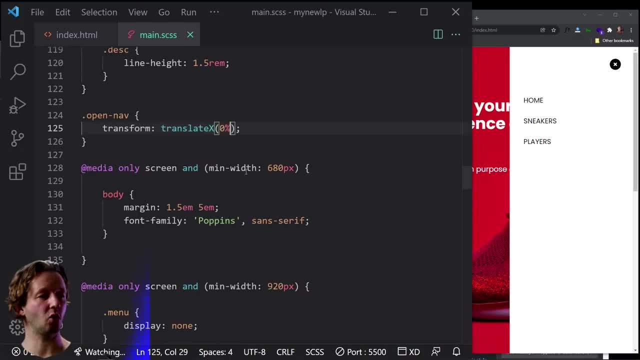 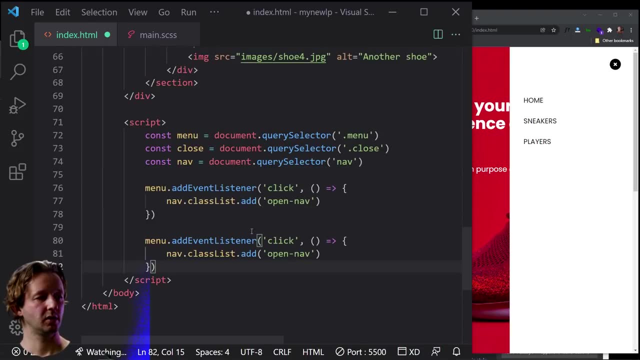 Why You guessed it. We have to go over To here. We'll copy this Now for this. This is going to be close, So we add an event listener on close, click Now we just say Remove, Click that. 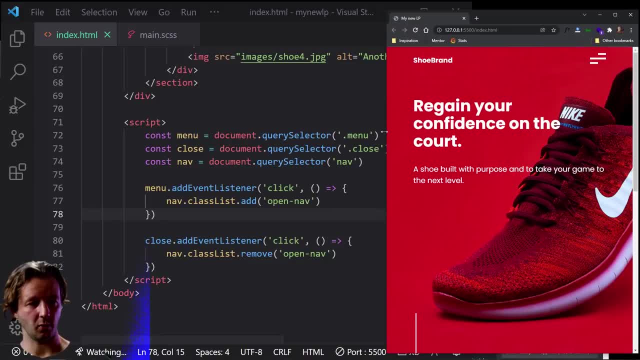 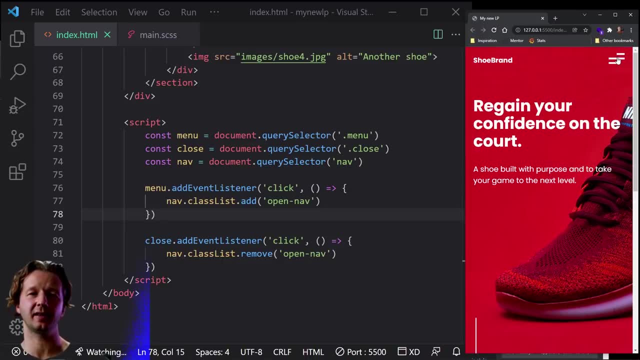 Click that. Oh my god, Look at what you just did And you know what. You probably understand it pretty well. You know what's something that's bothering me. This is looking pretty big. I don't like the look of this. 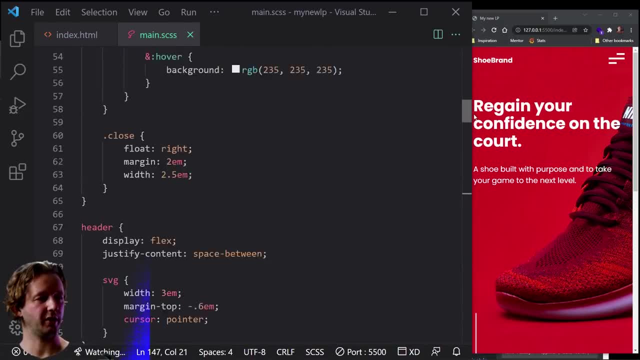 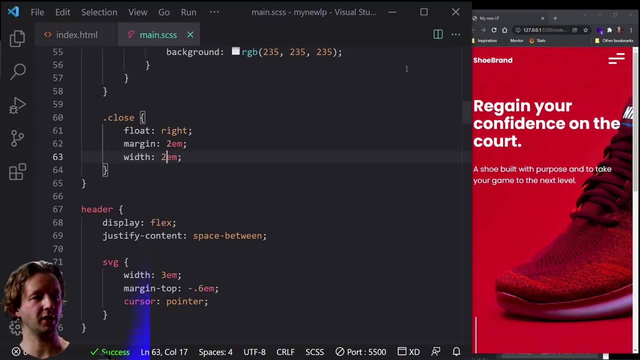 For some reason It's setting in my reference code as that, But that just does not look good. So I think that's called. close Width is 2.5.. Let's try 2.. Let's make sure. Oh, was that in a media query or not? 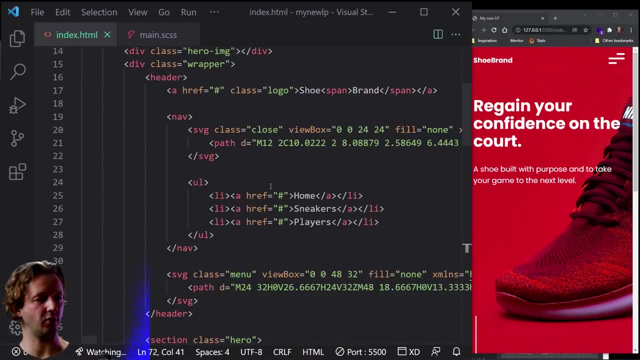 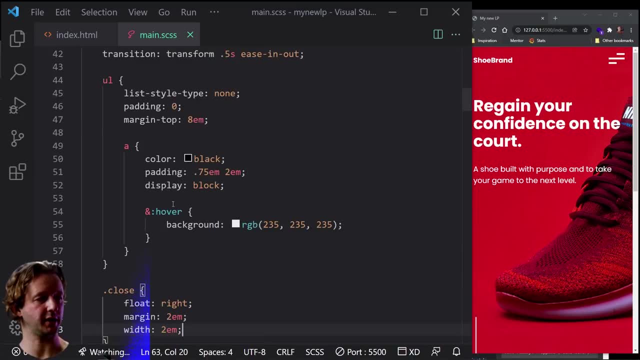 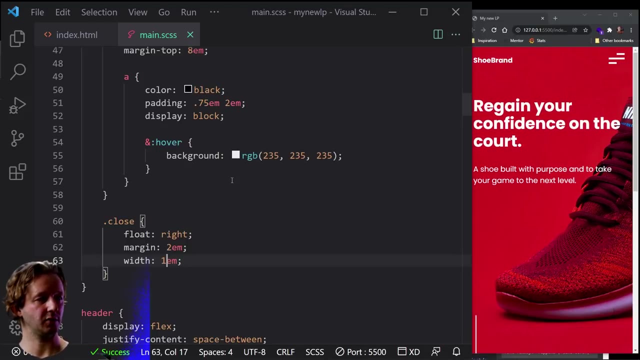 No, it wasn't. So let's go back here to our code. It's called SVG classes- close- Alright, So it is close Right here With 1M unit, So it's not changing, For some reason, The value. 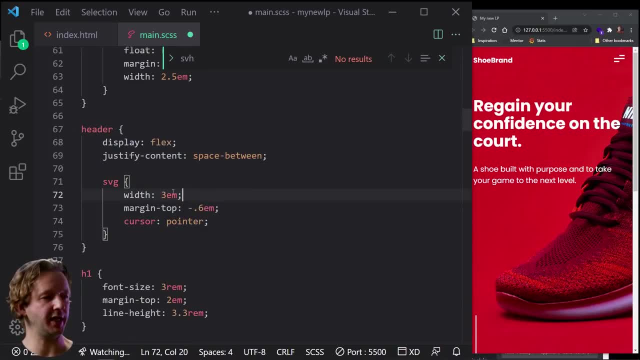 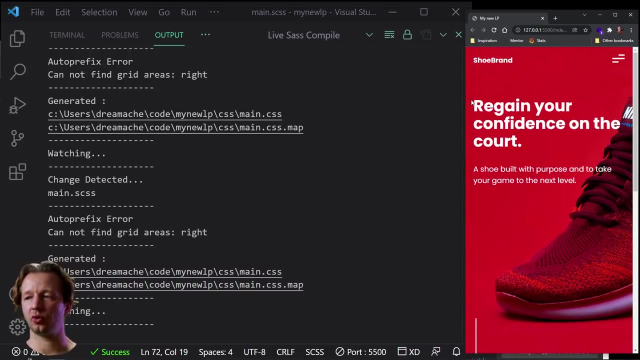 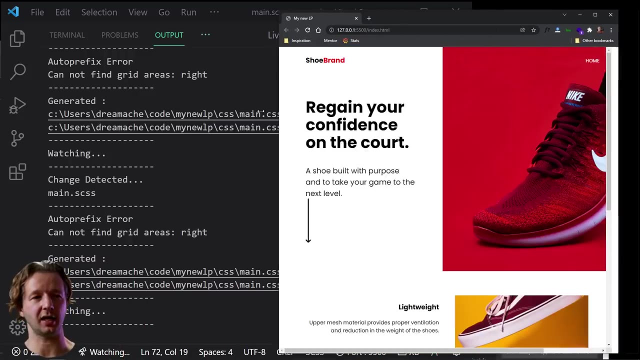 Oh, sorry about that. That is actually header SVG. It changed from 3 to like 2.3. And that's a lot better Of a size, Alrighty, So Sorry about that. There was like a blue tint thing showing up. 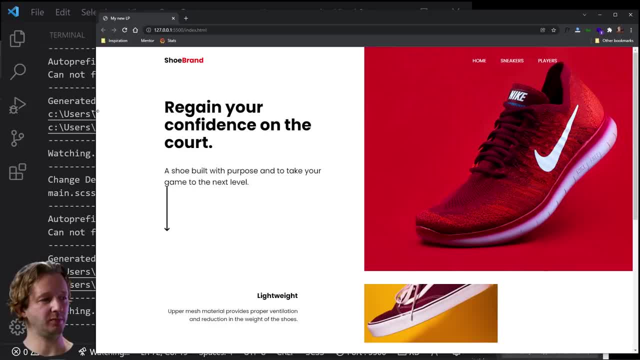 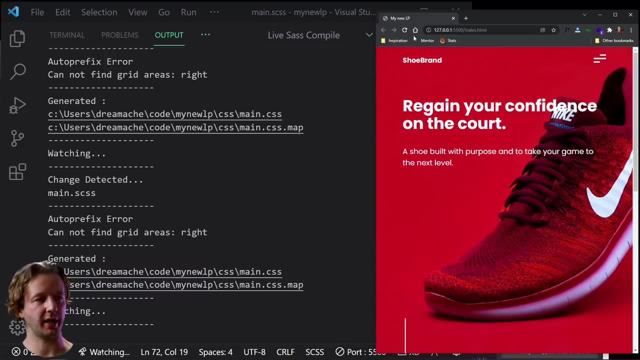 Because of my green screen in the background, It's getting dark outside. That is it essentially. Looking at this, I kind of don't like the amount of Like if we look at Hold on one second here If I pull this. 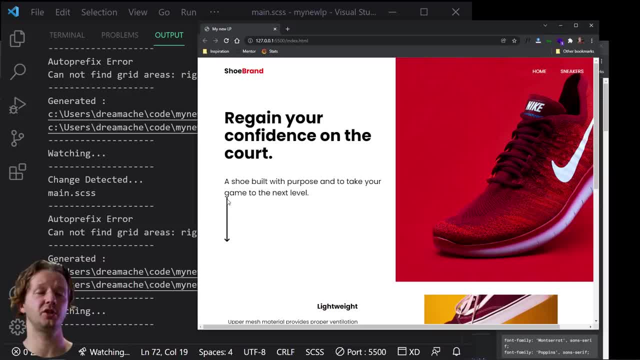 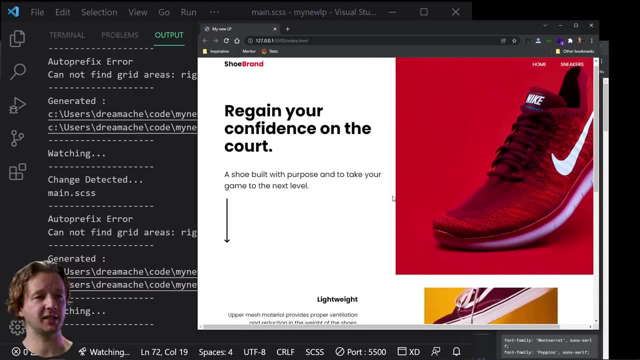 Pull this up. It's kind of going a little bit too close here. So what you would do, You could use margin to push this down In order to get that a little bit better aligned up. I'll let you try to do that. 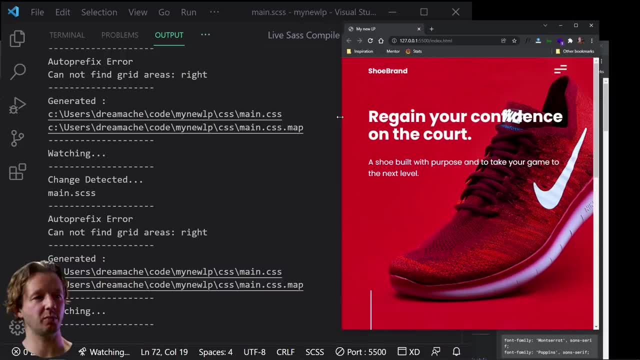 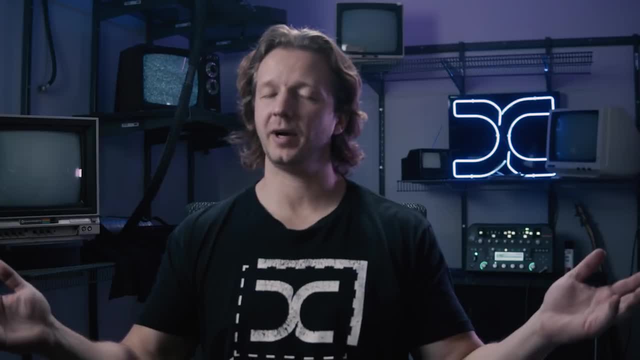 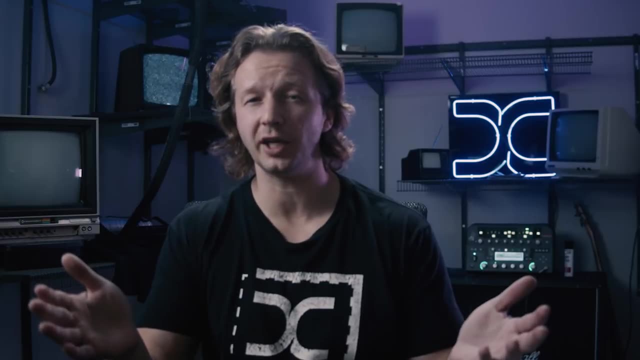 But that is essentially Front end development. Something a front end developer would do To take an existing design And make it a working reality In the browser. Alright, everybody, Hopefully you enjoyed that. You probably have a lot of questions If that's the case. 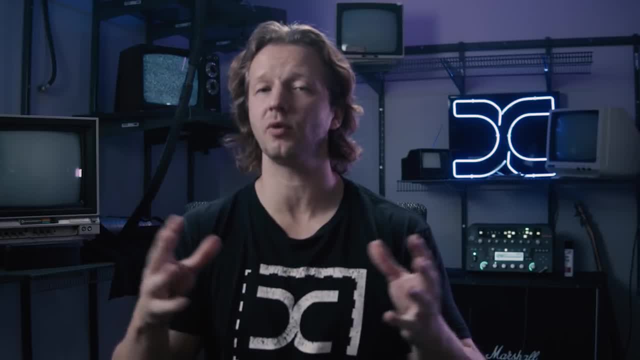 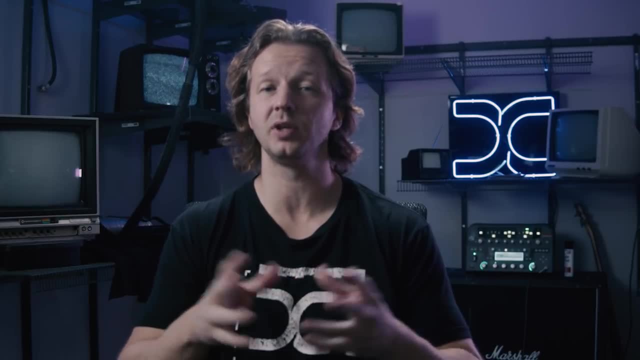 Please visit designcoursecom forward slash CSS To enter your email to be notified When my brand new interactive CSS course releases. And, of course, If you're watching this at a time When it's already released, Please consider joining. Check the YouTube description for any available discounts as well.